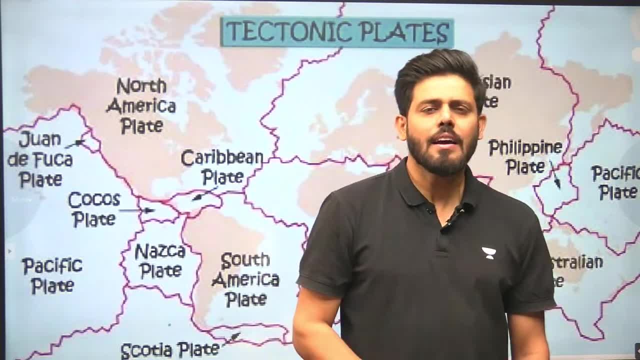 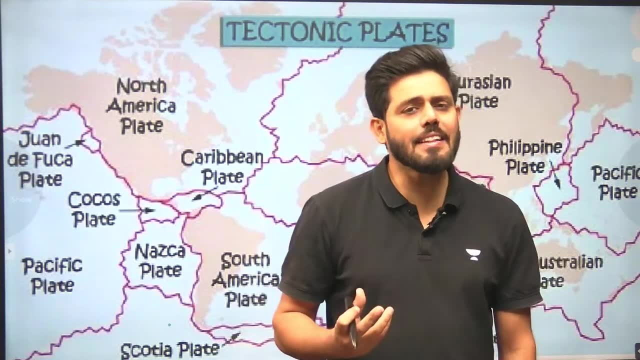 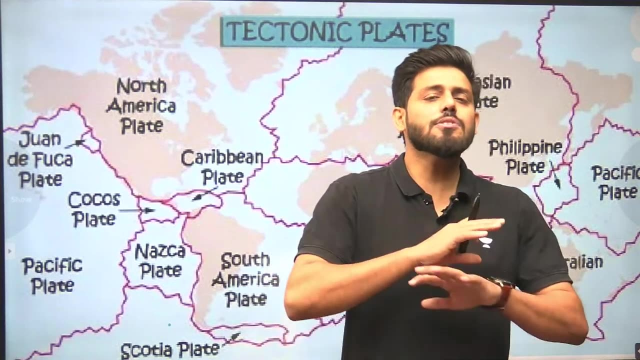 theory. In the last class we had studied continental drift theory in which Alfred Wegener sir gave responsible reasons that our continents drifted. All the reasons and forces were removed from the top. That is why further these theories have come, which we are going to read in detail. 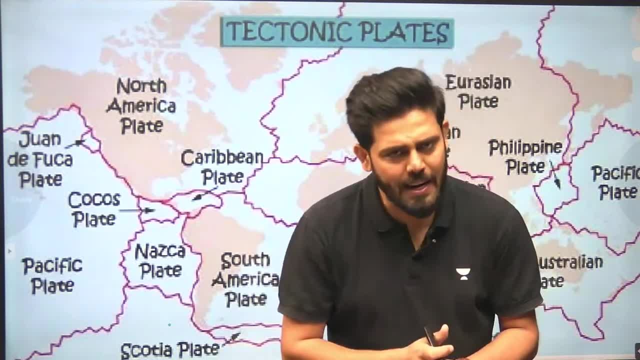 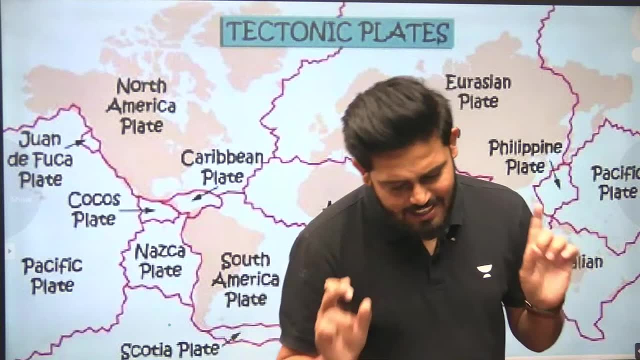 The first one is convection current theory. After that there is sea flow spreading theory, After that there is paleomagnetism and after that there is plate tectonic theory. Today we will cover all these theories in a single session with great detail. So first of all, 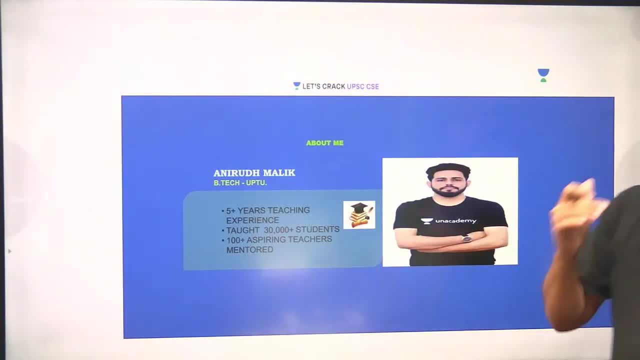 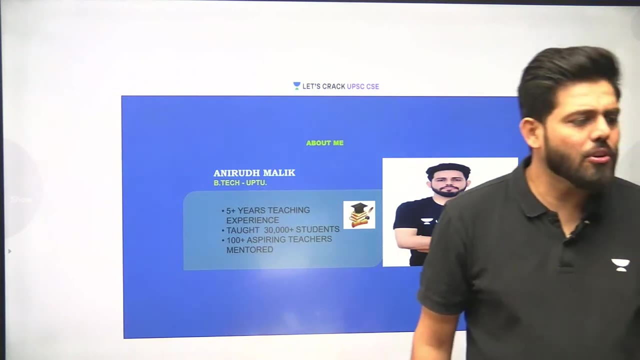 if I talk about myself before starting a session, This is Anirudh Malik. I have a teaching experience of more than 5 years. I taught and mentored more than 30.. I taught and mentored more than 30 thousands of offline students and lakhs of online students. 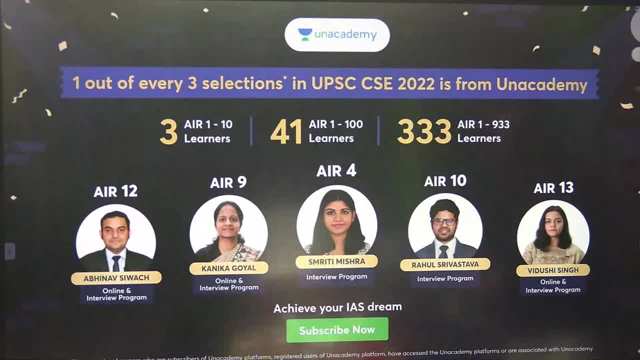 If I talk about further, you know that one-third total selection has been given by Unacademy directly, which were students of Unacademy's plus iconic and last mile program. That means, out of 933, Unacademy has given 333 selections directly. On Unacademy there is an amazing. 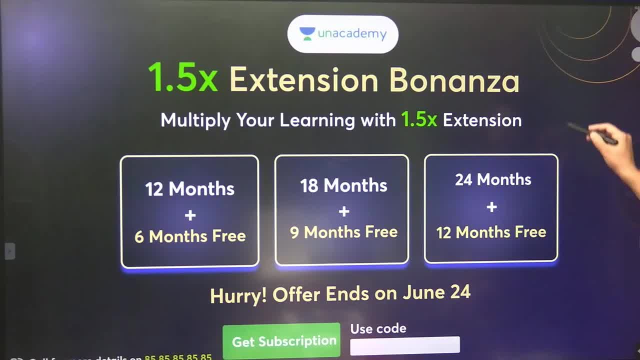 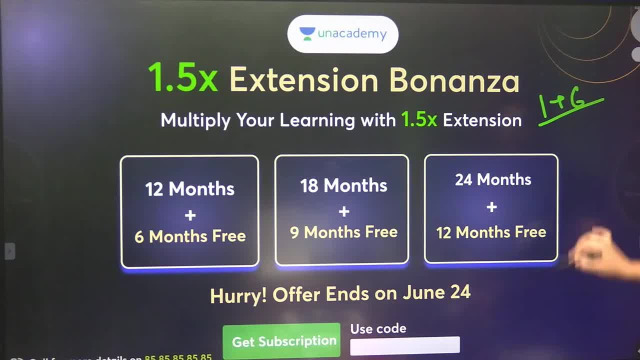 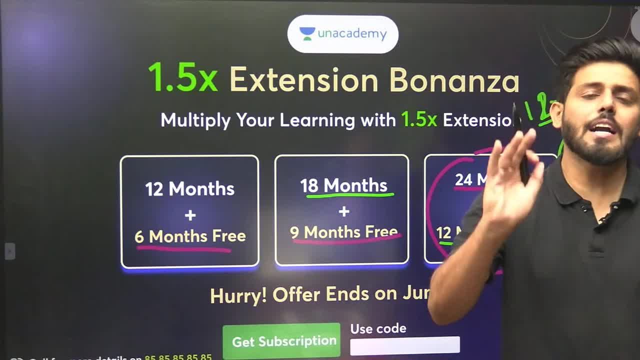 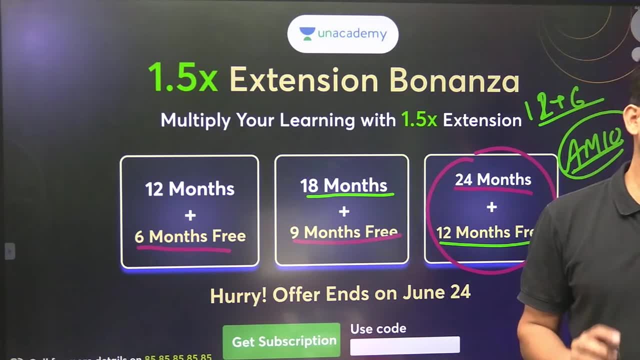 of Loving anyone that you get. your subscription is free For drugs. you can get it for just Rs 16000 and, by the way, if you follow this program, I have separated out everything, including mentorship, guidance, how to cover all the things. 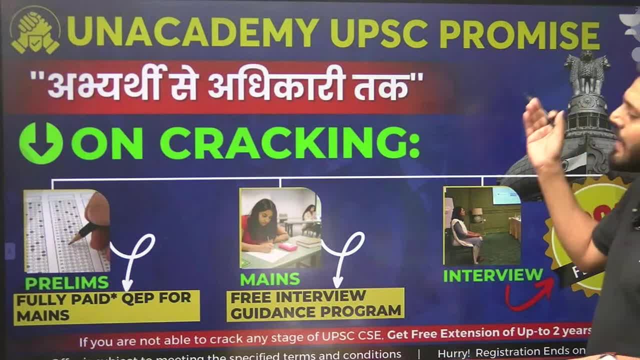 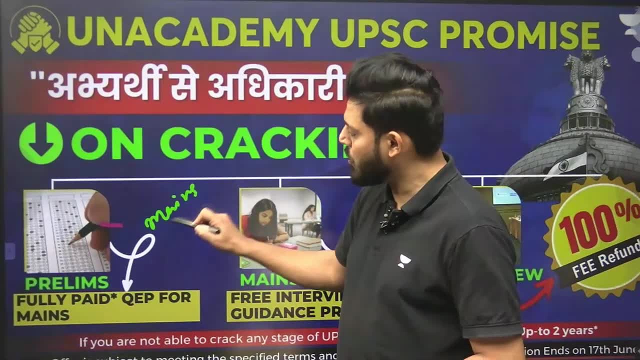 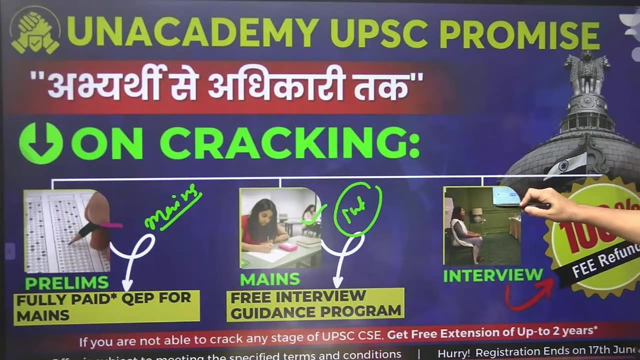 these things are going to be covered there. If we talk about the promise of Unacademy, if your problems are cleared, then you will get to live and eat in the offline center of Delhi. If your MAIS is qualified, then the entire preparation of the interview will be done from the end of Unacademy. 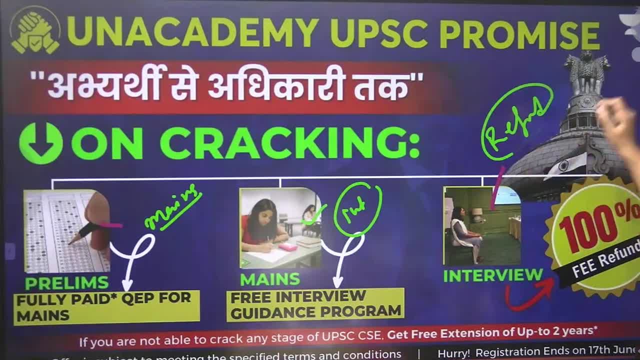 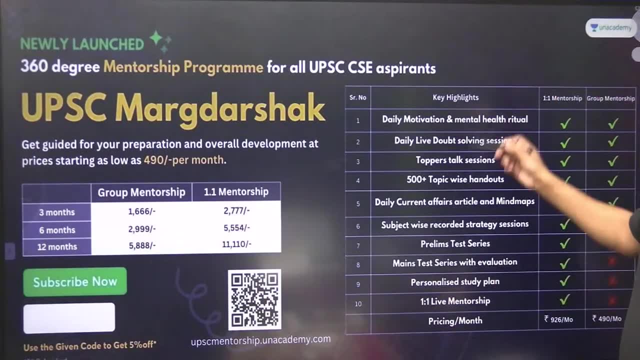 And if the interview is cleared, then your entire money will be refunded. That means you are going to get complete things. Guys, there is an Unacademy UPSC Mark Dashak program for you In which you will get two programs of group mentorship and one-to-one mentorship. 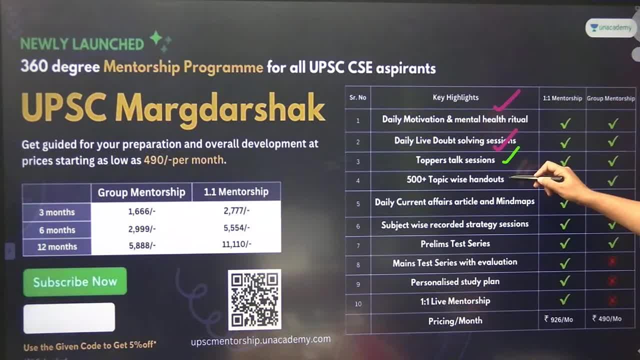 In which you will get daily motivation, daily doubt, solving topper stock- 500 topics. you will get handouts daily current affairs, subject wise recorded strategy session. personalize: You are going to get mentorship in the group and one-to-one. 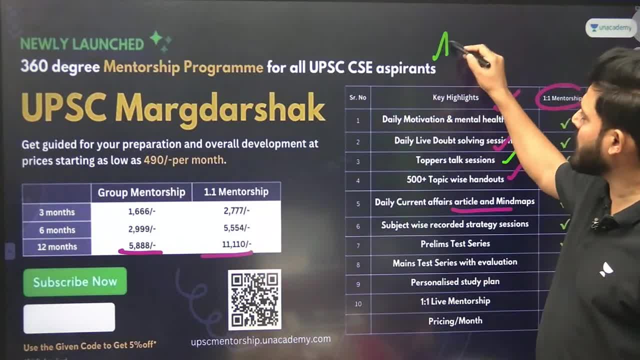 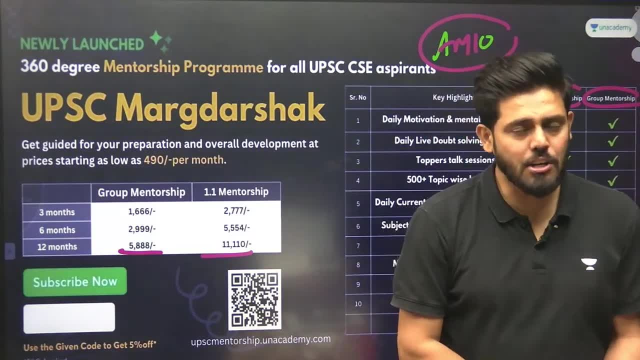 The price of both is the same. And the price of both is the same. You can take this Mark Dashak program by using the AM10 code And you know that my free mentorship program is going on Sankalp Mentorship Program, which is on the Unacademy app. 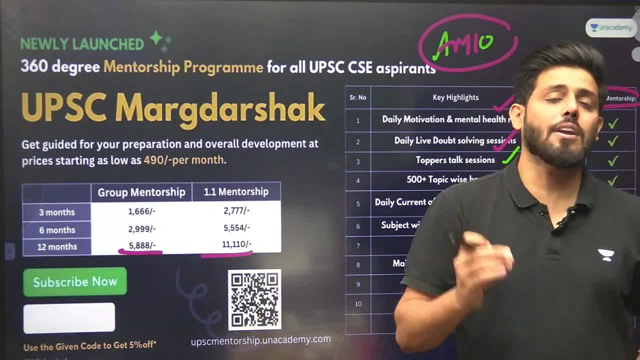 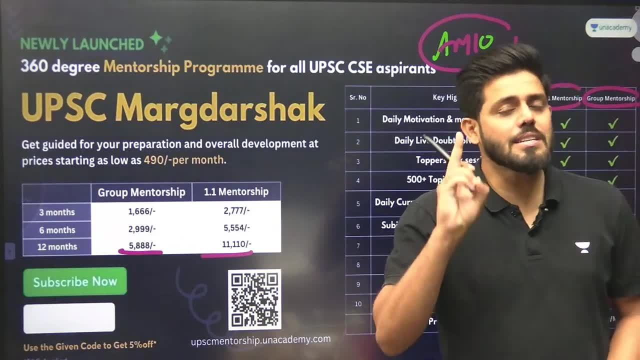 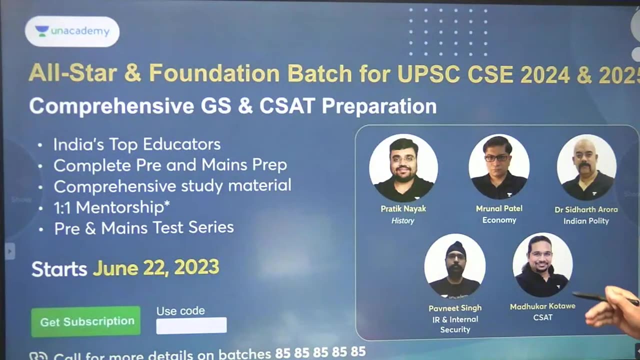 Daily. we meet you at 12 noon Where we solve the questions of top quality MC, And that session is covered in great detail, So you don't miss those things in any way. You can join things by using AM10 code. Guys, from 22 June the foundation all-star batch is starting for you. 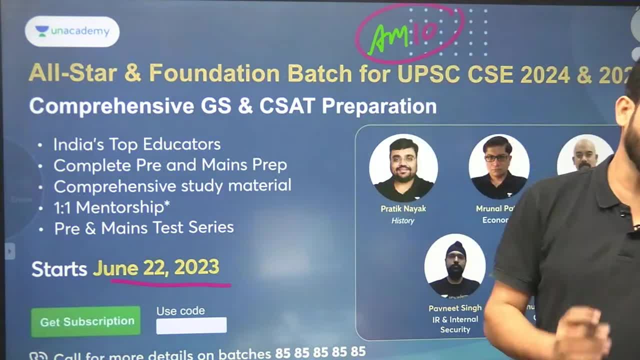 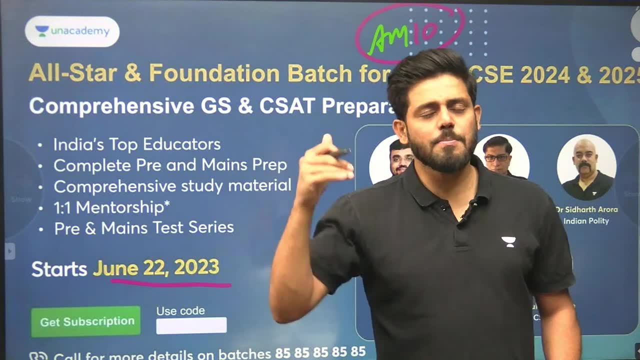 In which, if you take subscription by using AM10 code, Problems mains option interview, You will get all the things in one place. You don't need to go anywhere. You will get complete coverage with great detail Along with that, what you have to study, with which approach you have to study what should be the understanding. 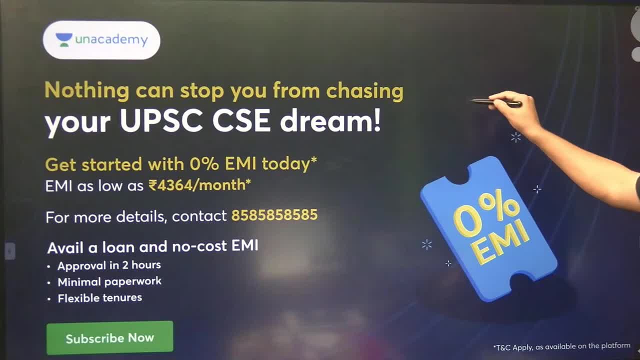 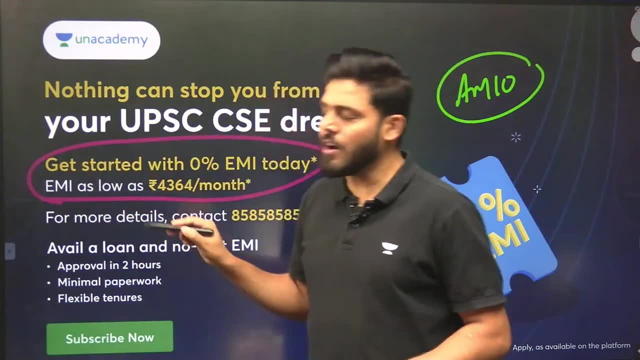 In all those things you are going to get help from my end. There. you can also take through EMI, But remember you will get the loan at a very nominal price And the most important point is that it is going to be interest-free. 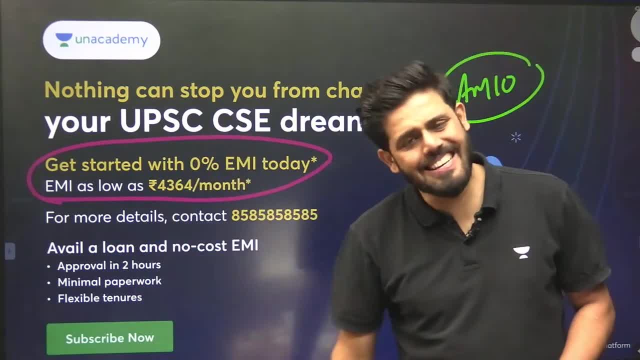 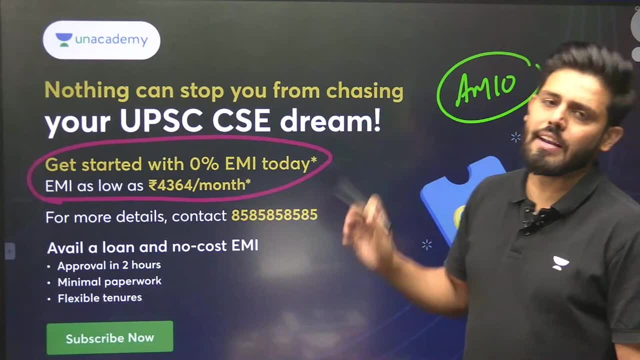 There are no extra charges. You can take it very easily in EMI And every student will get the loan. No such thing is necessary. There should be a very good earning. You can contact me regarding any doubt regarding the loan For subscription. that is unacademy__anrudmalik. 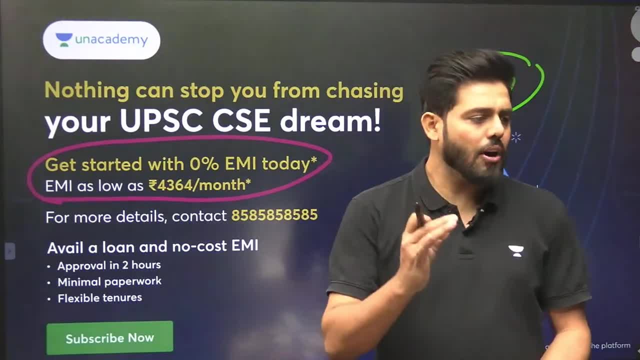 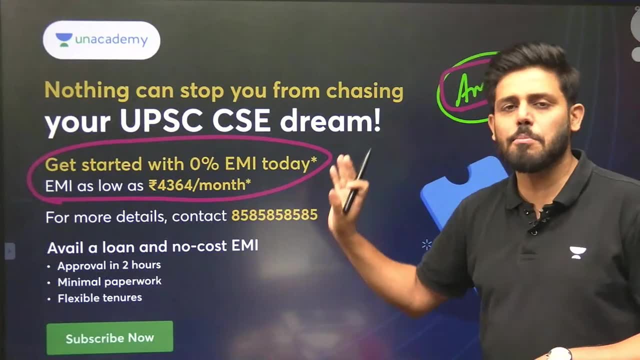 This is a telegram channel where you will get my contact number And you will get help with things There. you will get discount with the use of AM10 code, Plus mentorship: Talk to the sales team because many students face issues After subscription. 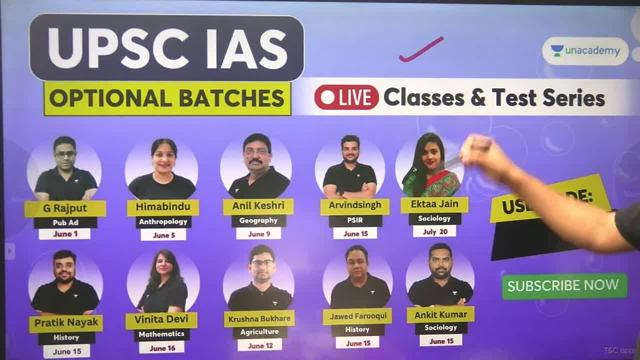 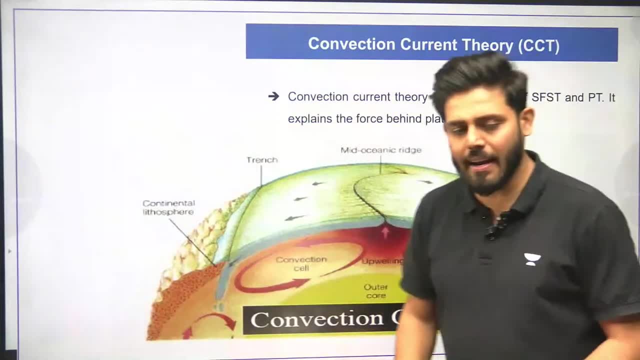 You will get all the optional batches in one place. There is no need to go anywhere. Plus, you get combo subscription as soon as you enter the code. Now we come to the topic in which we talk about our conceptual clarity. Quickly, all the students like the video once. 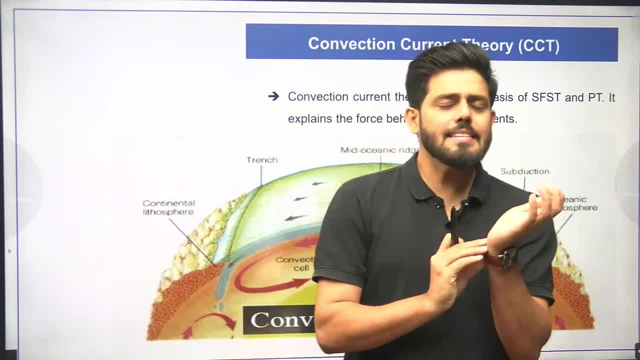 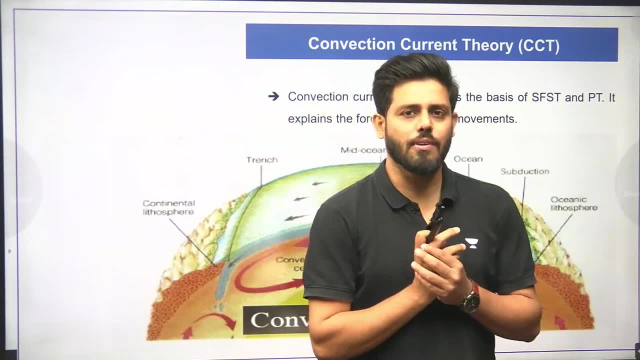 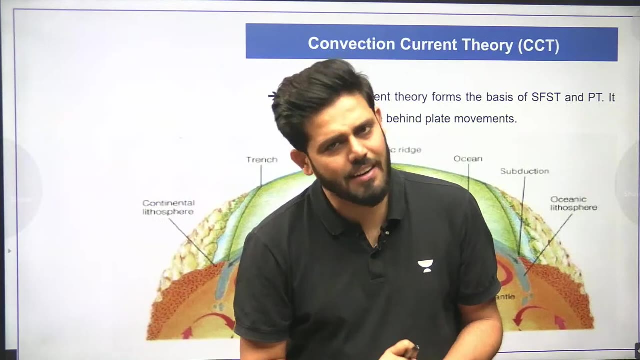 Share it, Because then we are starting things. Guys, see What was the problem in front of us? I will cover things very easily and with each point. That's why I want all the students to watch this video till the end. Today's content is going to be around 75 to 80 minutes. 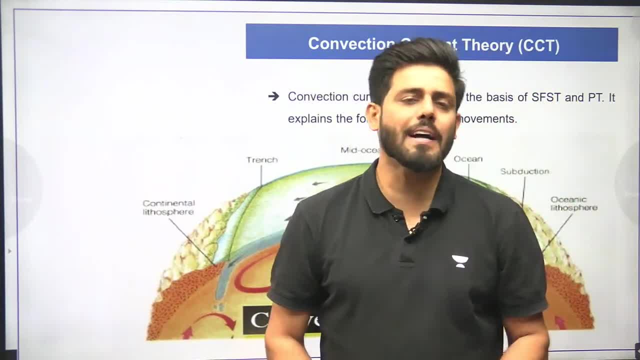 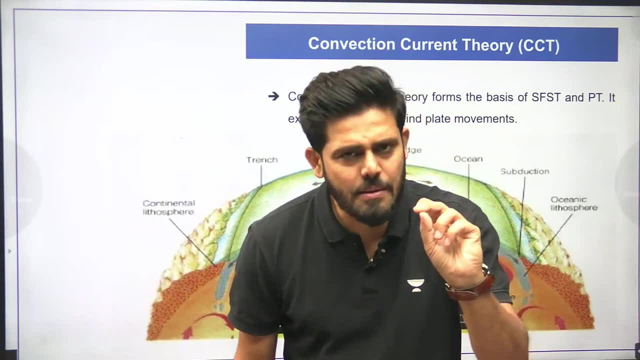 Because I will cover three theories, Especially if I talk about four, In which I will talk about convection, current theory. Along with that, I will talk about sea flow spreading theory. I will talk about paleomagnetism, Which is the magnetic polarity of our earth. 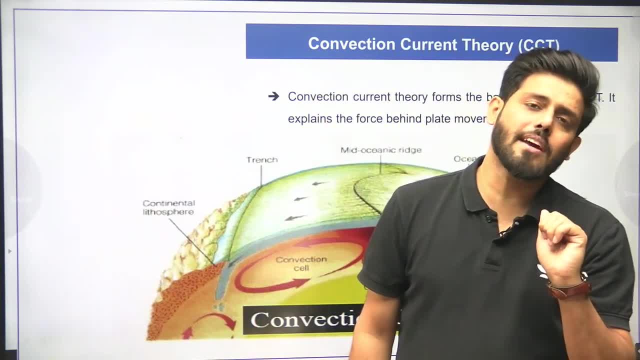 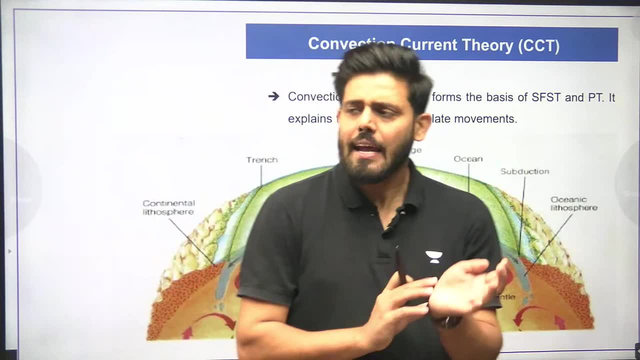 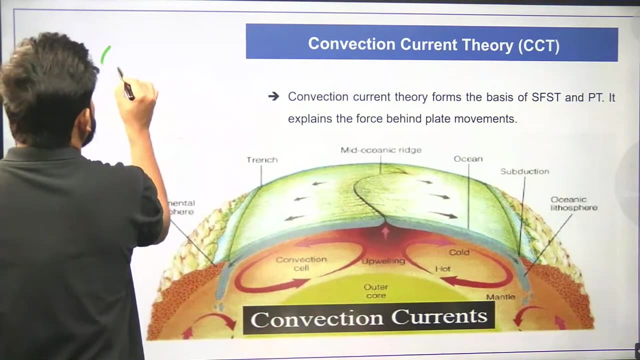 And in the fourth theory I will talk about plate tectonic theory. We will understand all these theories very well, one by one, So without any delay. First of all, I will tell you things to make your understanding better. In the last class, I told you about continental drift theory. 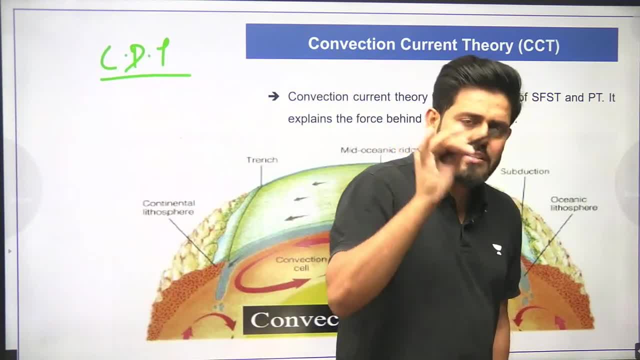 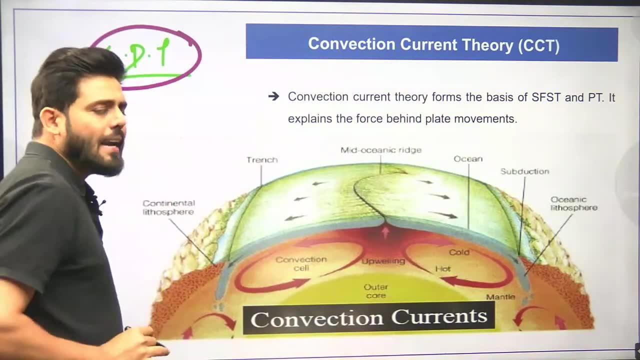 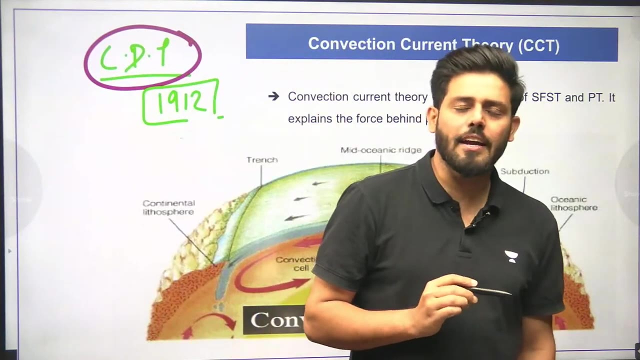 The students who are completely new. Once you see this theory after this session, Then you will get more conceptual clarity. Our continental drift theory In this. I told that in 1912.. Alfred Wagner told that our continent. Why are they drifting? 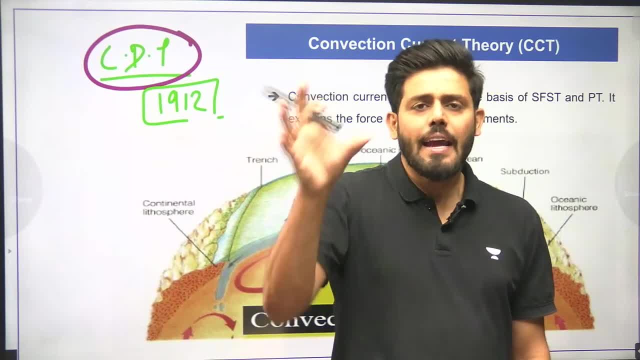 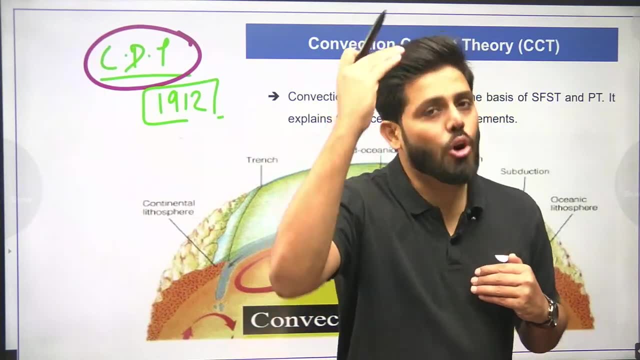 He told that 200 million years ago There was a single land mass whose name was Pangea, And that Pangea broke And with that your Angara land, Which is called Laurasia, And the southern portion is called Gondwana land. 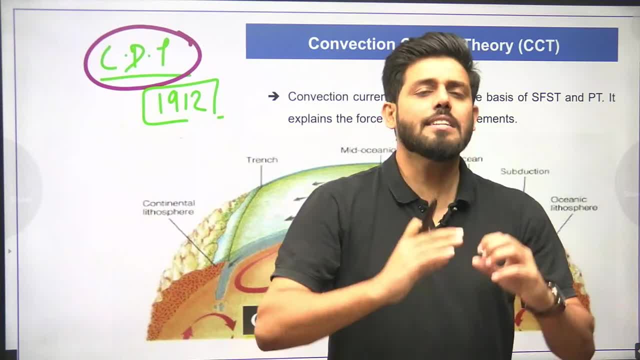 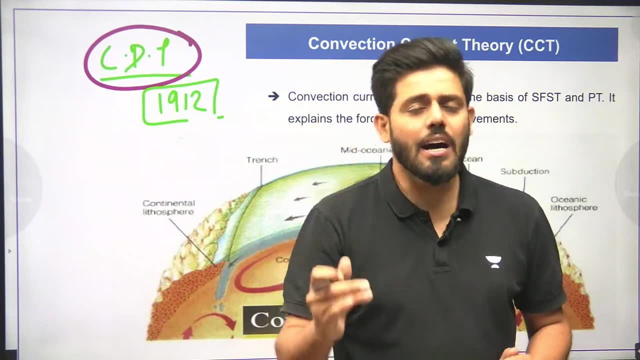 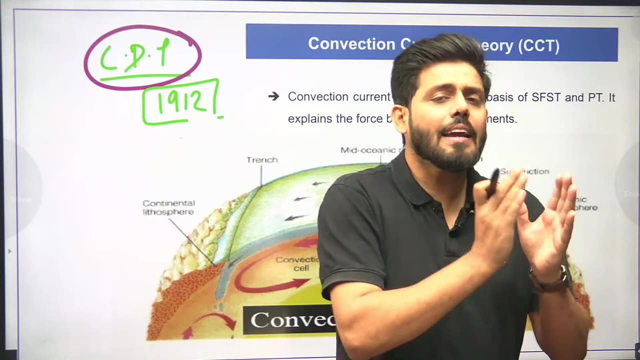 And after that they started to further split, Due to which, at present time, Different continents were formed: South America, North America, Eurasia, Asia, Australia, Antarctica and Africa. All these continents- Our continental drift theory, told That this continent was previously a single land mass. 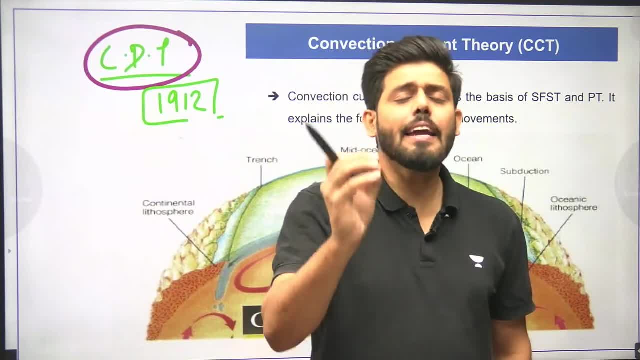 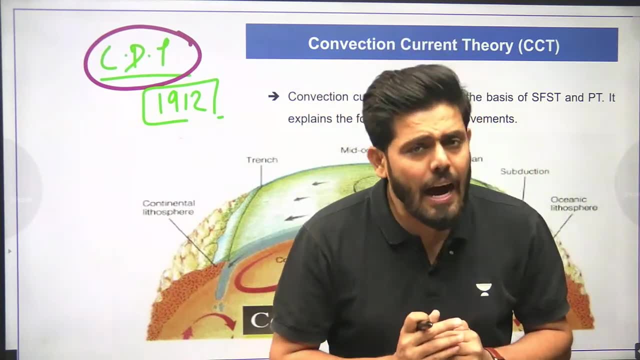 But they were asked That you tell me That these continents, Which you have told That they were previously a single land mass, After that they have broken separately. What is the reason behind this? Why have they broken? Which force is responsible? 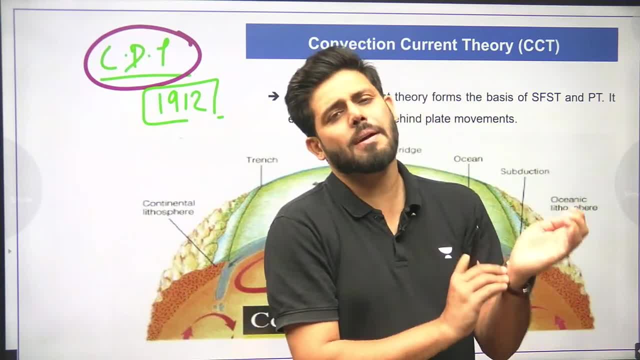 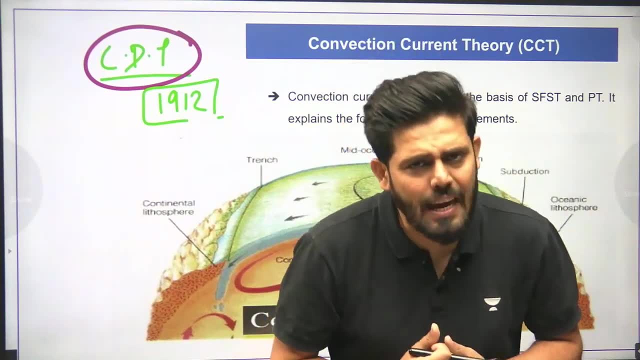 Due to which these continents have broken. Alfred Wagner told There is a buoyancy force And there is a tidal force, But our great geographer At that time, They have explicitly denied That, your buoyancy force And tidal force. 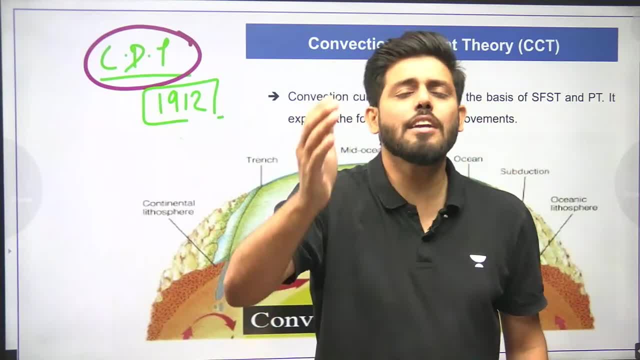 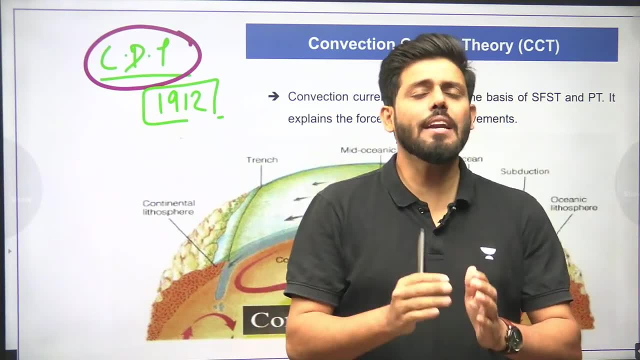 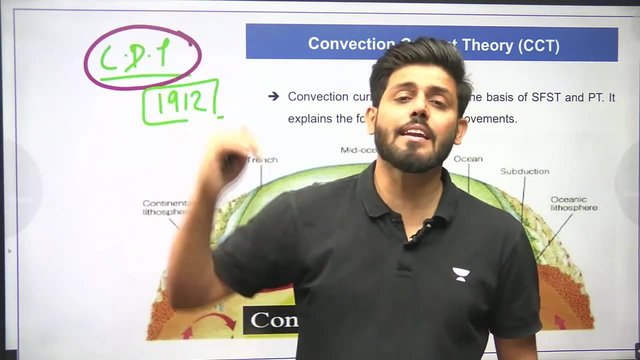 Tidal force is not that strong, Our gravitational force Of sun and moon Is not that strong, Due to which our continents drift. So their theory Was denied, But this theory Was a very important theory. This theory opened The ways of the future for us. 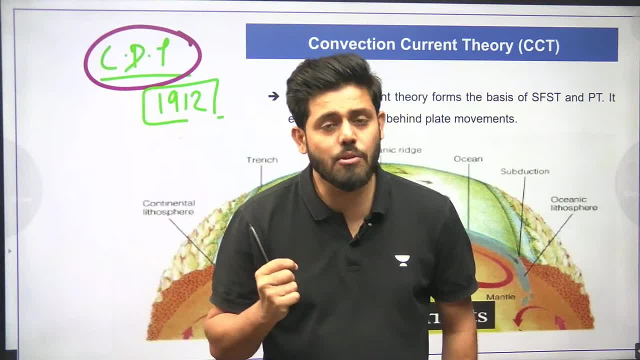 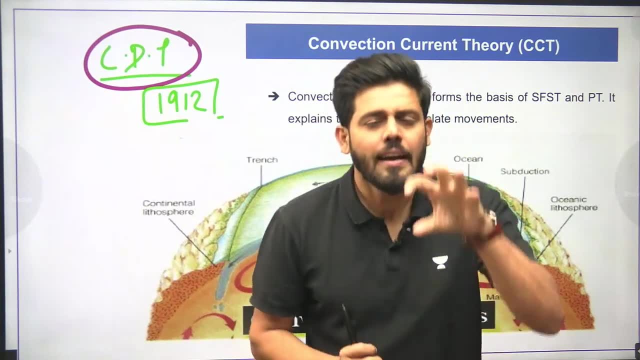 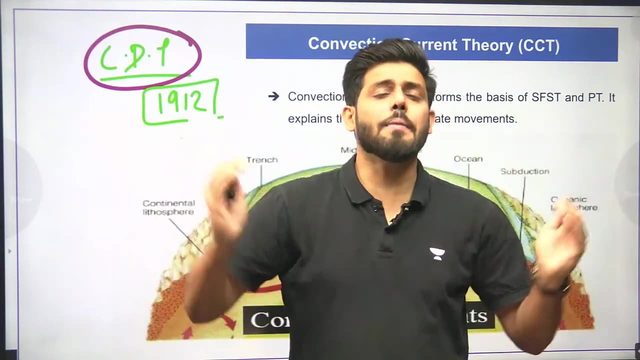 This theory has opened The ways of the future for us and expanded our future aspects. This theory said that one thing is absolutely right: that our earth used to be a single land mass which was called Pangea, and from that only our continents have been made different. 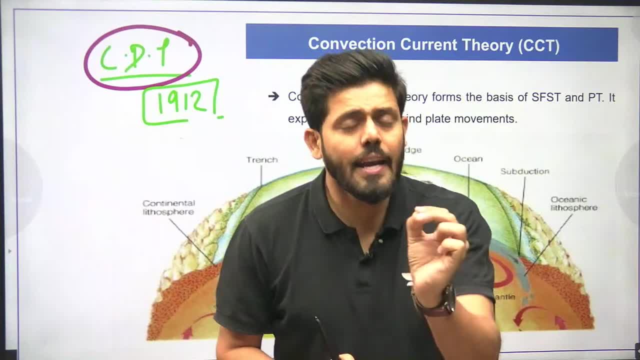 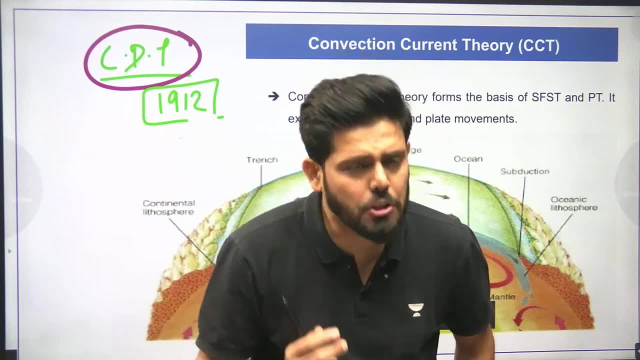 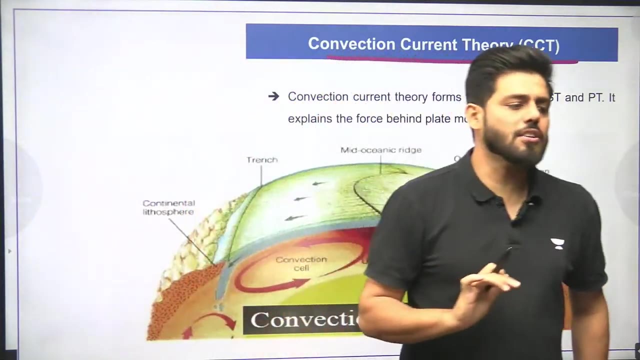 But no one was able to tell why they have become different. Which forces are responsible behind them? Regarding this, the first and most acceptable theory came. That theory is called Convection Current Theory. I will explain you very well about this. What is Convection Current Theory? 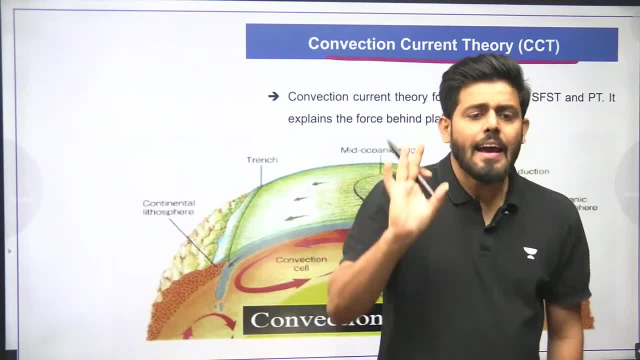 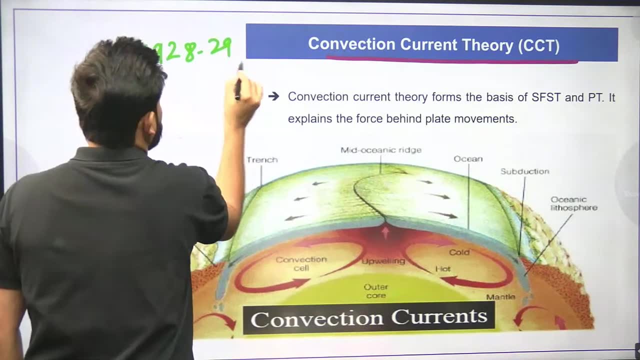 It is very important to try to understand. Is it clear, What is Convection Current Theory? Sir, it is a matter of many years before today, of 1928 and 1929.. There was a geologist whose name was Arthur Holmes. 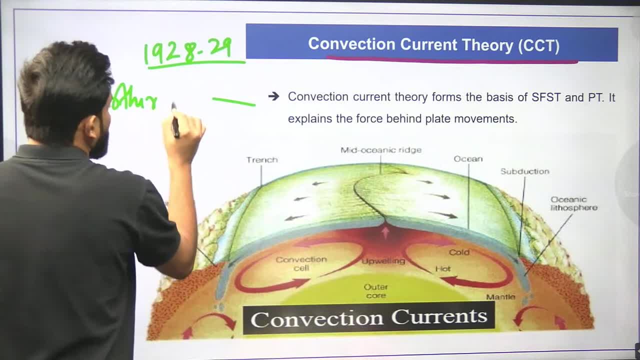 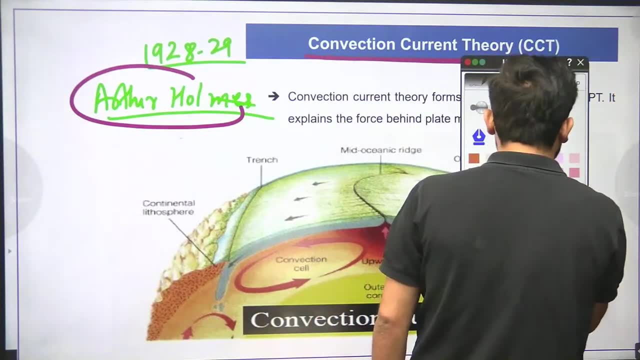 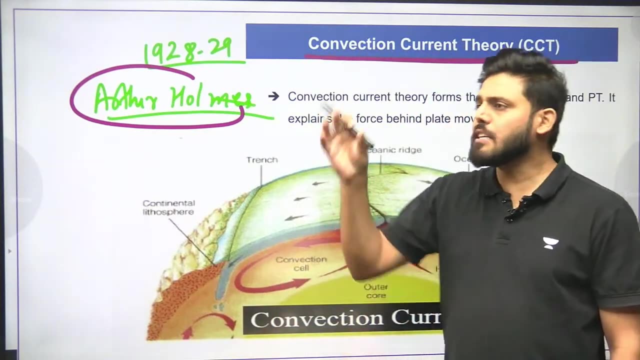 Remember there was a geologist whose name was Arthur Holmes And this Arthur Holmes brought a theory which was called Convection Current Theory. What did he try to explain? Try to understand it with me. Arthur Holmes, who brought this theory, wanted to tell that what is the reason behind the volcanic eruption on our earth? 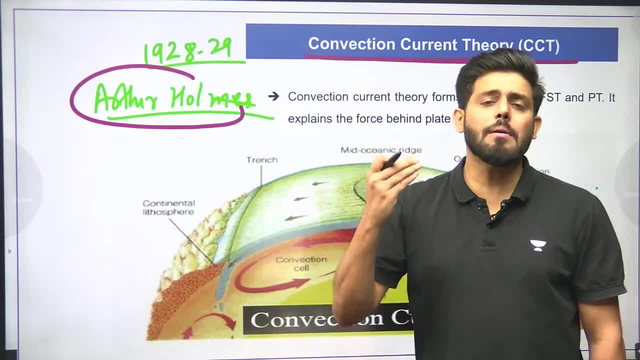 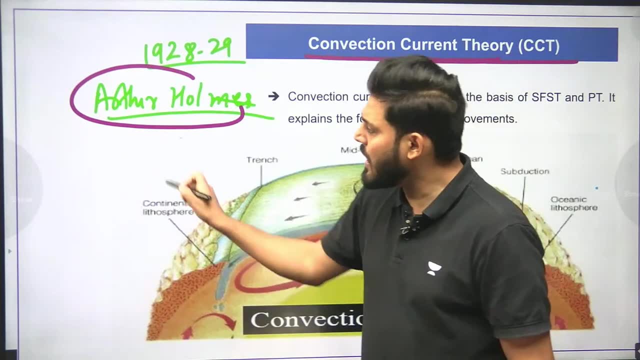 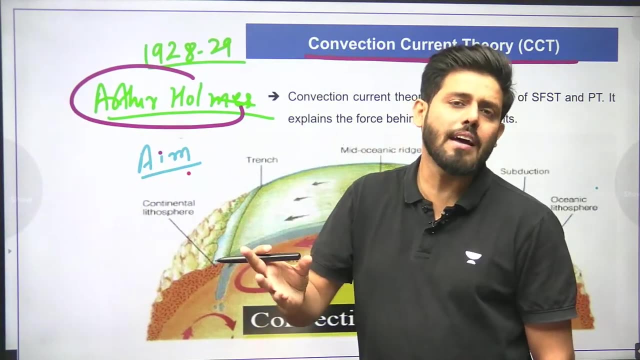 Along with that, Arthur Holmes wanted to tell that what is the reason behind the mountains on our earth? And the aim of Arthur Holmes was to solve the mystery of our study of volcanism. What is the reason behind it And how is the origin of our Fold Mountain? 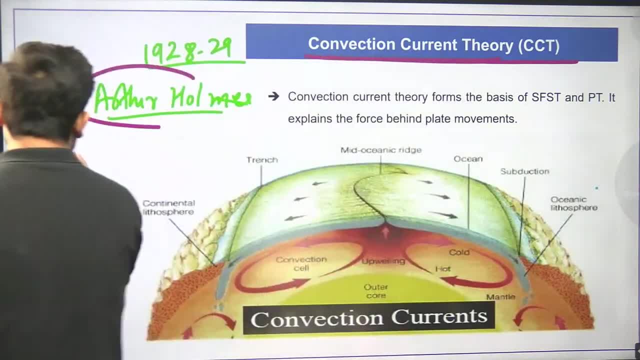 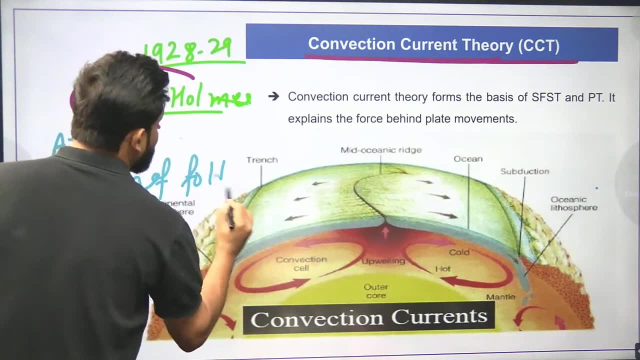 So remember the origin of the Fold Mountain. What was his aim? If I ask you, tell me, Sir. the aim was to explain how the origin of the Fold Mountain happened, How our Fold Mountain was formed. He wanted to explain this thing. 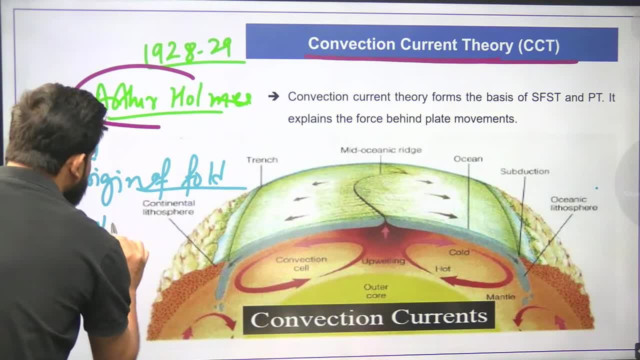 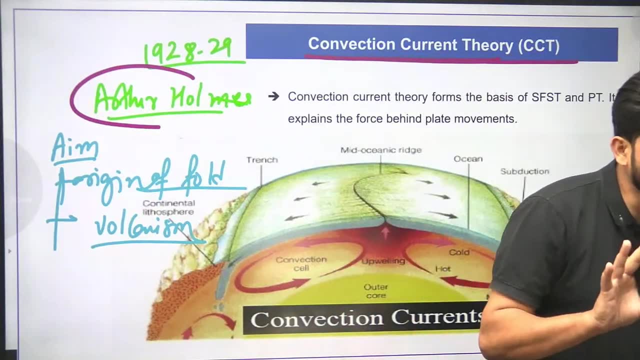 What else did he want? The other thing he wanted was: what is the force responsible behind the volcanic eruption? There must be some forces right From where the volcanic eruption is happening. Did you understand? So he wanted to explain those things. 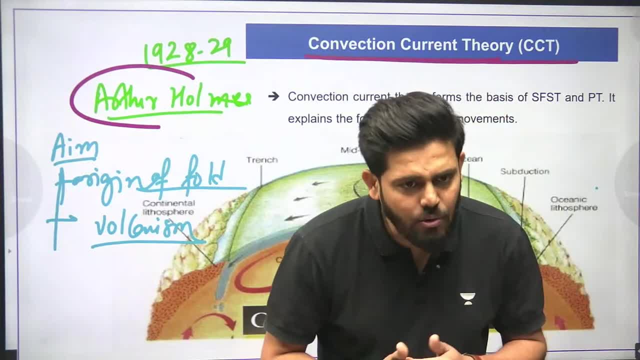 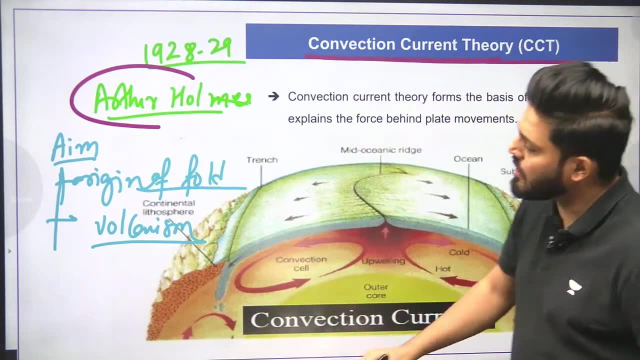 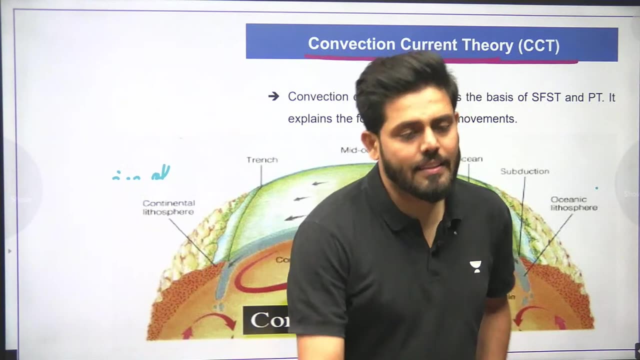 Did you understand Now what happened As things progressed? Arthur Holmes brought a very good theory: Convection Current Theory. Now let's talk about what he wanted to explain. in Convection Current Theory, Arthur Holmes explained very well that Look at our Earth. 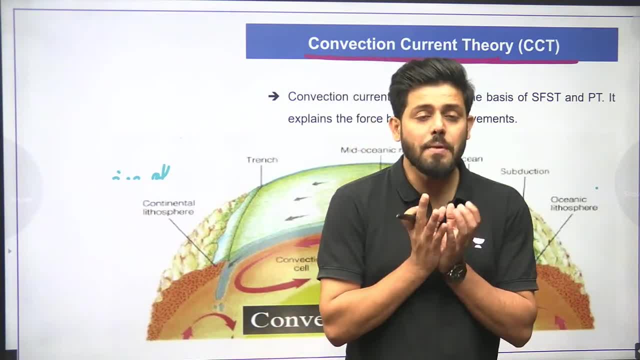 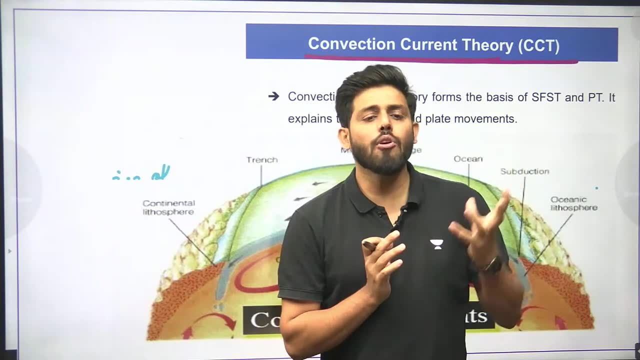 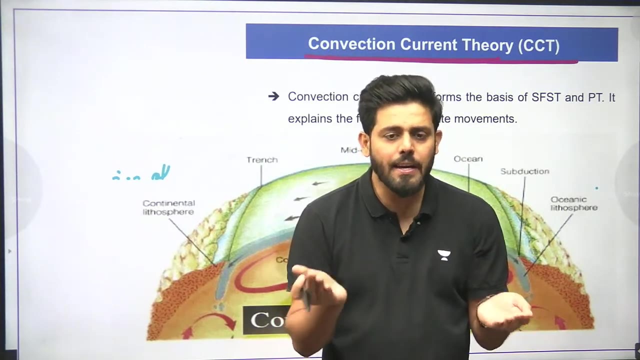 Try to understand. He tried to sort out the major relief features on our Earth, How volcanic mountains were formed, How our Fold Mountain was formed. He tried to explain these things. Who did he? Arthur Holmes. He said that the driving force behind the formation of the mountains 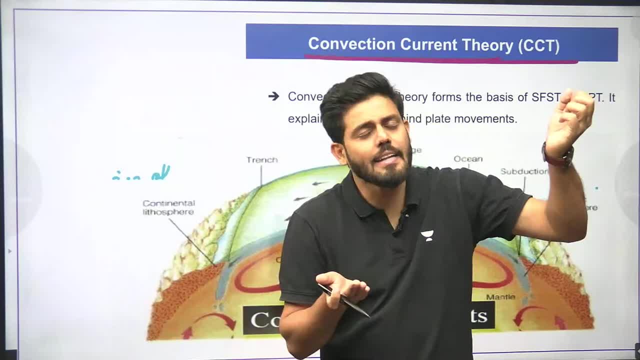 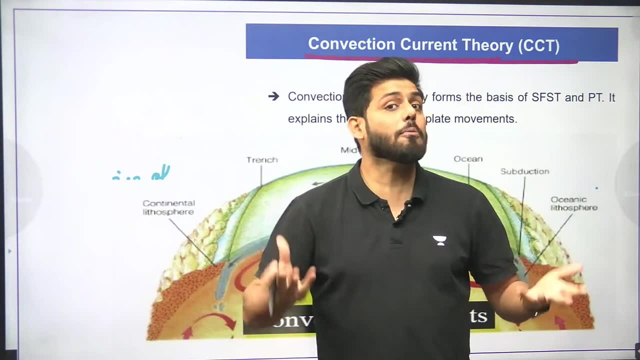 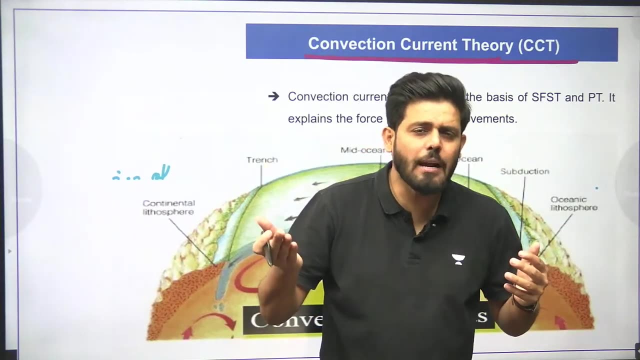 the responsible force, the polar feeling force, which Alfred Wagner had mentioned, was to drift the continent. But he is telling us how the continent drifted And the different relief features behind it: the mountains, the Fold Mountain, the volcanic eruption, the Rift Valley. 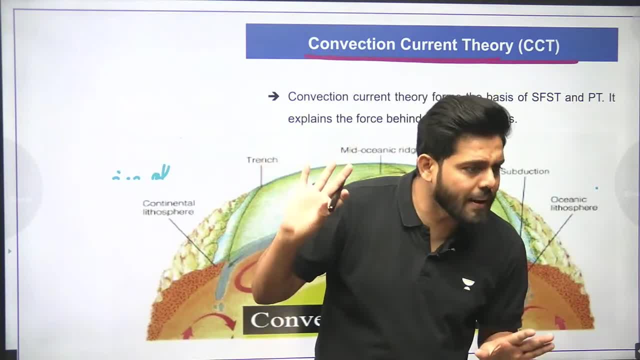 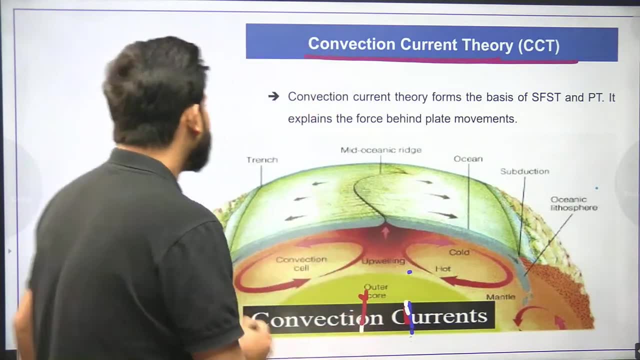 What is the responsible factor behind them? These things have also been explained by Alfred Wagner. You have to understand this. Alfred Wagner said that: Look, we know that the interior of our Earth is the interior of our Earth, The top layer of our Earth. 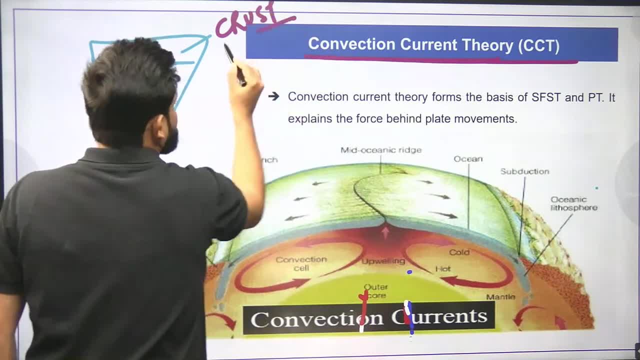 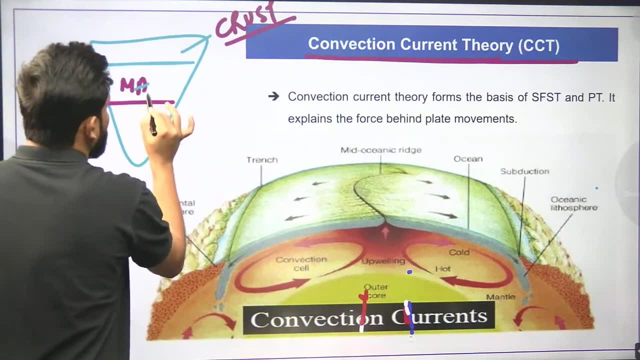 we call it the Crust. We call it the Crust And along with that I told you that the second layer after the Crust is called the Mantle, And you all knew that. the top solid portion of the Mantle below the Crust, 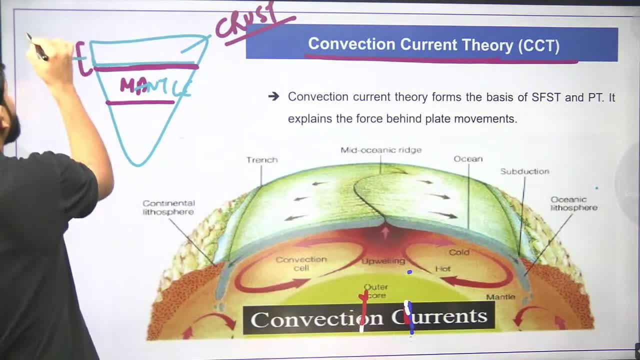 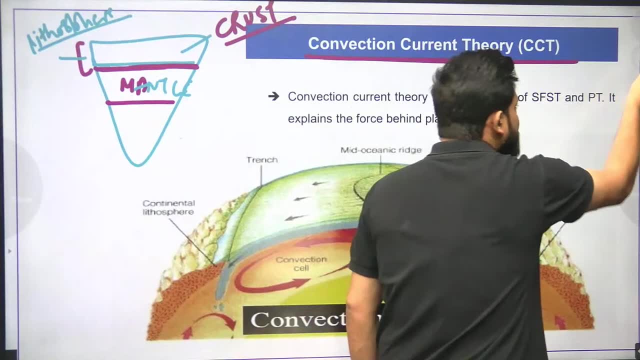 is this one. This is the solid portion, Plus by combining the Crust, we call it the Lithospheric Plate. Lithosphere, That means our plates are the Lithospheric Plates. And after this he told us that 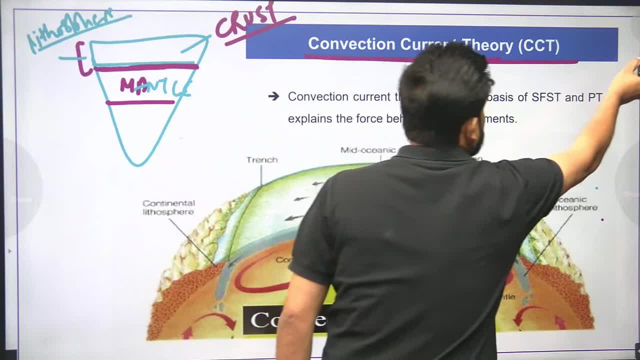 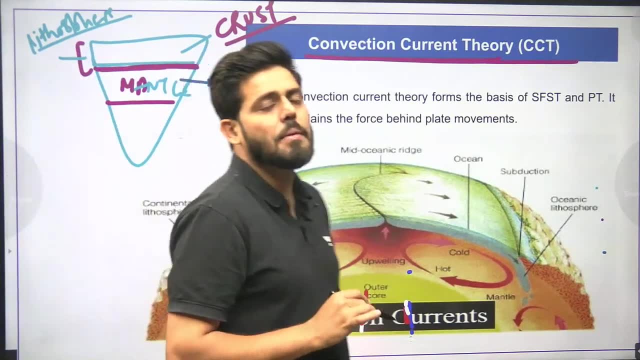 the interior of our Earth, the portion below it. he called it the Mantle. What did he tell you, guys? He called it the Mantle. And then he told us that the Mantle in the interior of our Earth there. 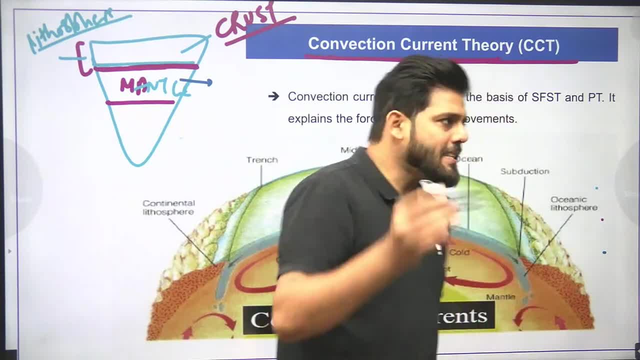 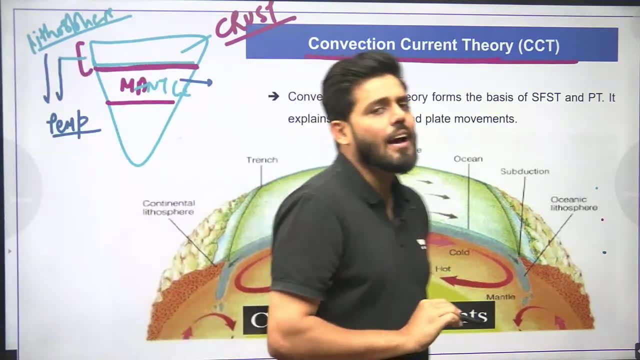 our temperature is very high. That means as we keep moving in the interior of the Earth, our temperature is increasing. So he told us that due to that high temperature, there are radioactive elements in our Earth. There are radioactive elements in our Earth. 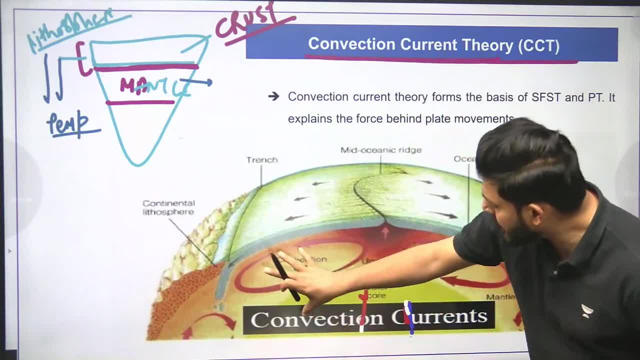 And when there are radioactive elements in the Earth Due to the high temperature. Since their temperature is high, These radioactive elements are starting to heat up. Their temperature is increasing. As a result, the heat in the interior of the Earth is increasing. 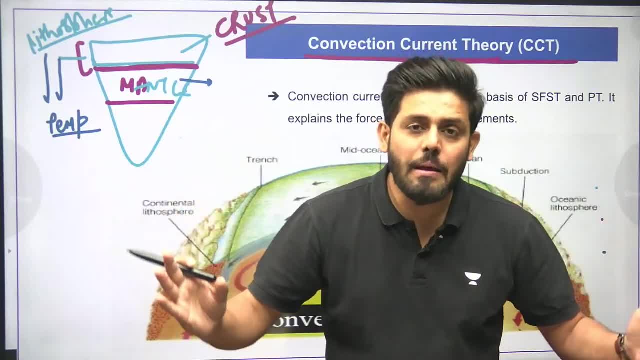 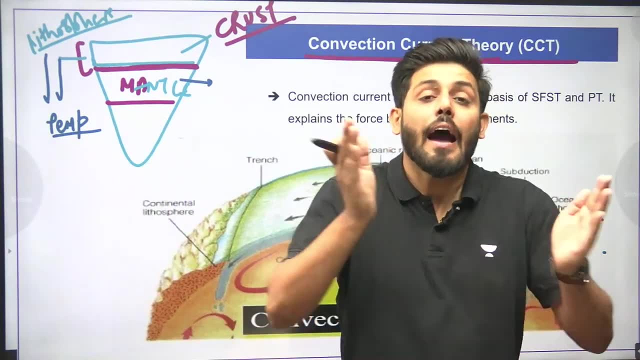 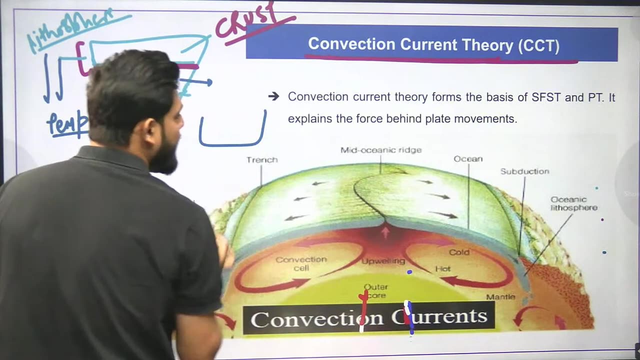 It's getting hotter, Whether in T Windows or in modified theatre. Your very nice concept, And you must have seen one: Guys, if we have this water, Okay, We will set it on fire from under. it assume We will set it up on fire. 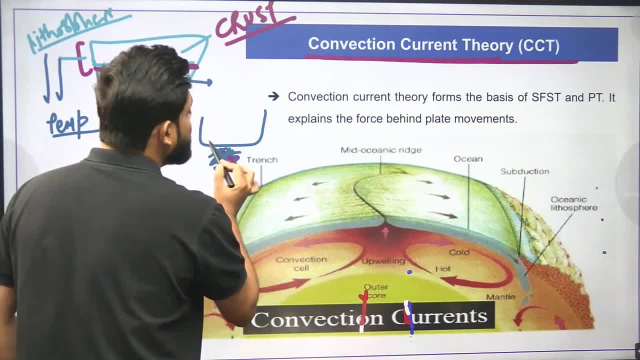 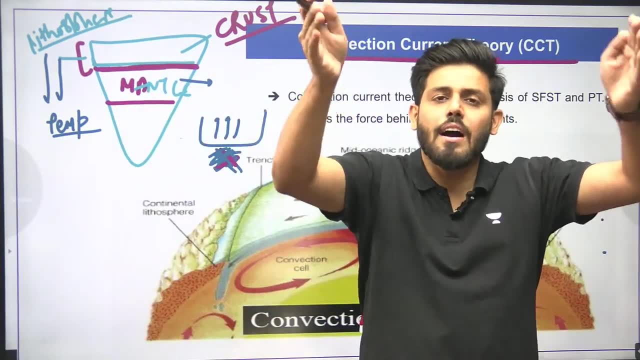 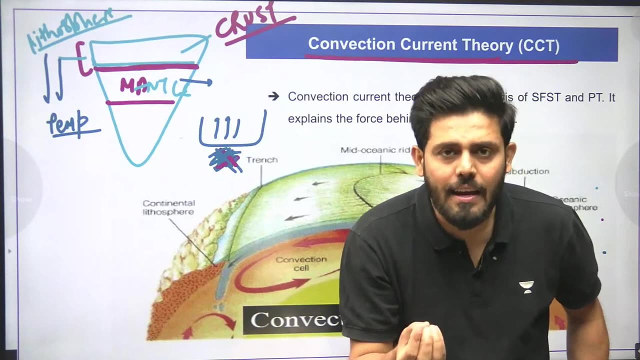 Okay, All right. So you will see that the water will rise upwards and become hot. The hot water will start going upwards and the cold water will start going downwards. Convection will happen in the same way when the temperature on the equator is the highest on the Earth. The temperature on the equator is the highest. So what does our warm air do? when it is hot, It rises upwards. What does warm air do when it is hot? It rises upwards. Similarly, the interior of the Earth is heated due to the heat generated by the radioactive elements of the rocks. 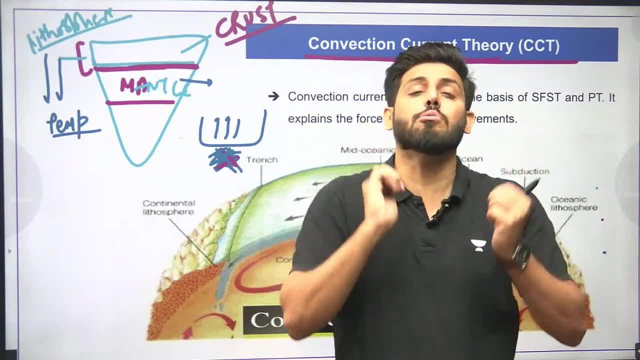 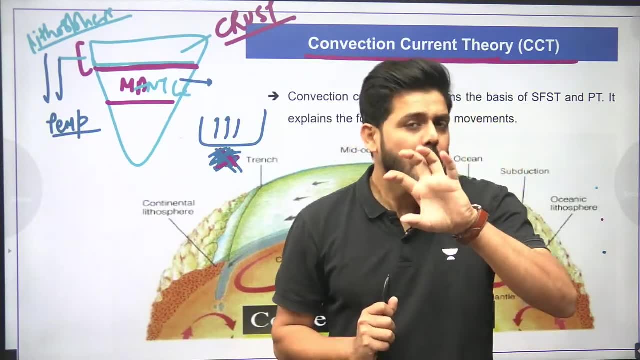 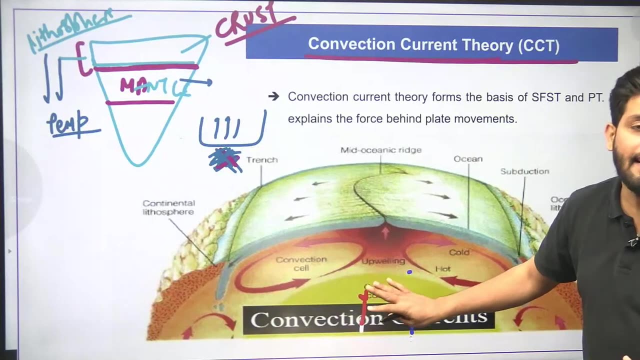 Convection current is generated due to the heat generated by the rocks. Alfred Wagner said that the continents are drifting, but he could not explain the logic behind it. He was explaining the logic behind drifting. He said The interior of the Earth. as we go downwards in the mantle, the temperature is increasing. 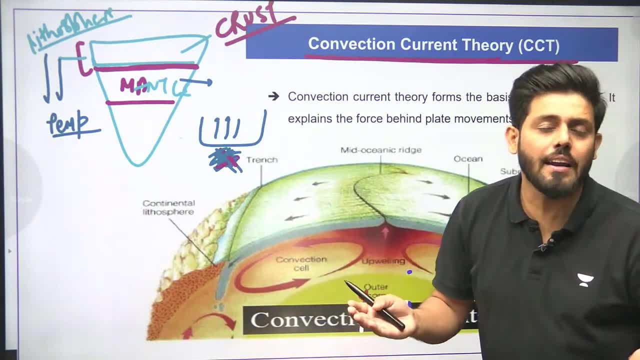 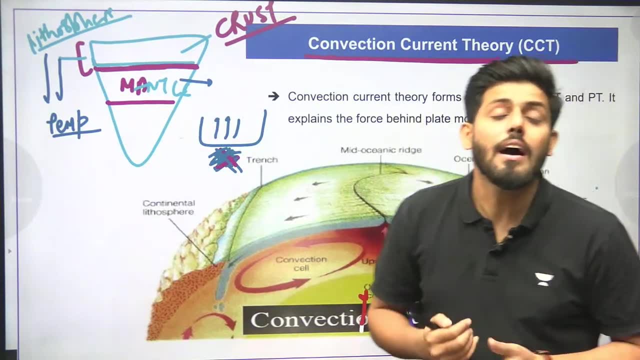 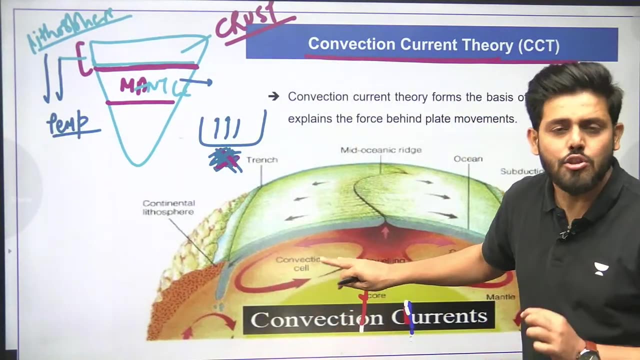 Due to the increase in temperature. the rock is getting hot and melting, The temperature increases, the heat increases and the convection current starts to form Along with this. Arthur Holmes said one more thing: The radioactive elements that I have explained in the mantle. more than that, the radioactive elements go to the crust. 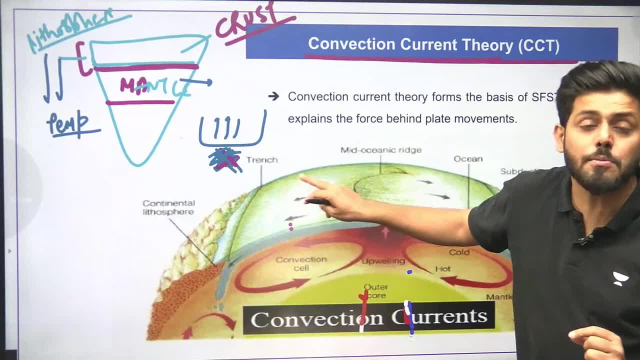 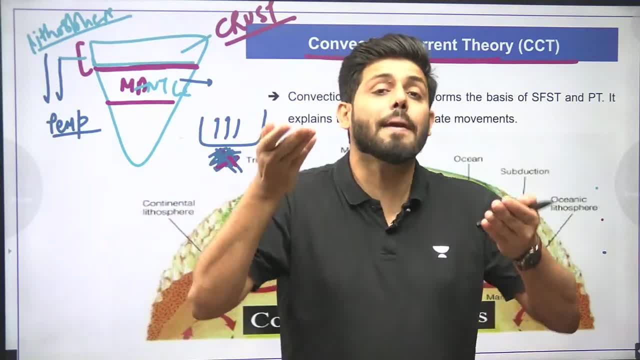 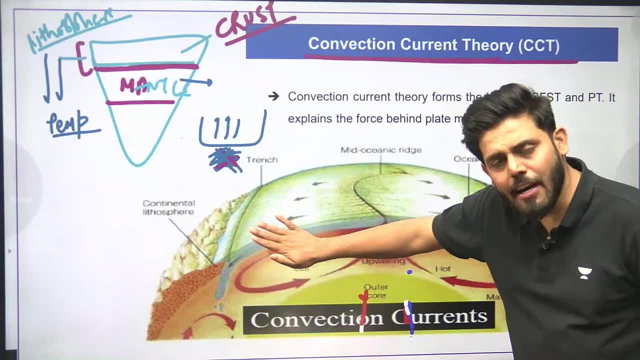 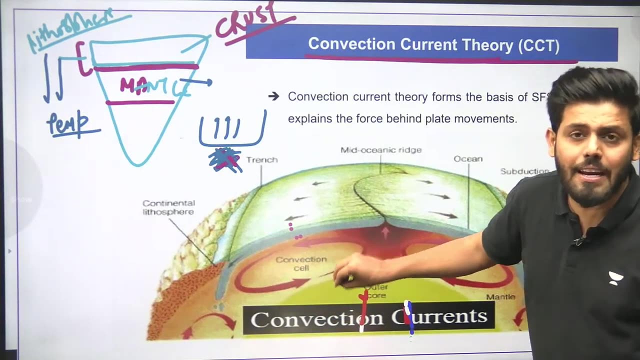 is not so high that the temperature of the radioactive elements increases and the reactions start happening between them. That means he said that our radioactive elements are also present in the crust, But the temperature in the crust is not high. This is why the temperature of the radioactive elements in our mental is high. 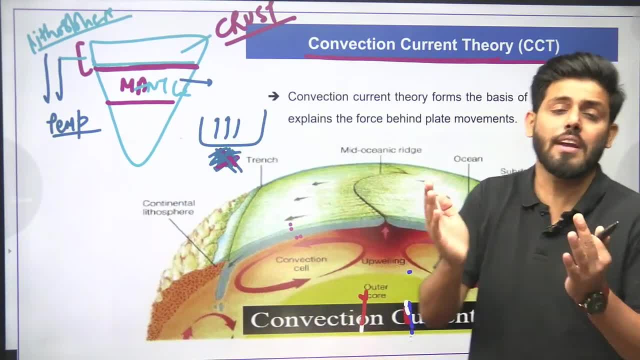 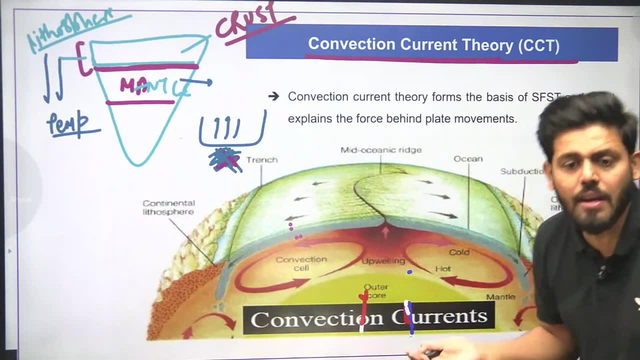 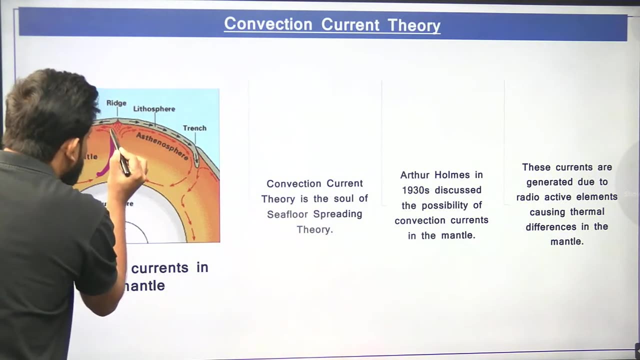 and due to coming in the molten form that convection current is being generated, The things that are hot will start coming upwards. Try to understand. So he said that the things that are hot will come upwards and that is why he said that the magma inside us is rising upwards. 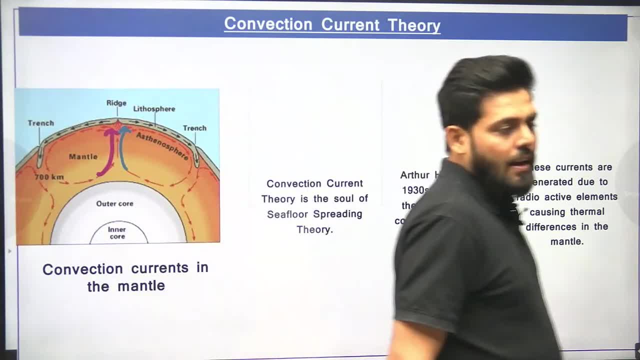 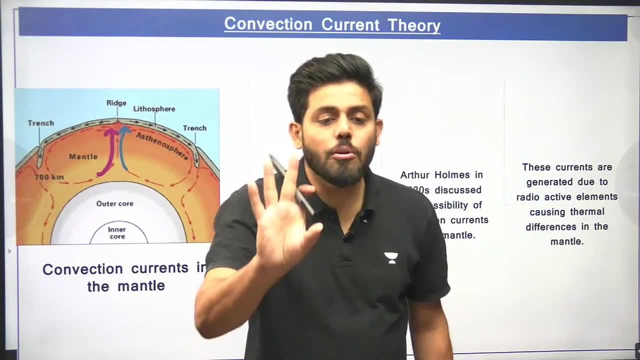 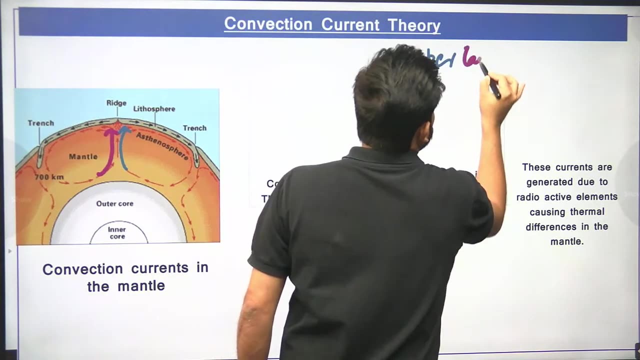 He called this convection current. What did he call this Convection current? Who, Arthur Holmes? Try to understand. Arthur Holmes said that there are two things in our earth: One is the upper layer And the other is the lower layer. 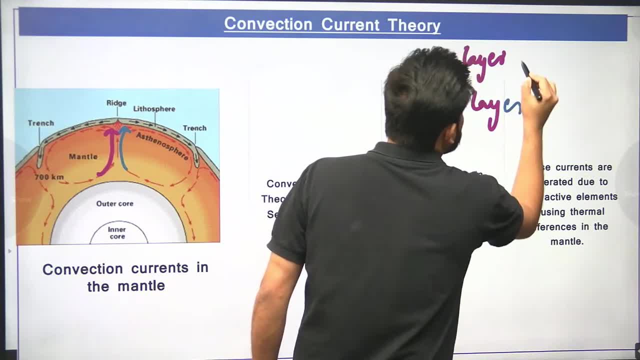 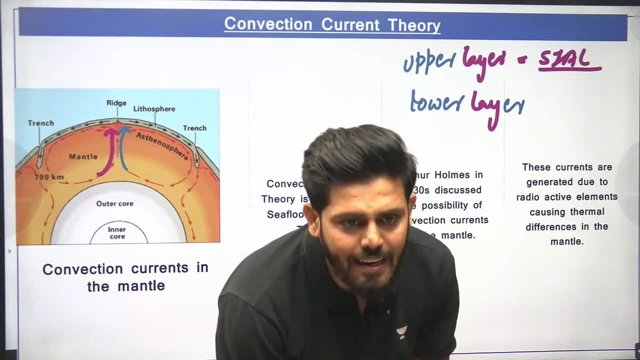 The upper layer, which we call the crust, is made up of slag which is light and has a low density. On the other side, what did he call our mental? He called it sub-stratum. What did he call this Sub-stratum? 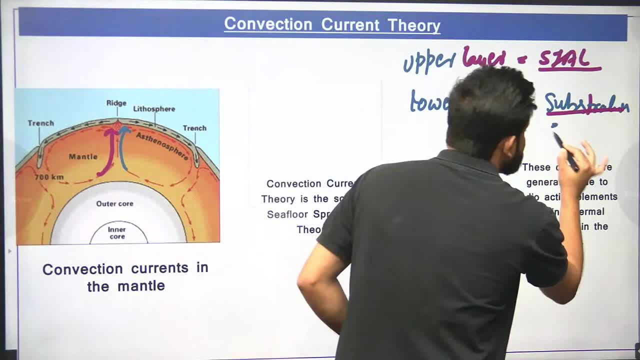 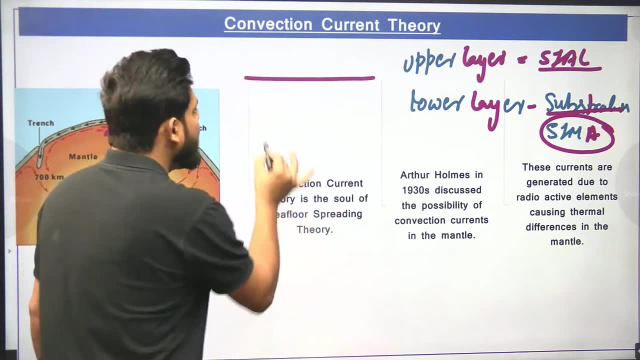 And this sub-stratum, which is the mental lower layer, is made up of slag And its density is high. So he said that, look, this is our crust Right. It is floating on top of this mantle. It is floating on top of this mantle. 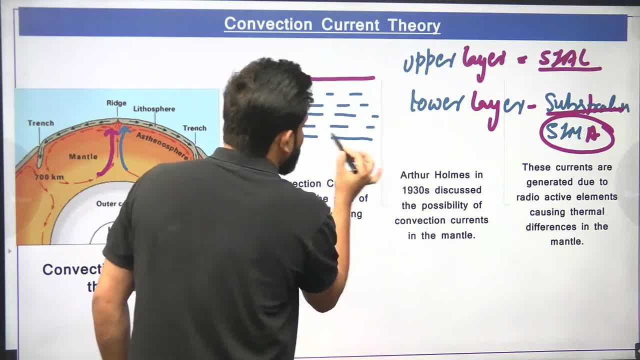 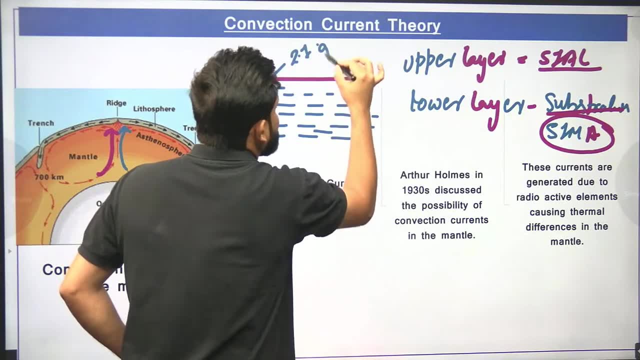 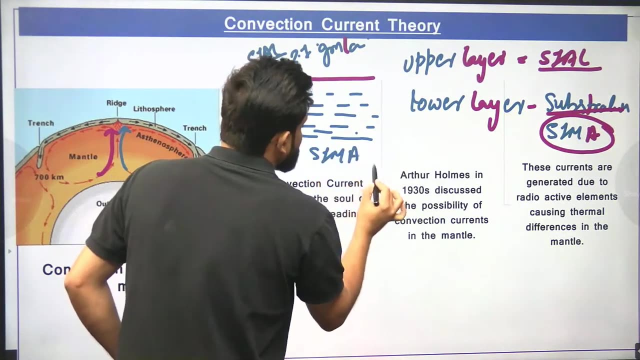 Because our mantle is in liquid form. In what form? In liquid form, And because of this, our upper crust, which is made up of slag whose density is 2.7 grams per centimeter cube, And on the other side, our inner asthenosphere is made up of sema. 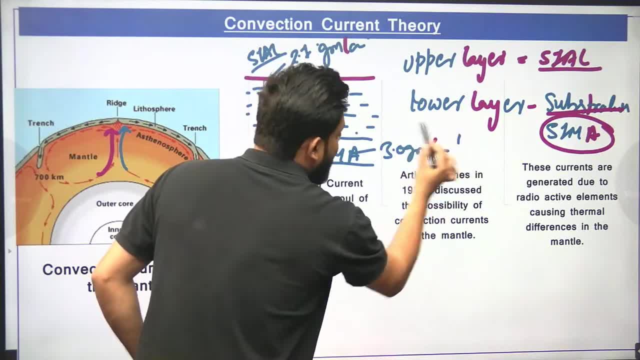 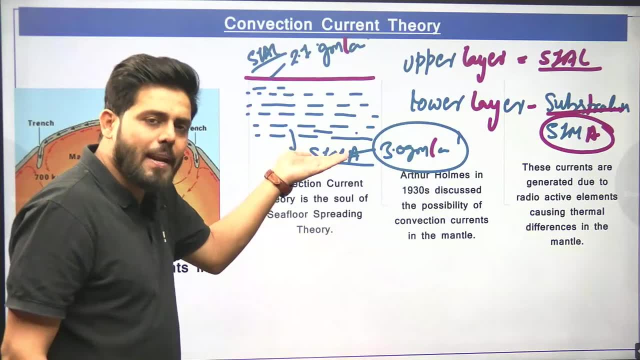 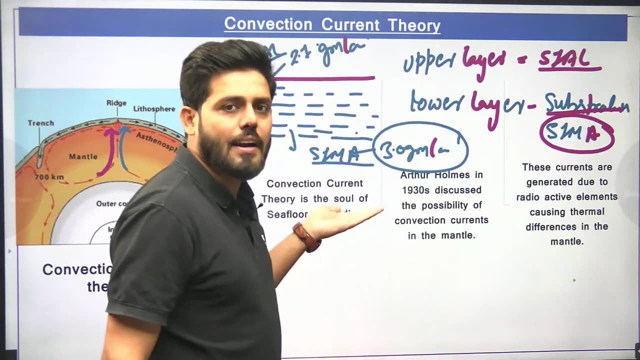 And its density is 3.0 grams per centimeter cube. This is heavy and this is light And it is floating on top of it. Now, because of floating, when its temperature increases, what will be generated in this, Sir? because of increasing temperature, it will have convection current. 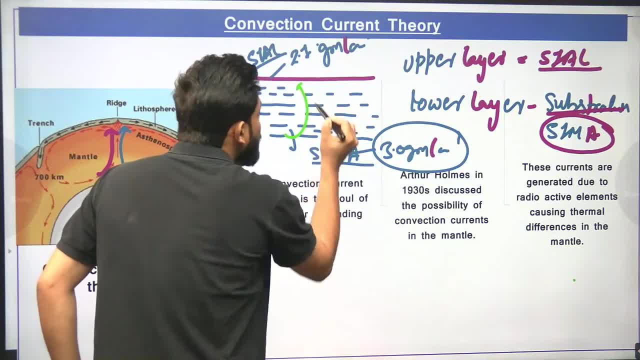 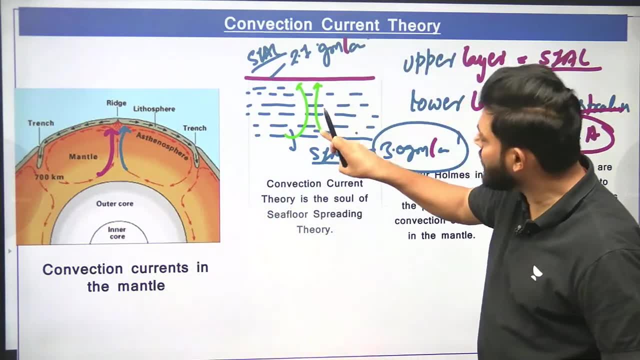 Now, when it will have convection current, then this magma will come upwards like this, And when it will come upwards, then temperature difference will be created here And because of temperature difference, this magma will try to come out. What will this magma do? 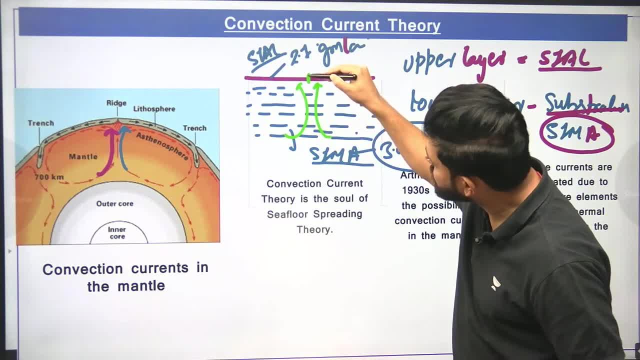 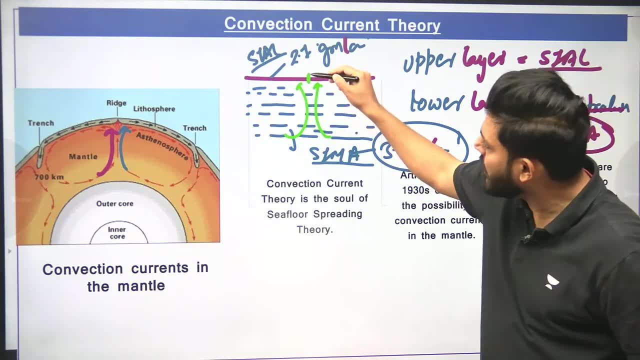 It will try to come out. When this magma will try to come out, then it will break our crust. Try to understand. When this magma will try to come out, then it will break our crust. It will break, And when it will break. 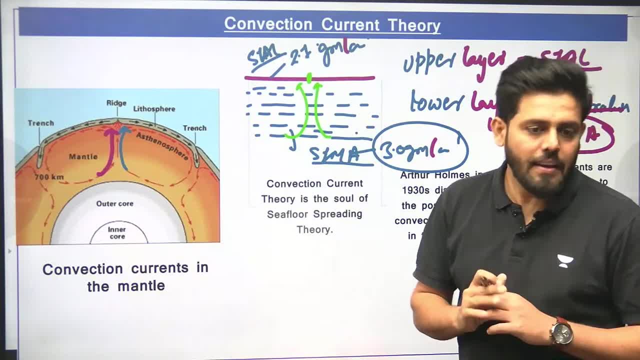 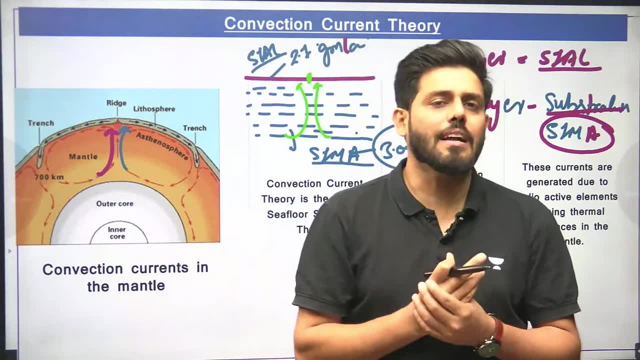 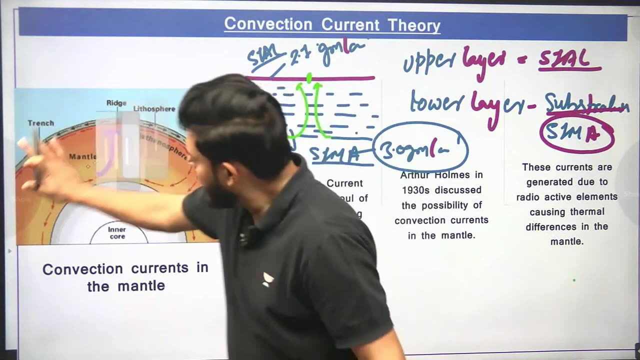 then our magma will come out from here. You should understand these things. So he said that our convection current comes out of two types. One is divergence and the other is convergence. I will tell you both. He said that when our magma will be hot. 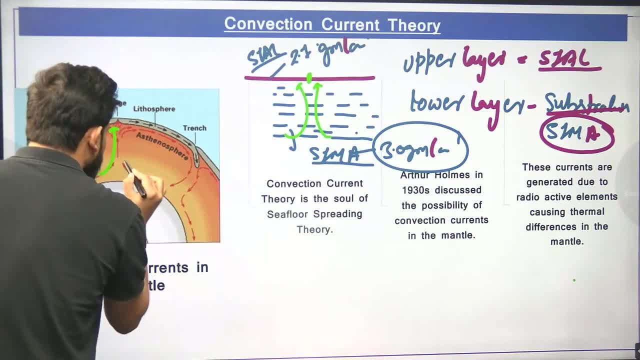 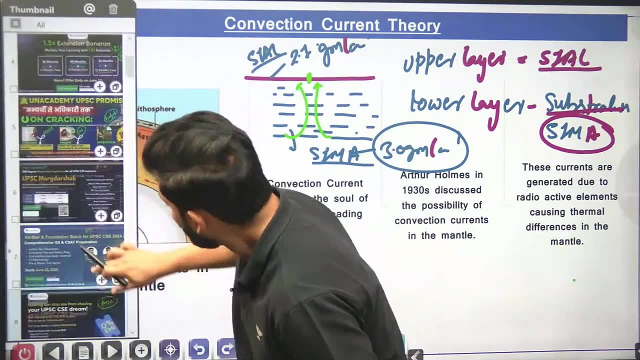 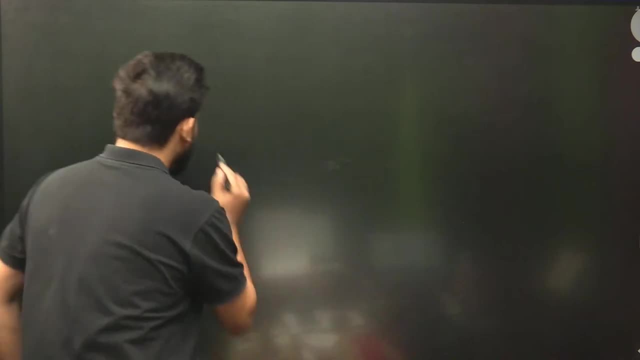 that hot magma will try to come out from here. And when it will try to come out? now this is our crust. I will take you forward so that you can understand things better. Very well, He said that: look, brother, the upper crust of our earth. 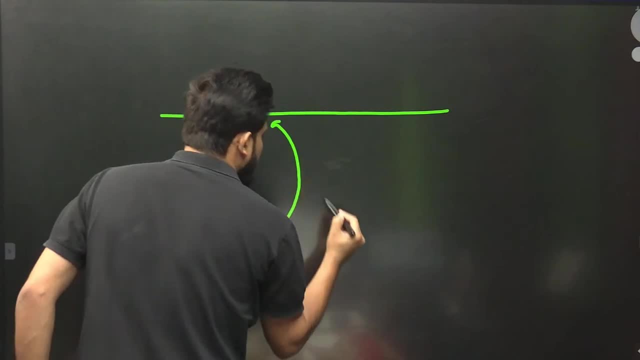 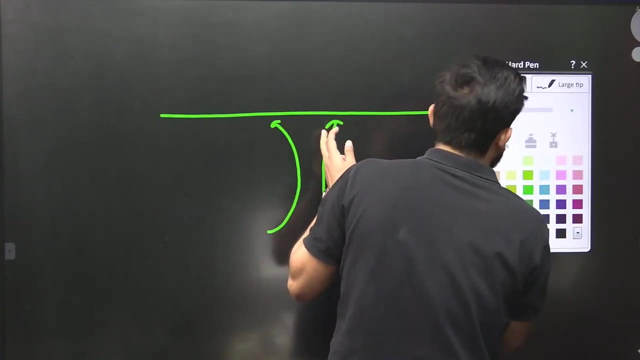 below. this is magma. Now this magma will come upwards. Convection current will be created in this way And it will try to crack here. Convection current will try to crack And when it will try to crack, then magma will come out. 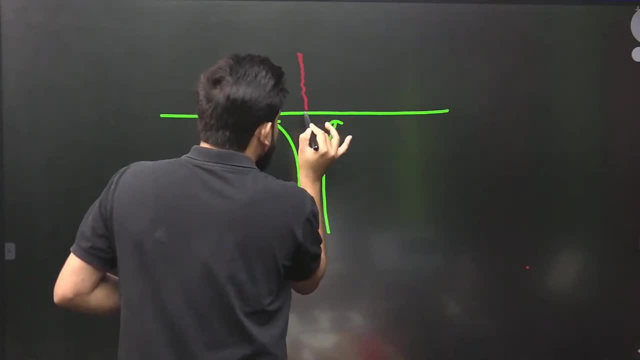 And that magma is coming out like this from here, A crack will develop here, In this area, our convection current- will develop a crack And after developing a crack, magma will try to come out from here. And when magma will try to come out, 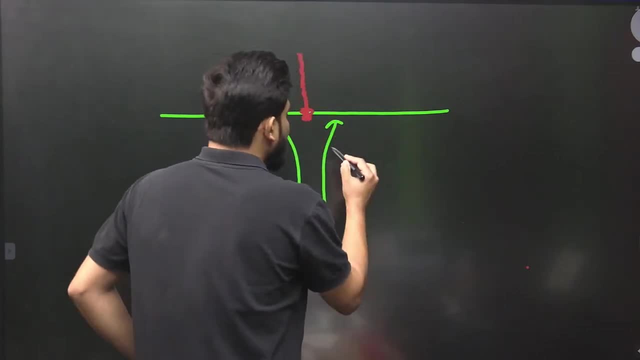 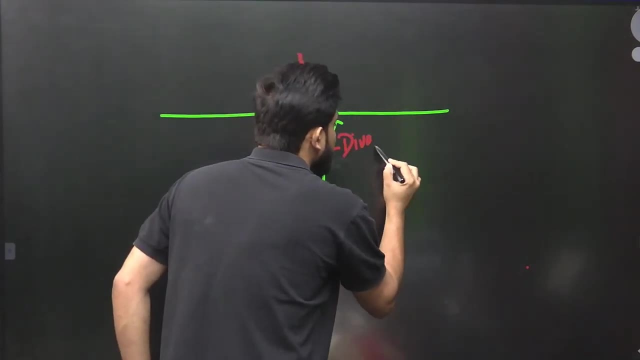 then magma will be deposited here And where. this is ours, which is ours. try to understand which is ours, which is ours. Divergence plate: That means our convection. current is diverging, things Diverge And from where it will diverge. 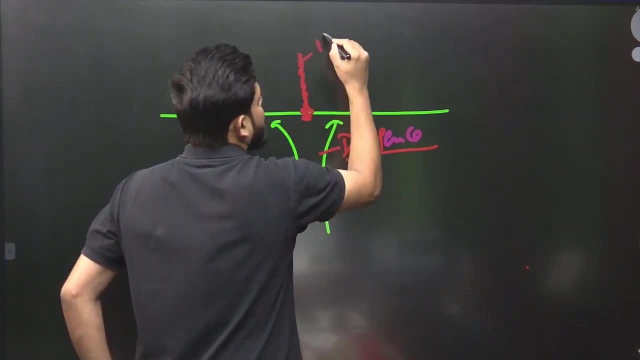 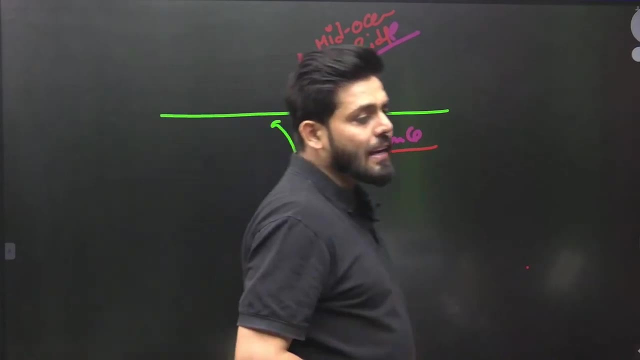 from there the crust will break And after the crust breaks, there will be a mid-oceanic ridge. What will be made Mid-oceanic ridge? Try to understand Now. he said that our magma, which will come out from here. 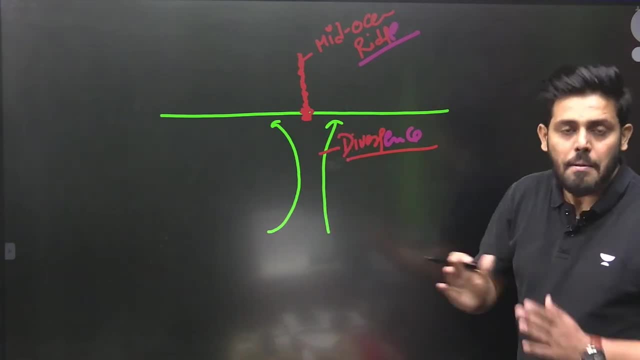 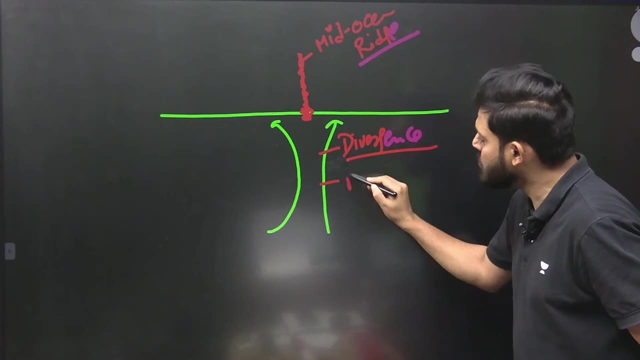 from inside. this is rising limb. This is called divergence, Means it is diverging, Our crust is breaking it. It is diverging. He said this is divergence and this is called rising limb, Because this is rising convection current. 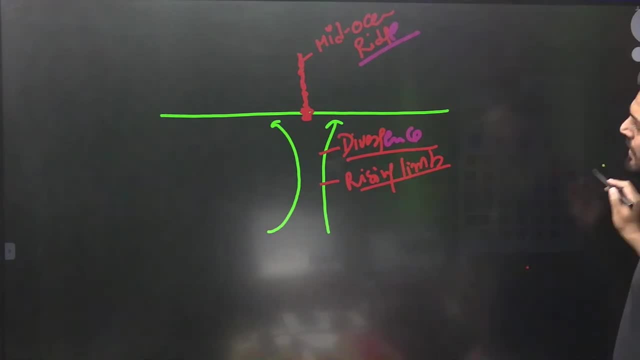 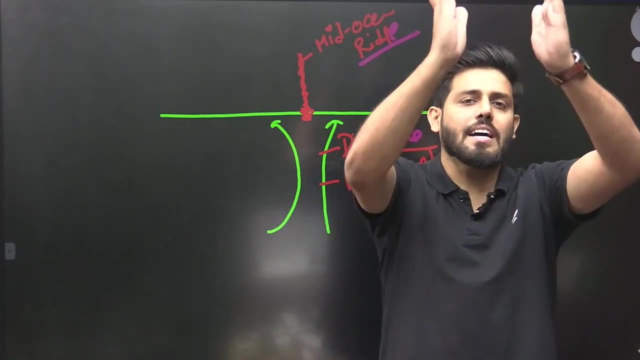 Now he said that this rising convection current, now it has risen. You must have heard that when our gases are hot, when the air is hot and goes up, then sometimes it gets cold, Then after getting cold it will come in this way: 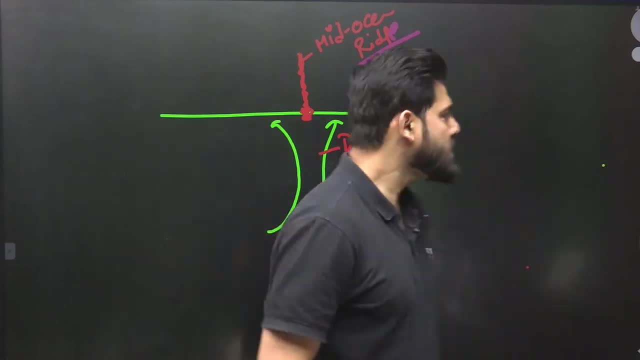 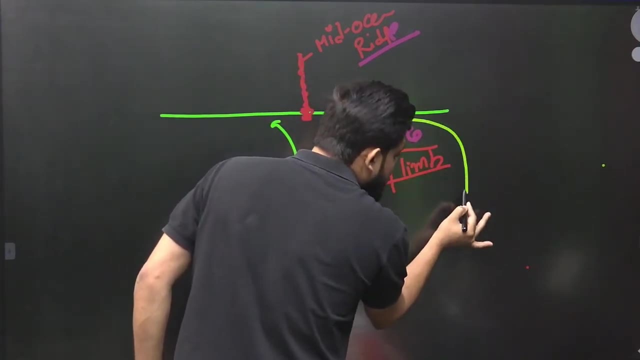 Then after that, it will subside down. It does In the same way when this current, when it rises, it will rise Now, after rising, it will go here Somewhere, it will diverge downwards, Downwards. 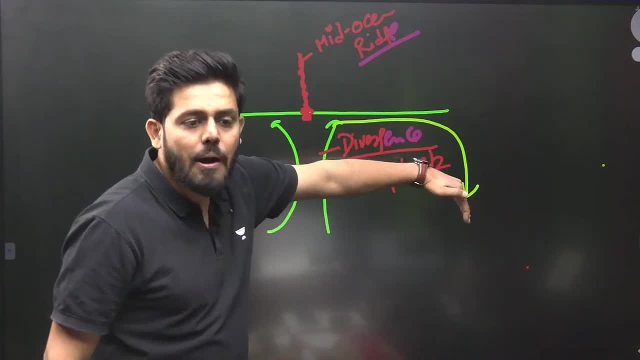 sorry, what will happen to you? downwards, It will go downwards. It will be a falling limb. In the same way, when it has risen, then somewhere it will also reach downwards. Did you understand? When it is your falling limb downwards? 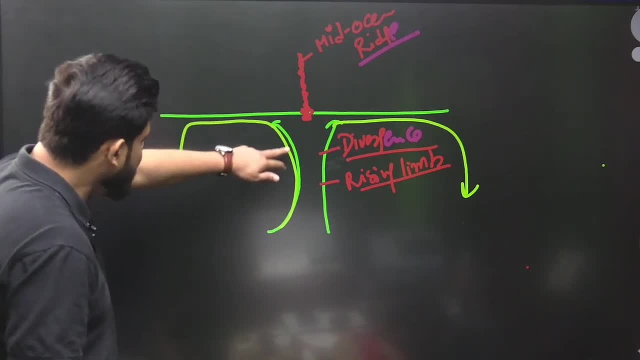 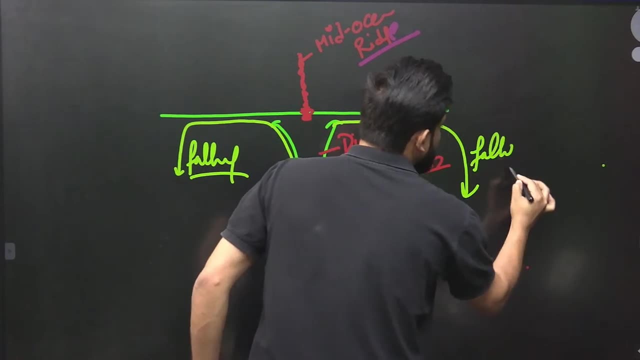 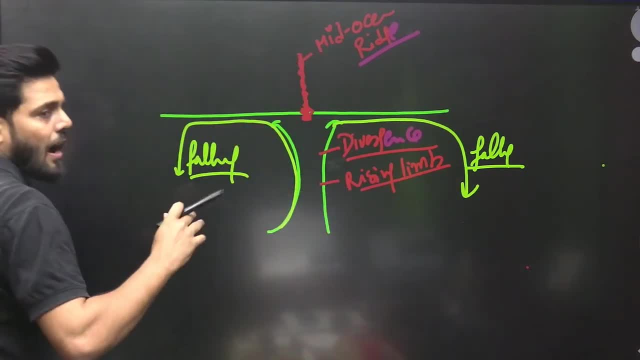 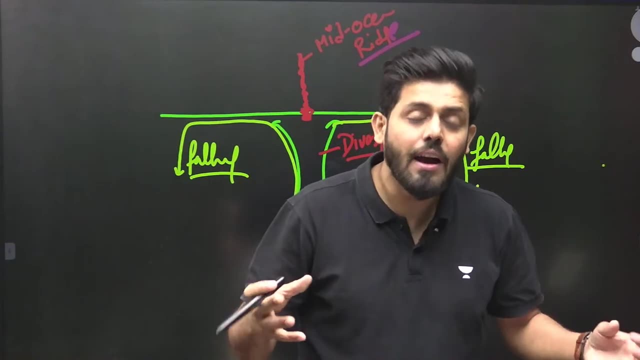 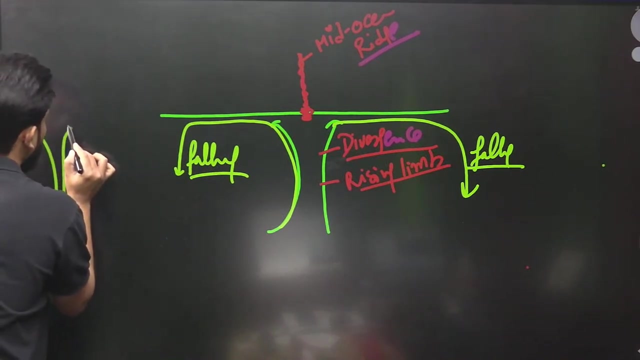 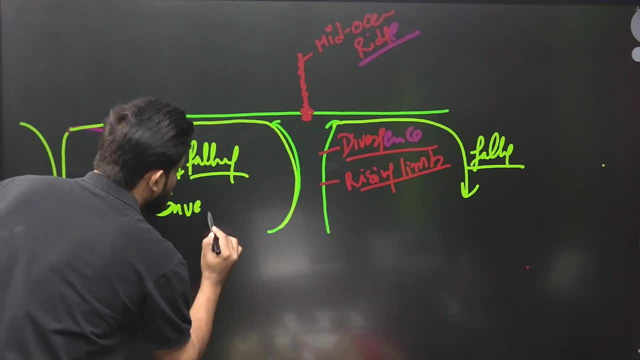 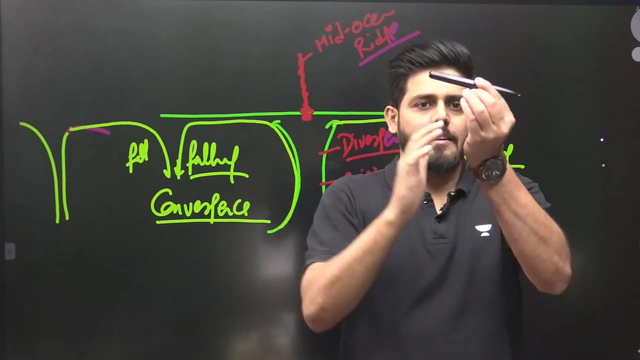 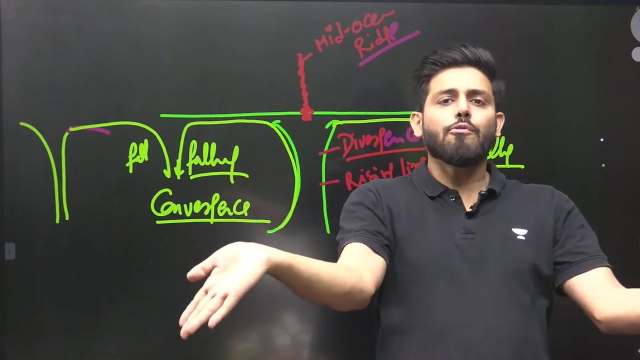 somewhere where both of them will meet. this point is called Convergence. Try to understand this point. this point is called Convergence. That means from here, this limb has risen. this is the crust of magma. This is the crust from here, the magma has risen. after rising, it will go like this, and after that it will fall somewhere. 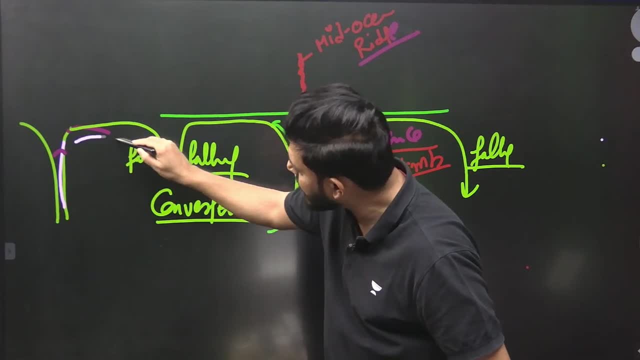 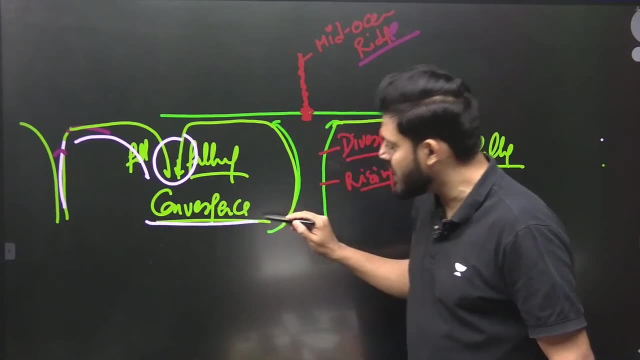 Now there is another limb here. it is rising somewhere. it will fall Where two limbs will fall and both the limbs will meet. there will be Convergence. And remember where Convergence will happen- there. I have told you what will happen. 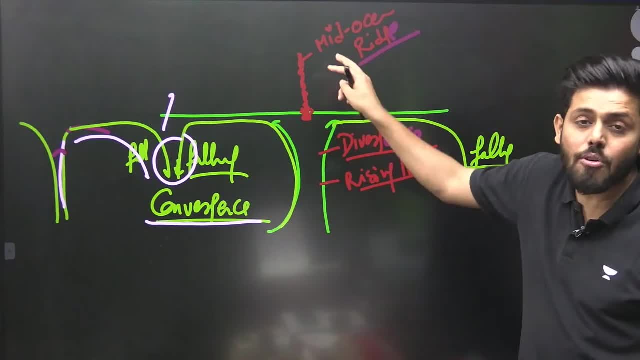 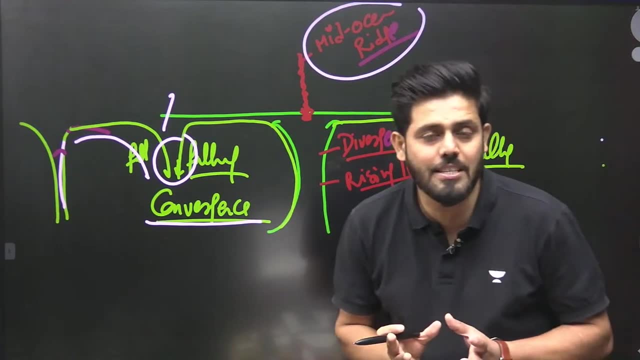 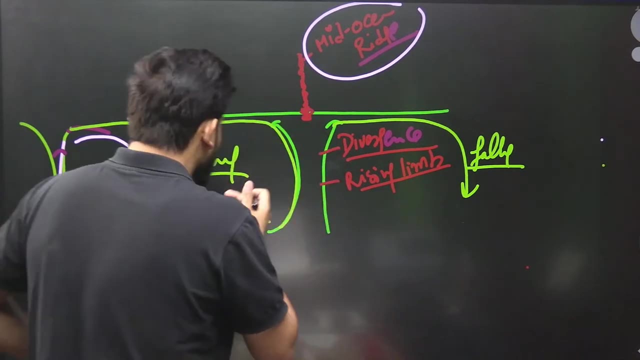 Try to understand where our limb will rise. there our mid-oceanic ridge will be formed And where mid-oceanic ridges will be formed. I have told you very well with a lot of points, And where mid-oceanic ridge is formed. on Divergence: 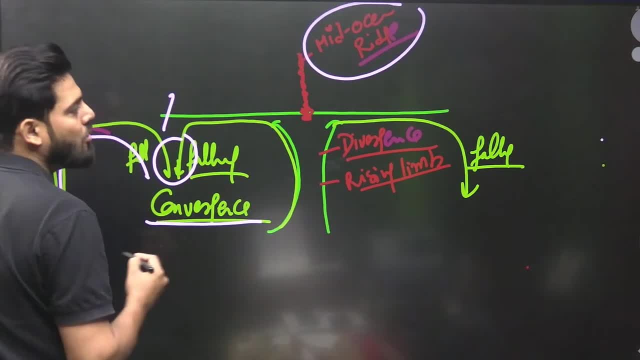 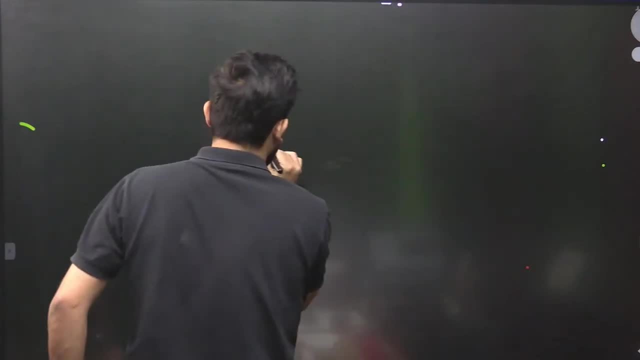 And with that only where Convergence will happen. what will happen there? Now try to understand here. I will tell you very well What happened here. This is our Earth. from here the magma came out. when the magma came out, then the crack developed here. 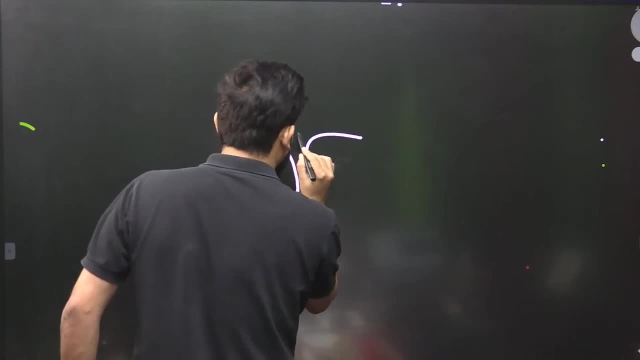 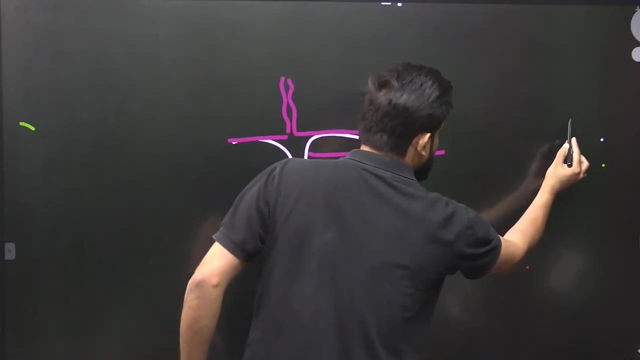 When the magma came out, then the crack developed here in this way, And what happened here? Mid-oceanic ridges were formed. Now this plate is one plate here and this is the second plate here. Now these two plates will collide. 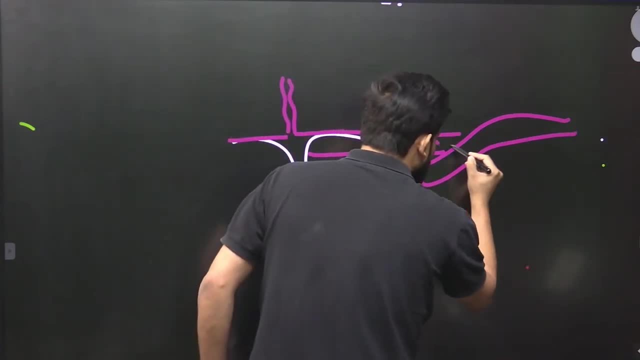 This plate will be subducted downwards Now. when it will be subducted, then what will happen here, In this area? a geosynclined depression will be formed When these two plates will collide here. what will happen by colliding? 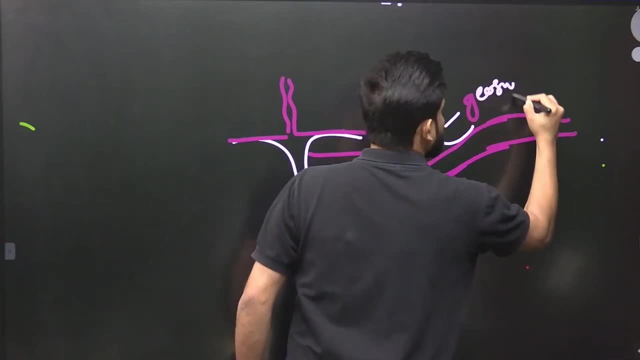 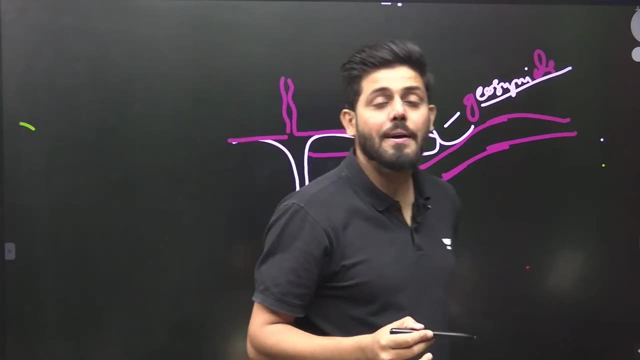 Here, a geosynclined depression will be formed. What will happen? Geosynclined depression will be formed. Remember this thing. And when this geosynclined depression will be formed? as I told you, when the Indian plate collided with the Eurasian plate. then what happened? by colliding, These two plates collided, These two plates collided From here, this plate was subducted below it. And when it was subducted, then what happened here? A depression was created here, And this depression is called geosynclined depression. 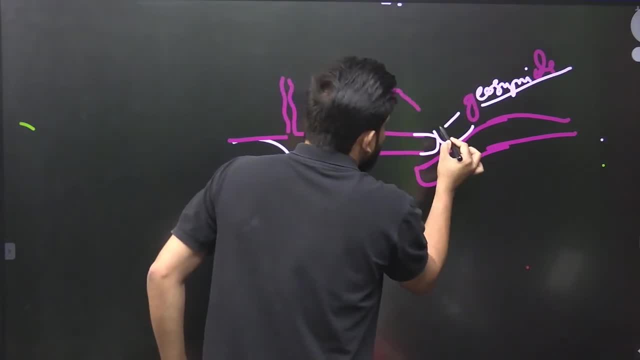 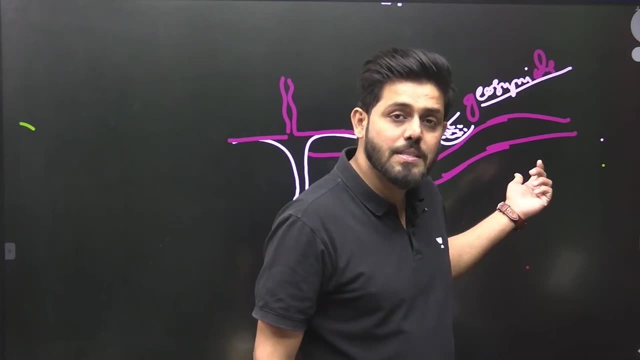 And from this geosynclined depression, the rivers that are coming from here will keep on filling the geosynclined depression, And when this geosynclined depression will keep on filling, there will be sediment deposits in it. 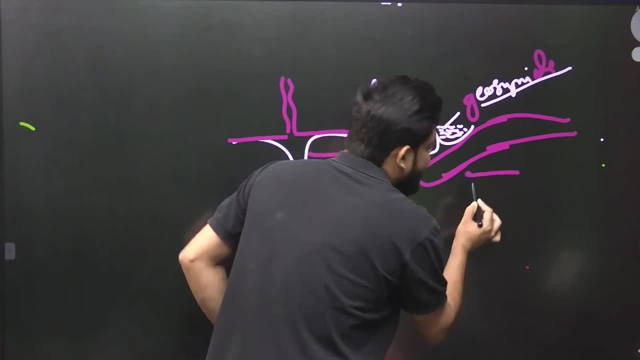 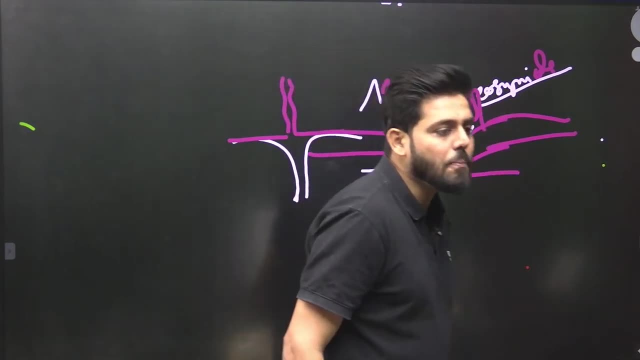 And when the sediment will be deposited, and this force will keep on applying continuously, the sediments there will squeeze and take the formation of the mountain. Whose formation will they take, Sir? they will take the formation of the mountain. Is it clear? 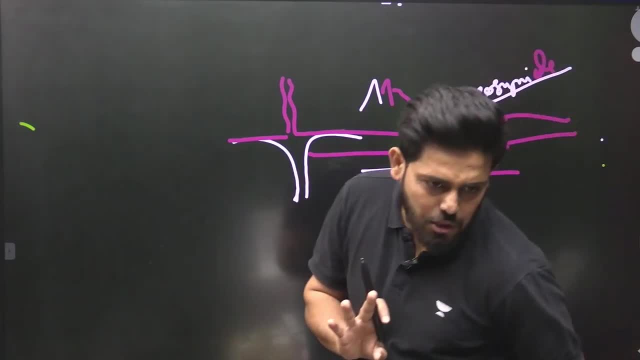 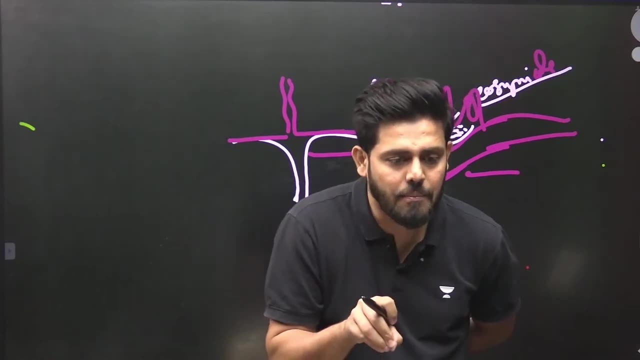 So always remember that, your convection current theory. What did it tell us? It told us that what is there in our earth? There are radioactive elements in our earth And when the temperature of radioactive elements increases, their disintegration will happen, So they will rise. 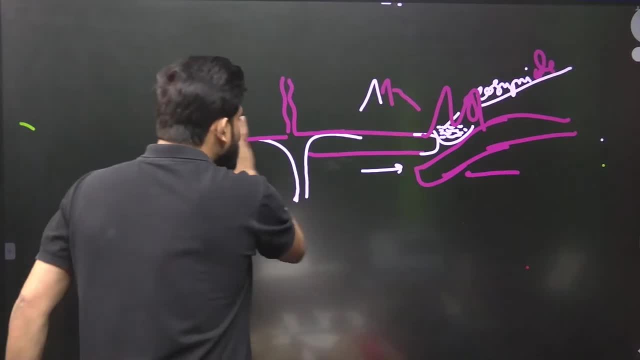 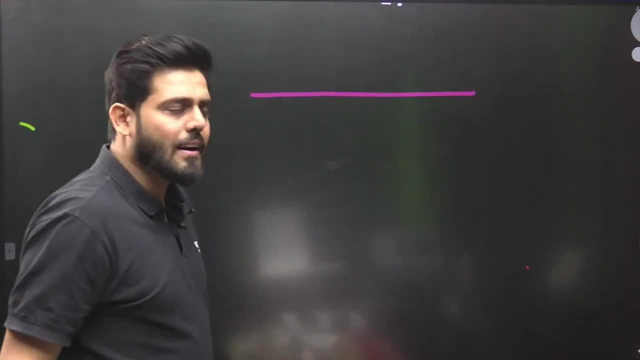 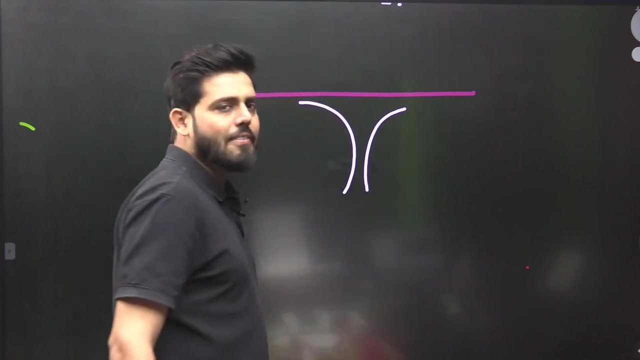 And where there will be rise, there will be convection current. So what happened? In the convection current theory? Arthur Holmes told that the earth below us has convection current And where this convection current will rise, the continent will drift from there. 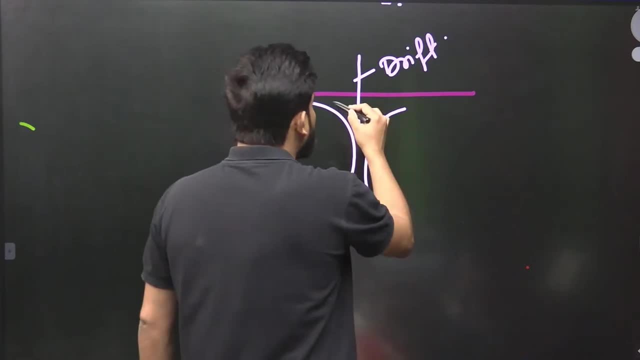 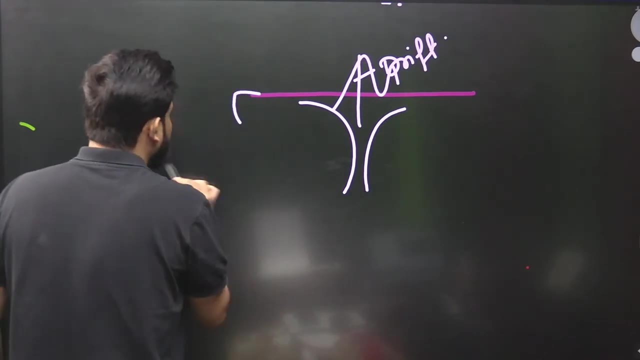 And, due to drift, mid oceanic ridges will form And there will be volcanic eruption too. Mid oceanic ridges will form and volcanic eruption will happen Along with that after the convergence. here it will diverge, Here it diverged. 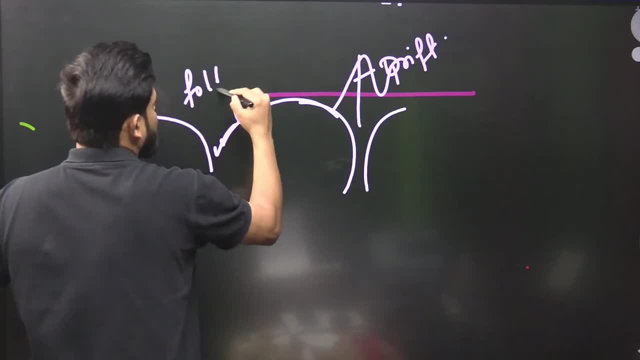 Here it will converge. Here it will form the fold mountains. Here it will form the fold mountains. Who told this? This was told by Arthur Holmes. Is it clear? Who told this? He told this in his convection current theory. Now let's read what Arthur Holmes said once. 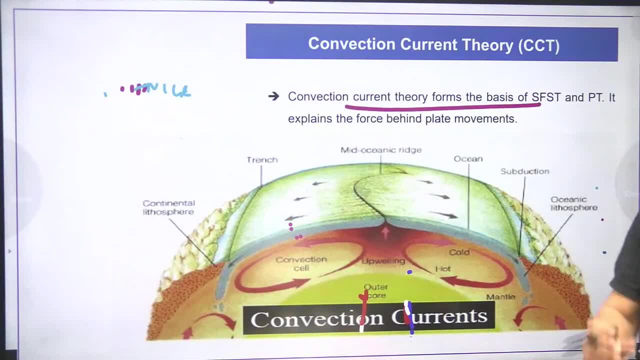 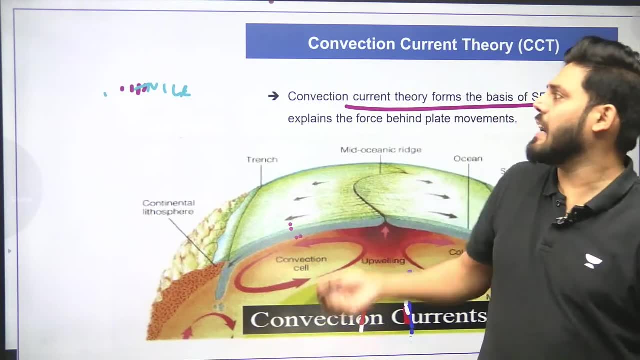 He said that the convection current theory, later the seafloor spreading theory will come And the plate tectonic theory will come. Their base is taken from the same theory which was given by Arthur Holmes in 1928 and 1929,. 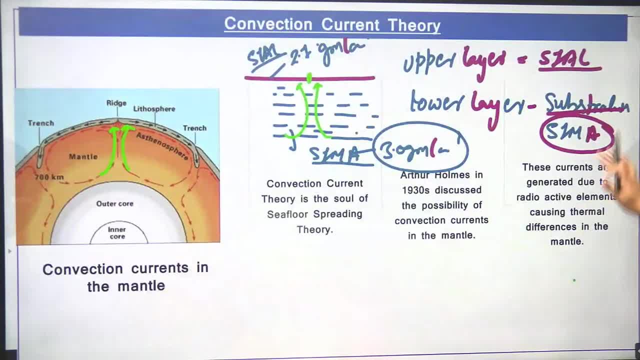 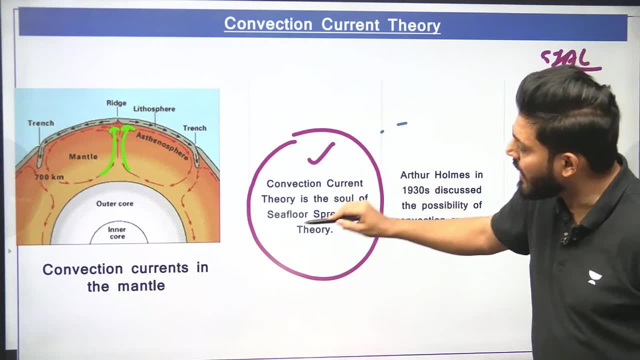 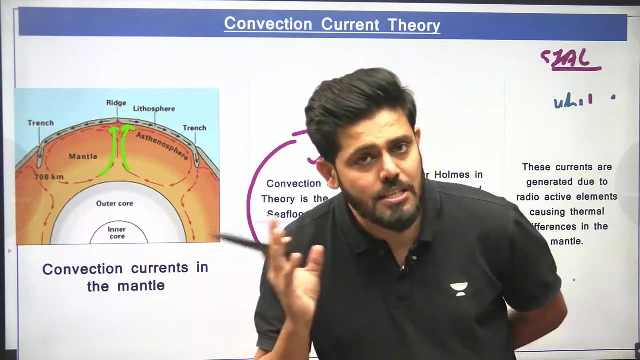 which is called convection current theory. What did Arthur Holmes say? He said that in the coming time the base of your seafloor spreading will be convection current. Convection current will tell things that our ocean seafloor spreading theory. 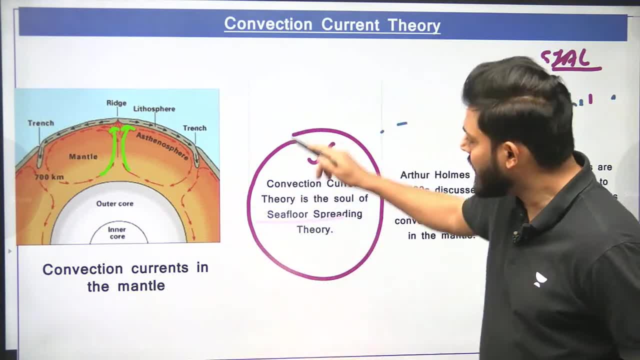 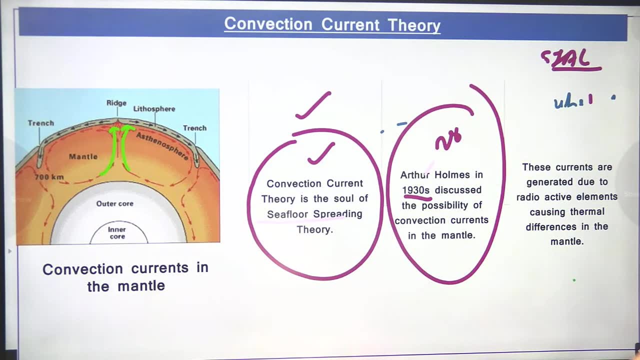 how it spread. This theory will tell you about all those things. Along with that, Arthur Holmes told the possibility- in 1928 and 1929, that the mantle in the interior of our earth, its temperature, is high, And due to high temperature, 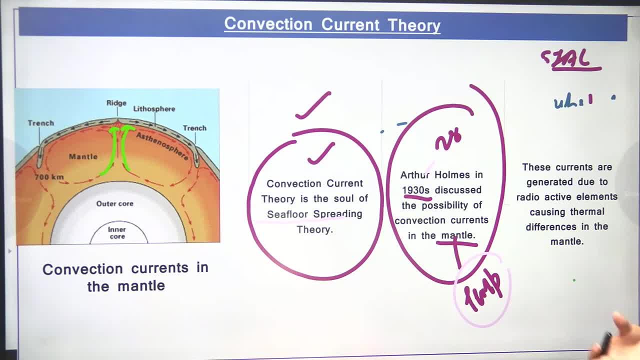 there are radioactive elements there. What will happen in them? Due to disintegration, due to increasing temperature, they will try to come out a lot. And when they will try to come out, then what will happen? The radioactive elements will create a thermal difference in the mantle. 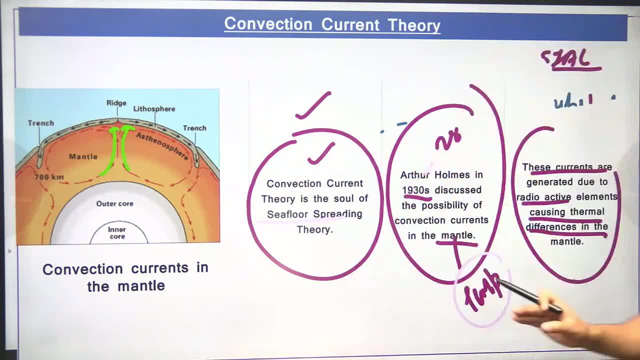 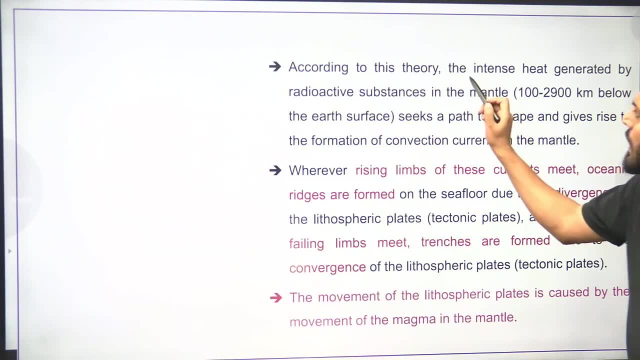 Temperature difference will be created, Due to which they will try to come out of the mantle, And when they will try to come out of the mantle, then intense heat will be generated. This is what has been said: The intense heat generated by the radioactive substance. 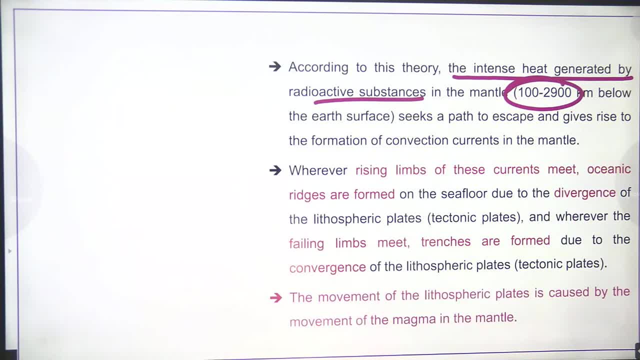 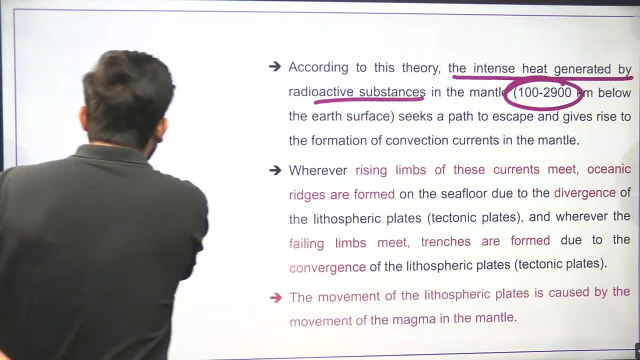 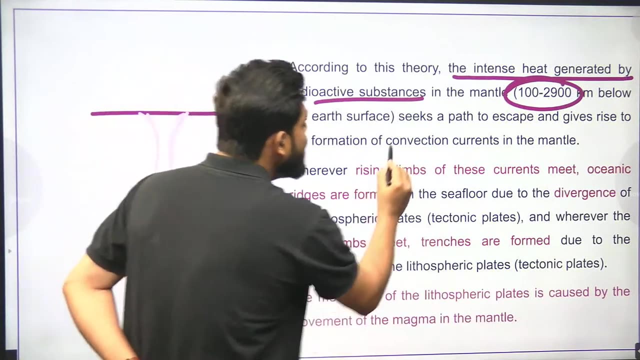 Where The mantle, whose depth is from 1000 to 2900 km, And after that the high radioactive elements, when they have become hot. they need some path to come out. They need some place to come out, So it seeks a path to escape. 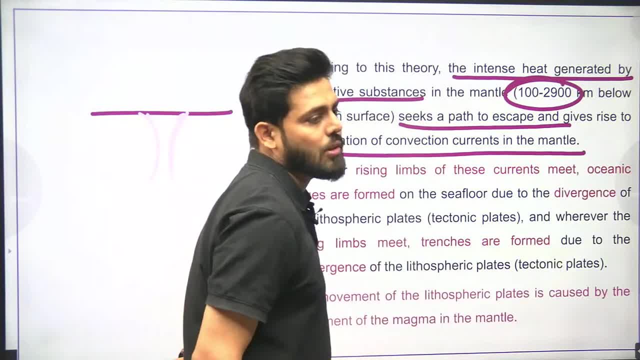 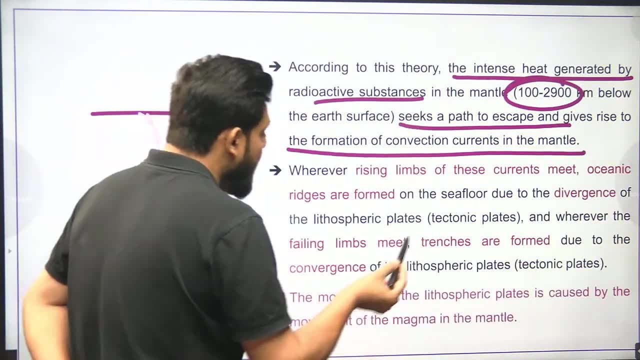 and give rise to the formation of convection current to the mantle. And what will they do? Rise of convection current from where? From the mantle. Remember this thing: Where there will be rising limb, Where there will be rising limb, This is the rising limb. 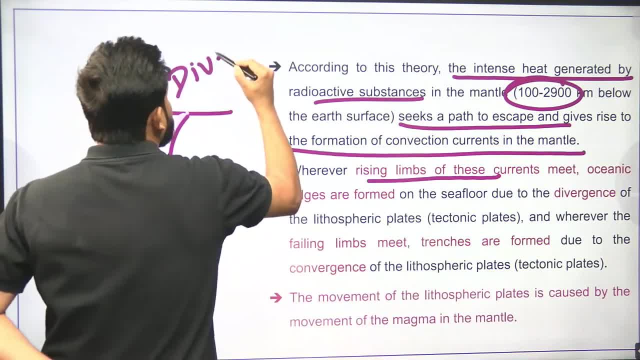 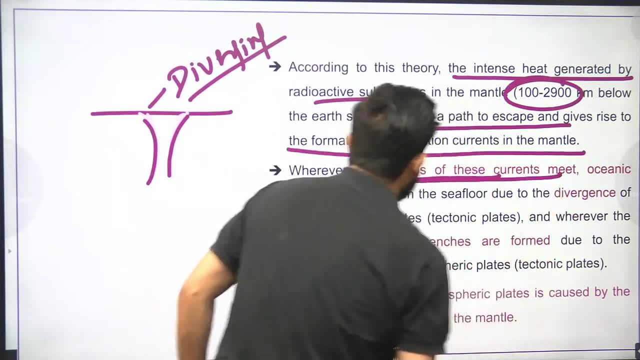 And what is this? rising limb, Divergent plate boundary? This is diverging, Diverging current. What is the current doing? It is diverging. So where there will be rising limb, there you will get to see the oceanic ridges on the sea floor. 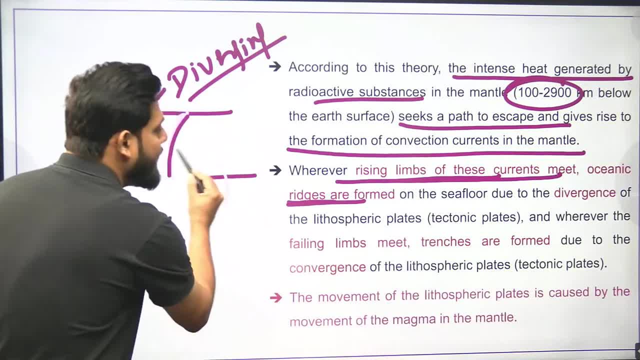 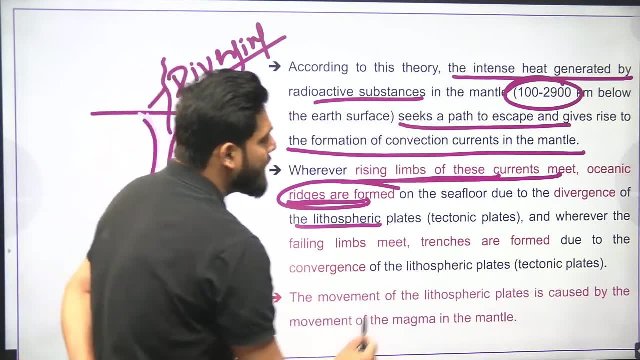 Okay, Remember that. the lithospheric plate, where there will be divergence. what will you get there? You will get to see the ridges here. And where the rising limb is, what will it do to you? Falling limb will be found. 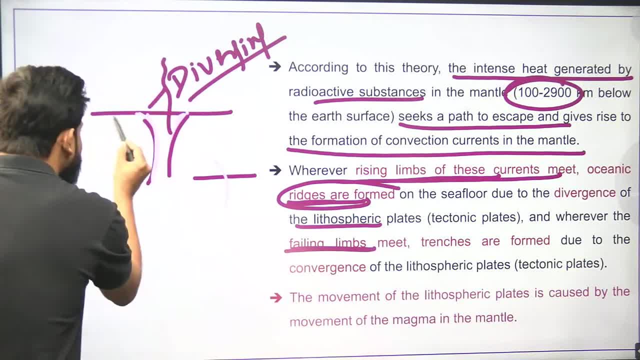 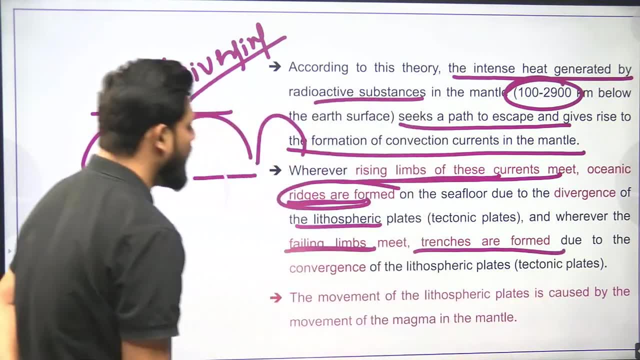 Failing limb will be found. Falling limb will be found Where it rises. where it falls, you will get the limb, And where it falls, you will get two limbs. There will be the formation of trenches. This is what they told. 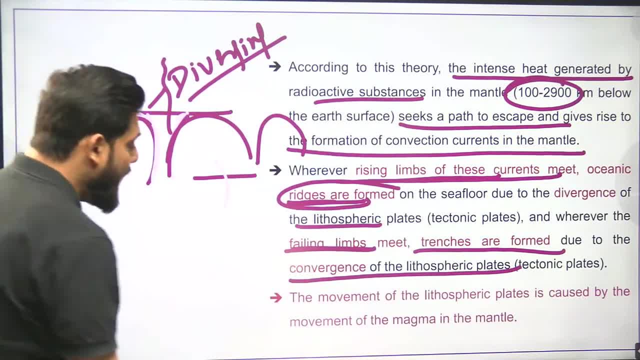 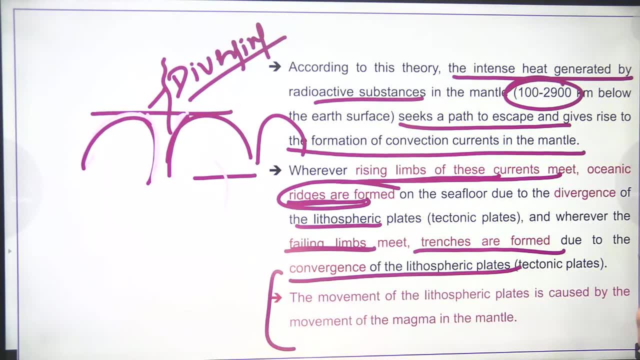 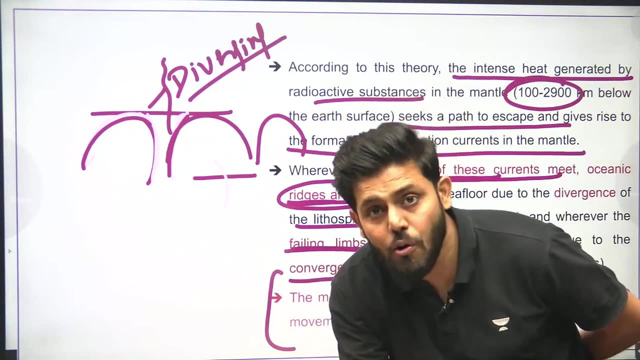 Who told you? Arthur Holmes. Arthur Holmes gave the reason That our continents, which have drifted, Try to understand. Arthur Holmes told that the reason behind the drift of our continents is the magma of the interior of our earth And that magma due to the high temperature. 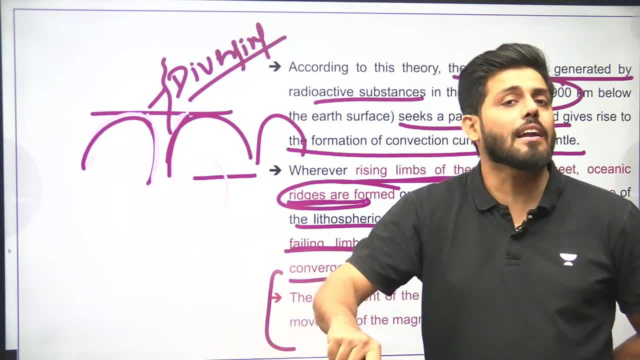 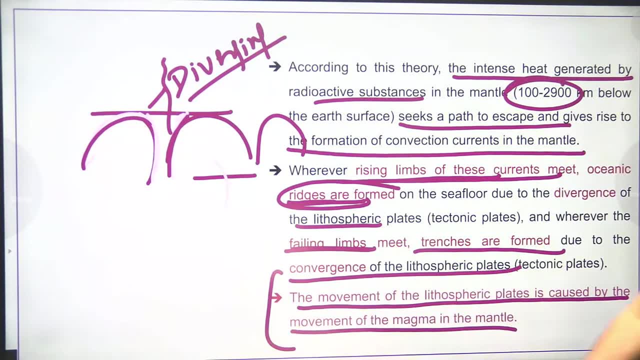 which has formed in the interior of our earth. because of that, this whole role has been played. So the movement of the lithospheric plate is caused by the movement of magma inside the mantle. And what is the reason behind the movement of magma? 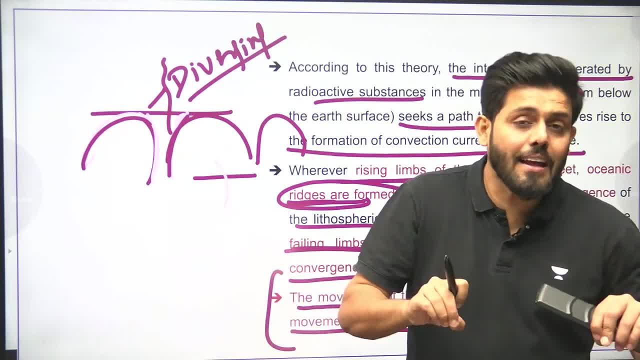 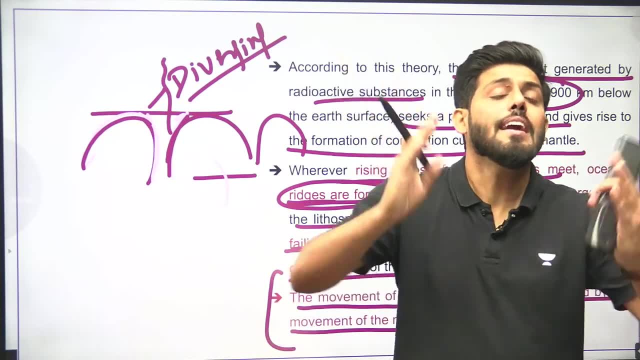 The reason behind its movement is that the mantle in the interior of our earth, the radioactive elements there. due to their high temperature, they will try to come out from somewhere, From where they are coming out from the upper side, From where they will come out from the upper side. 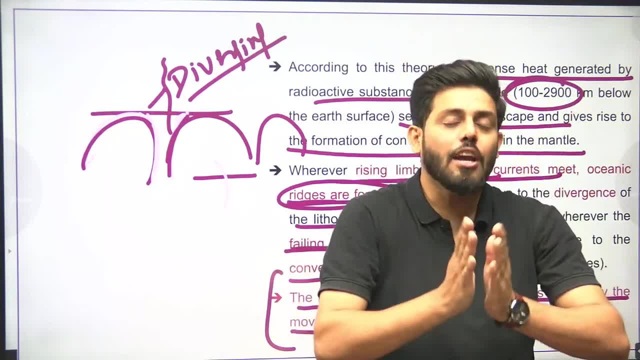 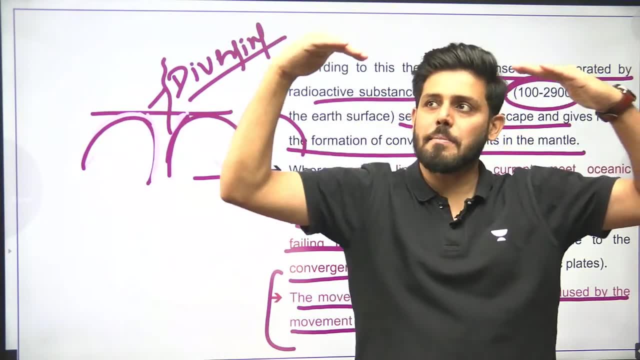 like this: there will be a ridge And where they will fall like this and along with that, another falling limb will be found, like this: When one plate will be subducted under the other plate, there will be the formation of trenches. 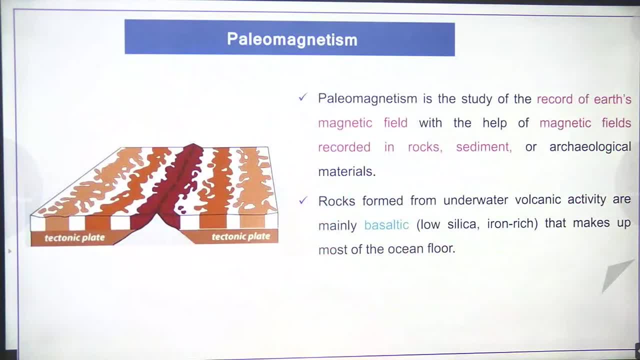 You will get to see this. This is what Arthur Holmes told, Did you understand? Arthur Holmes has no problem in any way. After that I will discuss paleomagnetism, But sea flow is spreading. I will discuss sea flow spreading first. 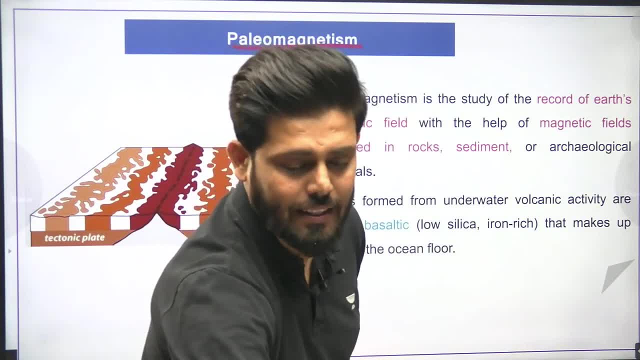 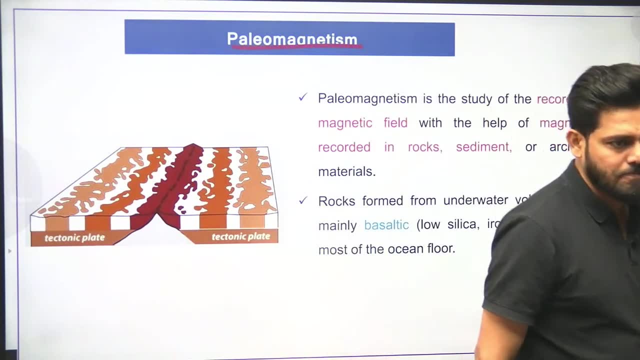 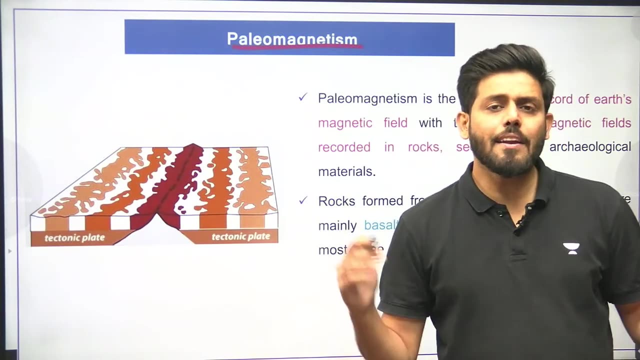 Now tell me how many students are there who have any doubt in convection current theory. Then I will discuss sea flow spreading and further things. Okay, Does it matter which plate is colliding with each other? Now the plate also matters, right? 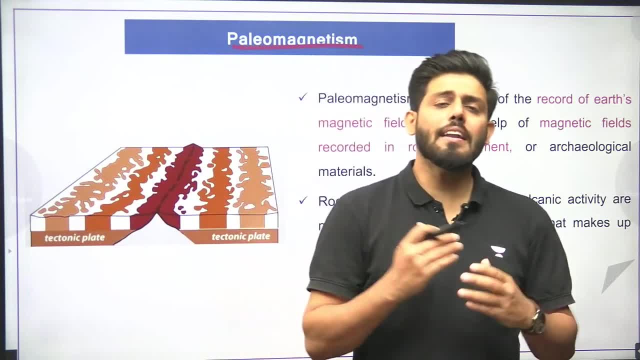 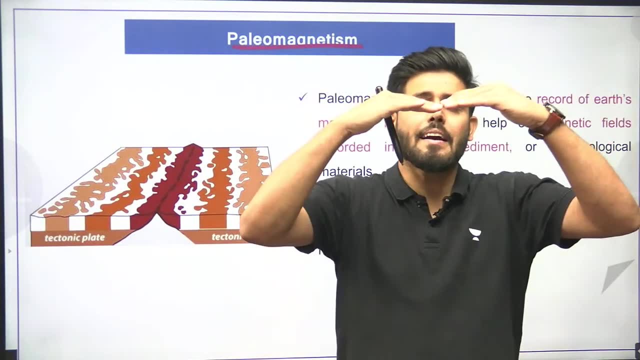 If oceanic plates collide, trenches will be formed. If one continent and one oceanic will collide, then what will happen? Trenches will be formed. If a continental plate is colliding there, then geosynclined depression will be created. 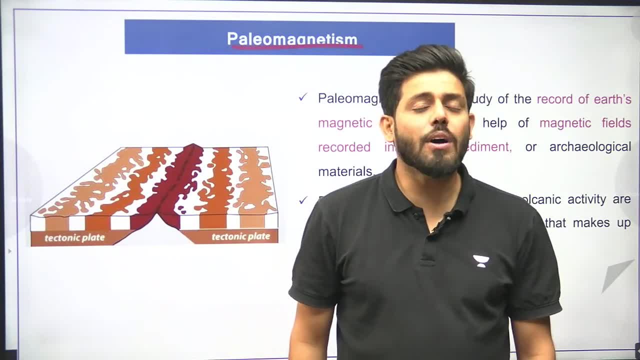 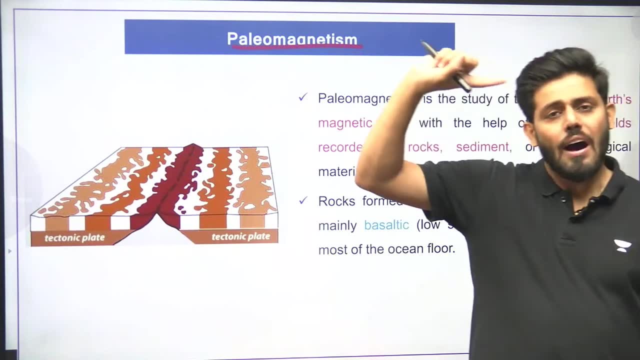 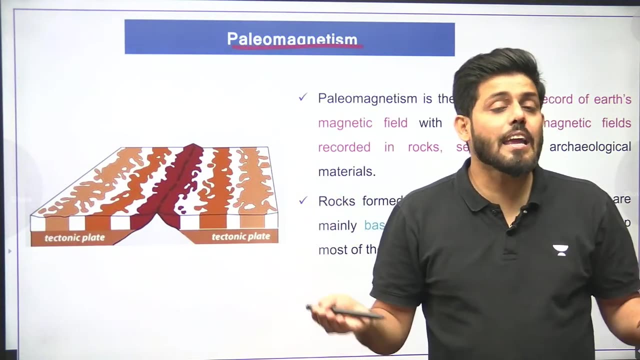 Just like the formation of the Himalayas, So it matters which plate is colliding. This can also be important When I will teach you further mountain building: different mountain buildings of the world, volcanic arcs, island arcs, how they formed. 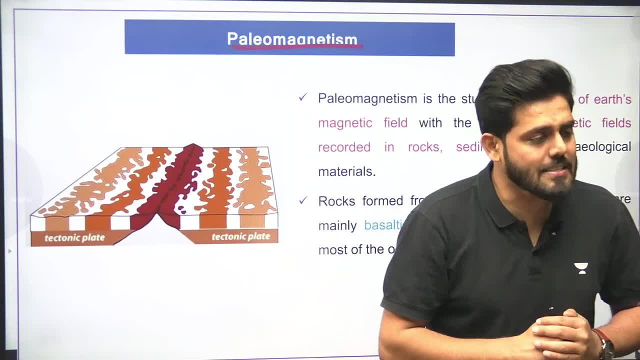 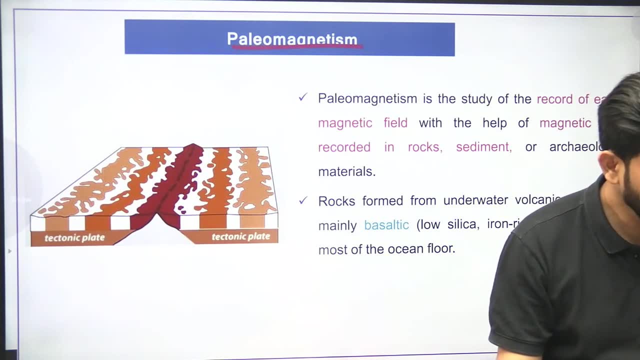 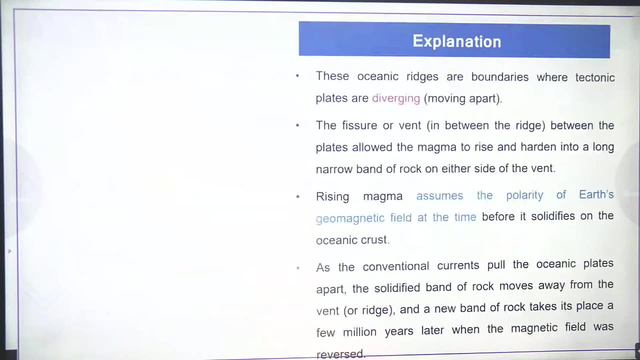 then you will understand how things are formed by colliding with plates. Do you understand? Let's move ahead. Does anyone have any problem? Is everyone clear? Let's move ahead to the next point. Now we will talk about sea flow spreading theory. 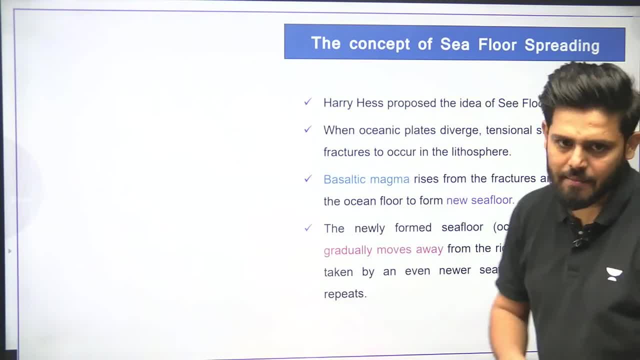 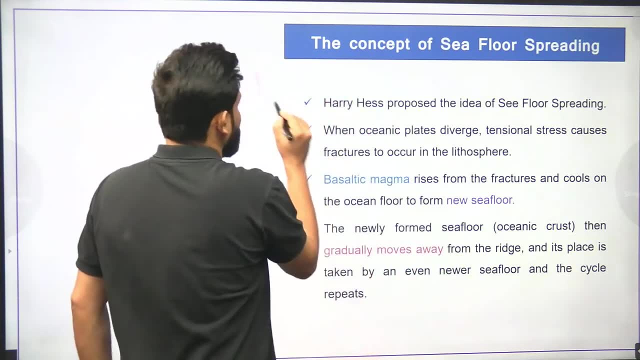 What is sea flow spreading? After that we will talk about paleomagnetism. Sir, who gave the sea flow spreading theory? This was given by Henry Hess. Who gave it? Harry Hess? Harry Hess gave this theory. When was it given? 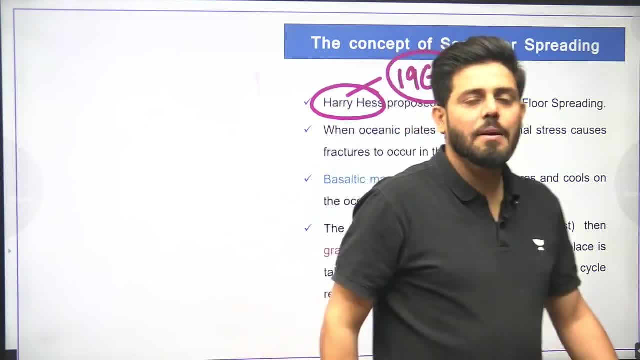 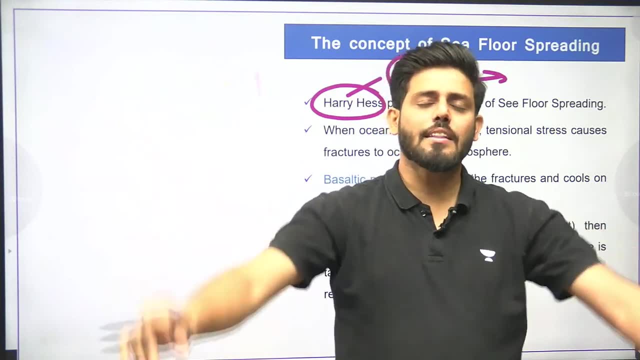 In 1960.. Sir, how was this theory given In 1960. Look from today, 75 years ago. 75-80 years ago, the second world war was going on To defeat each other. powers, powers of two different worlds were different. So at that time, submarines were started to be made Because countries wanted to attack through the waters, Through the oceans. they wanted to attack other countries. So, because of this, countries started to make submarines. Now, when they started to make submarines, 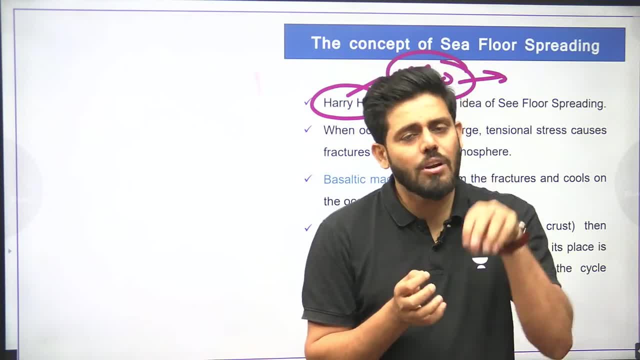 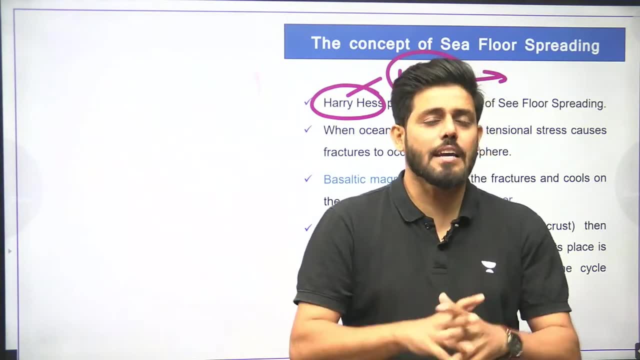 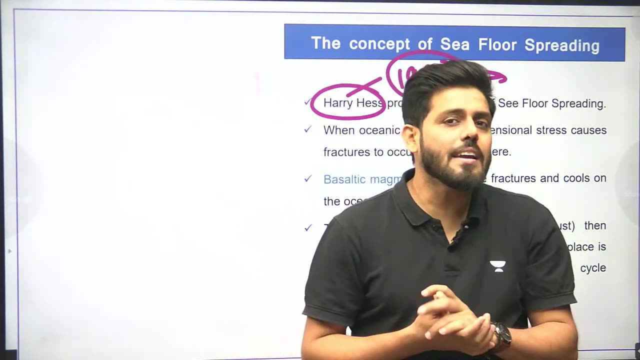 people thought that we will take the submarines to the land, into the ocean. At least we should know about the mapping of the ocean, the surface inside the ocean, Because if our ocean is uneven then our submarines will collide and they will get destroyed there. 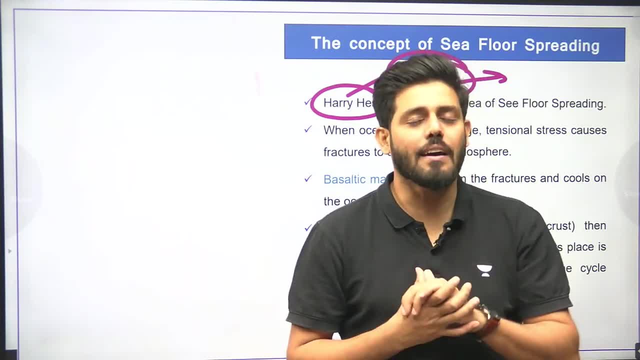 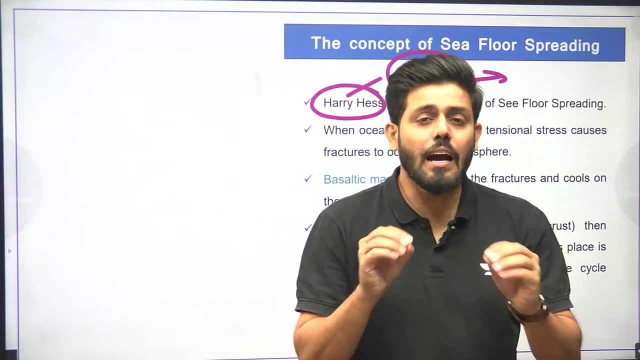 So first it was said that we will do geomapping of the ocean, How the ocean looks from inside. we will do geomapping, But they never thought about it. They never thought in their mind that our ocean will be so uneven When they went inside the ocean. 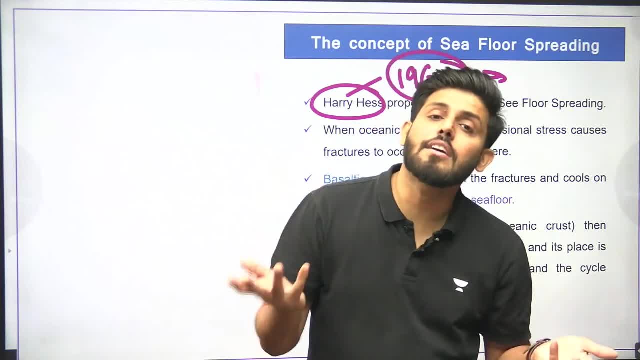 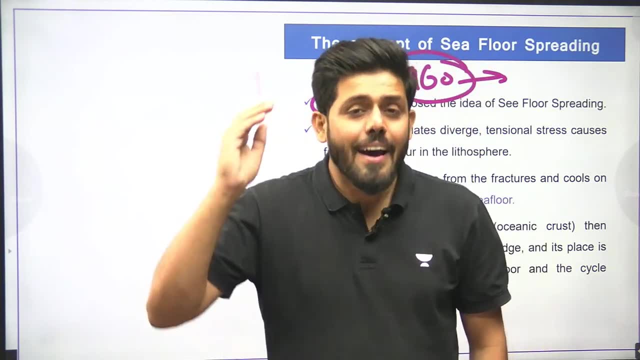 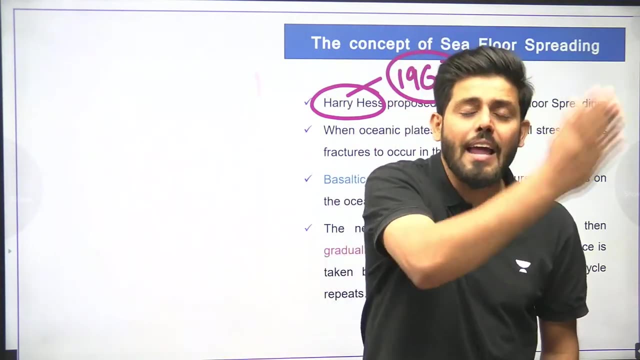 they studied things from the submarine, then they got confused. They didn't believe that we talk about our land- mountains, plateaus, rift valleys- But when they went inside the ocean they got confused. They didn't believe that our land is more than that. 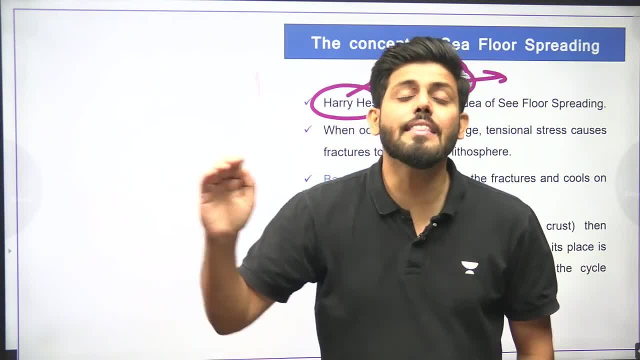 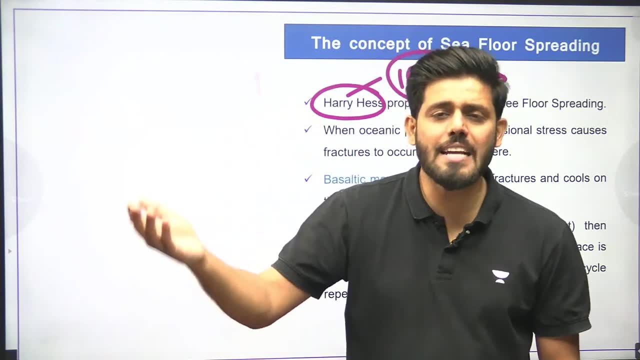 The physical features. we got to see them inside the ocean. We know that inside the ocean there are different features. There is continental shelf, continental rise, abyssal plains, gaiotes, trenches and ridges. We got confused after seeing them. 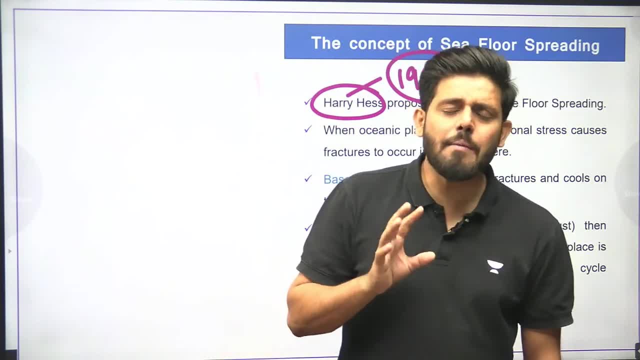 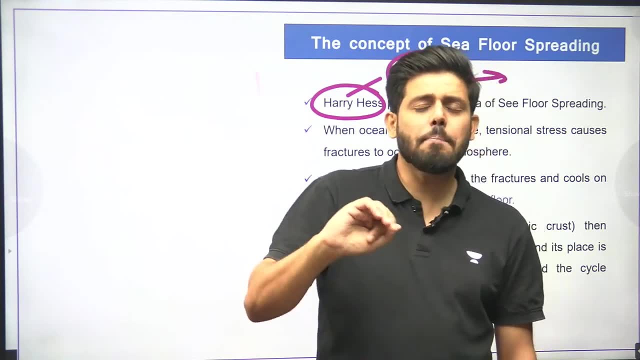 There are so many things inside the ocean. When we came to know all these things, when It is about 1948-1947.. It is about the reasons around 1945.. It is about the Second World War. It is about the time before 1945.. 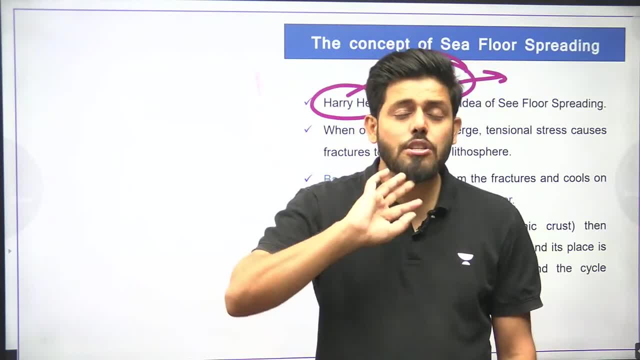 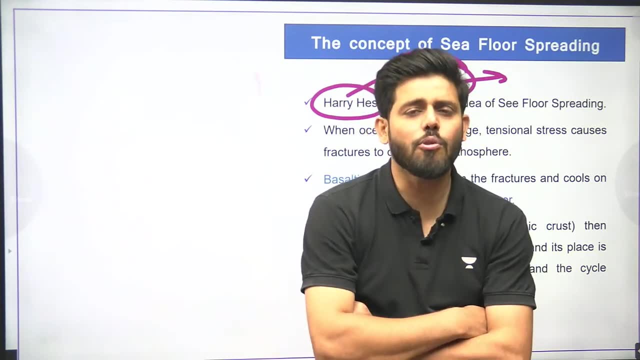 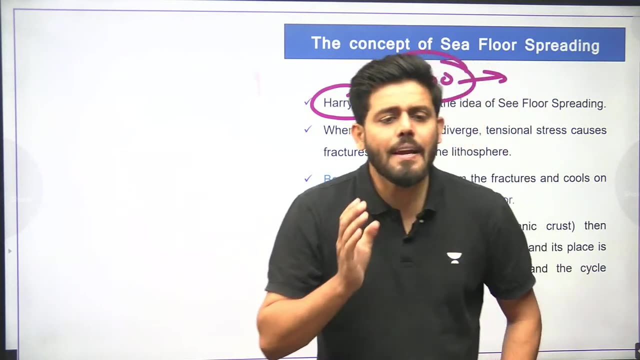 It is about the time around 1942-1943.. What happened there? When we started to know all these things, people got curious. What were the things inside the ocean floor that we got to see? Try to understand What were the things that we got to see. 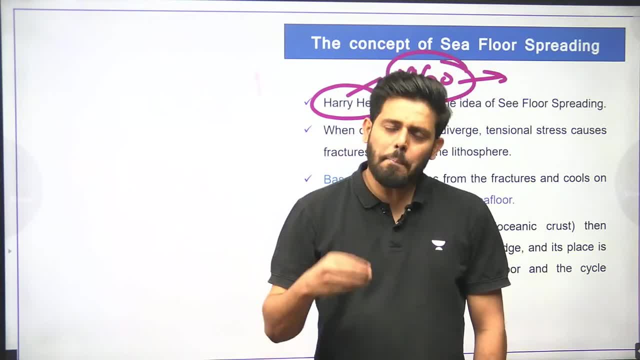 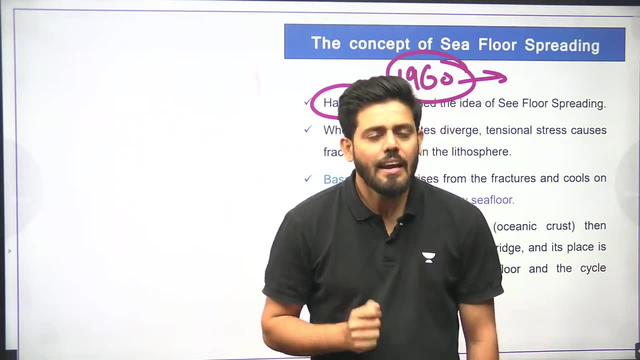 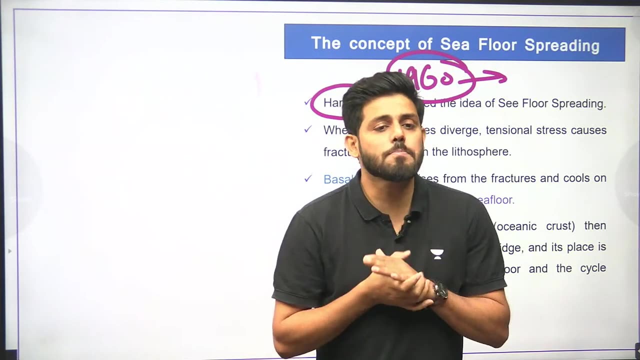 Then came a geologist. Try to understand. He was a professor, a geologist and an admiral of the Navy. His name was Henry Hess, Harry Hess. and Henry Hess brought a theory whose name is Sea Floor Spreading Theory. Remember. 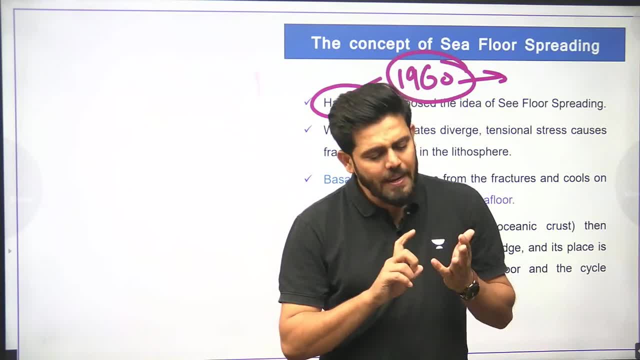 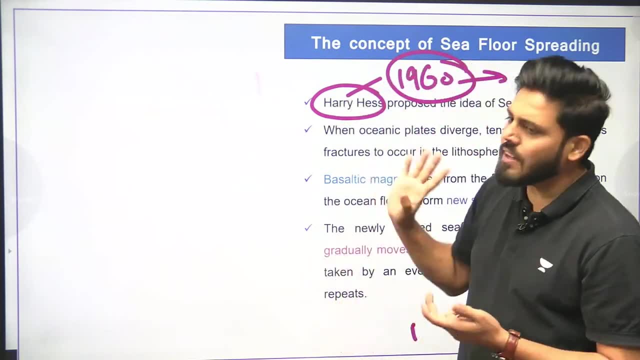 the plate tectonic theory that we will study in the future. in that plate tectonic theory convection, current theory, in that plate tectonic theory sea floor spreading theory and in that plate tectonic theory all the concepts of paleomagnetism. 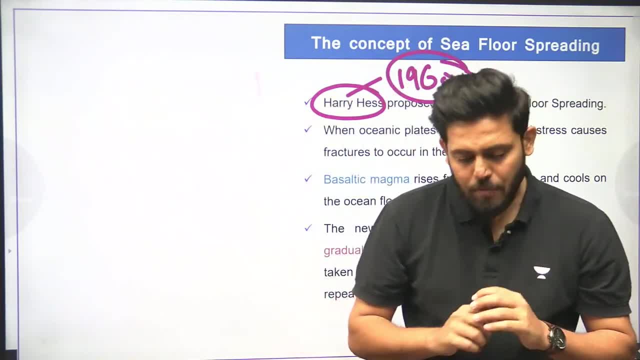 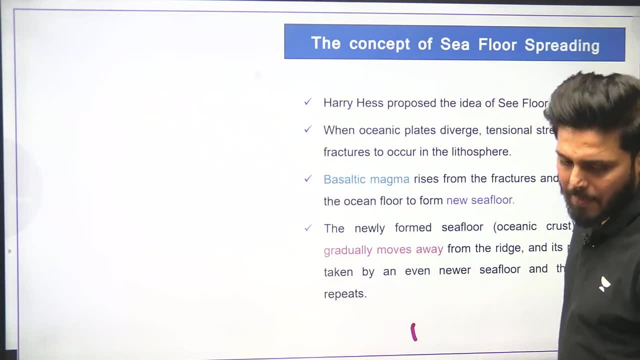 were your concepts? Remember this: What did they do? What did they do? They tried to study things And then, when they studied, how did it happen? We will talk about it. The biggest drawback of Alfred Wagner and your convection: current theory. 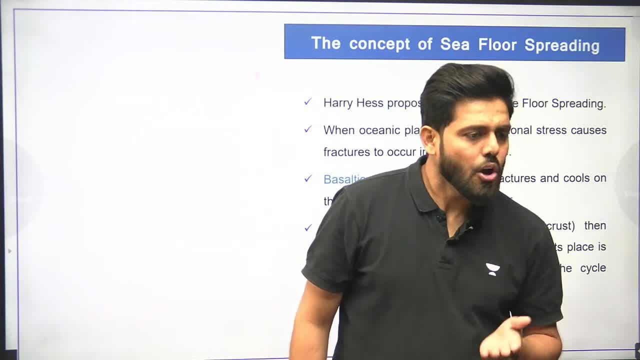 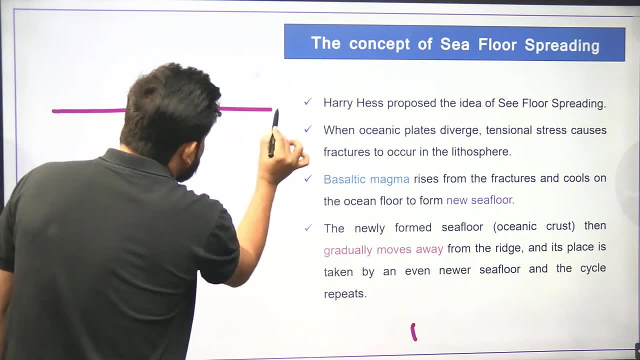 in that such a thing was not discussed about oceans, In that oceans were not discussed, They discussed about oceans. They said: look the convection current theory given by Arthur Ohms. when I went inside the ocean with that theory, 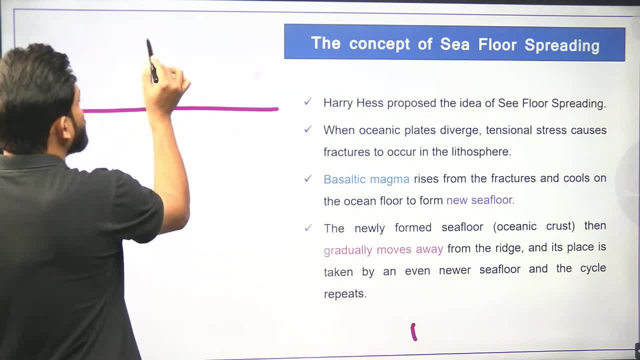 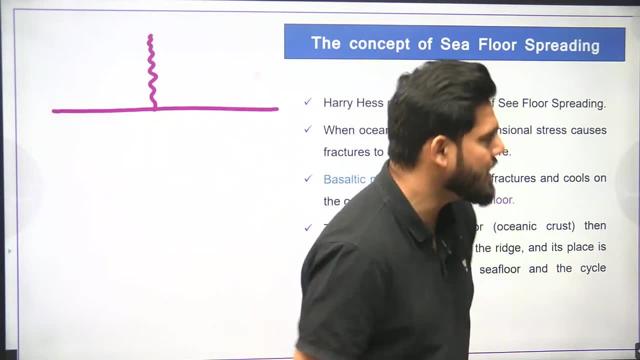 and I studied it and I studied it. so what did he do? He found that in that study, he found that there is a mid-oceanic ridge. He found that the mid-oceanic ridge is Now on both sides of that mid-oceanic ridge. 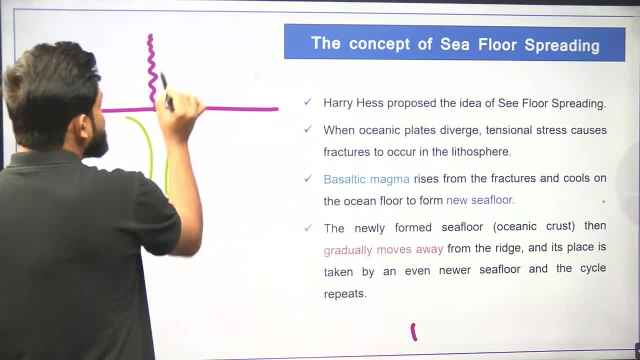 when from here there is a rising limb and on both sides of it. when he studied the rock sample, now the magma came out from inside. the magma came out and became solidified And after being solidified, when he studied, 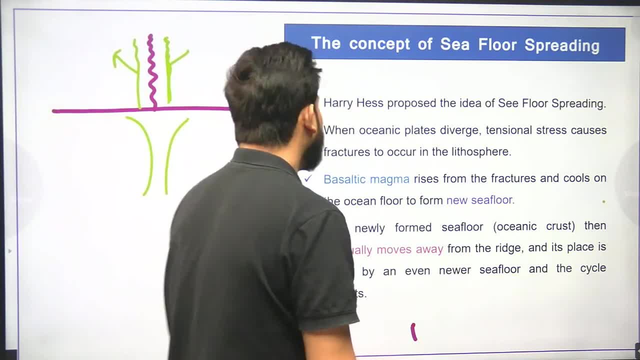 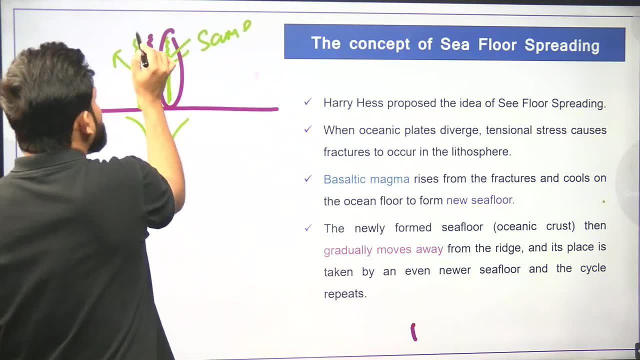 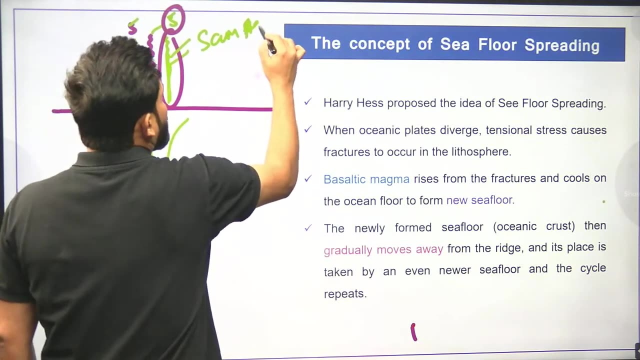 this rock. he found out that, brother, that the rock here is of the same age means the mid-oceanic ridge, 5 km this way and 5 km this way. the rock samples that I have taken are of the same age and have the same chemical properties. 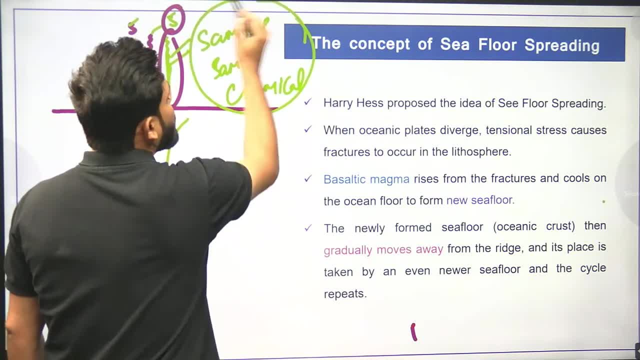 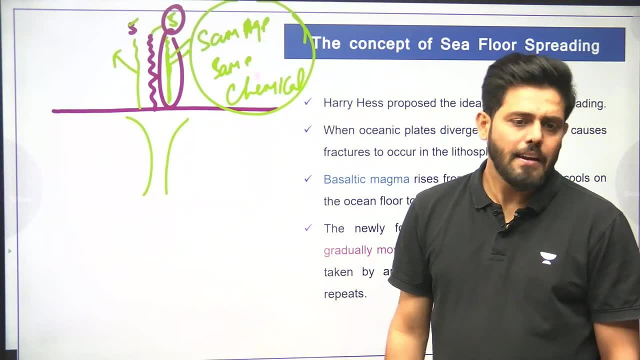 means they found out that our rock is of the same age and has the same chemical properties. they saw this. where did they see? they saw inside the ocean. where there are mid-oceanic ridges, there are elements of the same age and same chemical properties. 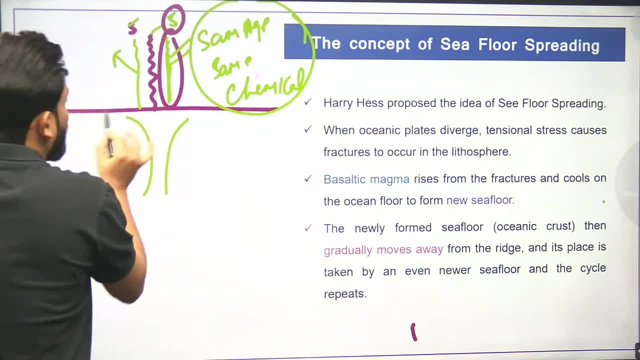 then they studied more. they saw that the rocks- this is the mid-oceanic ridge, here also this: what is on both sides this area is of rock. they saw that one rock is here and one rock is here. they saw that the mid-oceanic ridge. 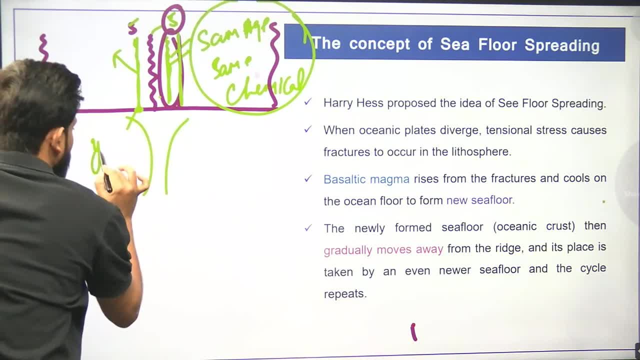 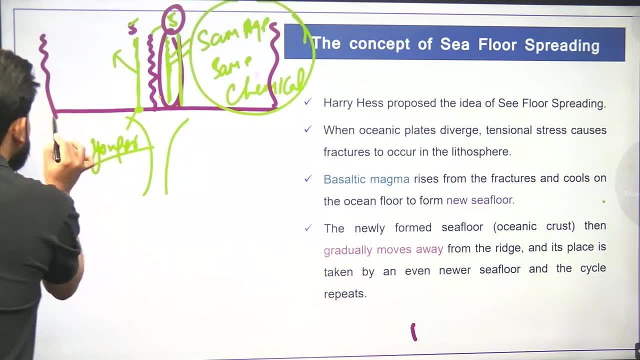 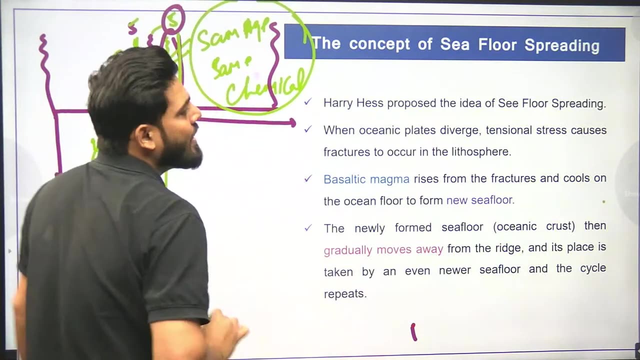 its near rock is younger means the mid-oceanic ridge, its near rock, its age is less. and the rock which is far away is older means, as we are moving away from the mid-oceanic ridges, our rock is getting more and more. this means, they said, 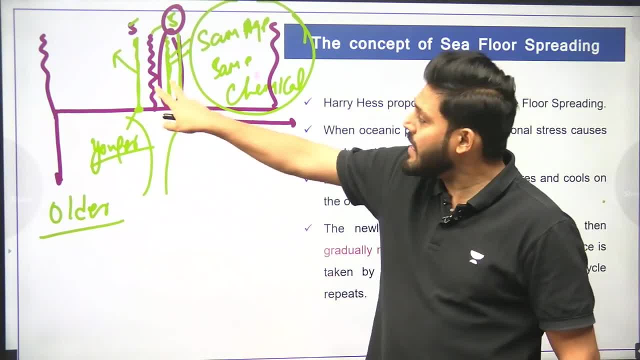 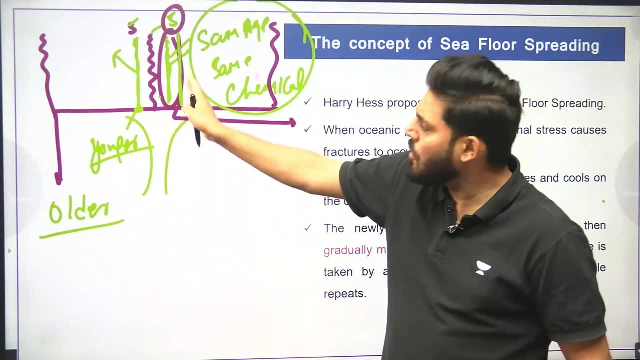 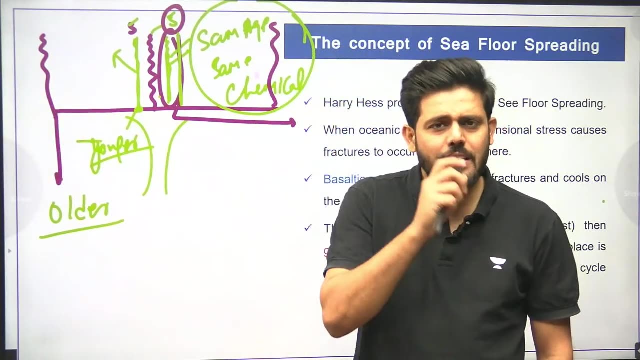 from where our mid-oceanic ridges are. new rock is coming out, new magma is coming out, it is getting solidified and after that, our age, that old rock. we have to look on the other side. so they said, this means our ocean is getting spread. 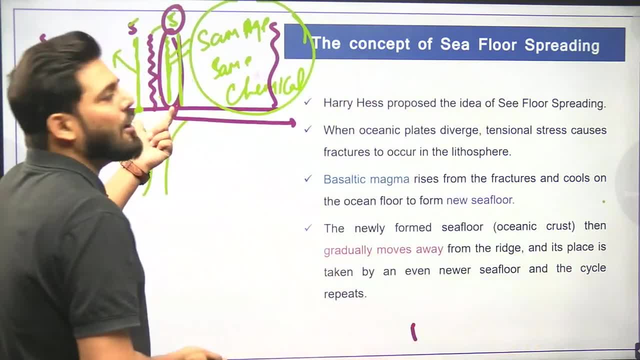 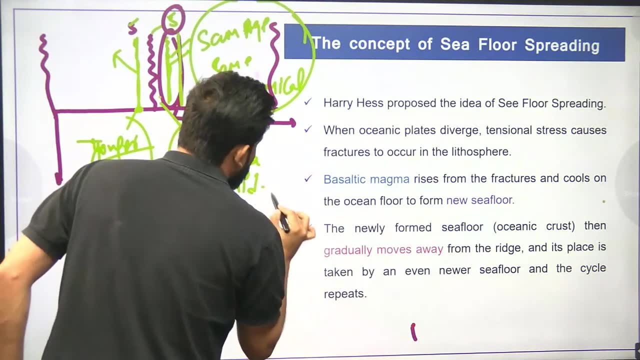 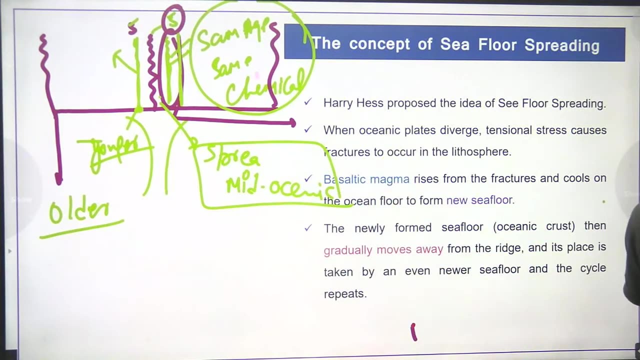 what did they say? that our ocean is getting spread, and where is it getting spread from where? from mid-oceanic ridges. they said that our ocean is getting spread, and from where is it getting spread? from mid-oceanic ridges. 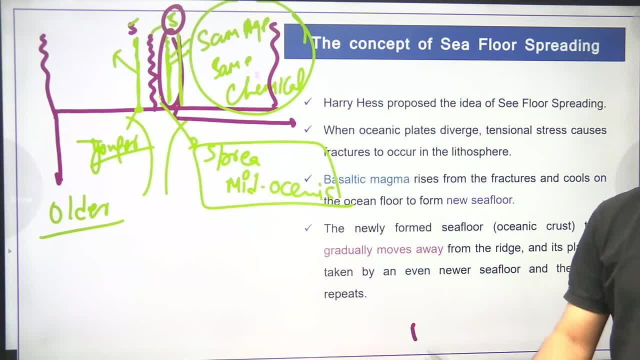 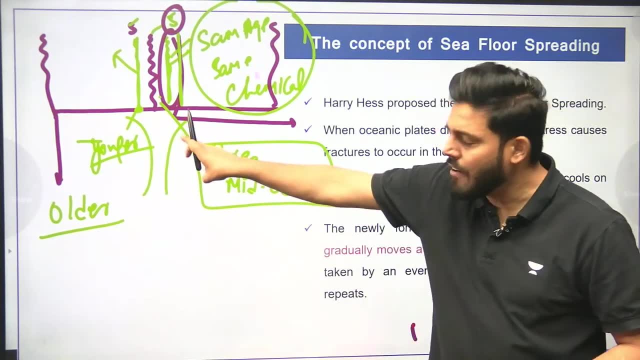 who told this? Henry Hess. he told that our ocean is getting spread from the mid-oceanic ridges. then he told the next thing. he told that the eruption of lava is happening from the mid-oceanic ridges. this means it has younger rock. 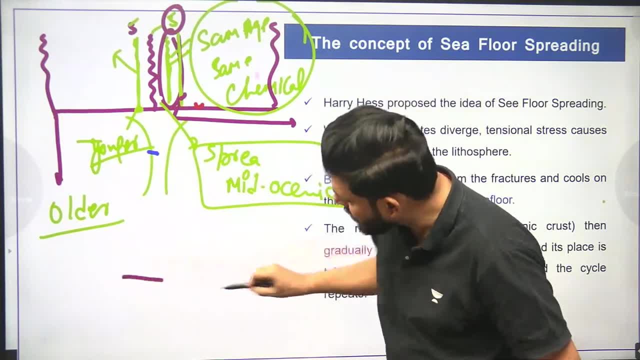 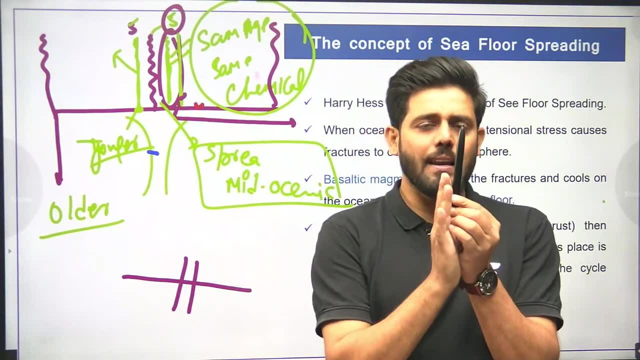 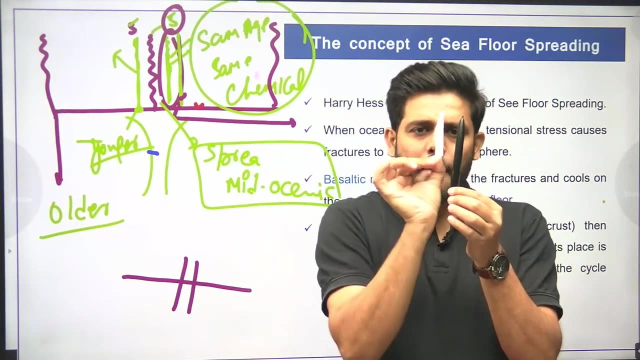 whose age is new, because if you study things, the rock which came out from here now- I will tell you that I have a point- magma came out from here now. this magma came out and deposited here like this is it clear: it came here and deposited when it came out here. 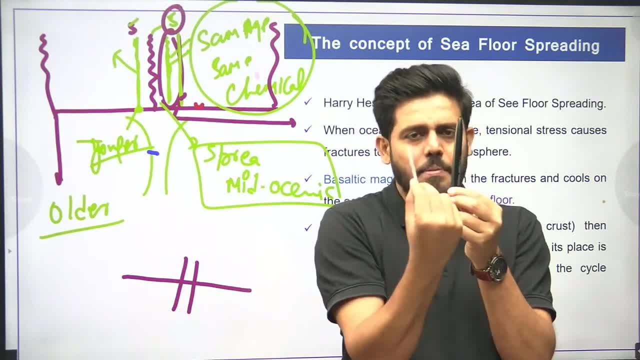 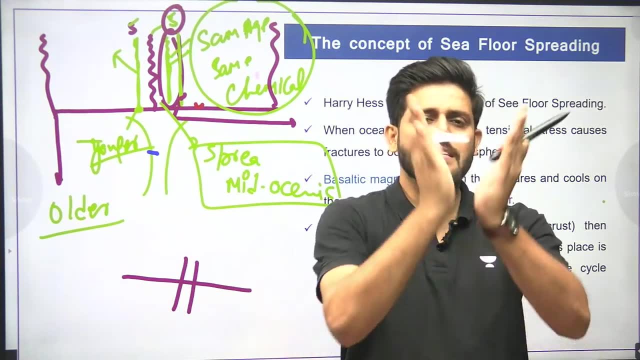 it will come out here also, so both are of the same age because it came out at the same time. if I am indicating here, you can take the same rock sample from here also, because magma will come out from the mid-oceanic ridges so it will deposit here also. 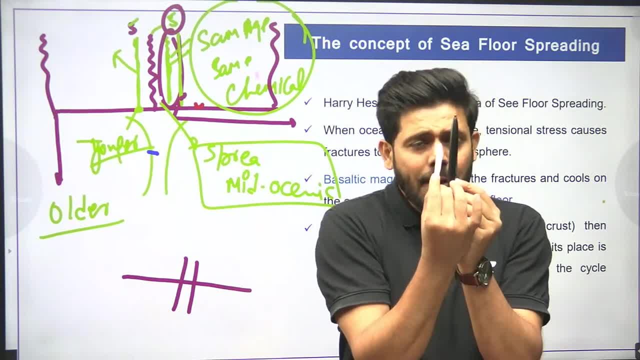 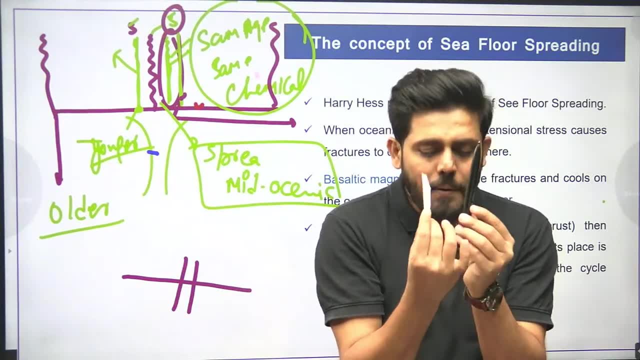 and here also now. magma came out from here and deposited here. now what will happen? after some time, magma eruption will happen again from inside, the interior of the earth, from where the oceanic flow is getting spread. so new magma will come out. so what will happen? 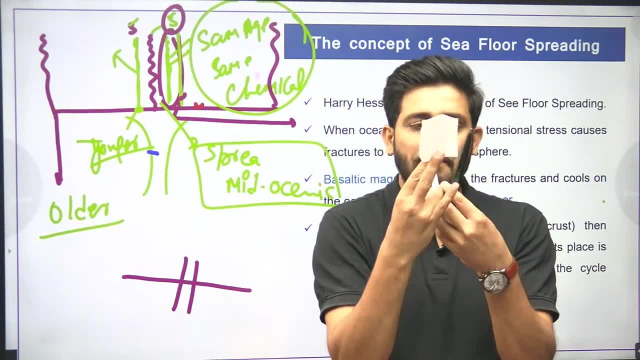 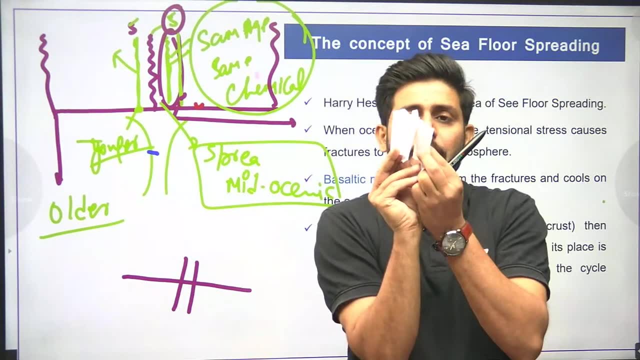 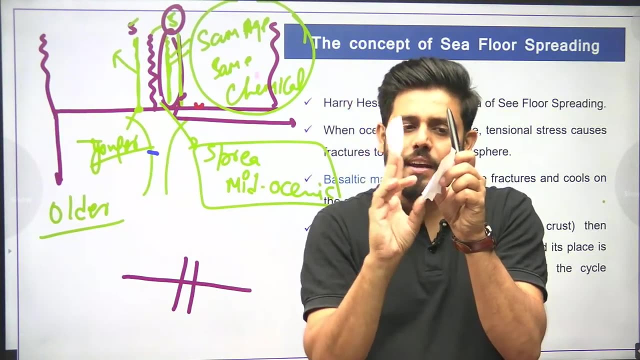 this magma will shift here and new magma will come here. now, what will happen after that? after some time, this magma will shift here. after that, new magma will come out, like this. so when they studied, they saw that the rock which I have- its age is old. 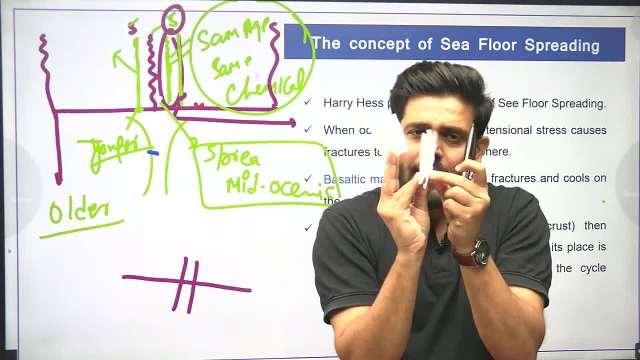 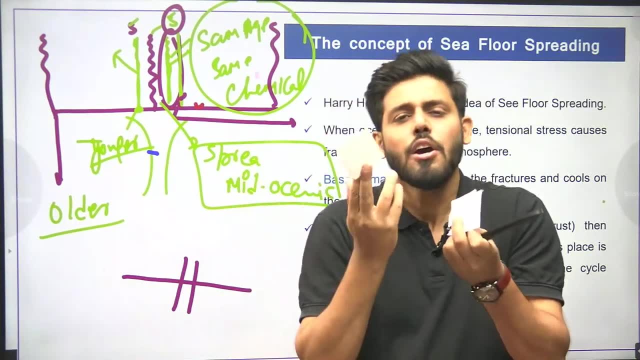 and, as the mid-oceanic ridge has this rock, I don't have this rock. why? because the rock which will come out here is new and, as you go further away, this is the previous rock. its age is older, so where did they find out? 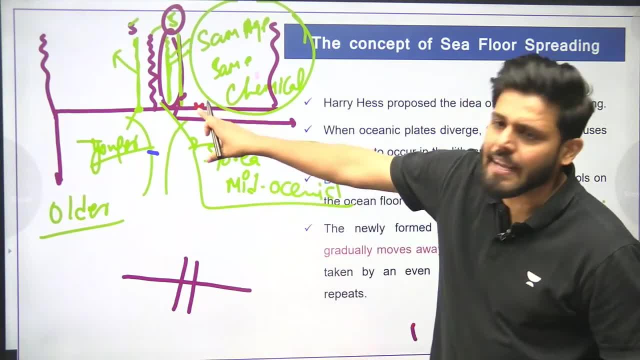 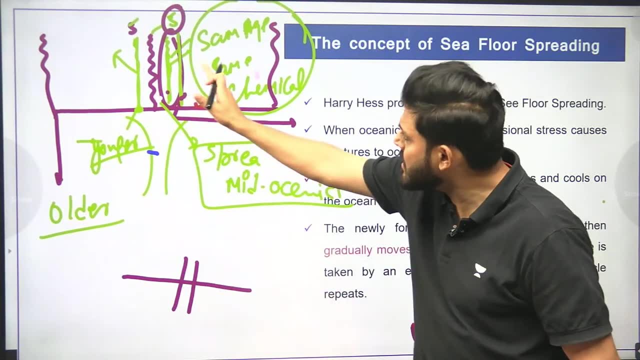 they found out by sea-flow spreading. they told that the rock which is here near the mid-oceanic ridge is younger. it is new and as we are going further away, its age is getting older. they told that the mid-oceanic ridge is erupting here. 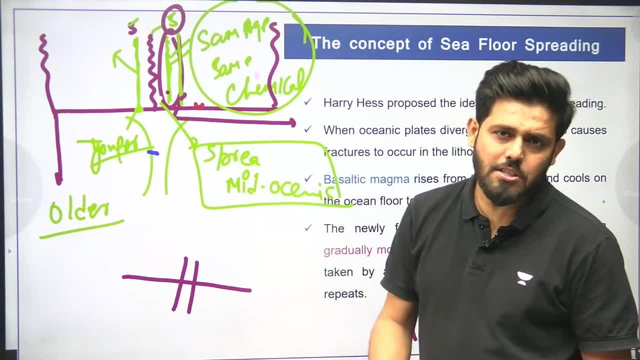 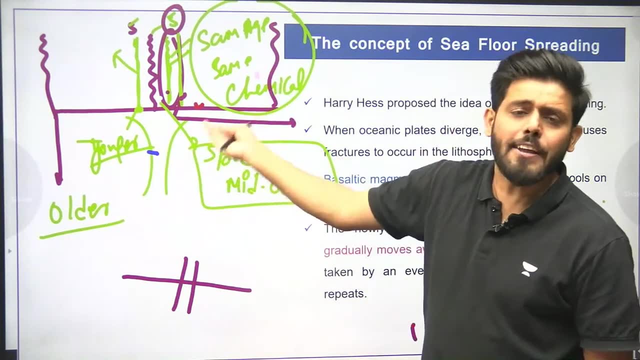 of magma, due to which new rock is getting formed here and the old rock is shifting further away. they told this, do you understand? after that, they studied. they found that the rock which is here is the mid-oceanic ridge. this is the mid-oceanic ridge. 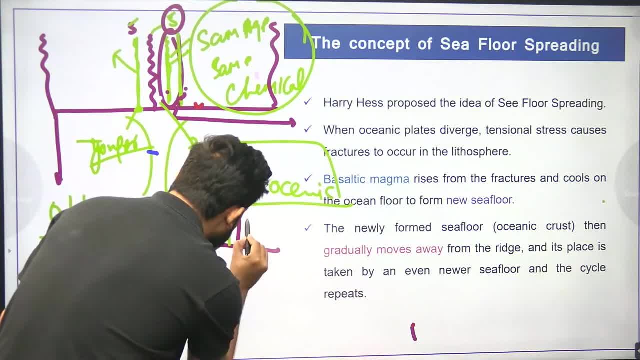 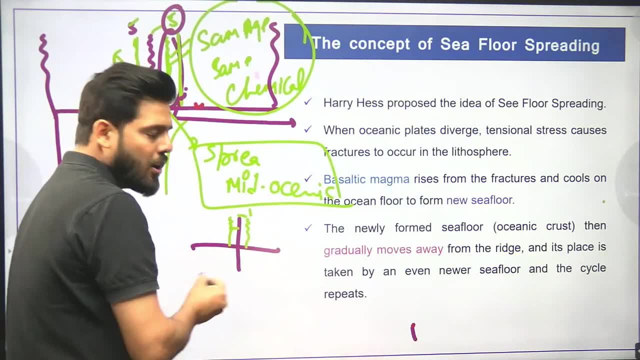 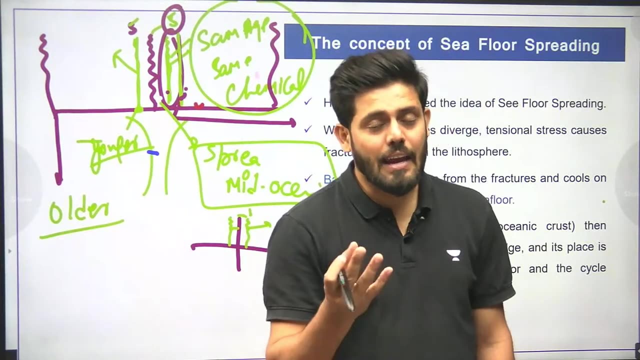 and they told that the rock samples of the mid-oceanic ridge are at equal distance means this rock is 1 km far and this rock is 1 km, so the equidistant rock. they saw a lot of similarities here. they saw the similarities that its chemical composition. 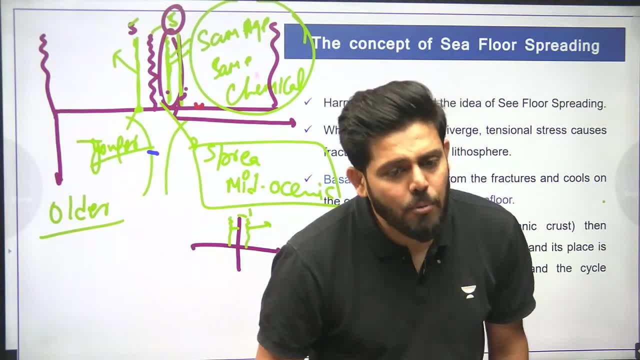 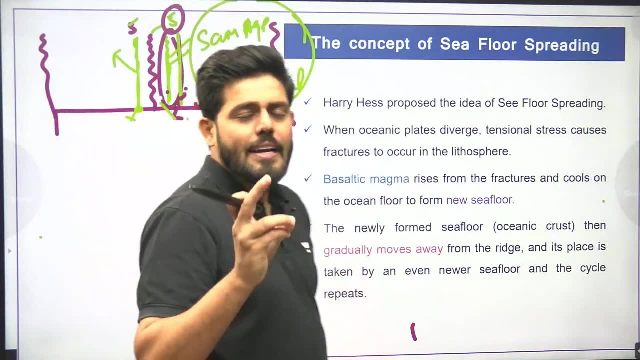 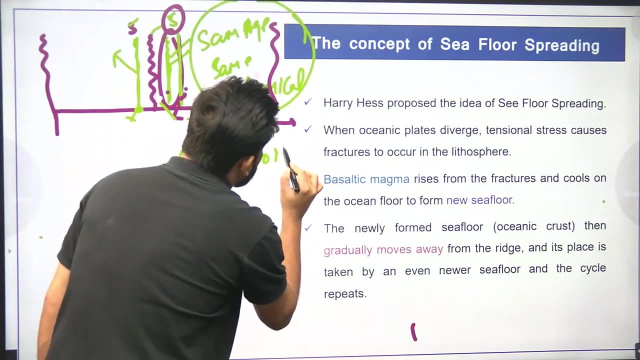 is same. its age is same. many similar things were found here. they noticed all these things, but they noticed one more thing. they said that when I took the sample of your continental crust, I saw that the rocks which are 200 million years old, the age of the rocks which are 200 million years old. 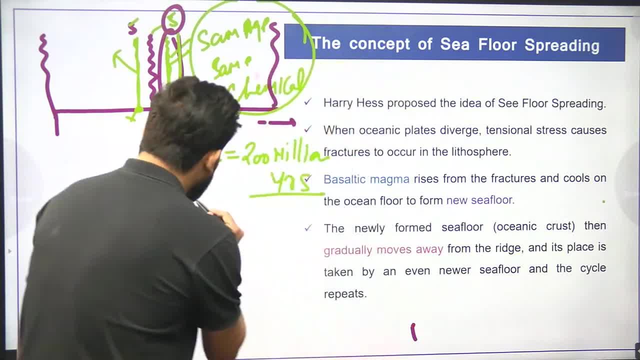 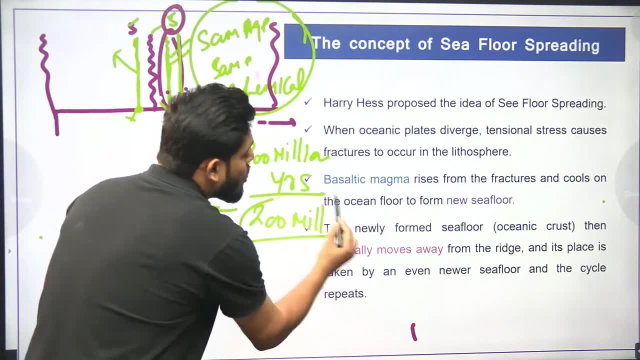 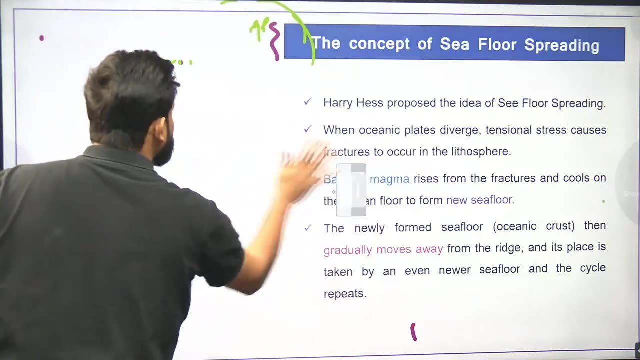 was found in the continental crust. but when I studied the oceanic crust I found that the rocks which are 200 million years old, I did not find them. so they later studied things and they found out that the mid-oceanic ridge, the mid-oceanic ridge, 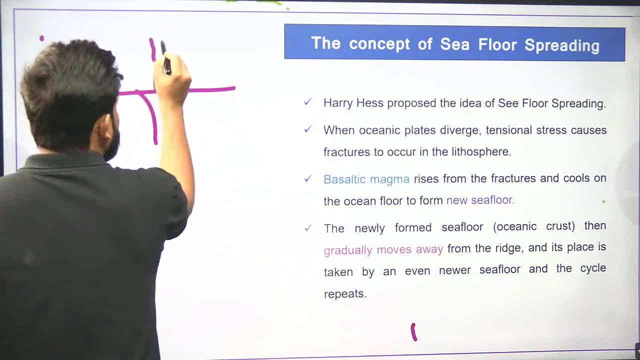 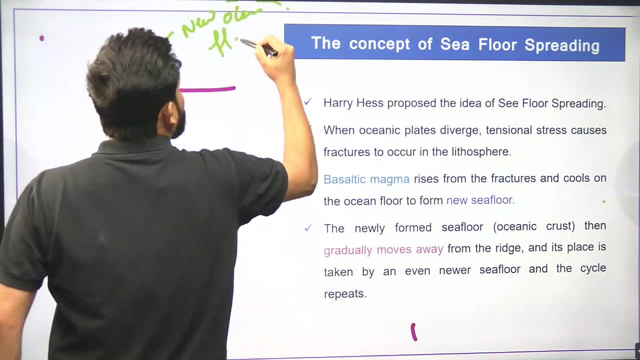 from where the lava is coming out, and this is the mid-oceanic ridge. it has a yanger. and what is happening here? our new oceanic floor is getting created. a new oceanic floor is being created, but they told that where this rising limb is. 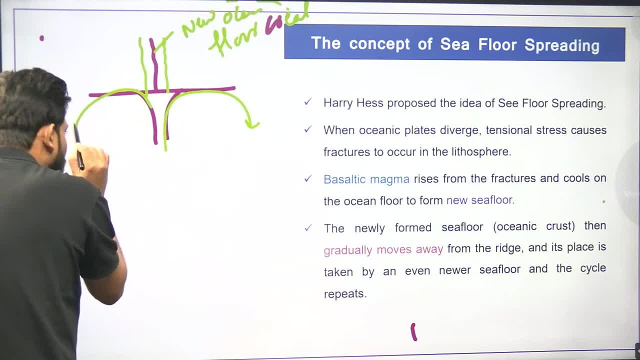 somewhere it will fall, somewhere it will fall, somewhere it will fall, and after that, somewhere it will fall. and where these falling limbs are getting, there are formation of trenches. and where the formation of trenches is happening, there is your oceanic crust. it is getting destroyed, it is getting finished. 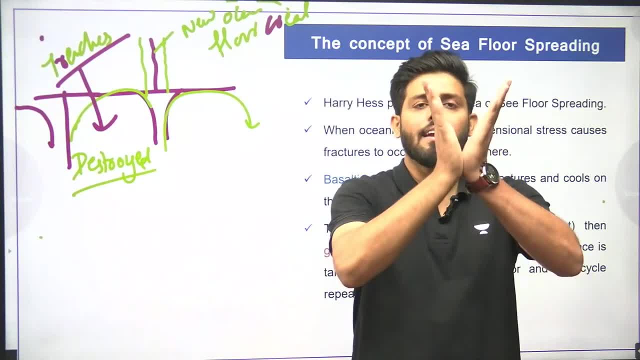 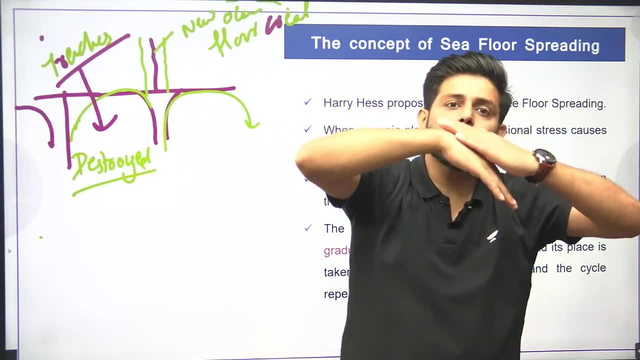 because when one floor, one crust is being created here, but when these two crusts come together and the falling limbs get together, then one crust will go under it and by going down, it will keep getting destroyed and will keep getting destroyed because of this where there are trenches. 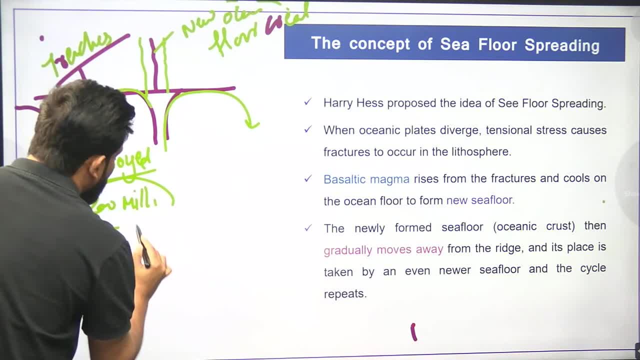 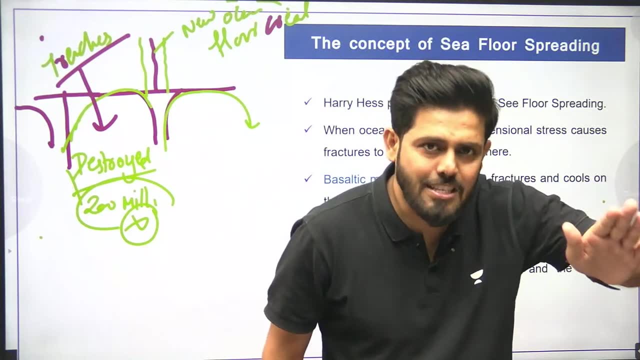 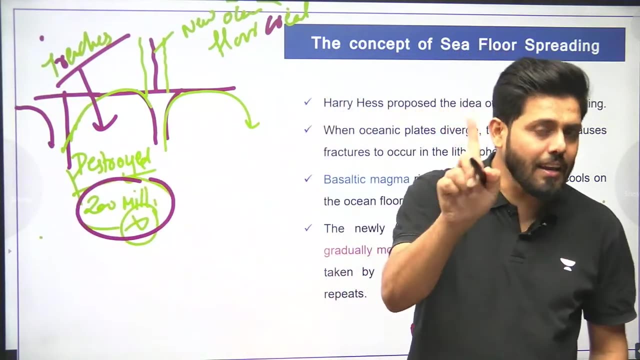 there are samples of 200 million years old rock. that is why they have studied that. the trenches are not seen on the continental crust, they are seen in the oceanic. that is why the oceanic rock is not 200 million years old and continental rock is 200 million years old. 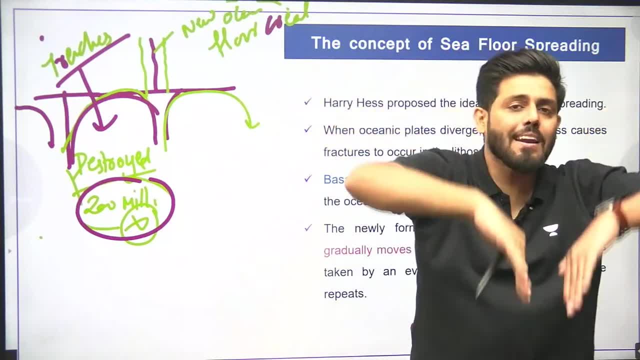 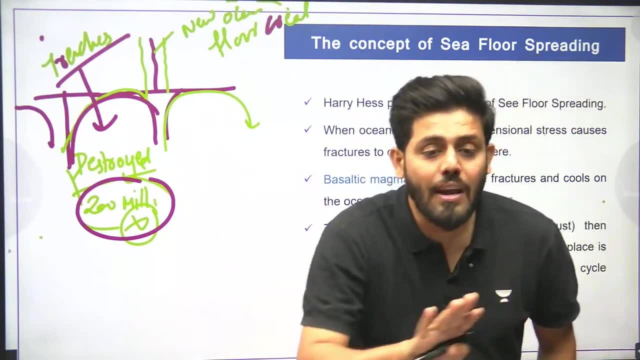 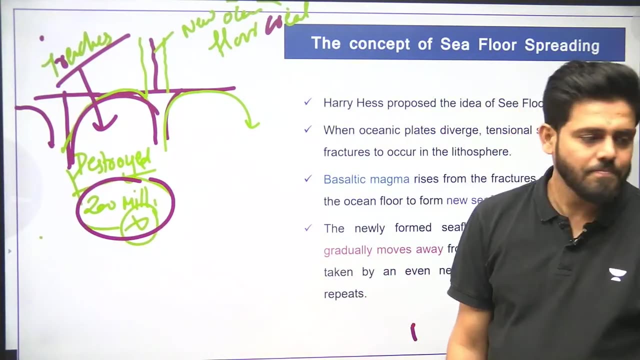 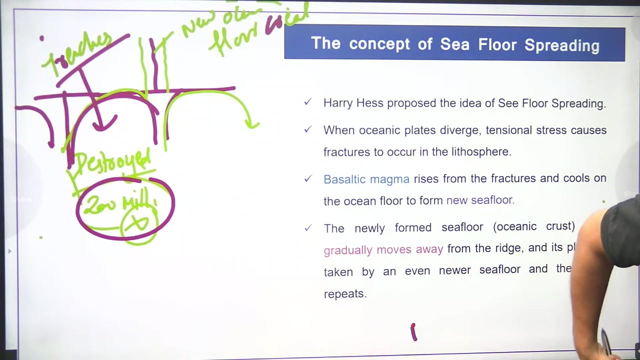 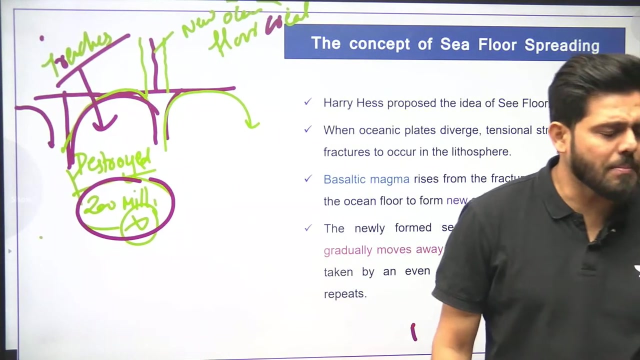 because where there are trenches, where falling limbs are getting, where convergence is happening, there that rock is getting destroyed and we are not getting evidence of that old rock. who told this? they told this. did you understand? if anyone has any problem, then tell me who all understood this. 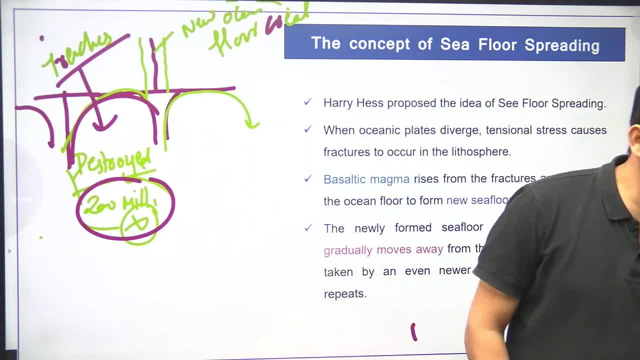 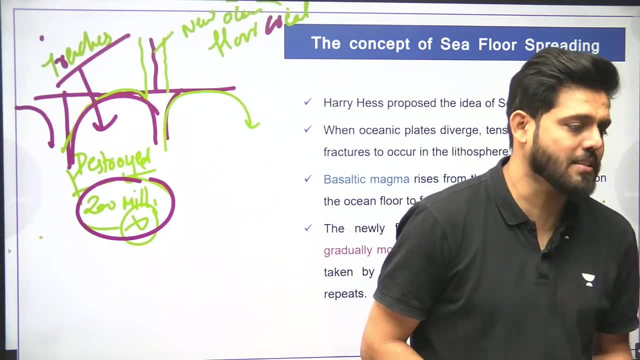 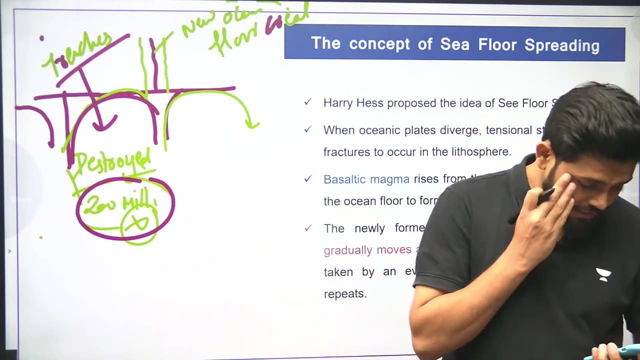 do like and share this video. if everyone understood this, do like and share this video and do comment. how many students understood this conceptual clarity? very nicely, the one who didn't understand you can tell me anyone of you that, sir, I didn't understand. please comment this quickly. 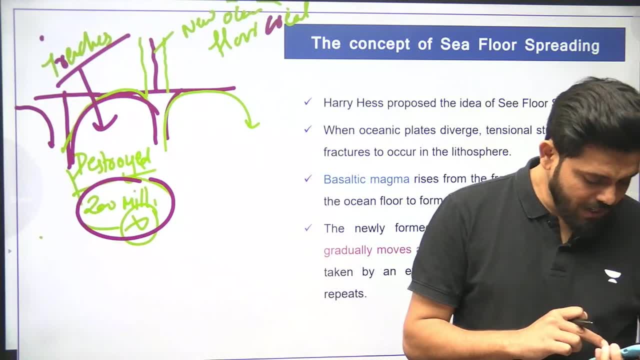 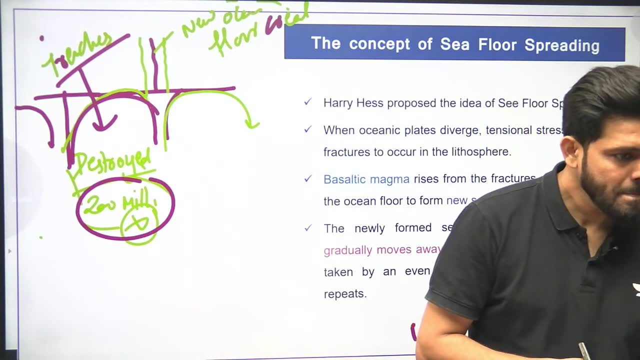 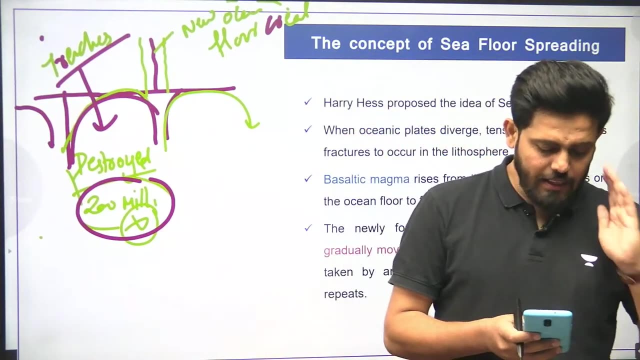 and all the students who understood, you can tell me, and those who didn't understand, you can also tell me. I will tell the trenches, I will tell you how the trenches are formed. I will tell you everything. just tell me here If there is any doubt here. 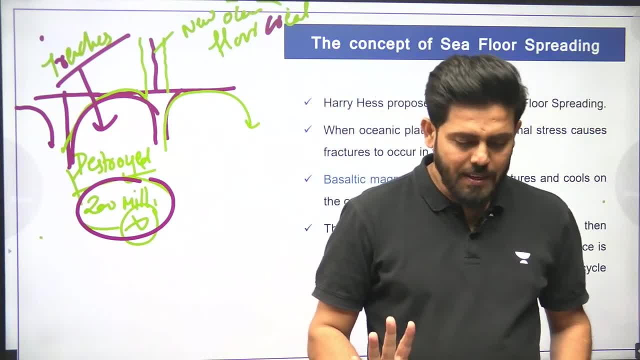 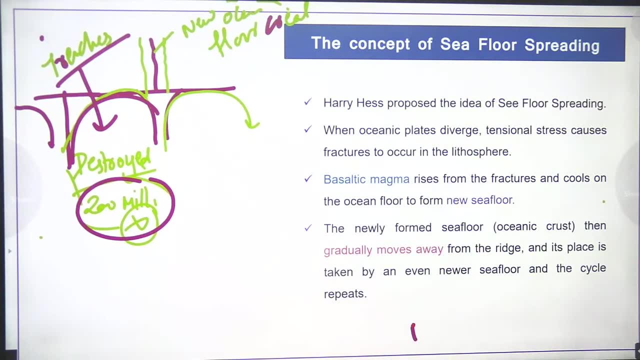 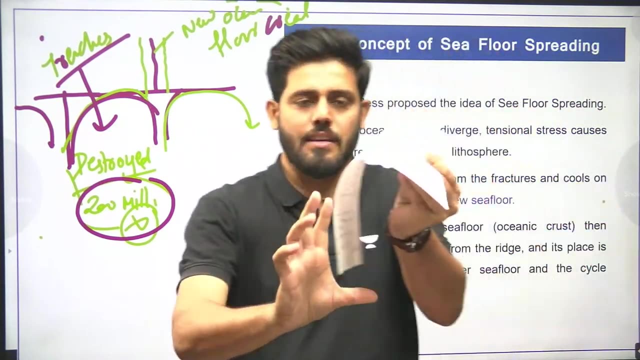 When you see here, try to understand. how should I explain to you What is the loom? Wait a minute, I will try to explain something nicely. This is our crust. He told me that when there is magma from the bottom, try to understand. 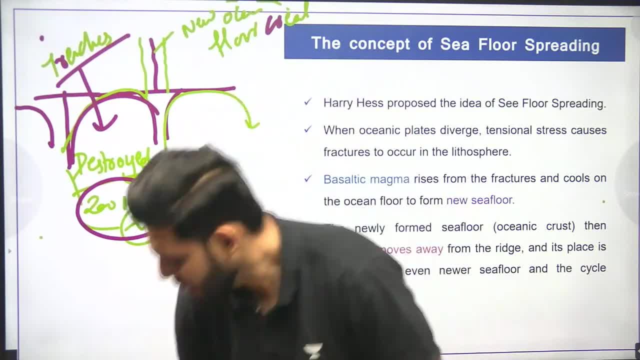 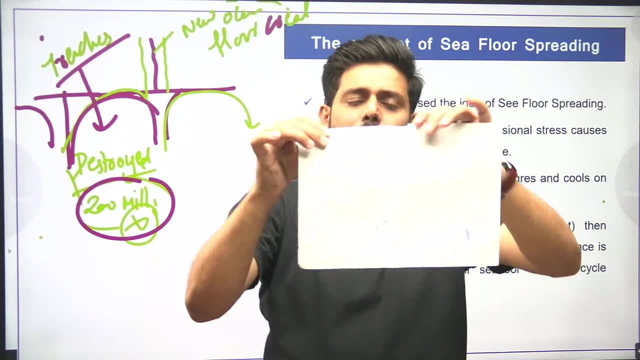 Magma will come out from the bottom, like this: Magma will come out from the bottom, Magma will come out from the bottom, Magma will come out from the bottom. So he told me that when our crust will break, like this: 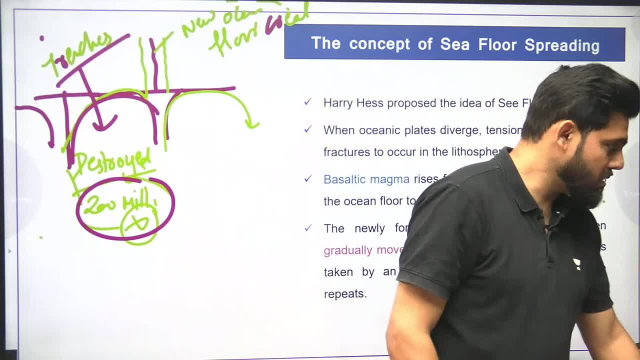 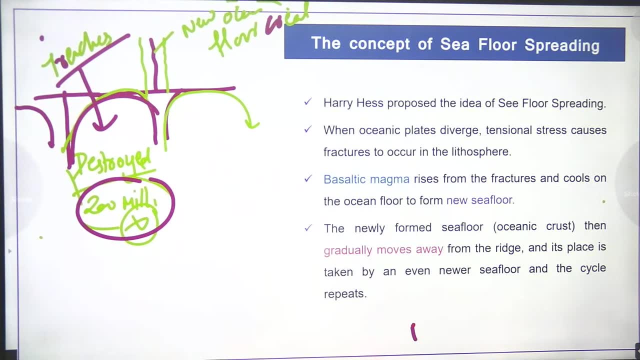 How can I explain to you? I will explain to you in some other way. Just give me one minute, Wait a minute. Just give me one minute. Just give me one minute, Wait a minute. See, this is our crust. This is our crust. 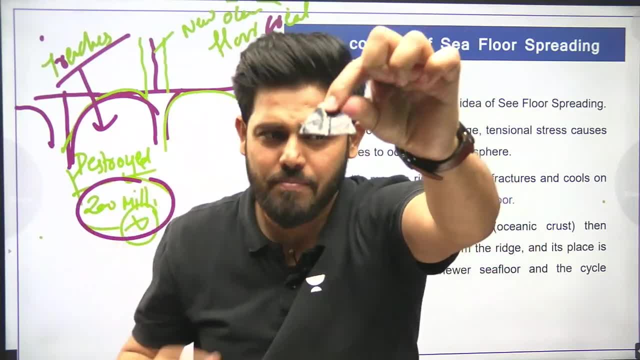 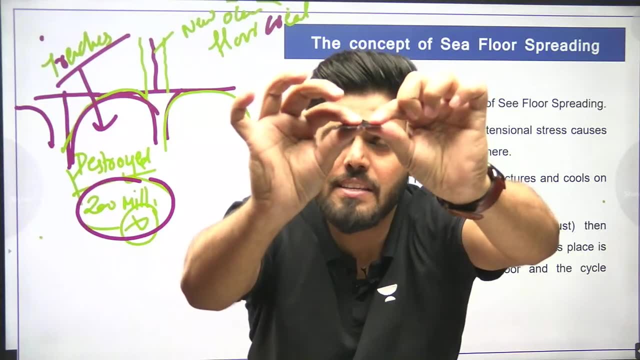 You can clearly see it. This is the crust of our earth. You can clearly see it. You can clearly see it. Now. the magma came out from the bottom. There was a rising loom. There was a rising loom From the bottom. the magma is doing one movement here and another movement here. 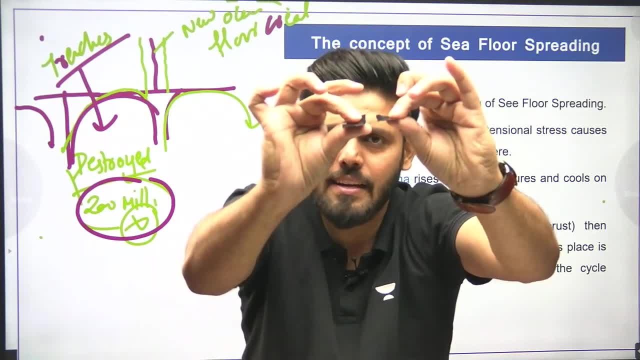 Now, if the magma comes out from here, then what will happen to this crust? In this way, there will be divergence. In this way, there will be divergence, But what is happening is that the magma is coming out from the bottom. 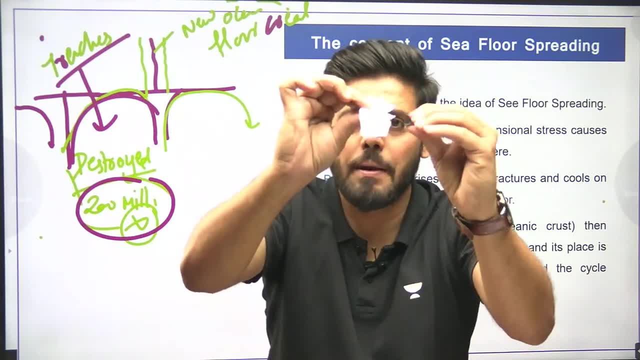 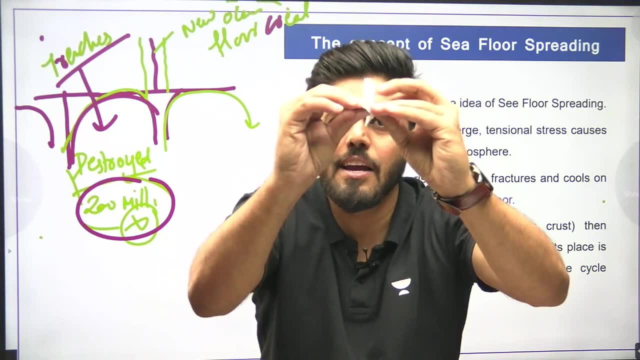 Continuous magma is coming out. So after coming out, that magma will solidify in the middle. So what happened here? The magma is coming out from this trench in the middle, Magma is coming out on both sides And our oceanic floor is spreading. 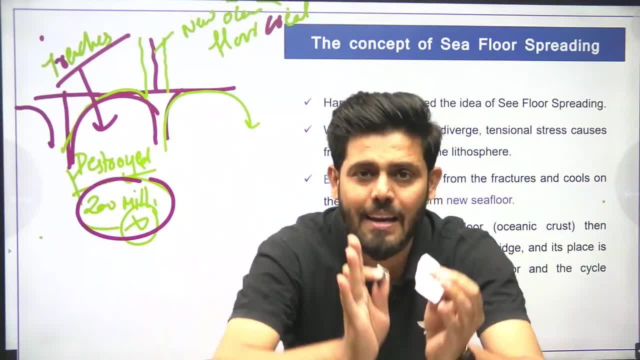 Magma is coming out from the bottom And the magma is also moving. Now the magma came out And after coming out, it will move in this way And it will move. The lithospheric plate on it will also move. 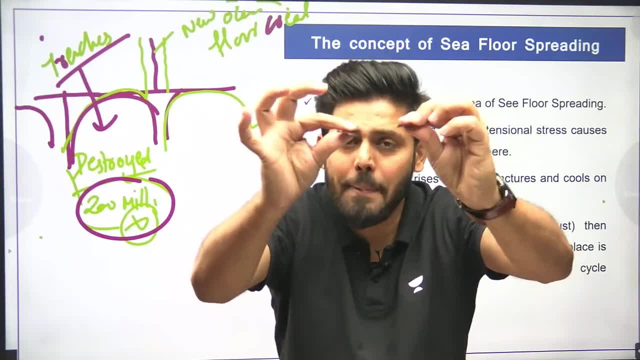 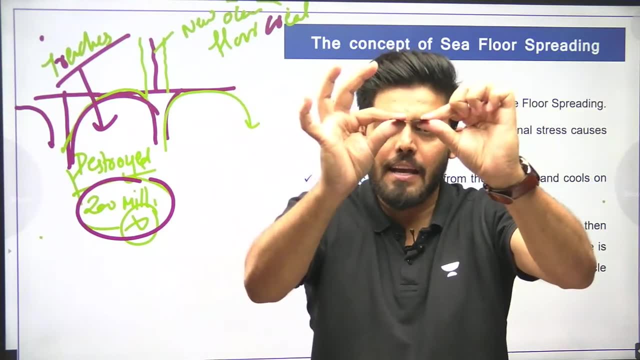 So our plate is moving in this way Now, both these plates are moving in this way. Continuous magma is coming out from the bottom. Now this much gap has come. Our plate was here. It has come here, The middle point of it. 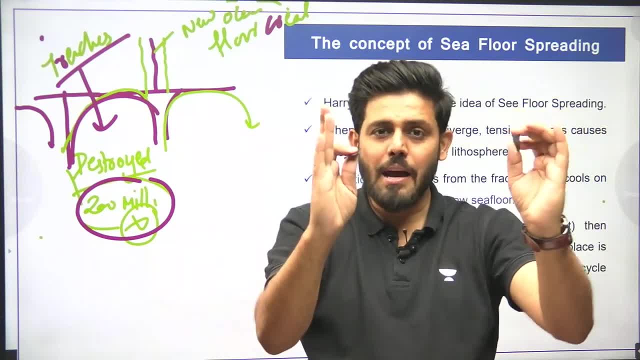 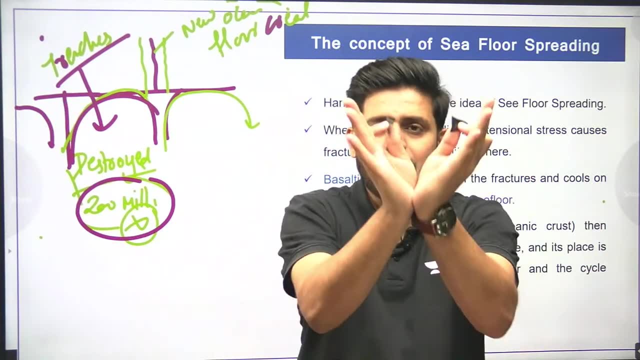 The magma has filled up here. So in this much gap, our new oceanic floor has been formed. In this much gap, our new oceanic floor has been formed. Now this magma will come out and rise in this way. It will come down here also. 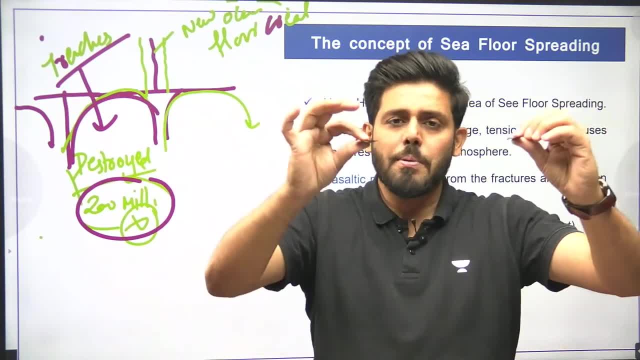 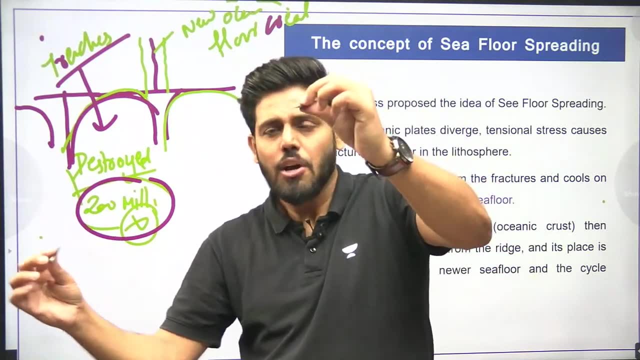 It has risen. Somewhere. it will also subside Now it has risen. So, coming here, When this magma came out in this way, This plate came out in this way, So from here also some other magma will be rising. 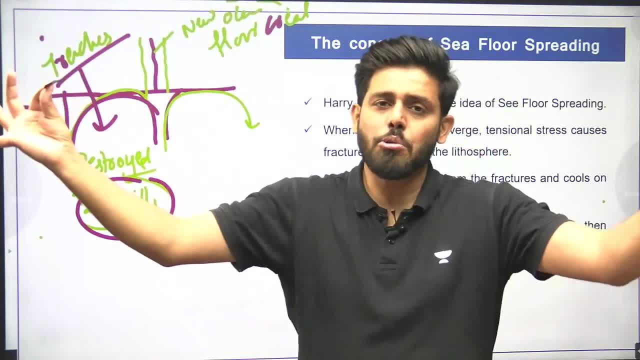 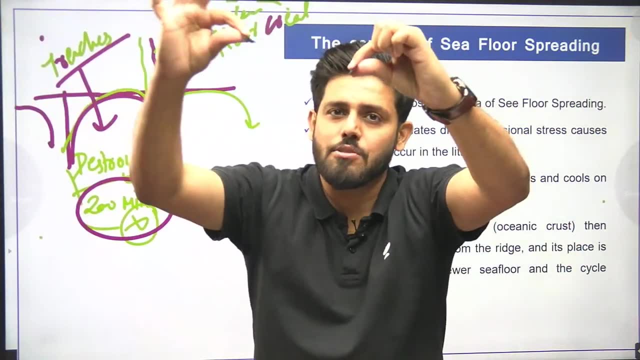 It will also rise here. It will also rise and come here. And when these two will rise and meet, By coming here, What was happening? Divers were happening, But by coming here, they will converge In this way. Now, if they will converge, 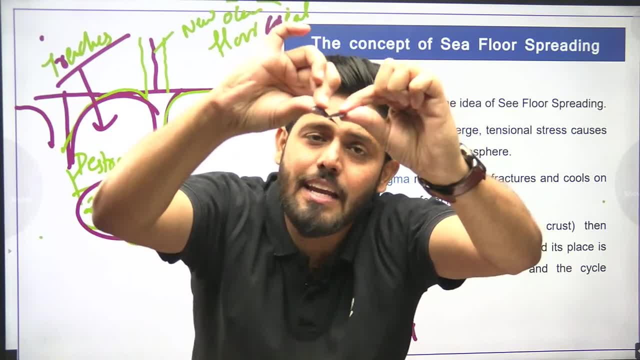 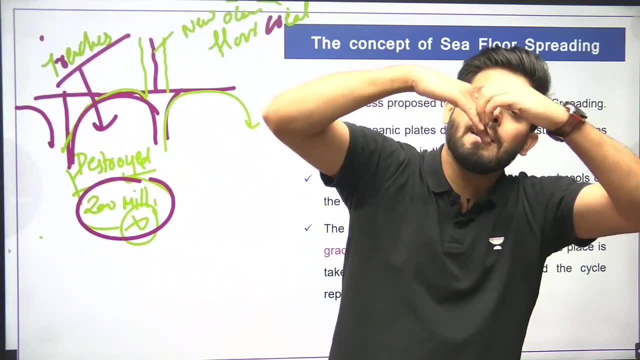 Then one plate will go down from the other plate, And when it will go down, Then it will be destroyed. It will be finished By going down. it will melt, It will be destroyed. Now, if it will be destroyed, Then a gap will be created here. 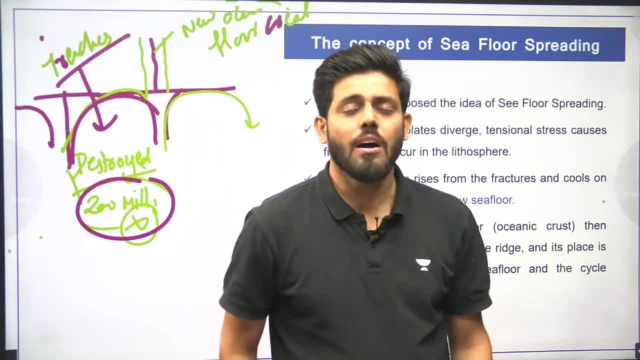 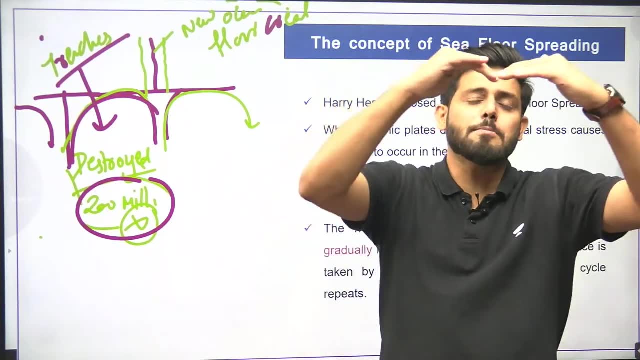 Which is called trenches. You must have heard about Mariana Trench. You must have heard about Java Trench. You must have heard about Aleutian Trench. These are the trenches when two plates collide, Due to which the formation of trenches happens. 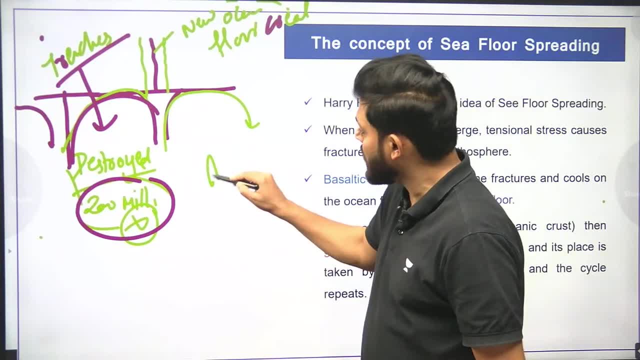 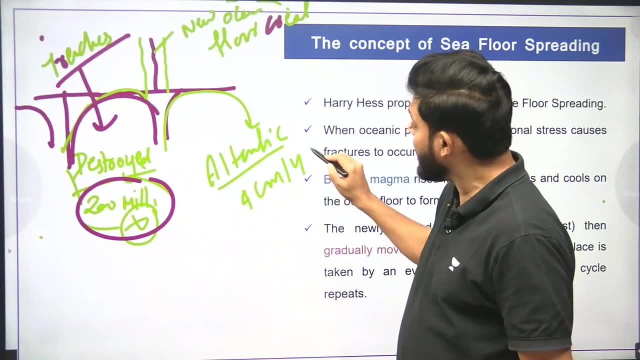 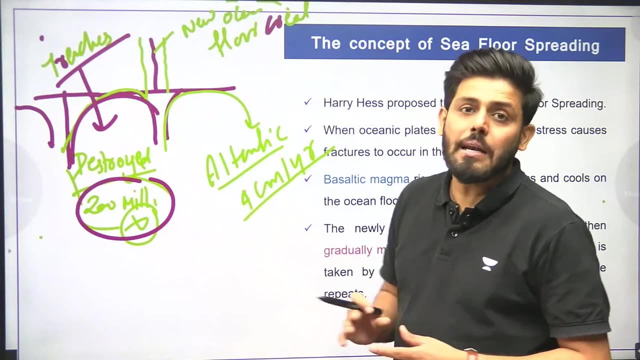 And you will read with things That our Atlantic Ocean, Our Atlantic Ocean. If you study things properly, Then it is spreading at a rate of 5 cm per year. Atlantic Ocean is spreading at a rate of 5 cm per year. I will give you a very good example. 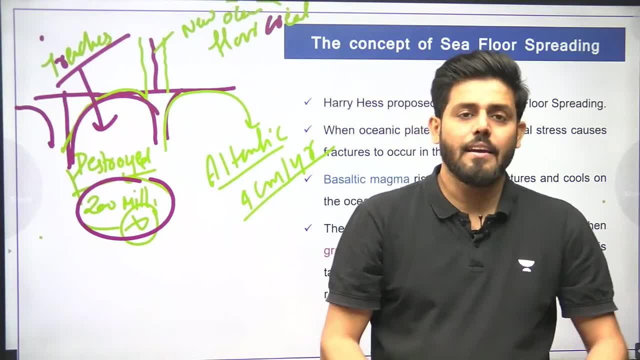 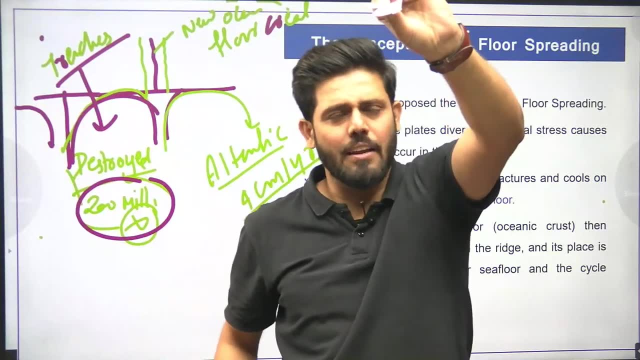 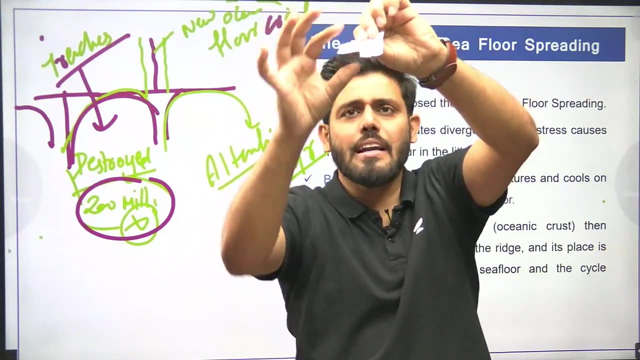 See here, See here, This is my one. What is this? This is my one plate, Oceanic plate. Try to understand. You can say: What is this? This is my continental plate. Now, there is magma under this continental plate. 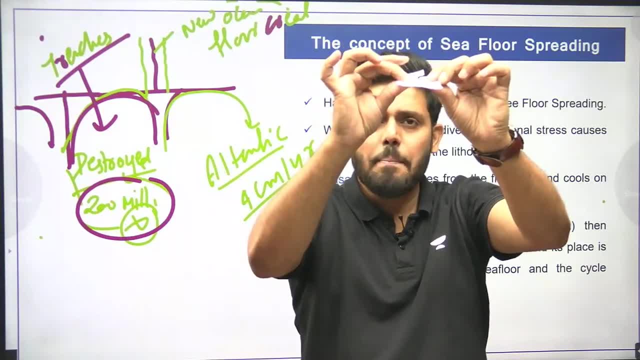 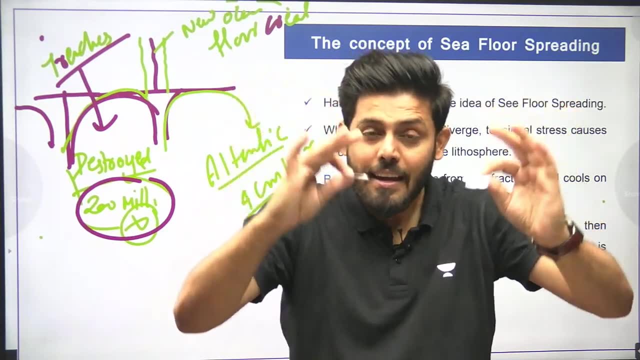 Now, what has this magma done? It has started to rise. This plate will go this way. This plate will go this way. Now. both plates are going separately. Now you understand The middle part of this plate. This gap has been made. 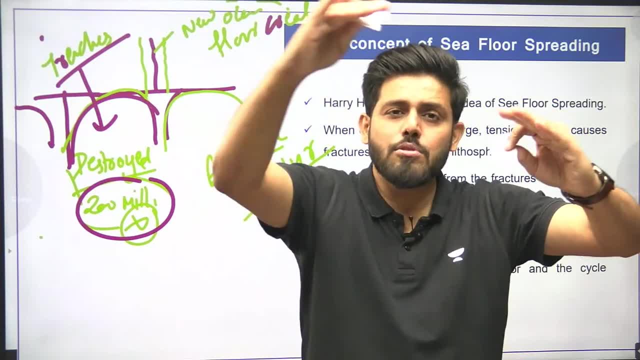 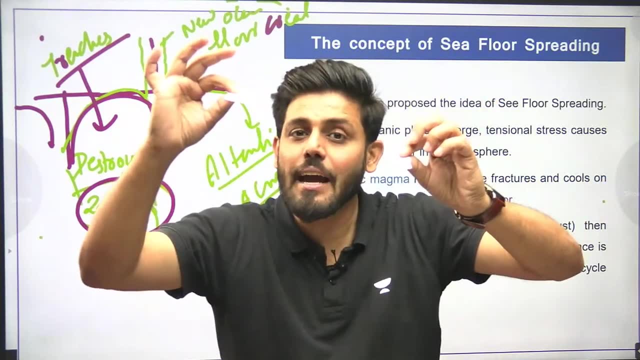 What will happen here? There is a floor below, But water will fill up on it. Water will fill up. So this portion of yours, What is different from this? Africa? Africa, And what is this made of? This is made of South America. 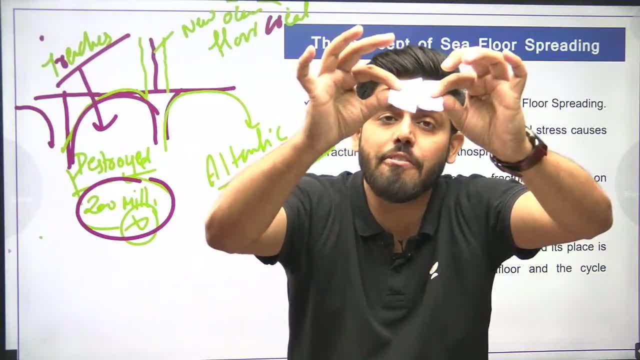 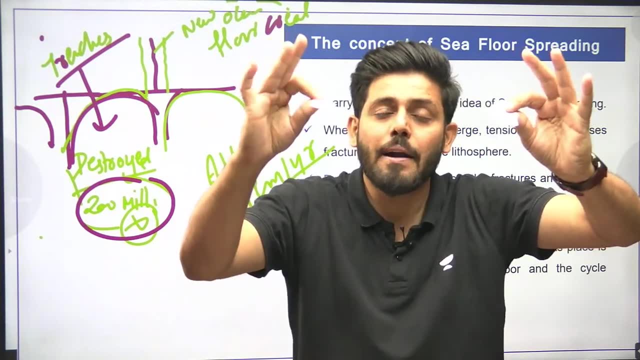 And see the jigsaw fit of both of them. It will fit What Alfred Wagner said. Now both will be different. The magma below will come out. Oceanic floor has spread, But the water has filled up in the middle part of them. 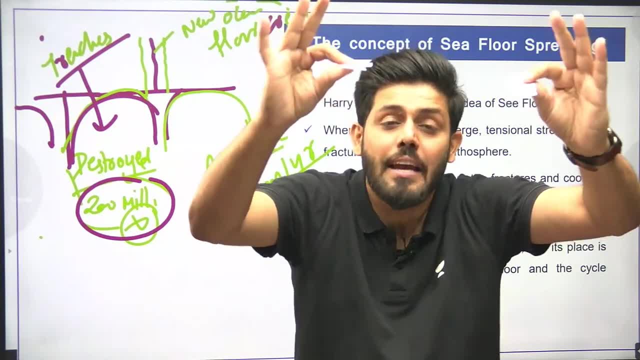 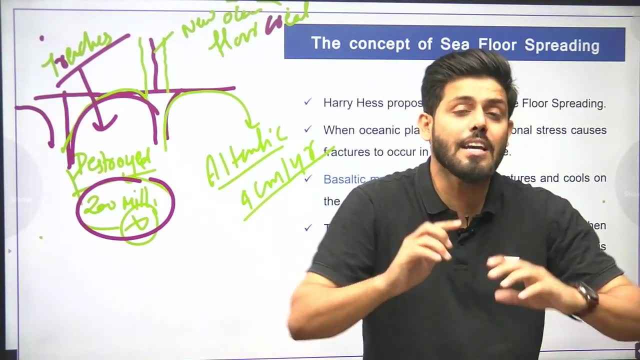 Of the ocean, That water has come and filled up there, Due to which The part of the middle part of both of them Has been taken by the Atlantic Ocean, And even today the mid-oceanic ridge Is actively working. Due to which The Atlantic Ocean, With the speed of 4 cm per year. What is it doing? It is spreading. If you read about the Pacific Ocean, Then the Pacific Ocean Is spreading at a rate of 12 to 15 cm per year. 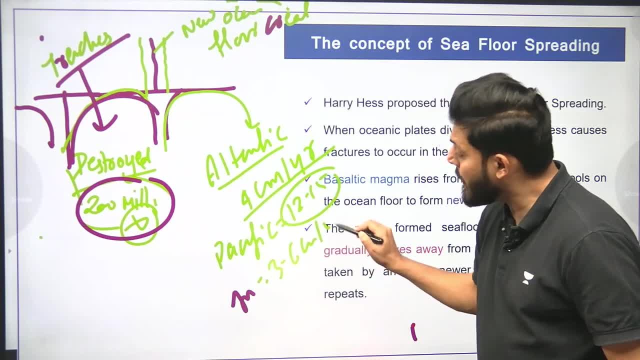 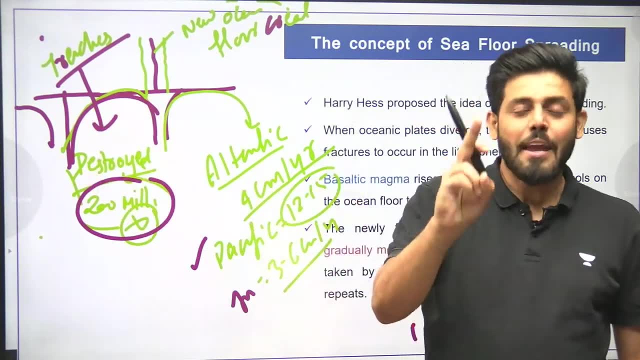 And if you talk about the Indian Ocean, Then it is spreading at a rate of 3 to 6 cm per year. So this means that the Pacific Ocean Is getting bigger. No, In the Pacific Ocean, The mid-oceanic ridges are active. 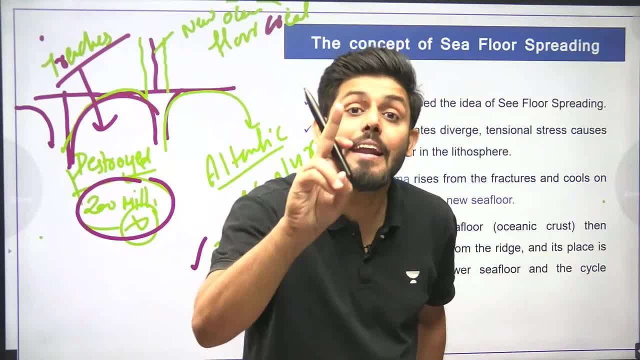 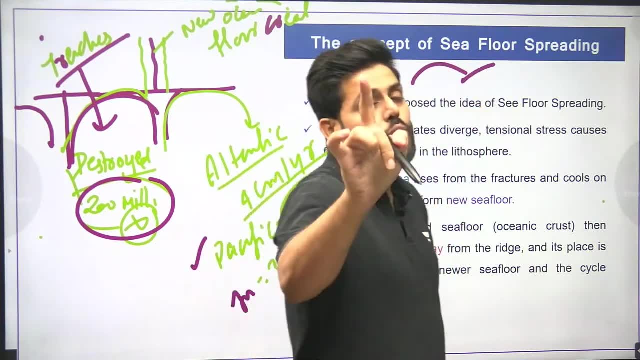 They are spreading it at a very high rate, But there are the most of the trenches, Due to which, when it spreads, Then the size of the trenches Is getting destroyed, Because of which The Pacific Ocean Is not getting spread. 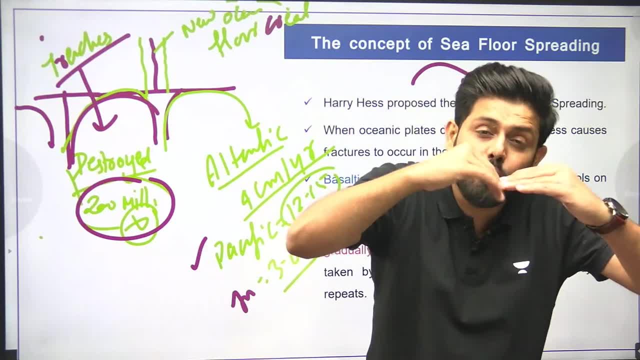 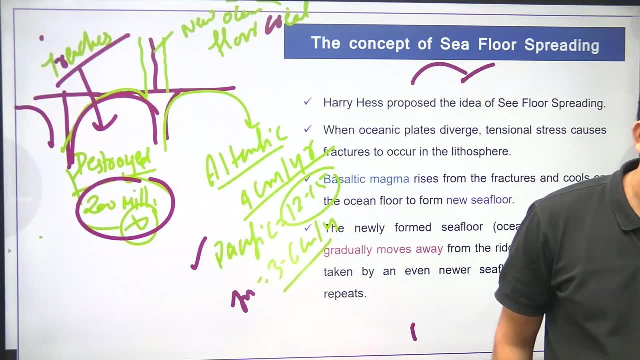 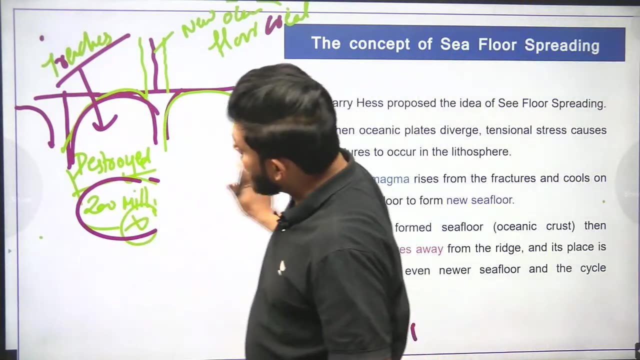 But it is getting sink, Due to which The submersion of the oceanic floor Is happening on those trenches. The submersion is happening on those trenches. Did you understand? The meaning of ridges is When the magma will come out from where. 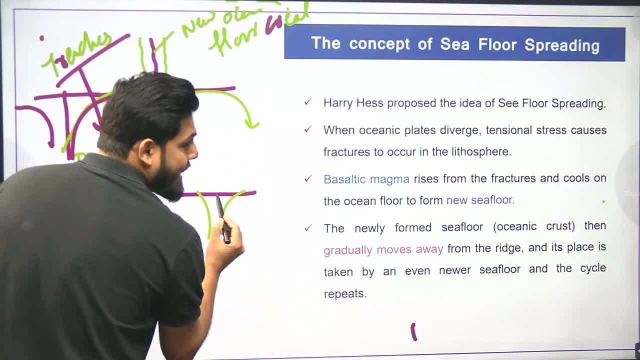 When the magma will come out from here, Then it will crack this crust And after cracking The magma which will come out from inside, It will make ranges in the mountain type. It will be called mid-oceanic ridges. First of all, this ridge. It was found in the mid of the Atlantic Ocean, Due to which it was named as mid-oceanic ridges, But as we moved ahead, Then we found out That these ridges are in the Pacific Ocean. These ridges are also found in the Indian Ocean. 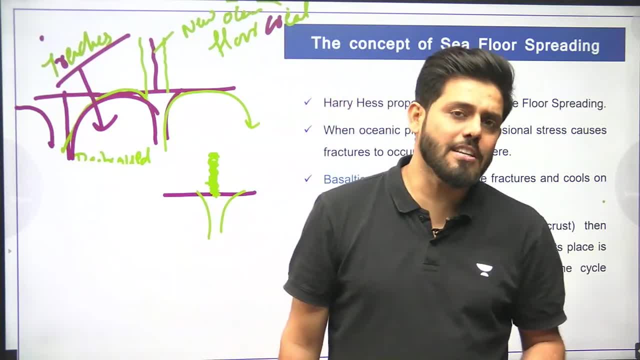 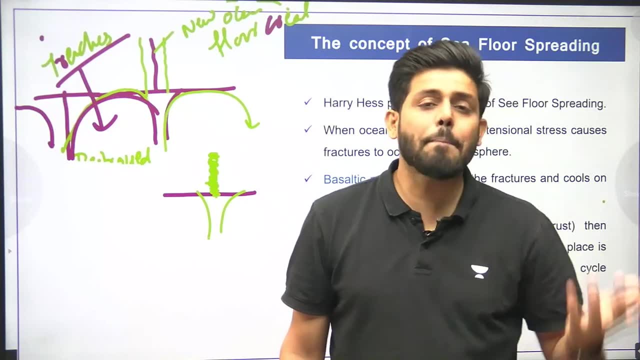 But they are not found in the mid, But, as in Indus Valley Civilization, In Indus Valley Civilization, If I talk about Indus, We call it Harappa Civilization, Which is the first civilization, city, Harappa, In the name of that civilization. 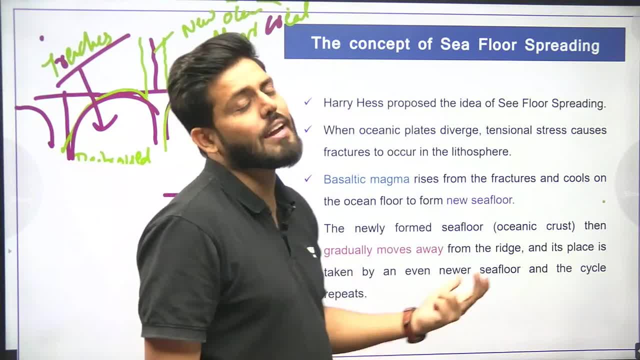 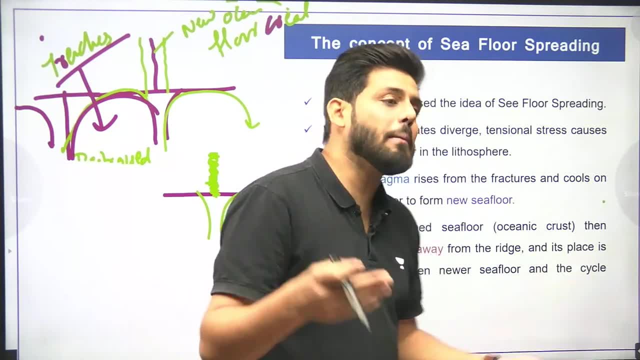 In the same way, Mid-oceanic ridges were kept Because it was found in the mid of the Atlantic Ocean And after that It was found in the Pacific and Indian Ocean, But not in the mid At the other point. 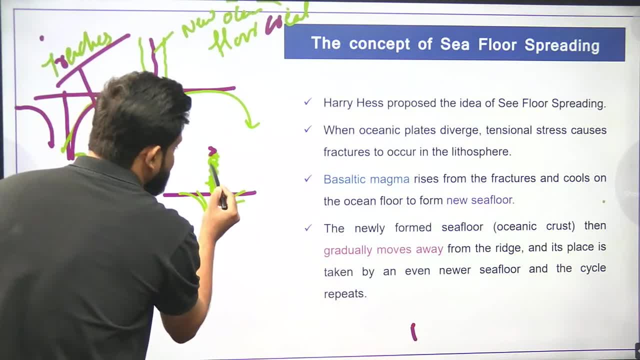 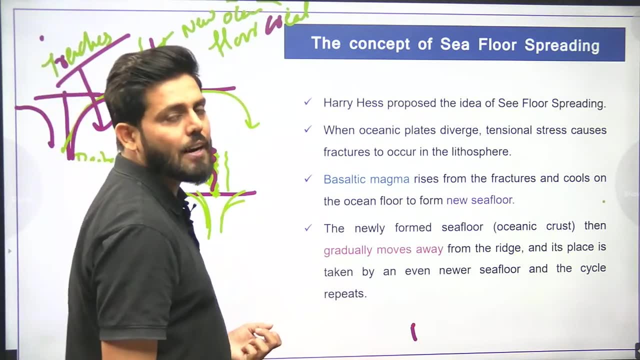 Where the magma is rising, From where the magma came out, A ridge was formed And on both sides of this ridge The magma was solidified. on both sides The rock was of different age Which was solidified. Now the magma which was rising. 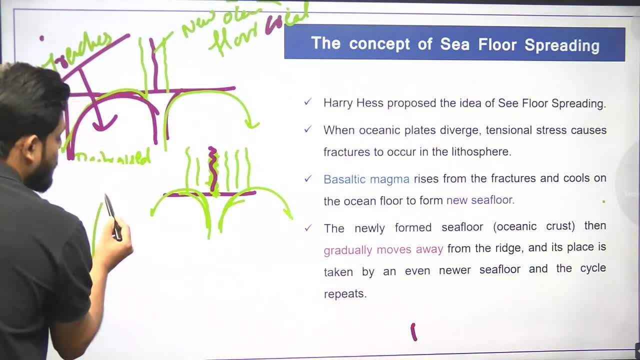 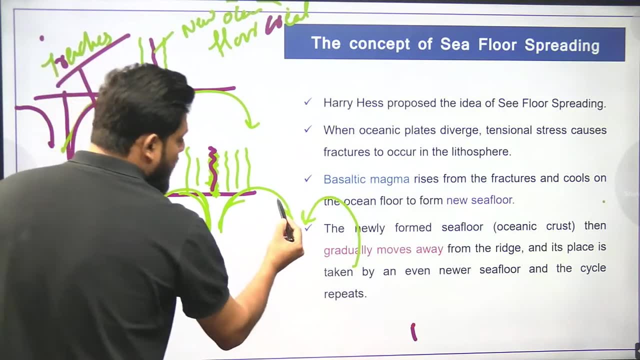 It will fall somewhere. It will fall somewhere. The same from here. The magma is rising And it is falling here. The same from here. The magma is rising And it is falling here, Where the falling limb will be found. Here it is diverging. 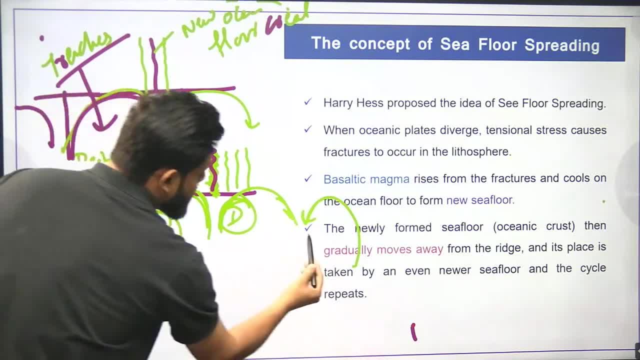 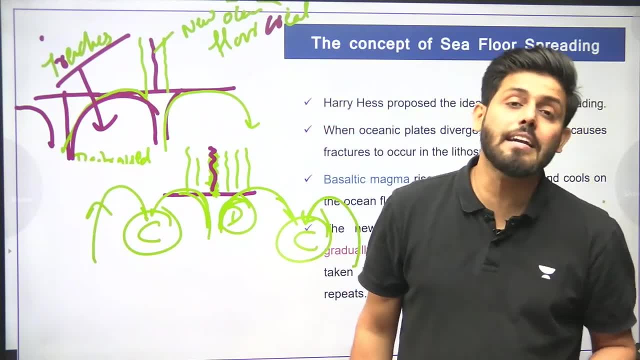 Diverging And here it is converging. So where the converging limb is, Where the converging limb is, There is the destructive plate boundary, And where the destructive plate boundary is, There is the formation of trenches. And where the divergence is. 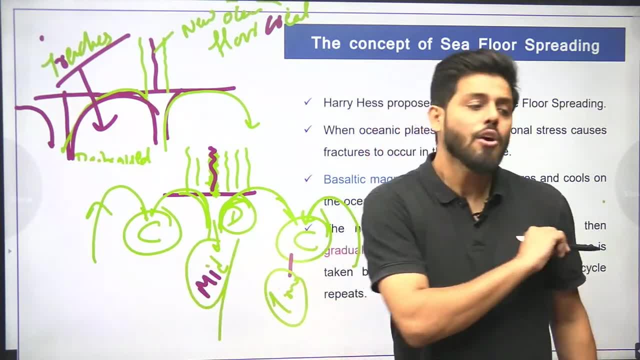 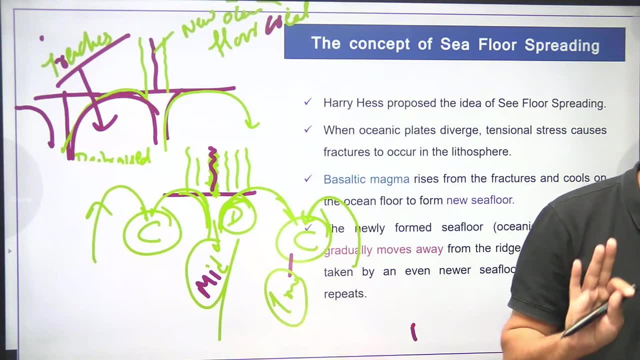 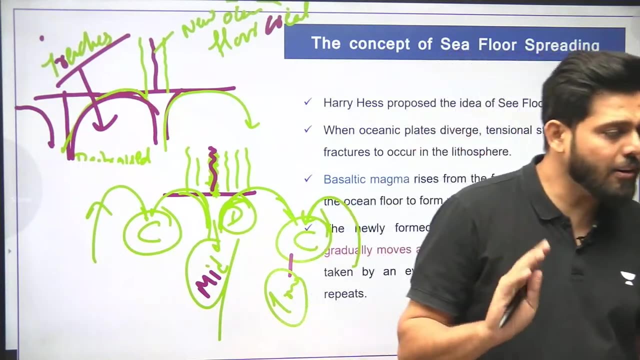 There is the formation of mid oceanic ridges In the ocean. How many students are there Who have any problem in any way? Even now, tell me Anyone of you, Sir, I have this problem. This is the problem Any one of you. 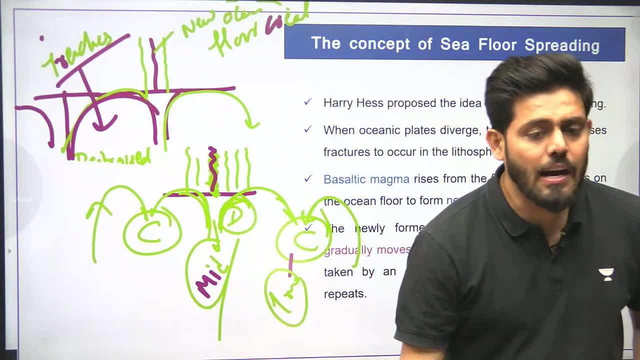 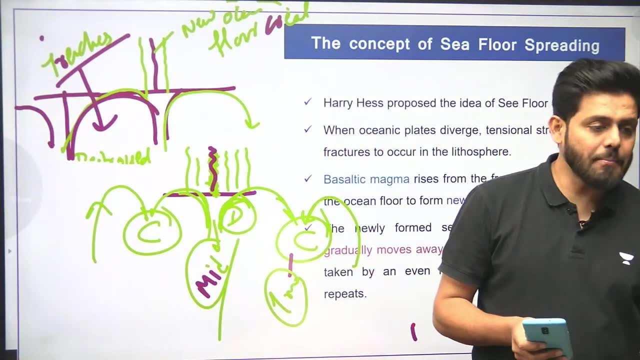 Then I will proceed. Tell me quickly, Because I have to teach Palaeomagnetism after this. After that I have to teach continental drift theory. I have to teach plate tectonic theory. Tell me till here Who have any doubt. 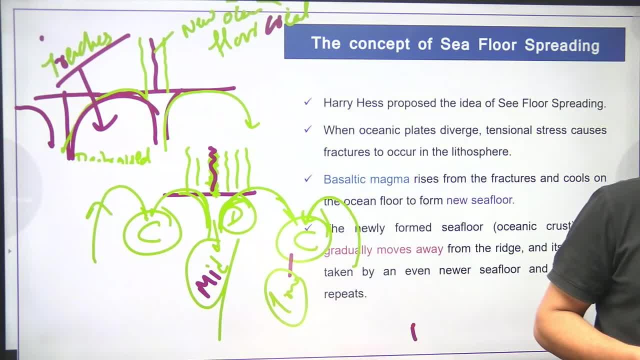 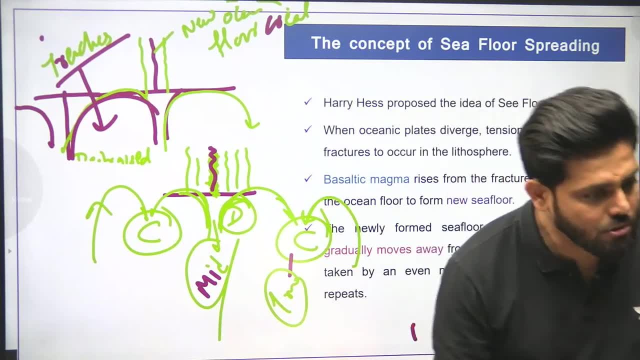 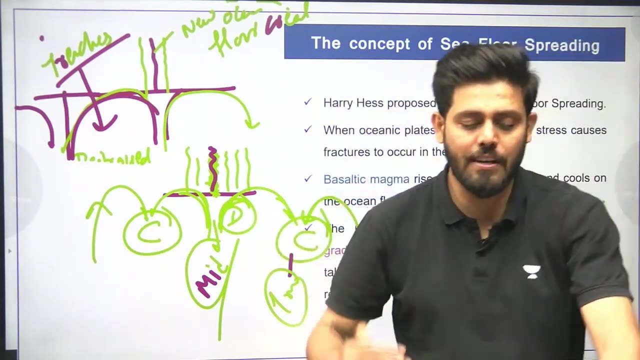 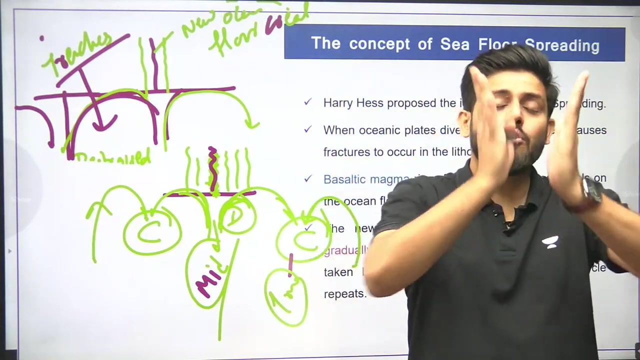 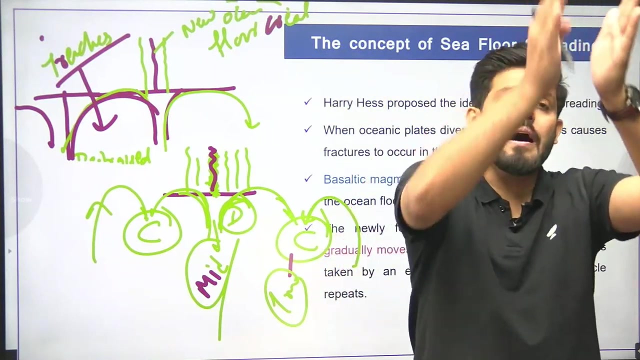 Yes or No? Quickly answer me in comments. Each and everything is clear. Seafloor spreading is clear. Anybody has any doubt. Now we will see the words. What do you want to say? Come fast On convergence. On convergence: where two plates will converge, then one plate will be subducted down, where there will be a deep trench below and where there will be a rising limb, where there will be a divergence plate, two plates will diverge. there will be the creation of a new oceanic floor and there will be mid-oceanic ridges. remember these things. 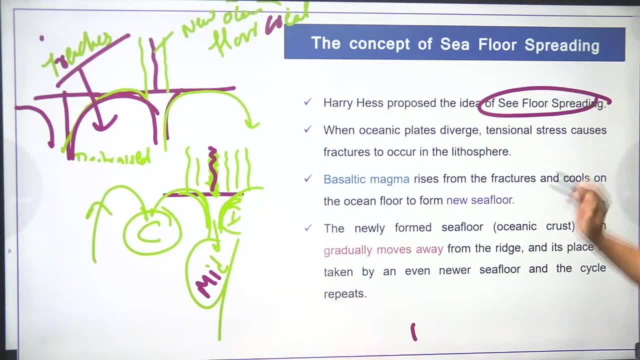 So Henry Hayes proposed the sea floor spreading theory. he said that there is a divergence in the oceanic plate. what will happen if there is a divergence? the magma will try to come out from where the fracture has developed. the break has developed, the crust has been broken. from there the magma will come out and after coming out, it will be cold, it will be cool down, due to which a new oceanic floor will be created. 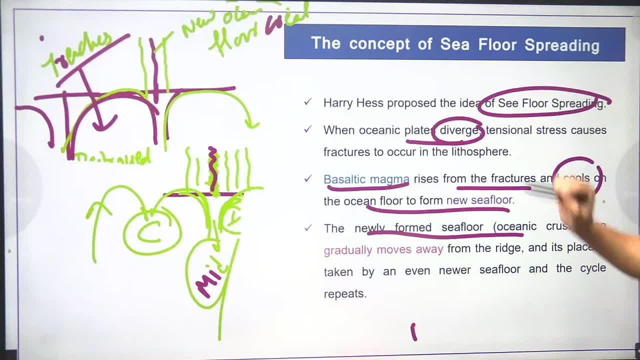 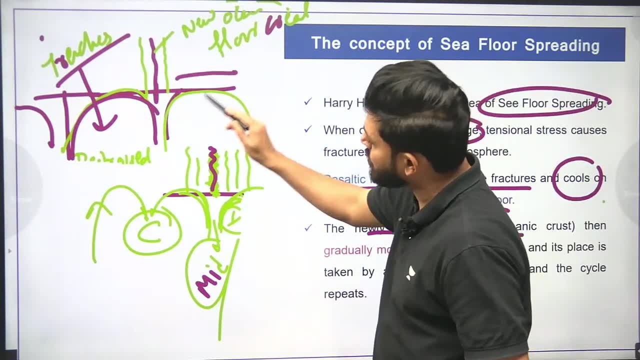 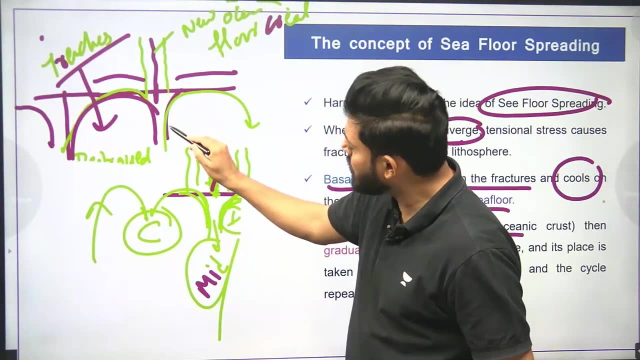 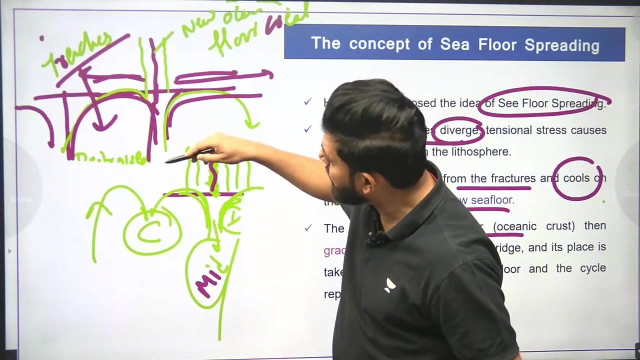 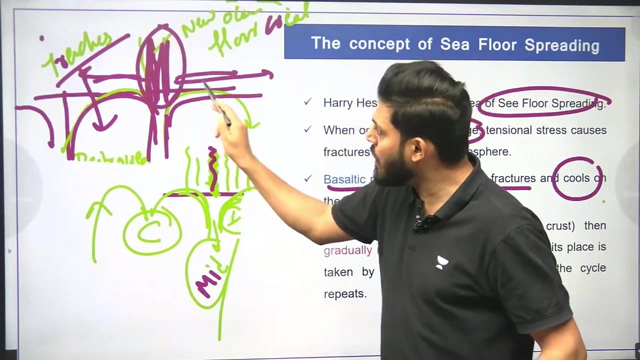 Now, where is the new oceanic floor being found? Where In your mid-oceanic ridges, where there is a divergence? now this oceanic floor will start spreading like this. because it is spreading like this, so the plate will spread here, so this plate will also move with it in this direction. so this oceanic floor will also shift in this direction. the magma that will come out below will keep filling up the middle part. so in the middle part, this new oceanic floor will be created and this oceanic floor will spread. 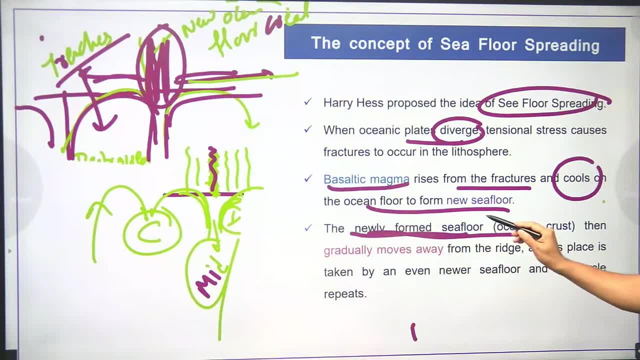 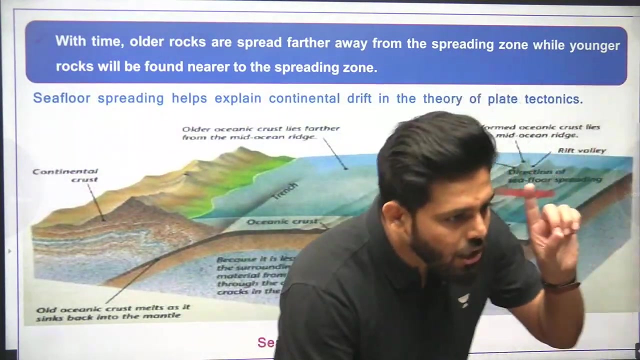 So your new oceanic floor will be formed and gradually your mid oceanic floor will move away from the mid oceanic floor And this will cause your new oceanic floor to be formed again and again, and this cycle will keep repeating. If you don't understand, then look at this figure. 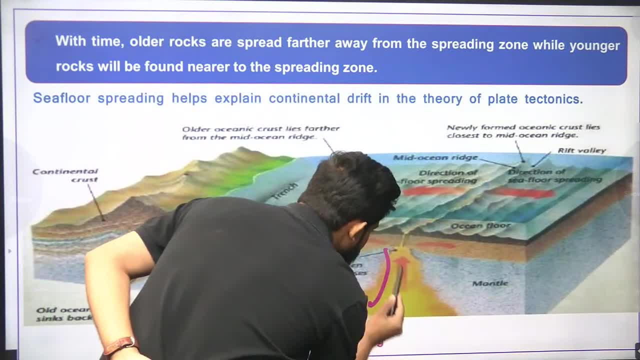 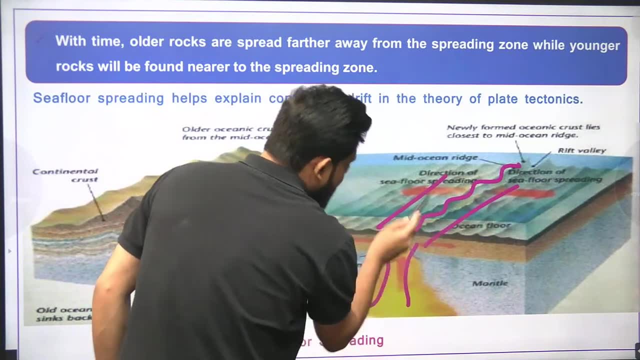 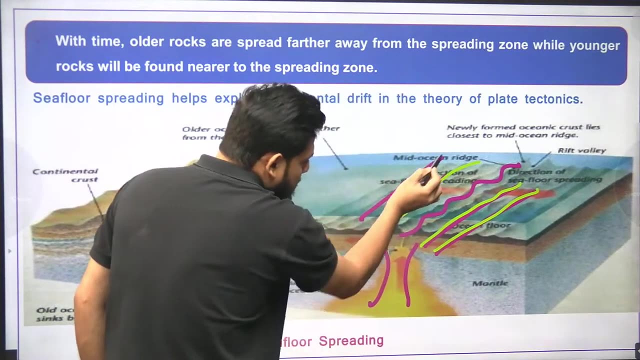 From here magma came out, and from here magma came out, and this is the mid oceanic ridges. Here the new magma deposited the lava in this way. This is the mid oceanic ridges and on its side the magma is being deposited. 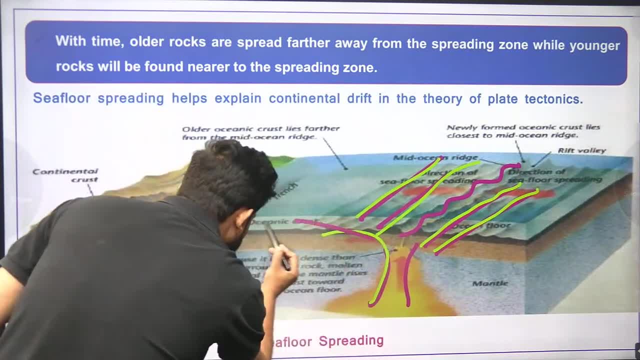 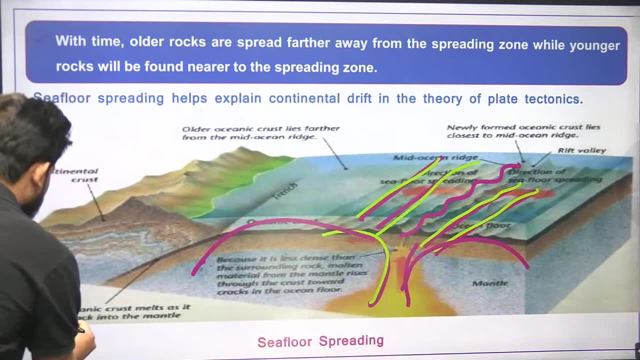 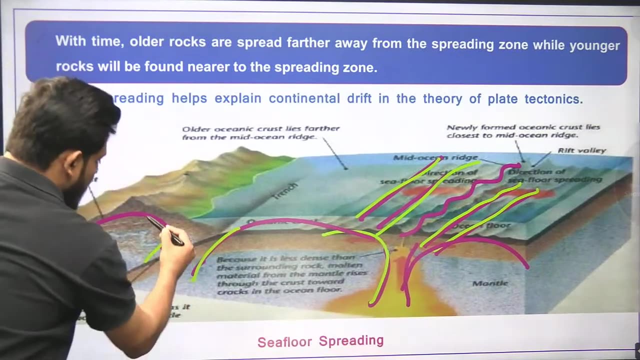 Now the rise of the convection current will diverge downwards, like this: Here it will diverge somewhere. Now there will be some rise from here and it will diverge somewhere, And when both of these diverges and converges here, then there will be the formation of trenches there. 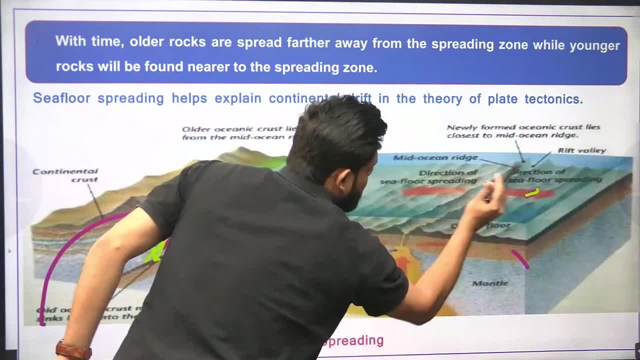 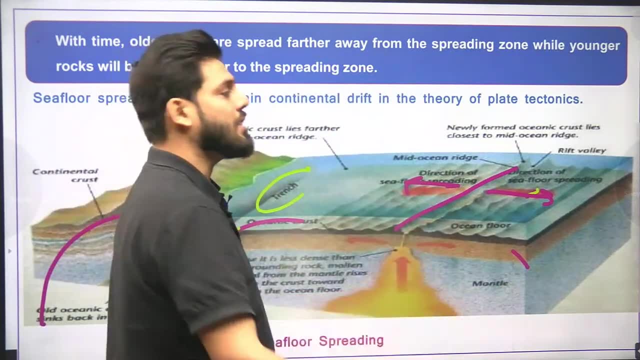 And where the rise will occur, the magma will come out. there will be a mid oceanic ridge and this oceanic floor will keep spreading in this direction. It would have spread a lot, but where there will be two converges, there will be trenches. 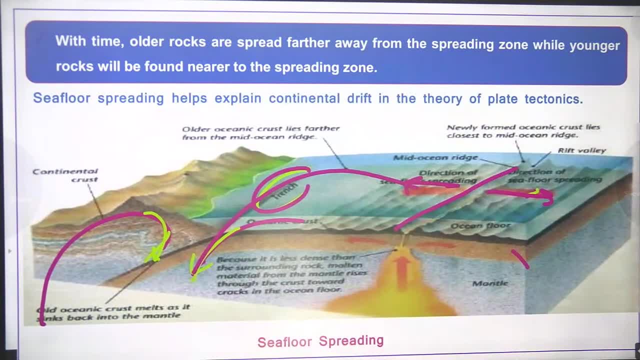 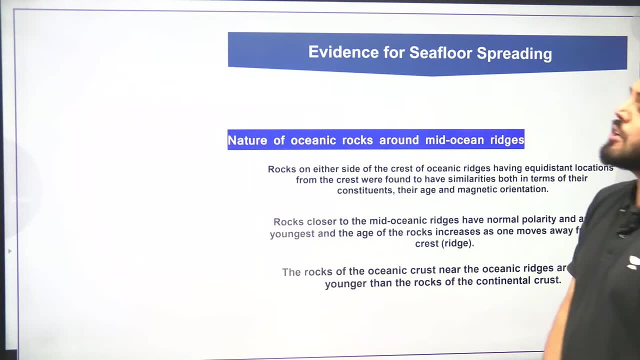 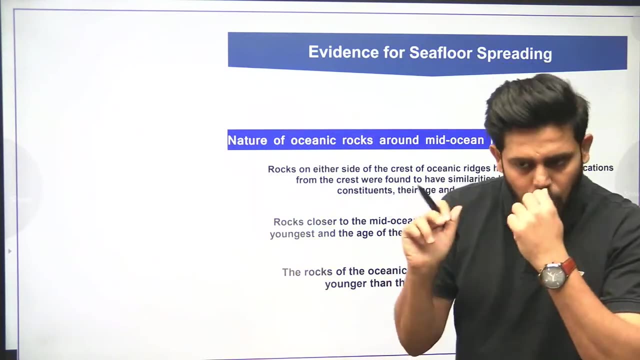 It will look like it is being destroyed. You have to understand this too. Is it clear? Does anyone have any problem? Now let's talk about what evidences we have got that our oceanic floor has spread. Now we must have found out something: that our oceanic floor is spreading. 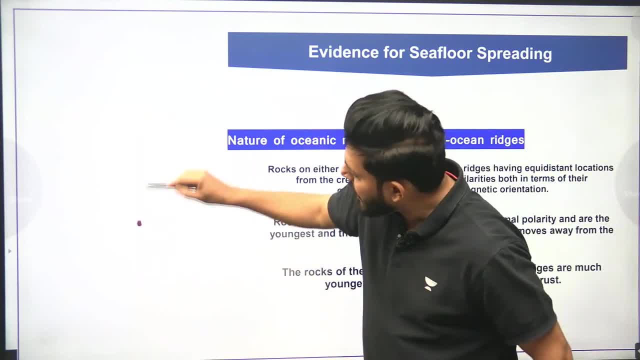 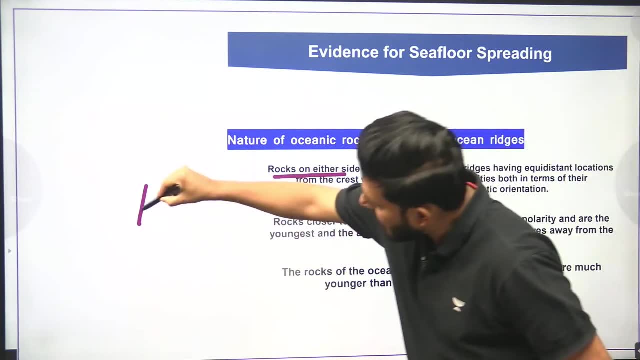 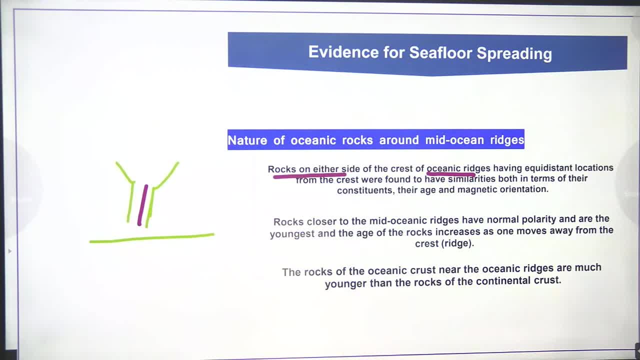 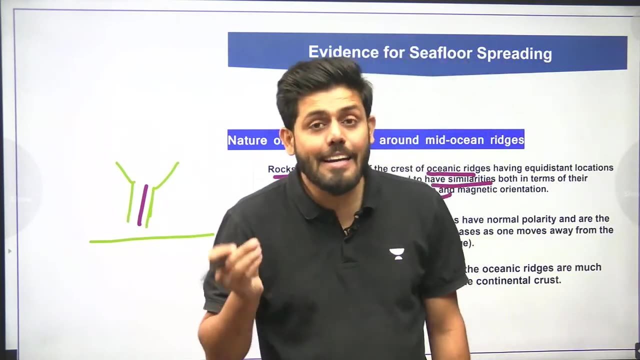 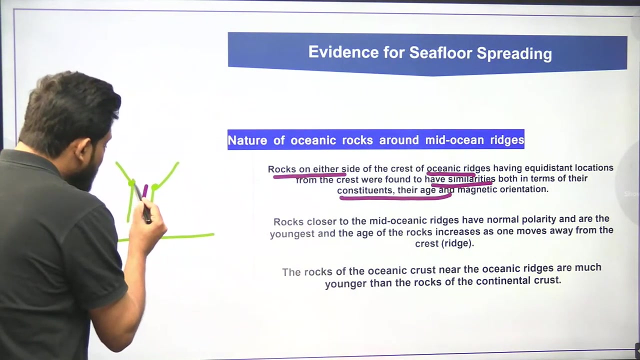 This is the mid oceanic ridges, So the rock on either side of this mid oceanic ridge. there are similarities In what In their age- same age- in their chemical composition and in their magnetic characters. We did not understand that the magnetic orientation when we saw that the magnetic property of this rock and the magnetic property of this rock is the same. 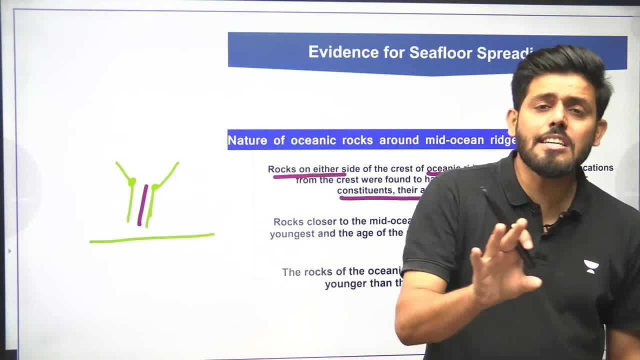 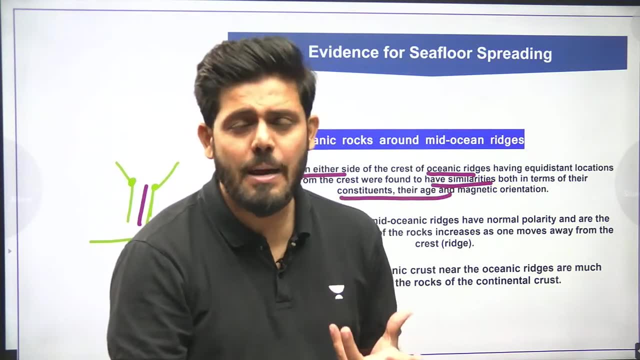 But we did not focus so much on this. But we did not focus so much on this. But we did not focus so much on this Because when we focus on this, we will give it later. We will try to focus more on the concept of our paleomagnetism. 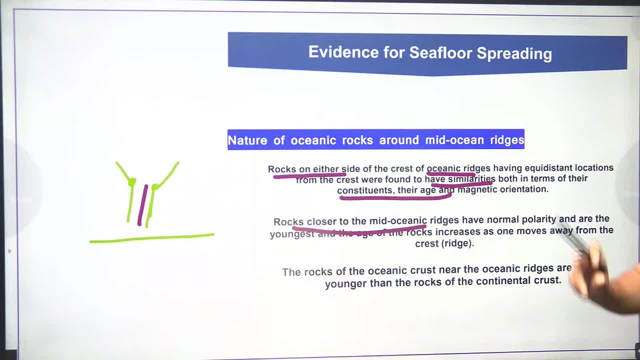 So we saw that the rock closer to the mid oceanic ridges, which is nearby, is your youngest. Their age is the lowest And as the rocks are moving further away, their age is also increasing. The rock near the oceanic crust. 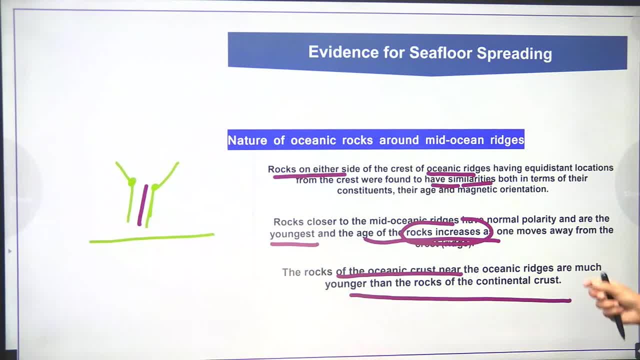 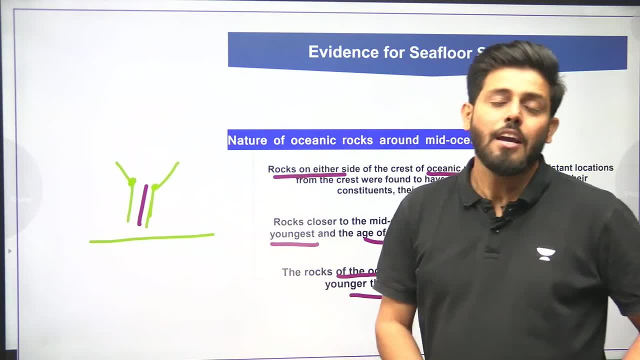 They are younger and they belong to the continental crust, So the rocks of the continental crust are newer than the rocks near the mid oceanic ridges. Because the oceanic crust is spreading, So the formation of the new crust is happening. 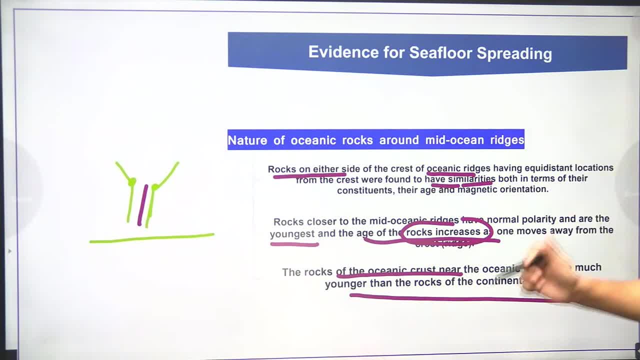 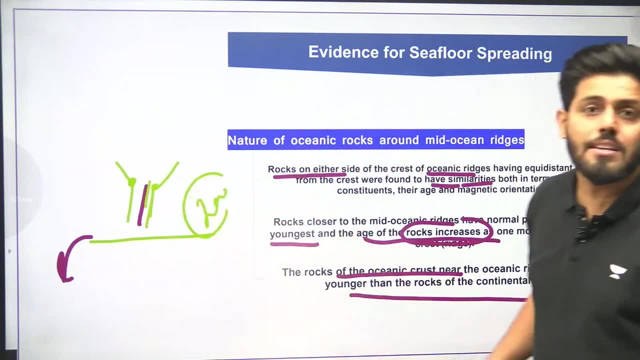 But there are no such things in the continental crust. They are old, But they are not getting older than 200 million Because they are being destroyed on the trenches And they are being formed new on the oceanic ridges. Okay, They explained this point very well. 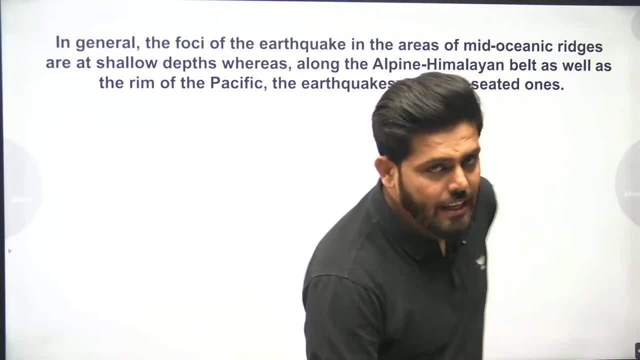 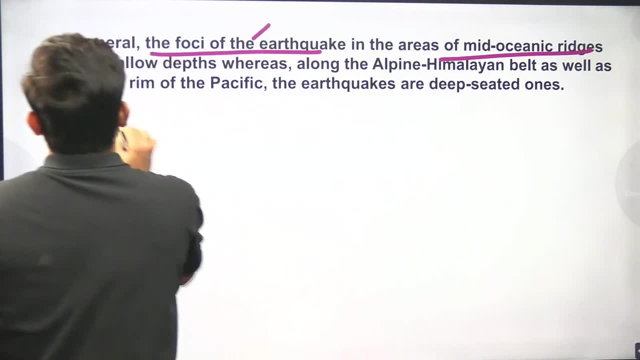 Now we will talk about it. Always remember one point- This can be asked by the UPSC question: The foci, that means the focus of the mid oceanic ridges, will get the shallow depth Meaning. I told you the focus in 2-3 ways. 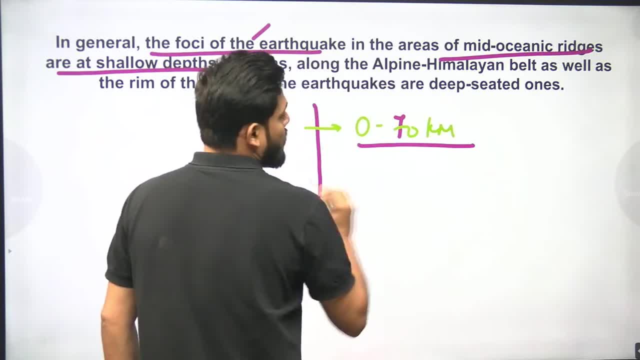 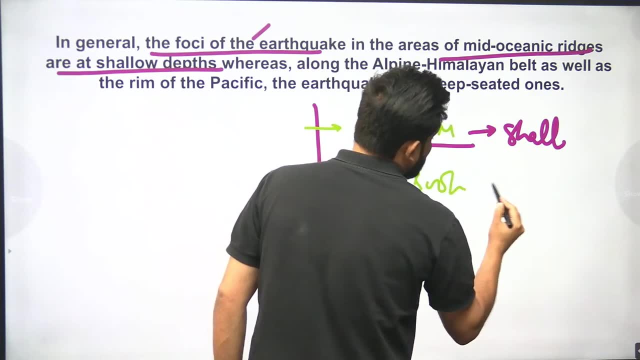 If the focus is on the depth of 0-70 km, then it is called shallow focus earthquake. If the depth is of 70-300 km, then it is called intermediate focus earthquake, And if the depth is between 300-700 km, then it is called deep focus. 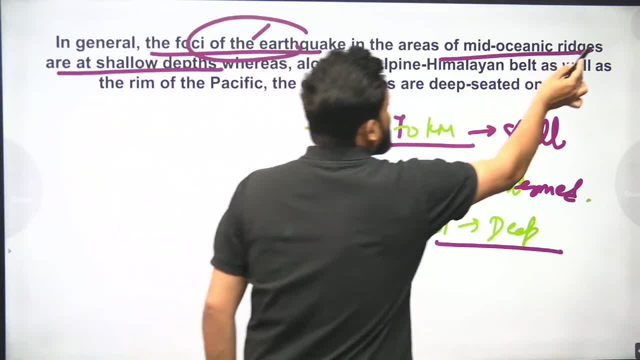 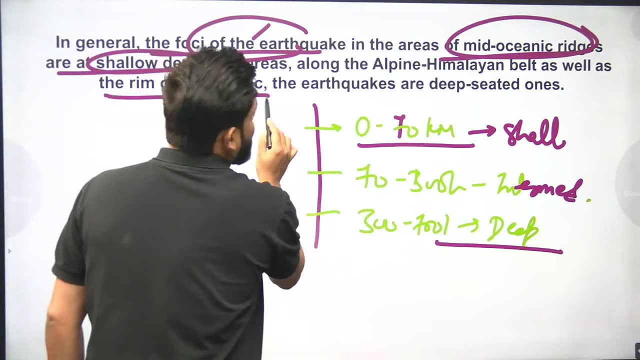 So always remember that your focus on the mid oceanic ridges will always be shallow focus And the Alpine Himalayan belt, the rim of pacific, will be deep seated. It will be a deep focus earthquake. You have to remember these things. 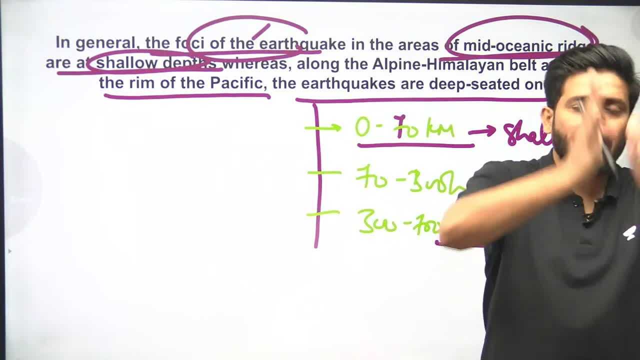 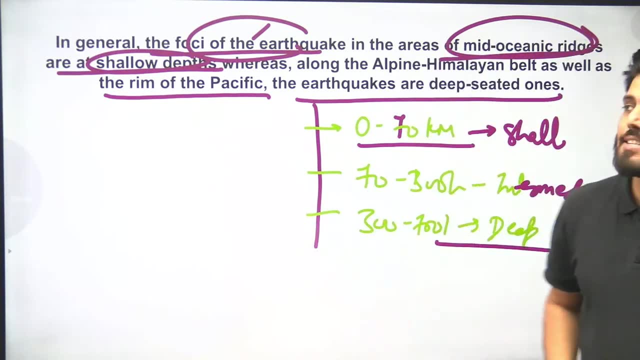 Because what is happening there? The plate is getting converged And where the plate is diverging it is shallow focus, earthquake, And where the divers are diverging, they are diverging on the mid oceanic ridges And where the Alpine Himalayan belt is, two plates are colliding. 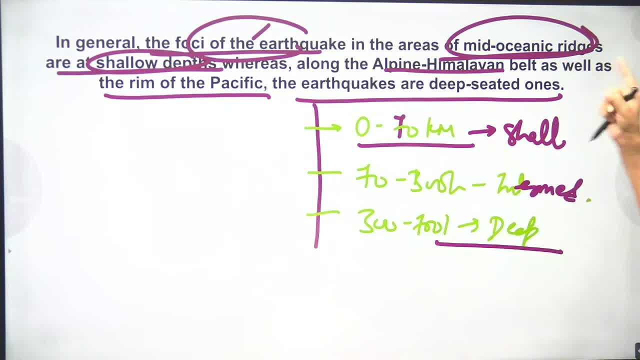 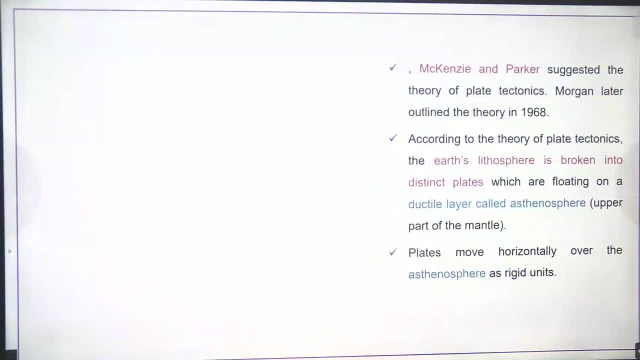 Things are happening due to colliding of Eurasian and Indian plates. So this is your reason. Now we are done with this topic. We study plate tectonic theory very well. Before that plate tectonic, let me teach you once about paleomagnetism. 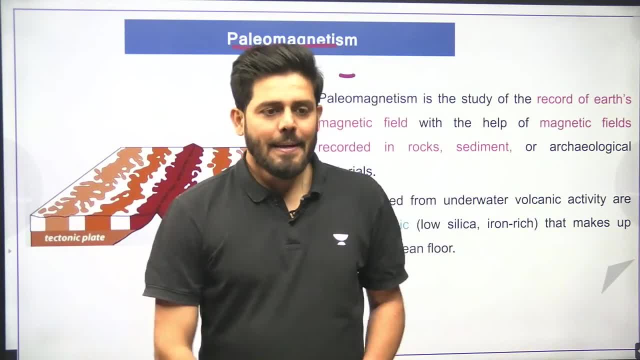 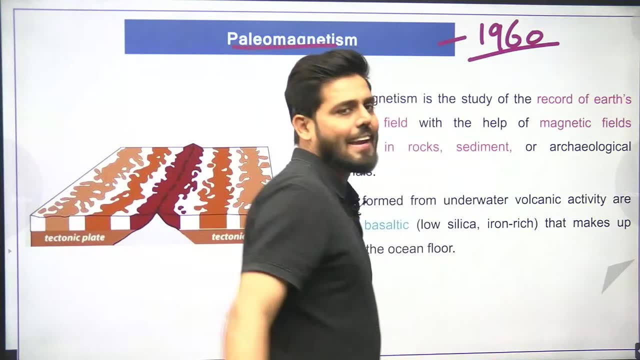 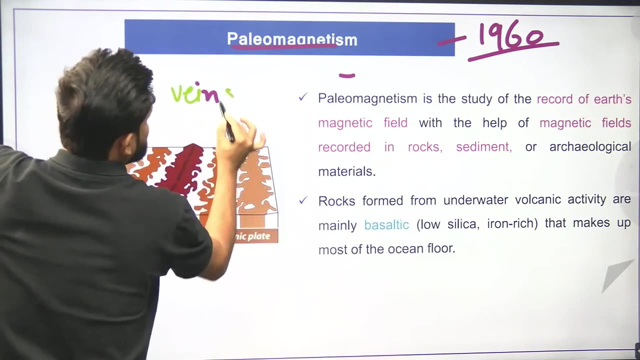 What is paleomagnetism? What is paleomagnetism, Sir? this paleomagnetism, when in 1960, seafloor spreading theory came with the help of Harry Haas, In 1963, another theory came with the help of Wayne and Matthews. 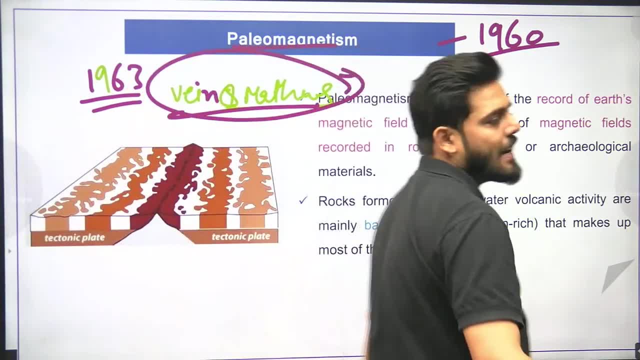 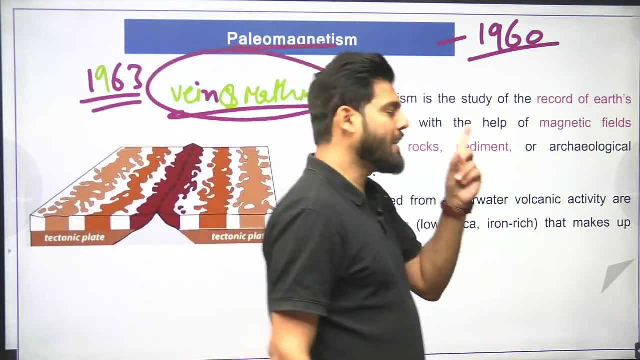 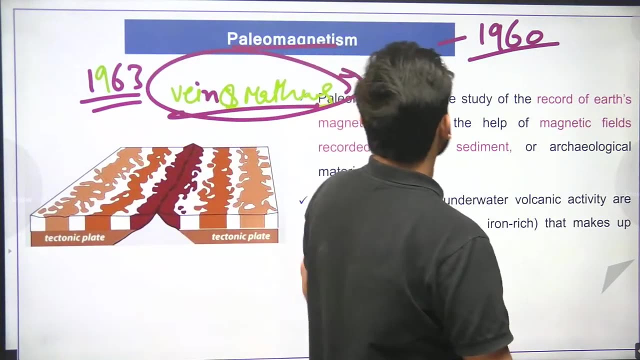 Wayne and Matthews. Wayne and Matthews came up with a theory which is called paleomagnetism. Okay, I have already covered two theories, I have done three. I have done continental drift theory, I have done convection, current theory. Now I have brought paleomagnetism. 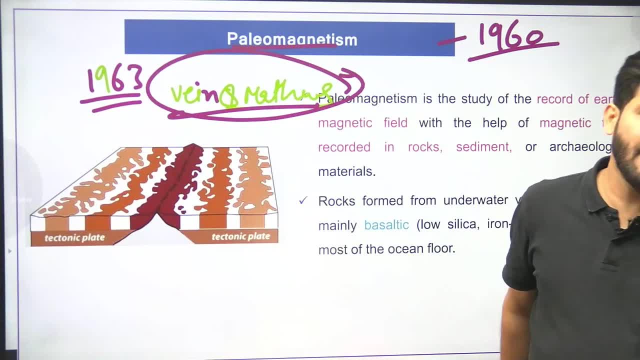 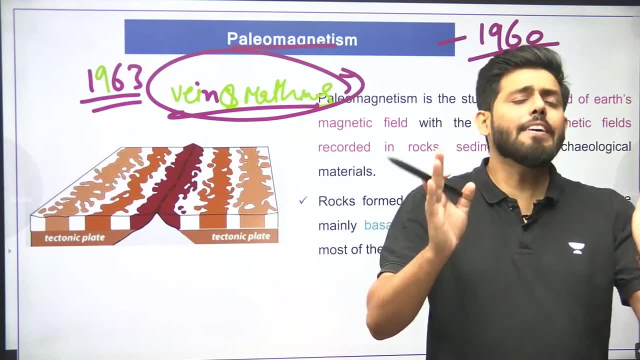 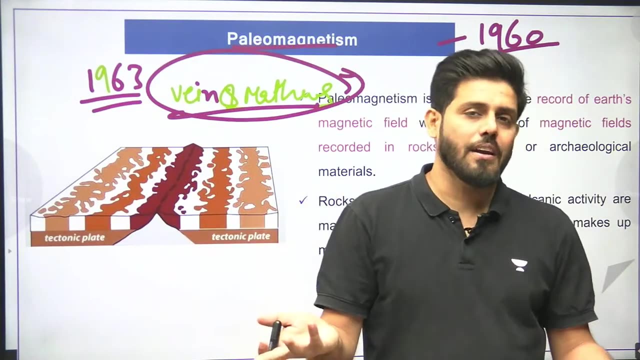 In paleomagnetism there was nothing about our polarity. We understood things there, That our rock, which is at the same equidistance. we saw their magnetic polarity same, But we don't know why it is same. We couldn't understand those things. 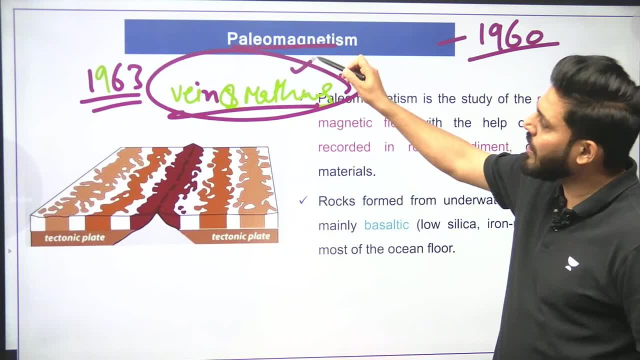 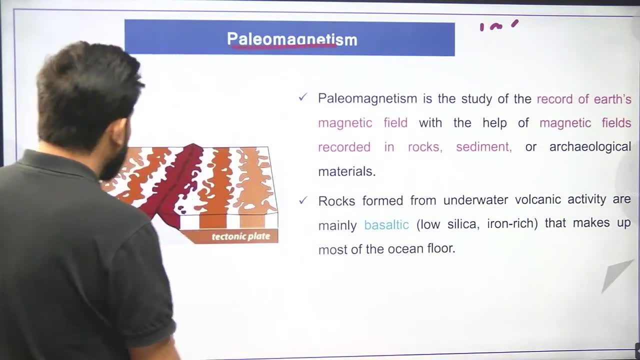 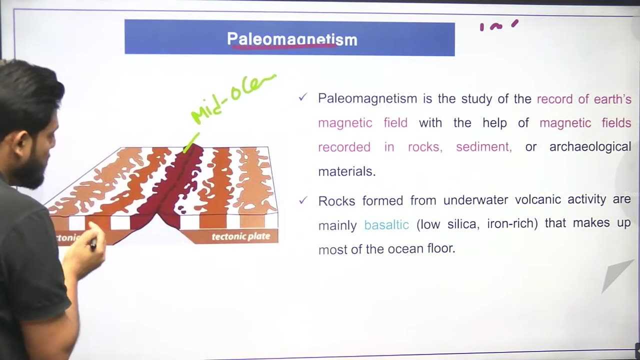 If we talk about paleomagnetism, we have brought Wayne and Matthews in 1963. They basically studied. When they studied, they found out that the one in red color is mid-oceanic ridge- Mid-oceanic ridge- And they saw that this rock of mid-oceanic ridge is the first. 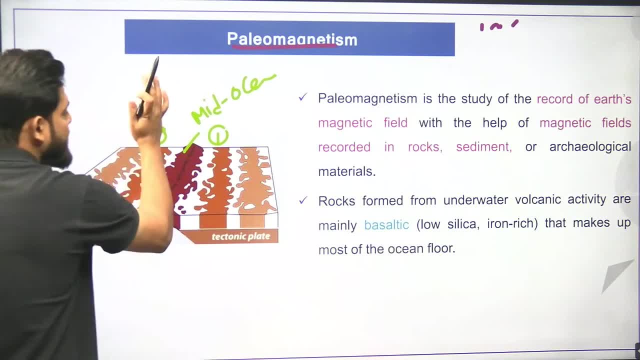 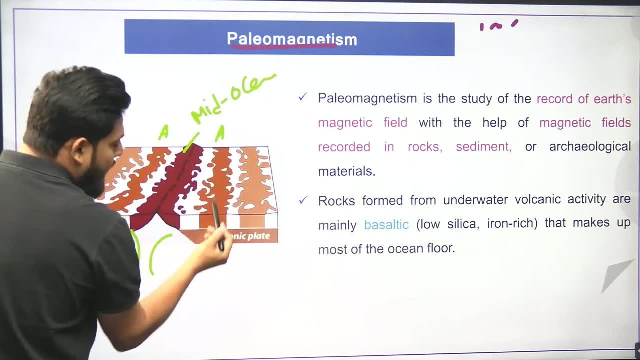 Which is on the other side, Which means it is of same age. If I am writing it as A, that means it is of same age. When these two rocks magma came out from below, it was deposited here, This side and this side. 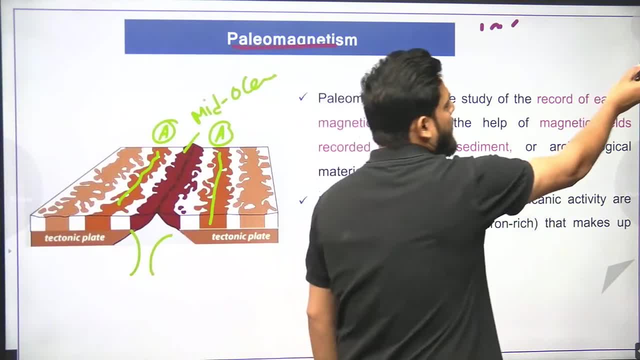 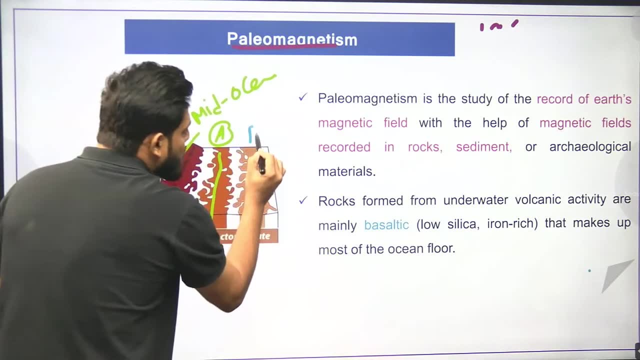 This is A rock. It is of same age. Both came out at the same time. Then we saw later that this rock is of B age, Which means it is of different age. So someone can tell me in the comment box which rock is younger. 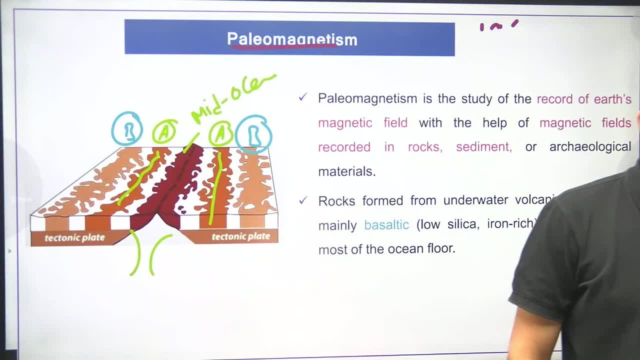 Is B rock younger or is A rock younger? Quickly tell me: Is A rock younger or is B rock younger? A rock is younger. Why? Because the magma has come out from below. It is cold, As we told, as we move away from mid-oceanic ridge. 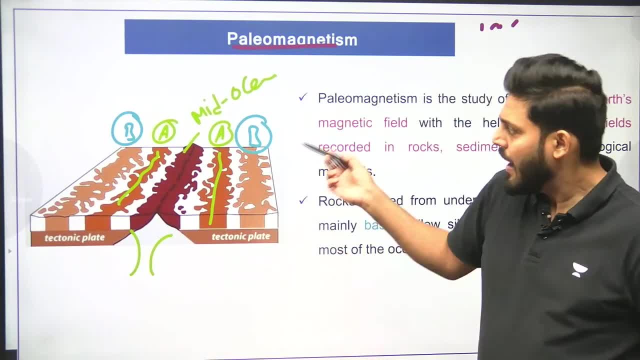 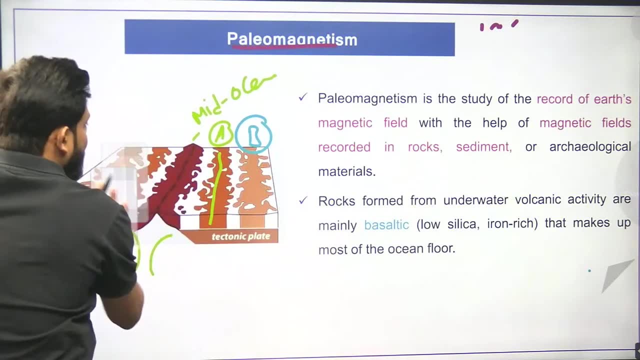 Our age of rock will get older. Now we understood everything with things. But we noticed one more thing: That our A this is mid-oceanic ridge, Mid-oceanic ridge, MOR, So the rock here is the north pole of this. 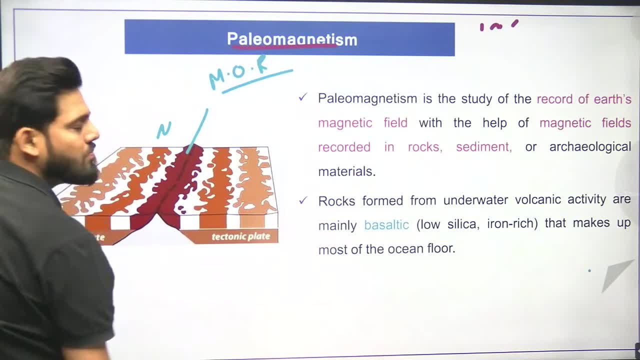 And this is the north pole of this And this is the south pole of this. This is the north pole of this And this is the south pole of this. But when we studied the rock further away from it, We found out that the pole here is the south pole. 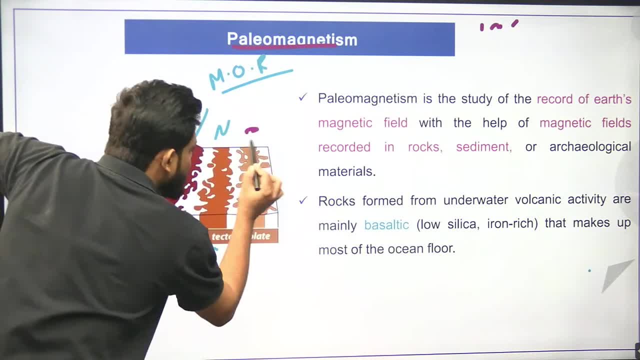 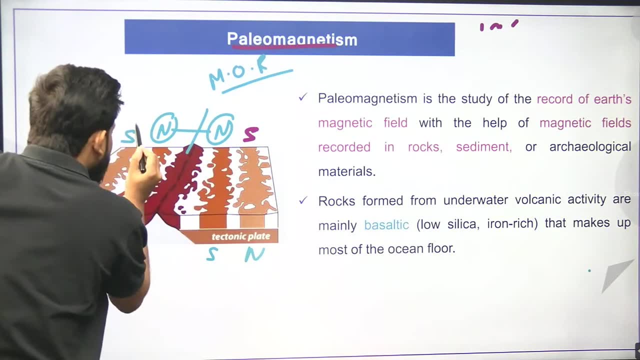 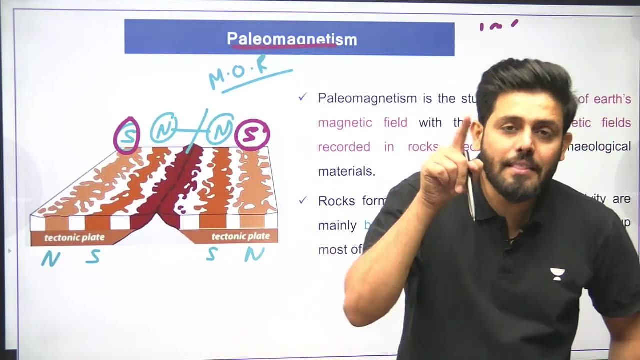 And the pole here is the north pole, The pole here is the south pole And the pole here is the north pole. That means the polarity of this rock is different And the polarity of this rock is different, that their polarity is different, and that is when we came to know that our earth 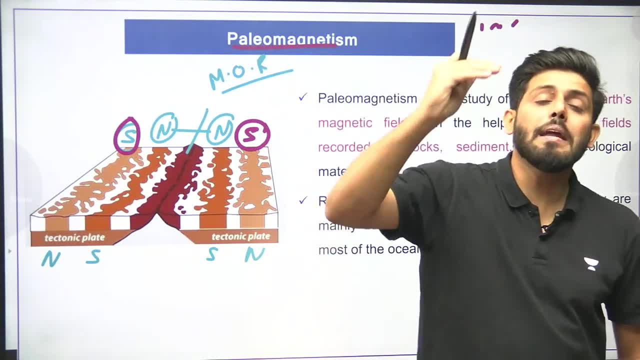 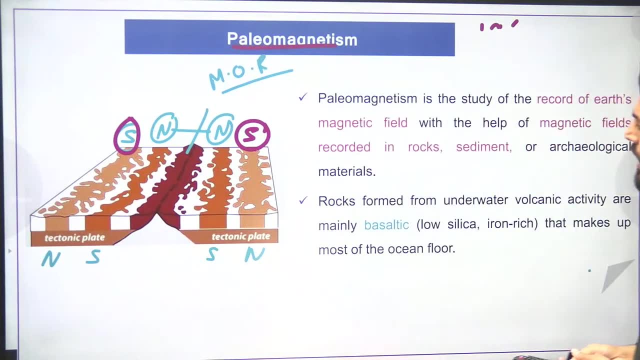 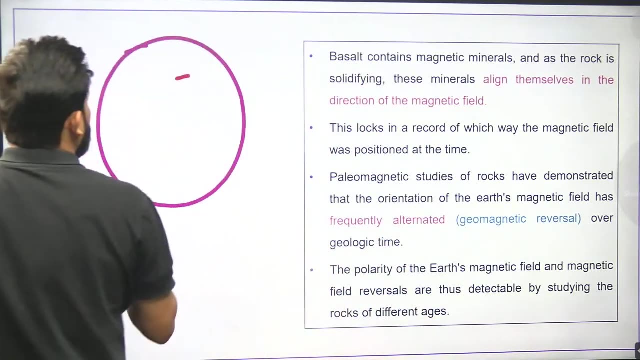 reverses its polarity, it changes its magnetic property. that is when we came to know. now let me explain you one thing very well. you try to understand this point with me, guys. our earth, this is our earth. you all know that our earth is tilted at 23.5 degrees. 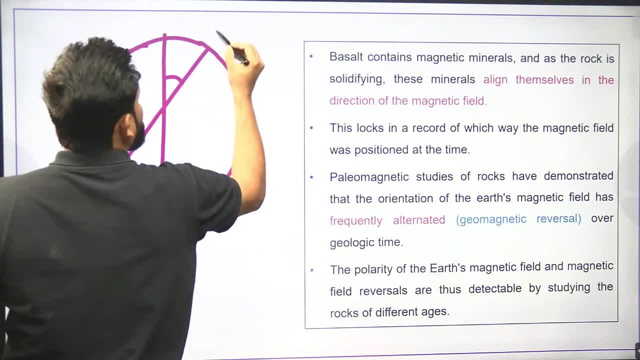 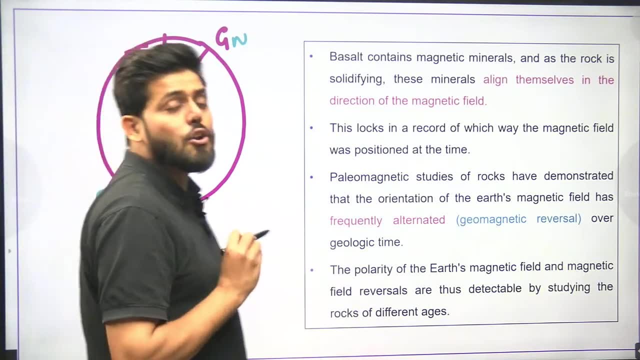 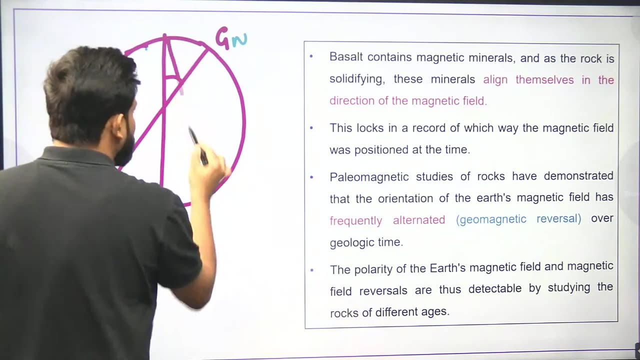 and the pole you see here. this pole is geographical north pole and this pole is geographically south pole. it is geographically north and south pole. similarly, our magnetic pole is also there. similarly, our magnetic pole is also there. if I talk about this pole, this is magnetic north pole. 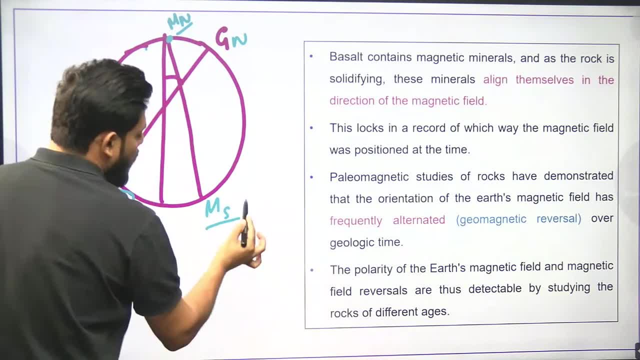 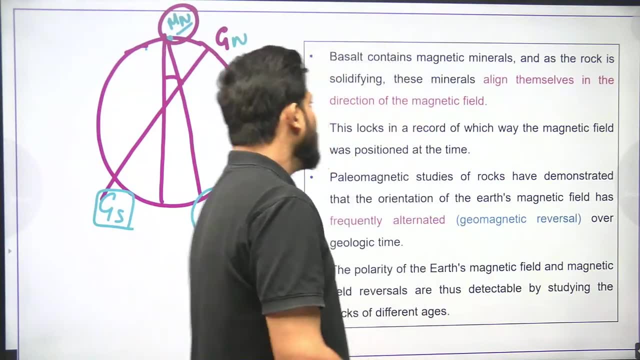 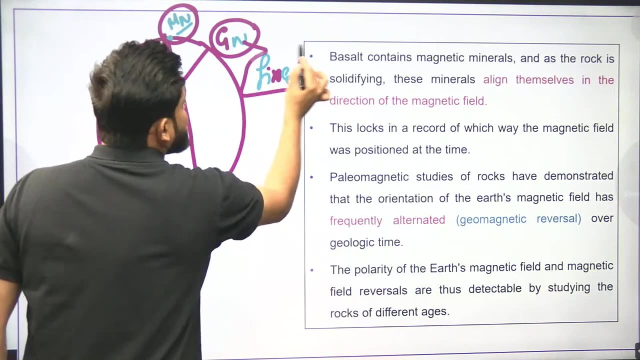 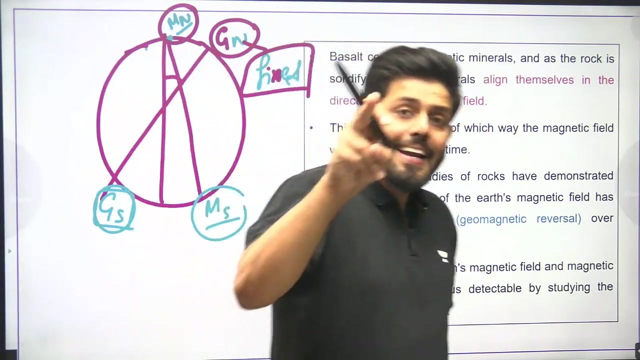 and this pole is magnetic north pole, magnetic south pole. So always remember this: magnetic north and geographically north are different, Geographically north pole and geographically south pole. their position is fixed, They never change. But in the core of our earth nickel and iron are present and due to that, 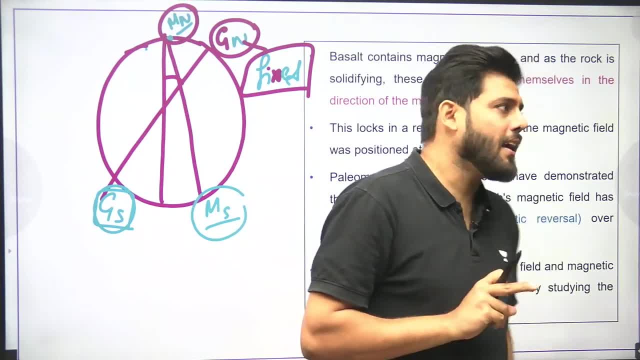 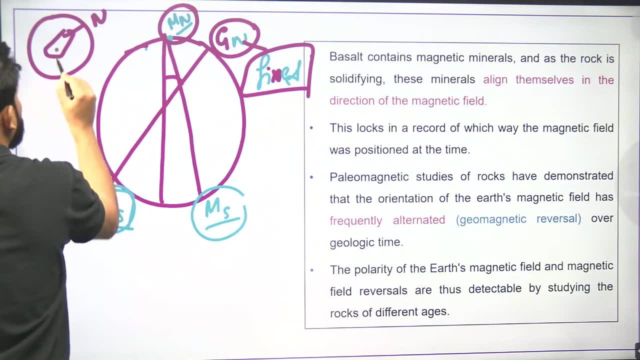 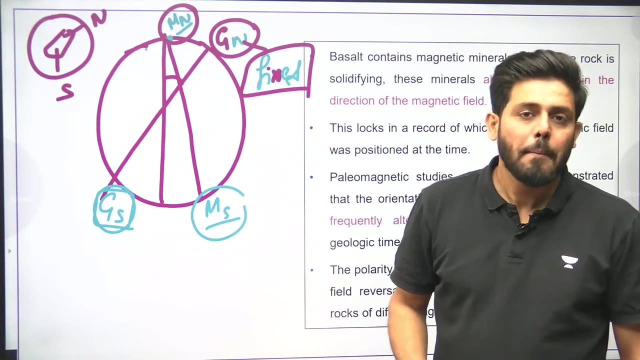 iron. our earth generates magnetic properties And if I talk to you about earth, then in our earth, our earth is a magnet. This is its north pole and this is its south pole. Earth behaves like a bar magnet. It has north pole and south pole, But remember our earth. 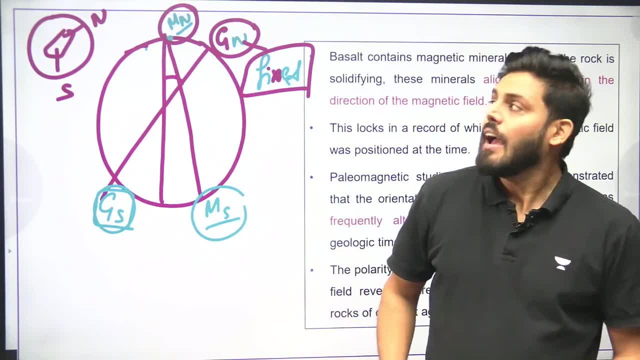 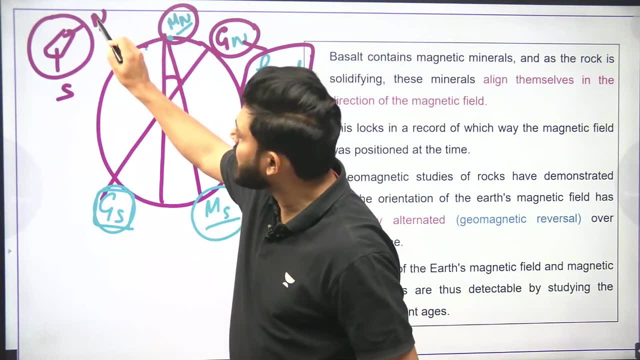 changes its polarity, reverses it. If today it is a north pole, then it takes millions of years and thousands of years for our earth to change its polarity. After some time this north pole will become South pole and this South pole will become 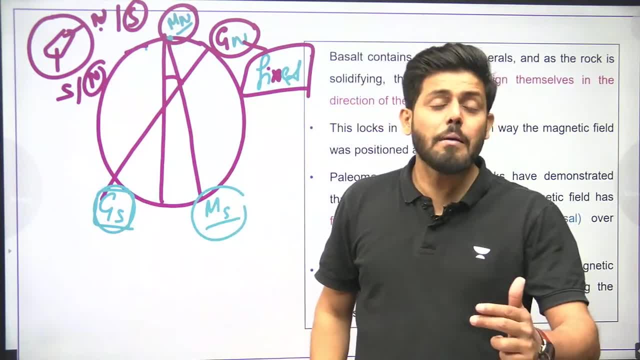 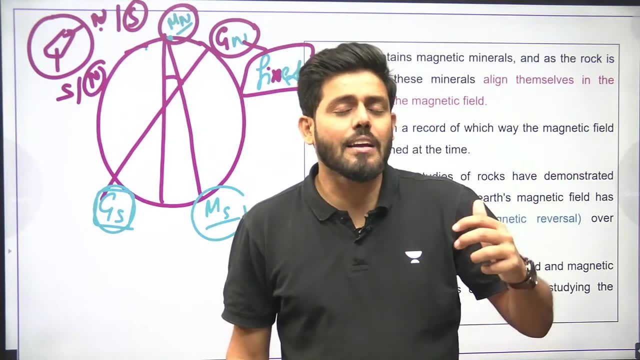 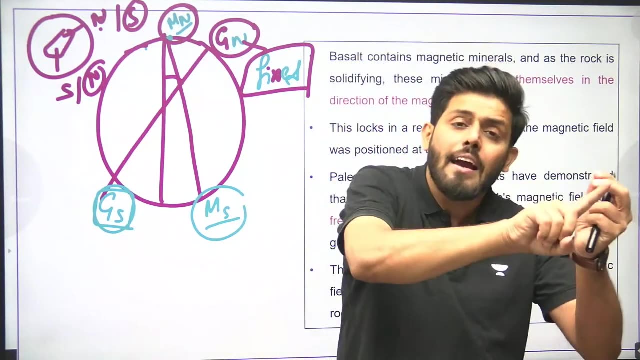 North pole after some time. This means that our earth's polarity changes. If you have read in the news some time ago that our earth'stopics are near the North Pole, which is near Almeria Island in Canada, But it is shift towards Siberia and Russia. So that means 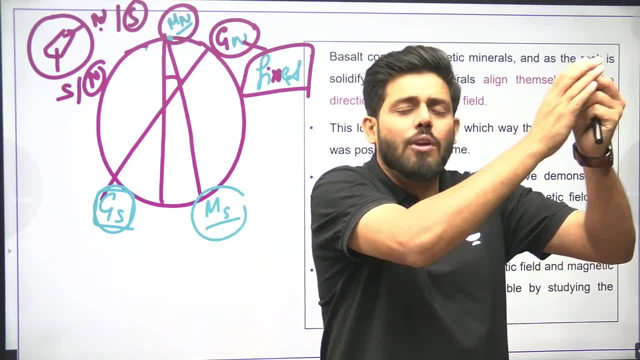 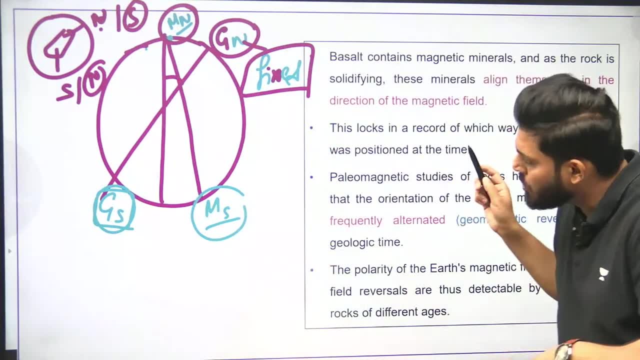 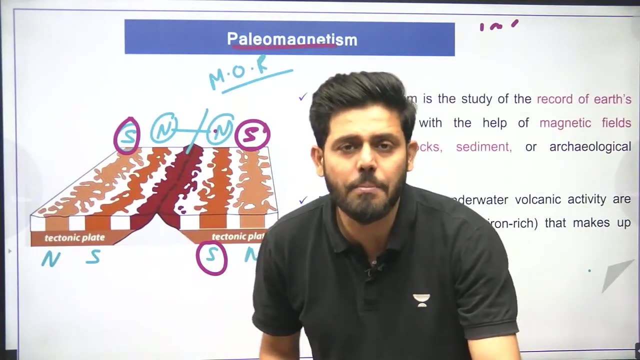 our magnetic north pole is shifting towards Almeria Island. We have a majority of our towards the Siberian point and from this we came to know that this rock here has a North polarity and a South polarity. this means that when magma comes out from the interior of the earth, 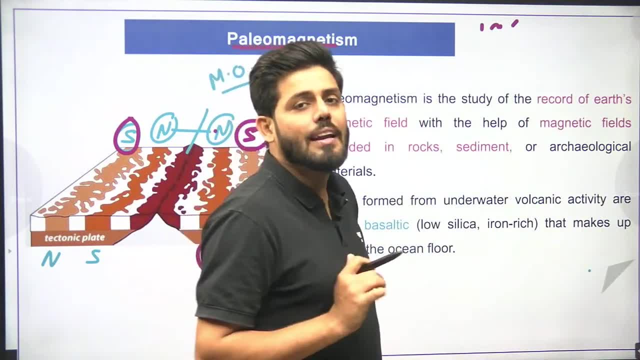 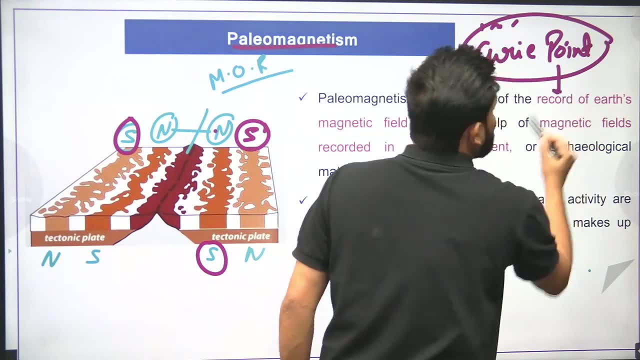 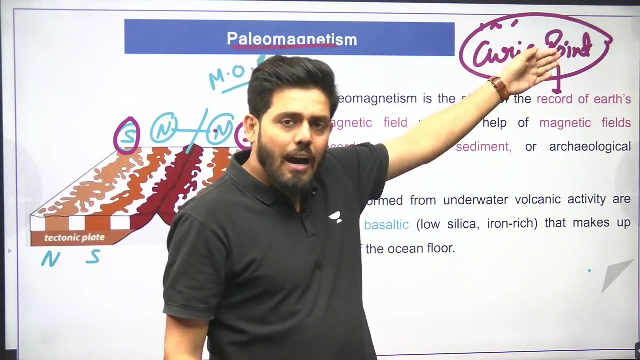 and after the magma comes out, until it cools down. there is a Curie point. write it as Curie point. Curie point is that point, that temperature if our rock cools down, until the rock cools down. if there is a temperature if the rock cools down. 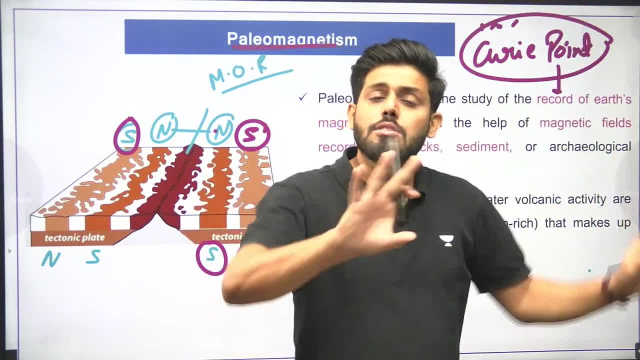 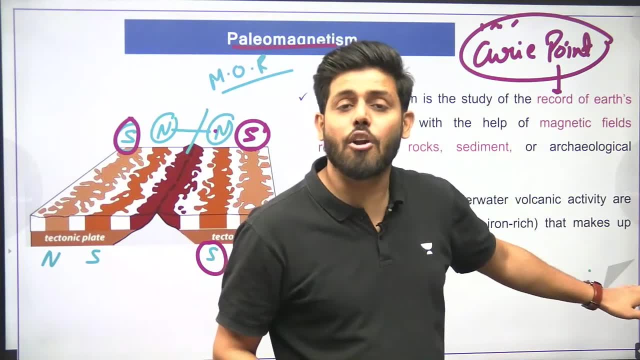 until the rock is more than this temperature from the Curie point, there will be no polarity, there will be no magnetic property, but the temperature of the rock will come below the Curie point. the polarity will come in the rock, which is the polarity of our earth. 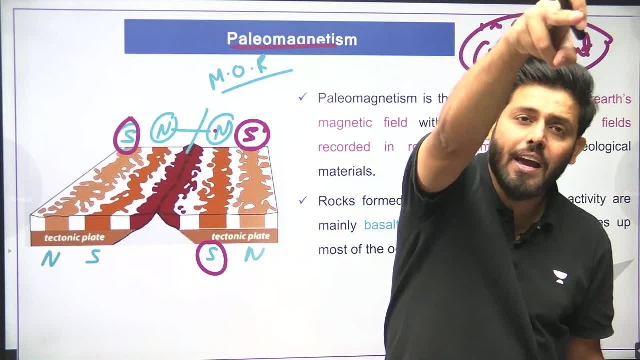 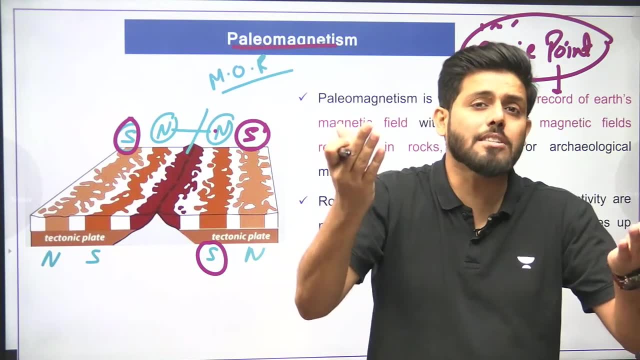 the polarity on which our earth is, if its North pole is that and South pole is this, when the rock comes out from the interior, it is very hot. the temperature is more than the Curie point, so its North pole will remain the same and the South pole will not have any polarity. 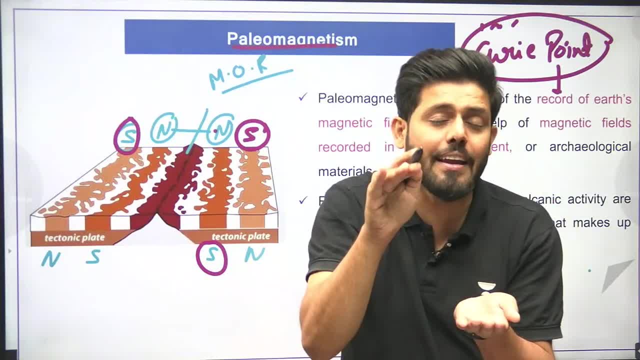 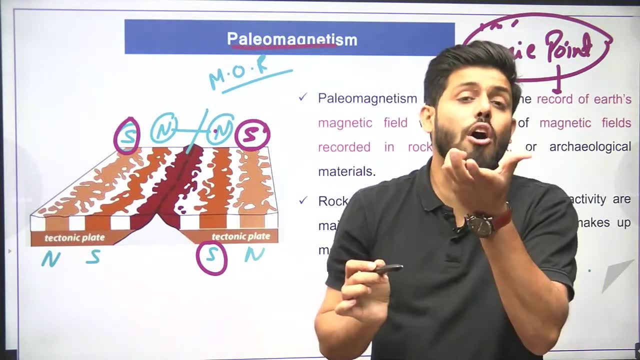 means if the temperature is more, its polarity will not remain anything, as the temperature is cold from the Curie point. so the polarity of the earth is North and this is South. so the rock which will come out from the interior, the lava which will come out, the magma will come out and will be solidified. 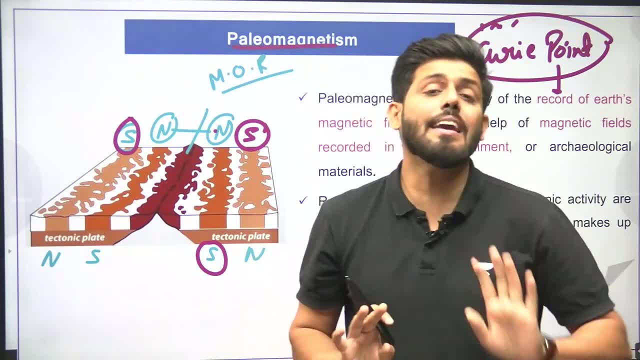 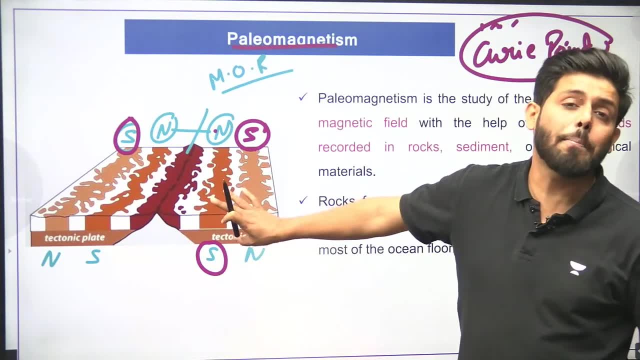 that polarity will be accepted according to the earth. as the earth has polarity, so it will take its own polarity. so this rock came out from the interior. till the time it was hot it did not have any magnetic property, but as it cooled down from the Curie point, 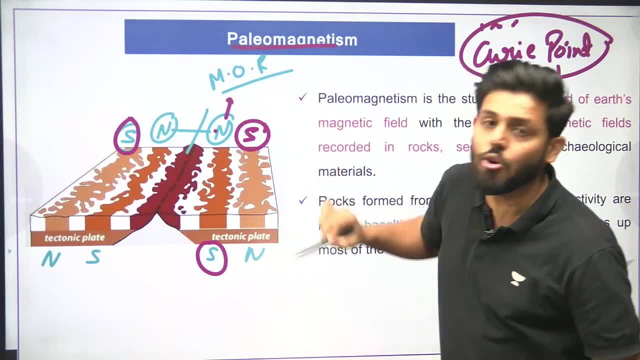 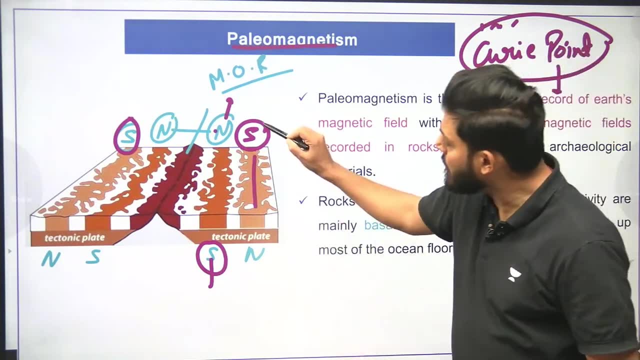 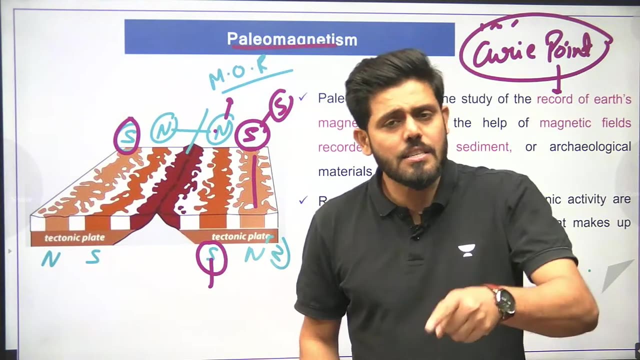 so the polarity of the earth will be the North pole of the earth and the South pole of the earth, but the time when this rock came out, at that time this was the South pole and this was the North pole. that means, according to the property of the earth, magnetic field. 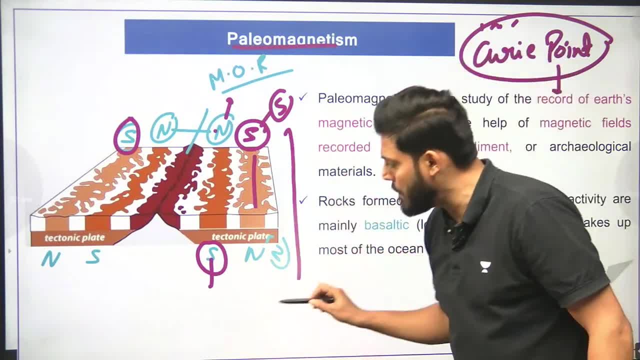 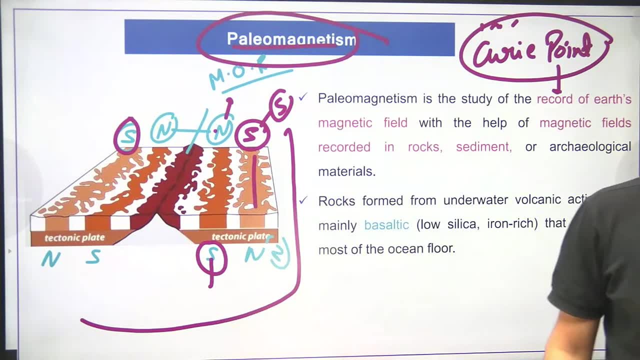 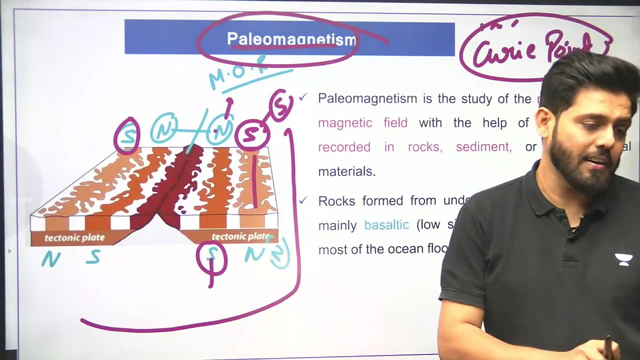 according to the magnetic field of the earth. in the same process, the magnetic field of the earth- and this is the concept of paleomagnetism- as the earth changes, its polarity will also change. you have to remember this point. how many students understood things and how many came out from above? 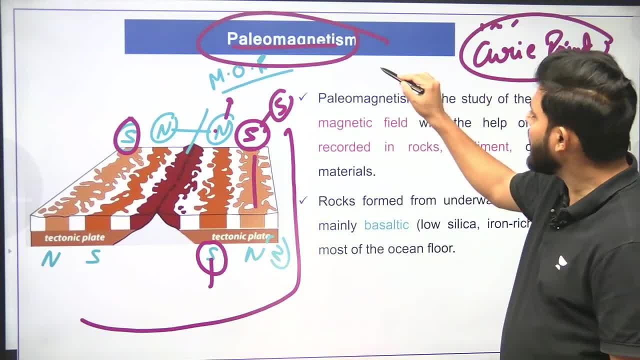 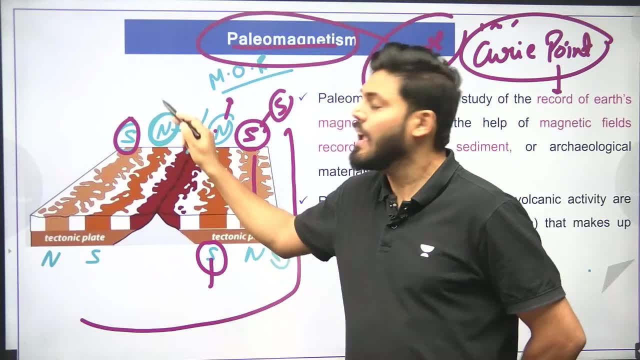 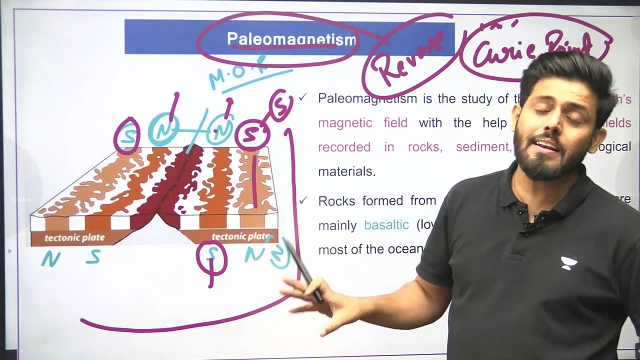 so what happened that we came to know that the polarity of the earth is reversed? and how did we come to know the reverse? when we changed the polarity of these rocks? because at different ages, if I had known that the polarity of the earth is different, but when this rock and this rock 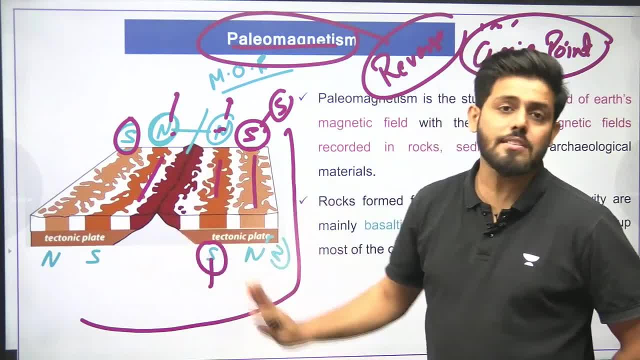 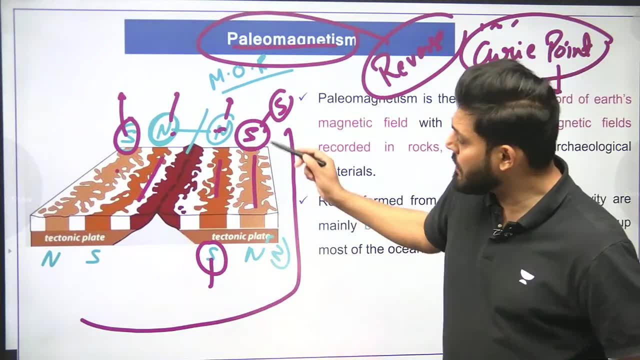 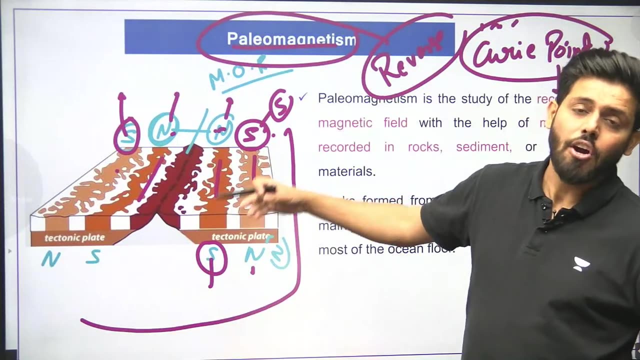 are of the same age means this one and this one. so we came to know that they are of the same age and it has a North and a South. but as the ages differed, the polarity of the earth is reversed. so what happened that when this rock got cold? 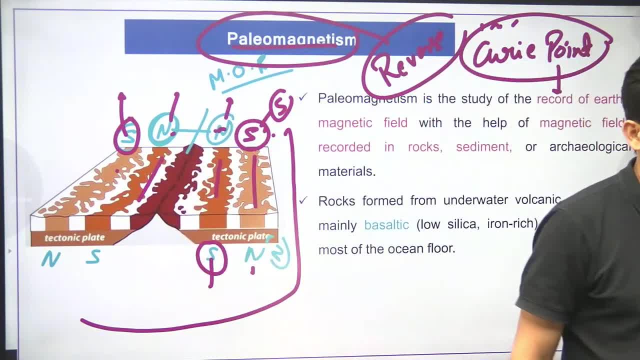 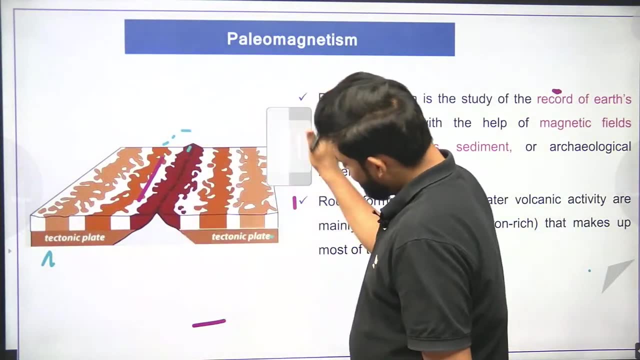 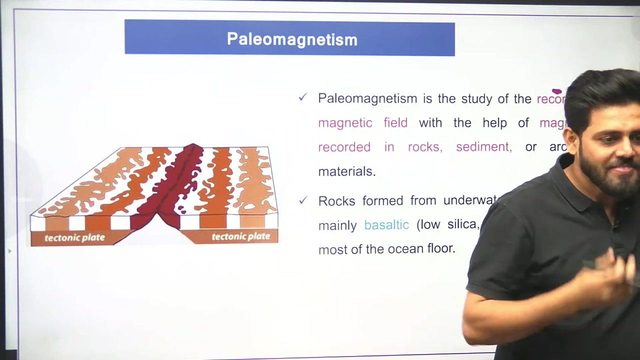 and the polarity that they adopted. the polarity of the earth would be differing in comparison to these rocks. who understood these things? please repeat: it didn't come. it didn't come. let's explain, don't worry. don't worry, I am explaining. I am explaining. I will explain everything. 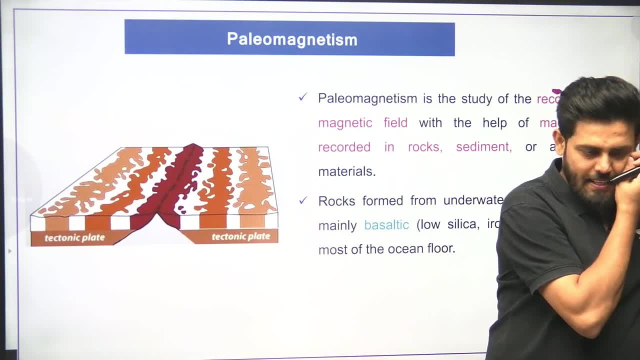 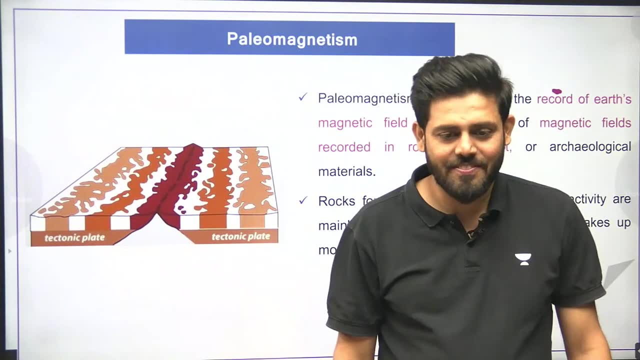 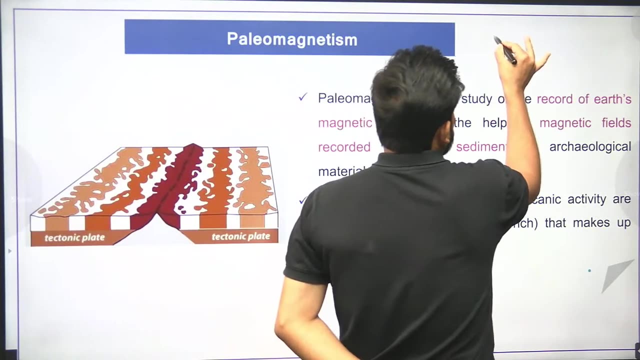 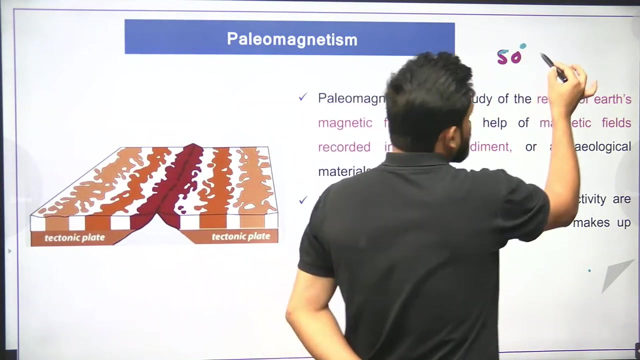 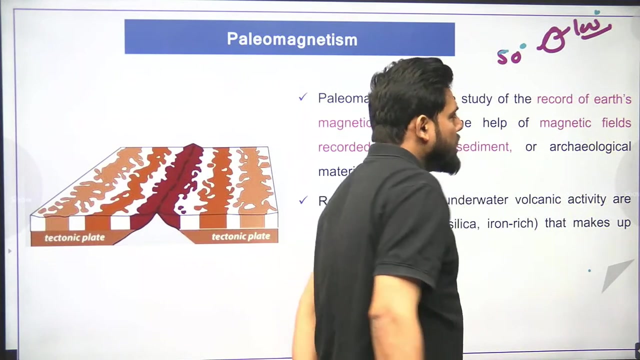 don't worry, come here. come here quickly cool down. don't worry, you will get tired. let's assume there is a temperature 50 degree centigrade. ok, our rock. here is our rock. the temperature of this rock is 100 degree centigrade. so, till the temperature of this rock. 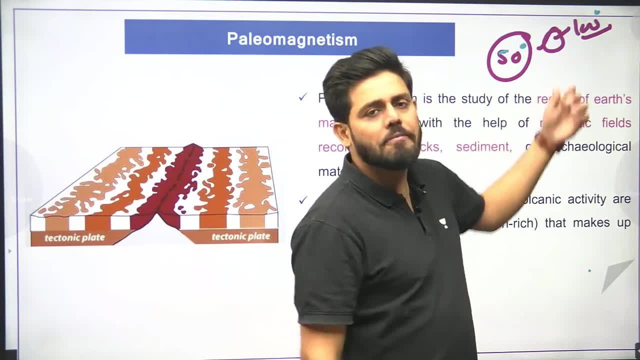 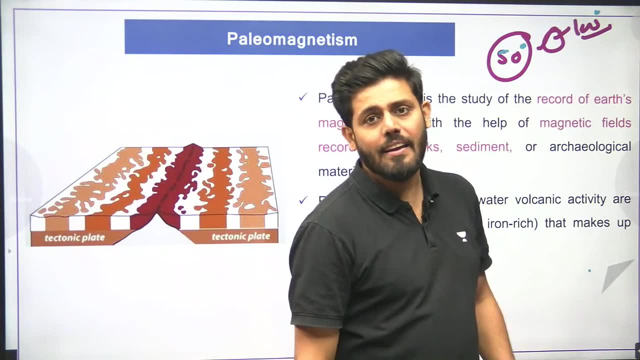 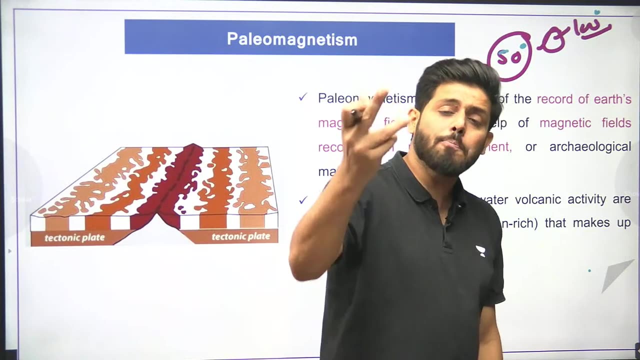 is not 50 degree, till the temperature of this rock is not 50 degree, there will be no polarity, there will be no magnetic characteristic, like if you have a rock. it also has polarity. it also has North Pole and South Pole. according to which, according to earth. 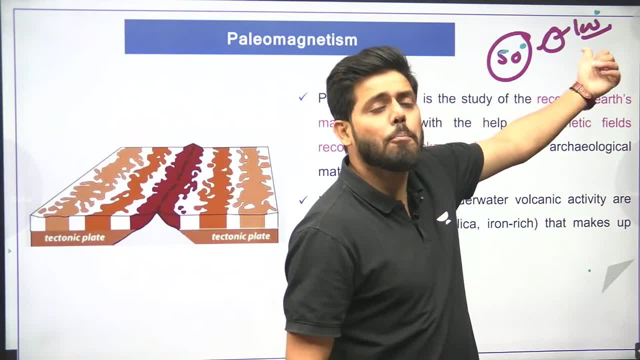 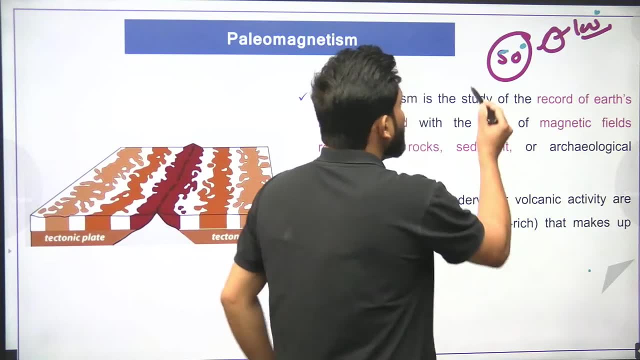 magnetic north and magnetic south of earth in the same direction. their polarity also gets inclined. but till the temperature of this rock is 100 degree centigrade there will be no polarity. curie point is a temperature. let's assume that temperature is 50 degree centigrade. 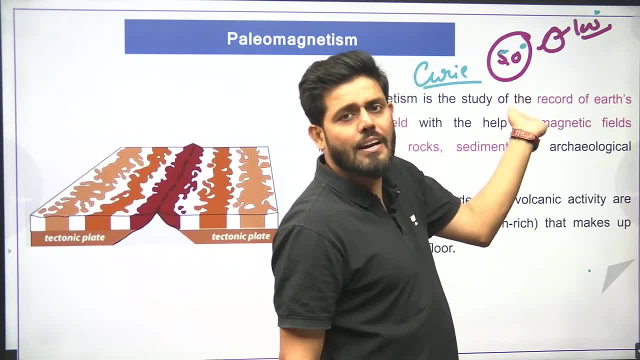 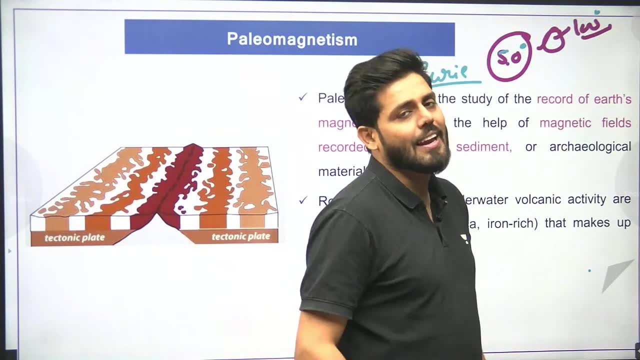 when this temperature will be 50 degree centigrade, the temperature of the rock will be below this curie point. then this rock will accept the polarity and the polarity of earth will be inclined in that direction. it will be inclined in that direction, which is the polarity of earth. 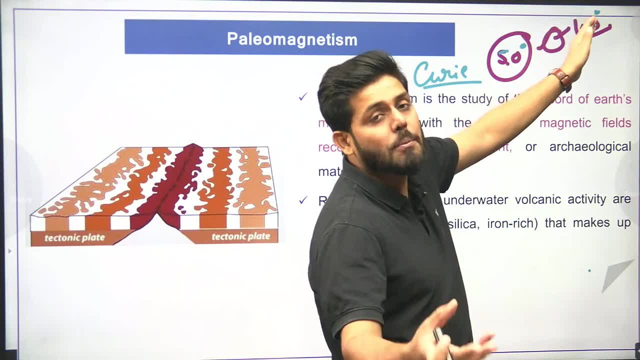 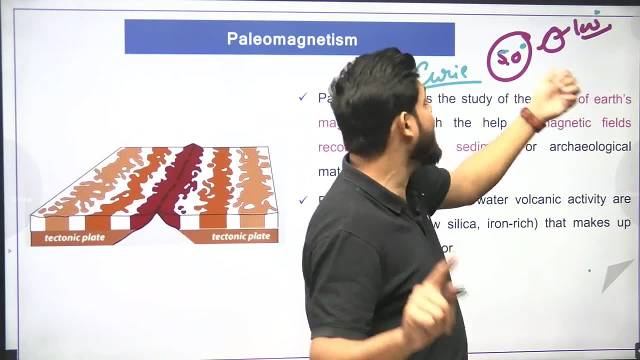 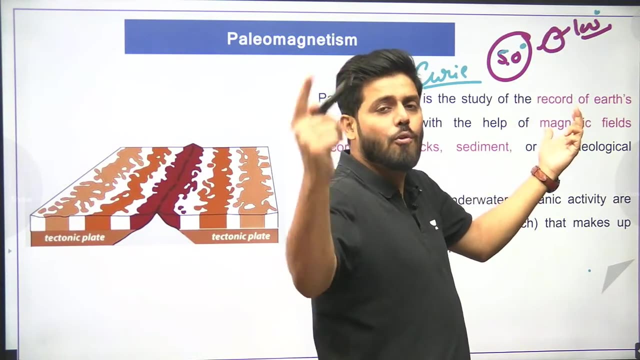 before that, the rock which came out from the interior of earth, but it is hot magma. it came out in the form of lava. the temperature is very high. but till the temperature is high from this curie point, till then there will be no polarity. but as soon as the temperature comes below this curie point, 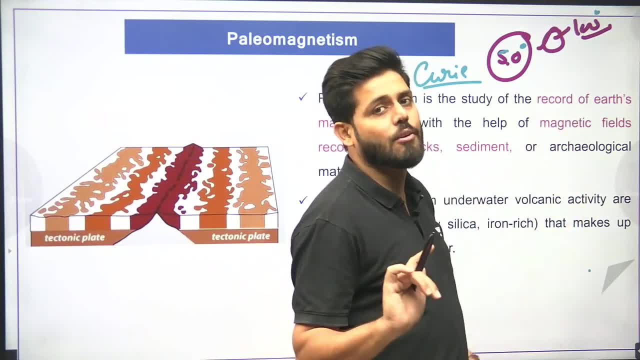 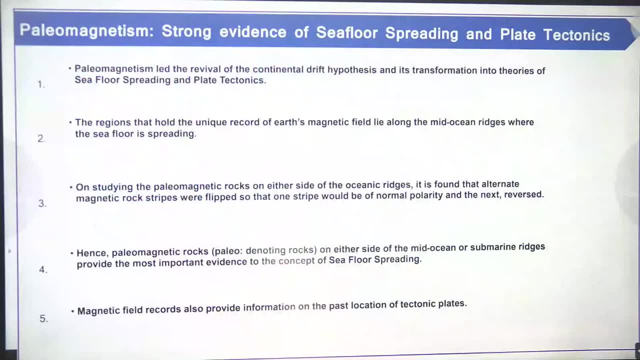 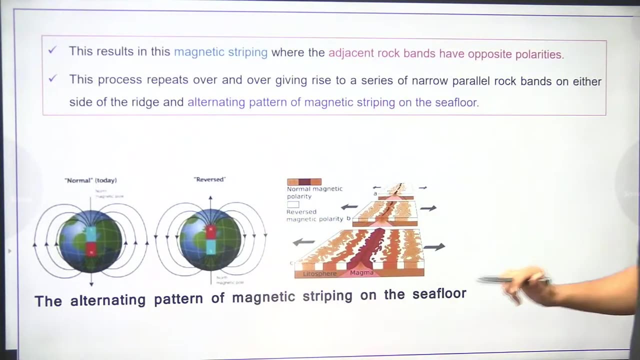 it will accept the polarity of earth and will be inclined in that direction. now, if I tell you what is our earth, you must have understood. curie point is any temperature, I am telling you, after which it accepts the polarity. now let me explain you one thing. see here, the polarity is this: 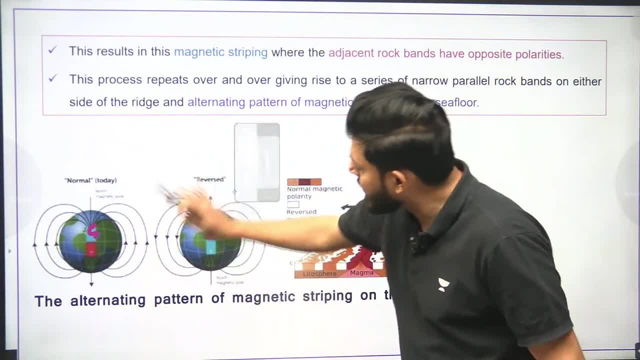 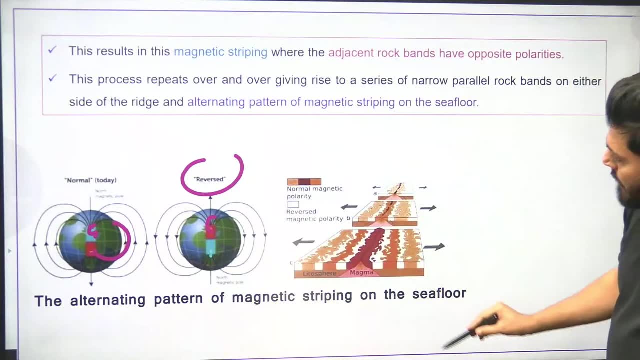 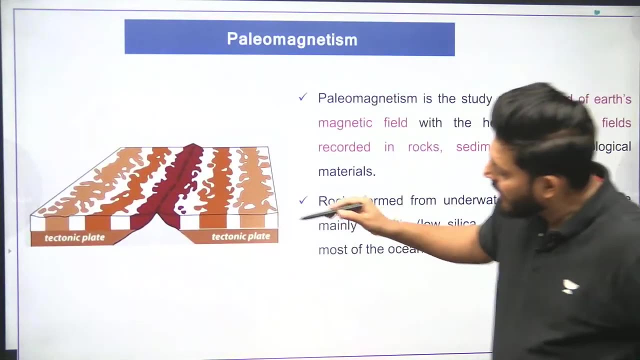 here it is your south pole, here it is your north pole. but after some time it will be reversed. here the north pole will go up and south pole will come down. if you see clearly this is your magma, this mid oceanic, you can say that magma is coming out. 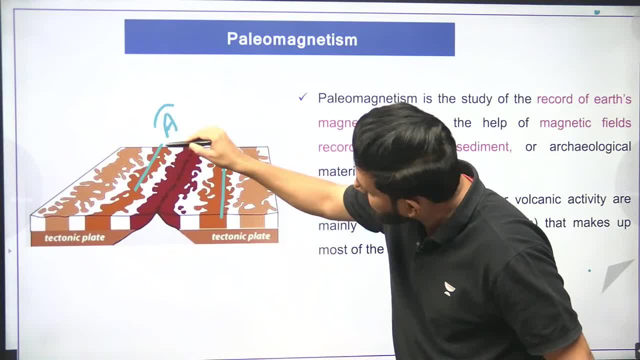 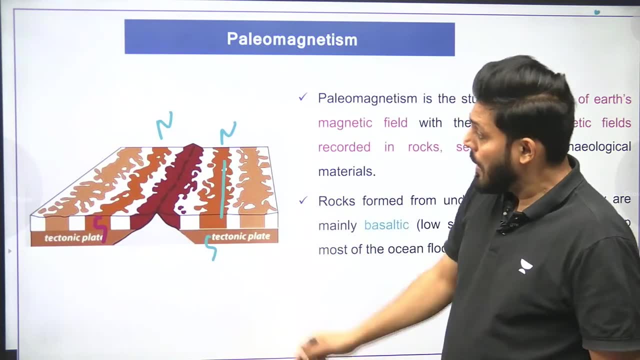 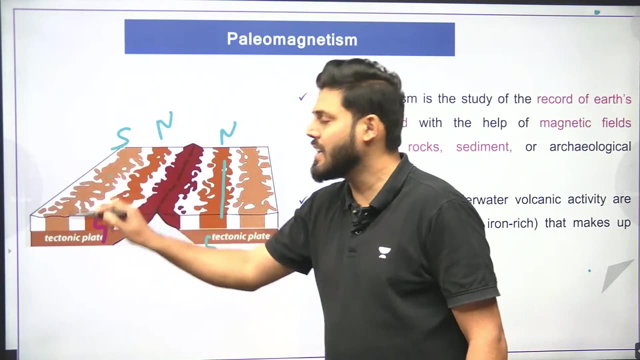 here, the rock which came out at that time, the polarity. this one will be north and this one will be south. then I am telling you, this one will be north and this one will be south, but at that time, what will be the polarity of earth at that time? 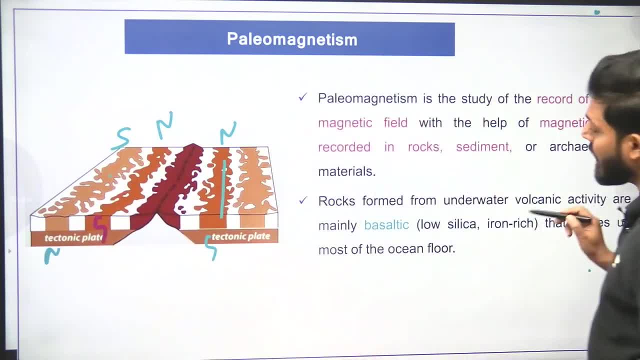 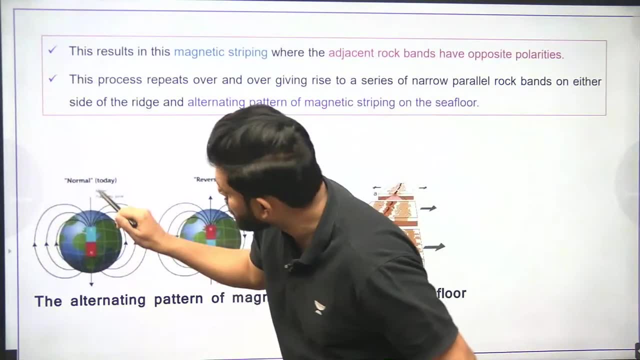 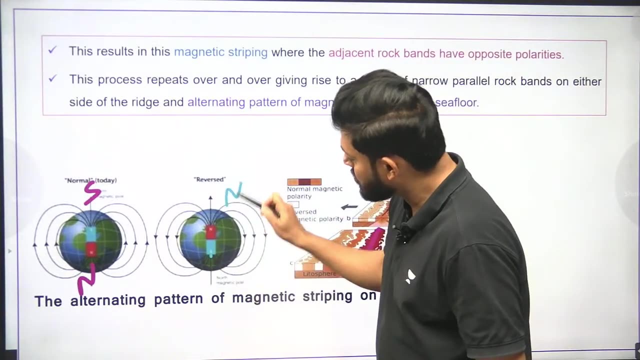 if the polarity of earth is south, then here will be south pole and here will be north pole. then how it will be reversed? how it will be reversed if it is south pole here and here is north pole. after thousands, millions of years it will change and here it will be north. 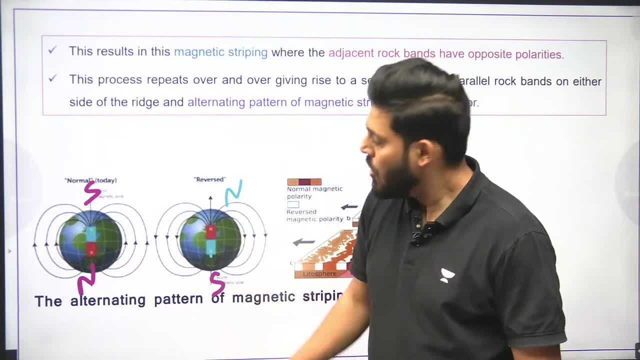 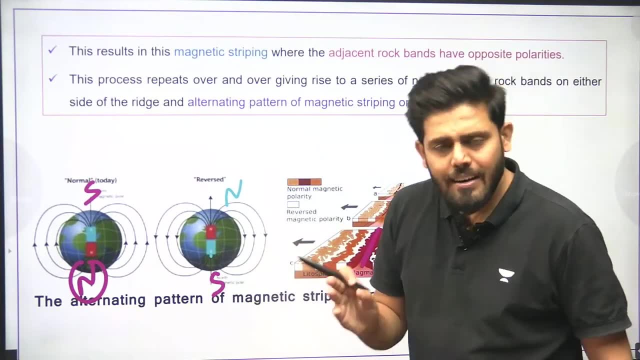 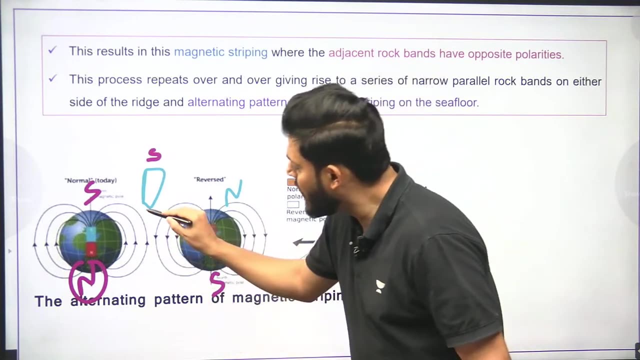 and here it will be south. if here it has south polarity and here it has north polarity and at this time a rock came out from inside and from that curie point its temperature decreased and it became cold, then if you study the sample of rock, then here it will be south pole. 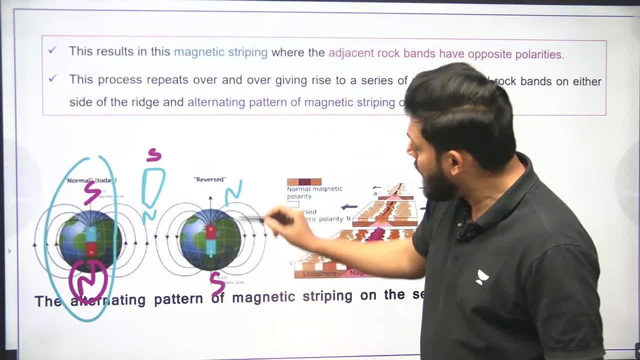 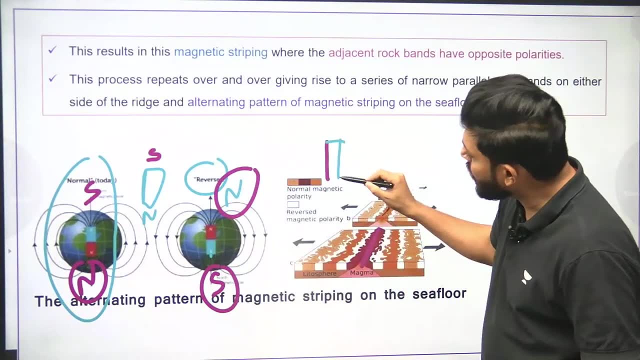 and here it will be north pole, which is south and north pole of earth. now the polarity of earth has been reversed: here is north pole and here is south pole. now the rock which will come out, then its polarity will incline itself according to earth. here it will be north and here it will be south. 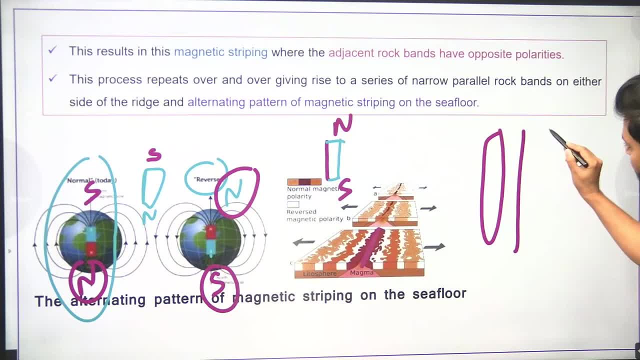 and when we noticed that this rock, this rock is of same age and this rock is of different age. so we saw that it has north and it has south. so it has north and it has south, it has south and it has north, it has south and it has north. 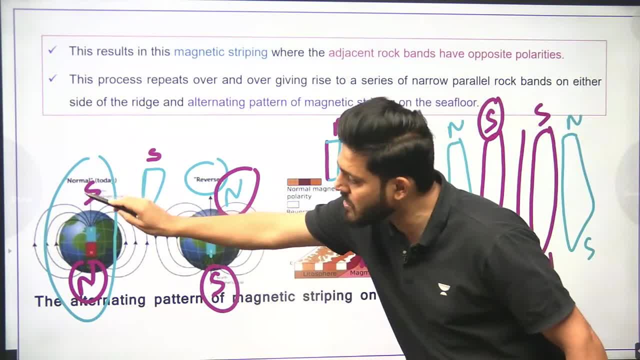 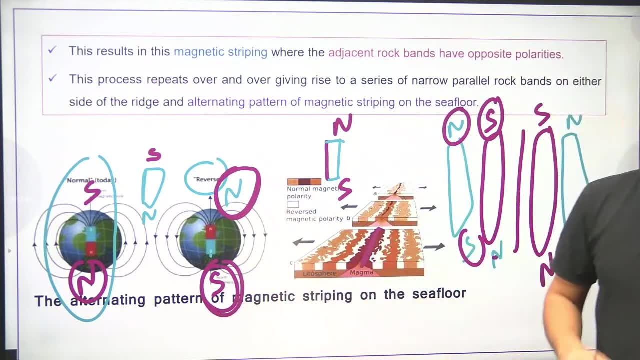 it has south pole and it has north. at that time our earth will have south and north, and at that time our earth will also have north and south. how we came to know this? by studying this rock. when we took samples of this rock, then we got different polarity. 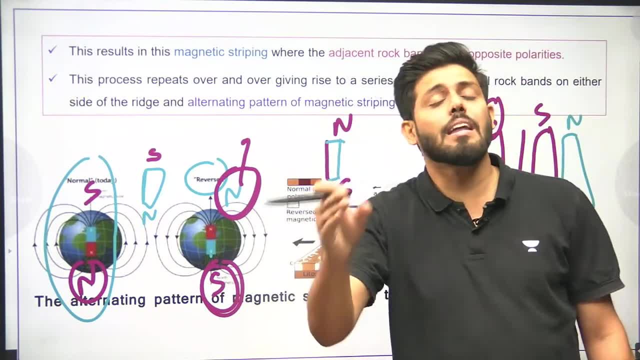 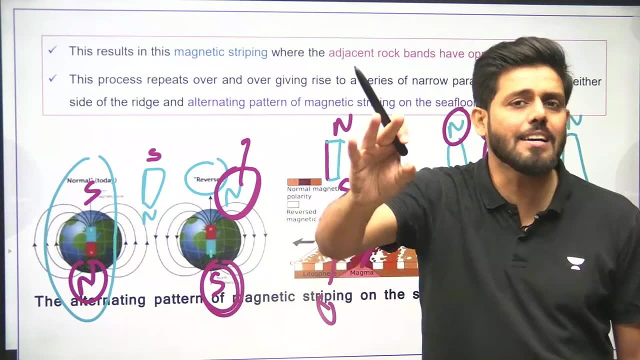 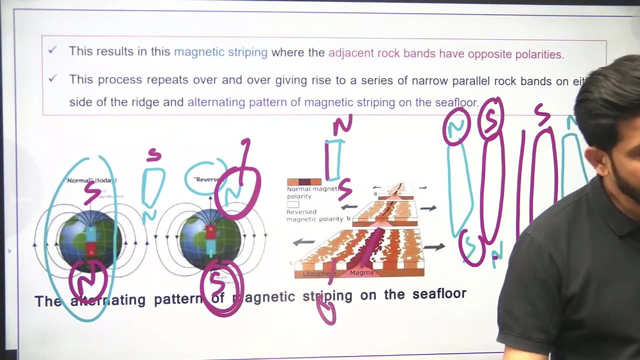 from that we came to know that because of this, the magnetic field of this rock will also be different. geographical north and south pole is a different concept, and magnetic north and south pole is a different concept. did you understand? now tell me how many students were able to cover things. 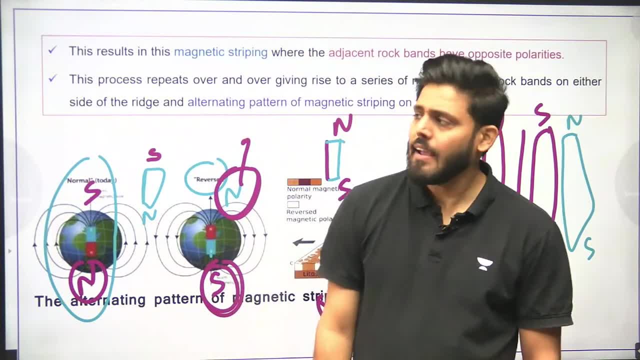 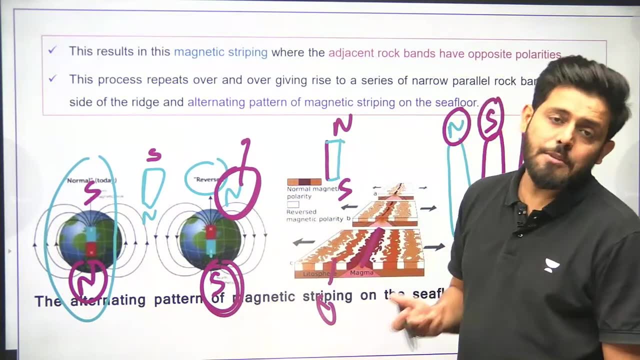 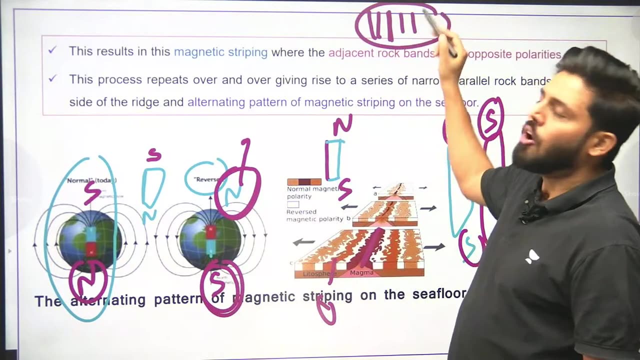 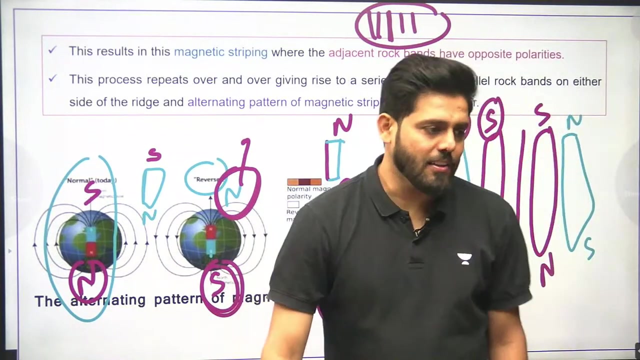 anyone. ok, now let me ask you, sir the wayne and matthews, where did they study things? carlsberg ridge, carlsberg ridge. they took samples of rock on both sides of the ridge in indian ocean and after taking samples, they came to know that their polarity is reversing. 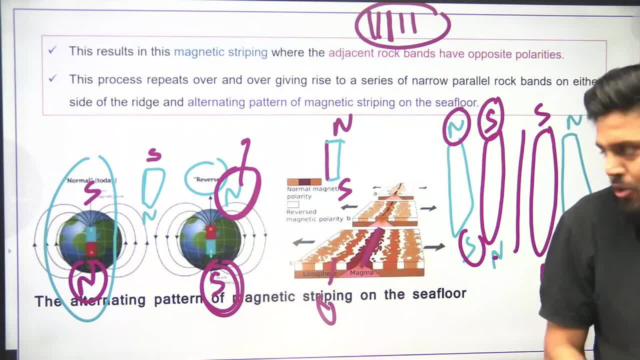 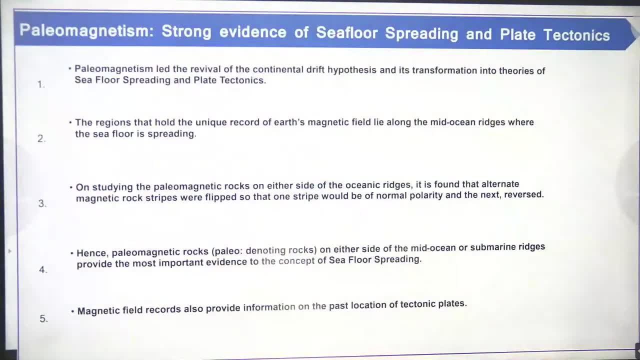 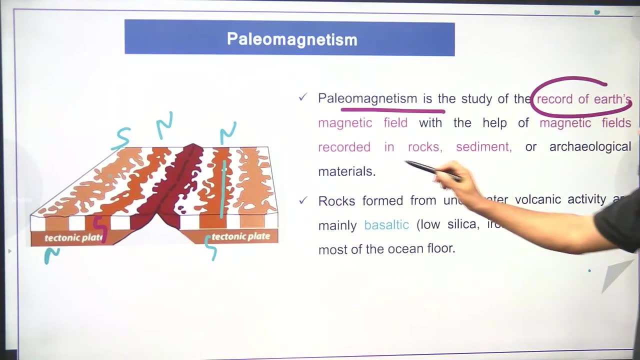 if you have any doubts, then tell me. if you want to study things, then come with me. i am ready to teach you in any way. you should be able to come. let's study the study of record of earth magnetic field. the record of earth magnetic field and with the help of magnetic field, 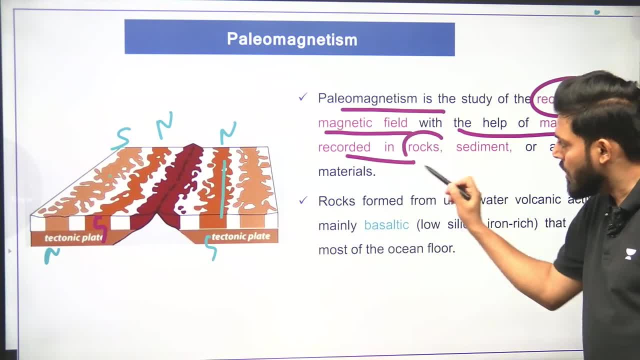 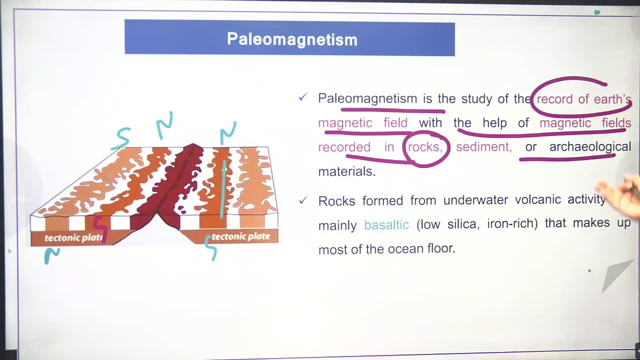 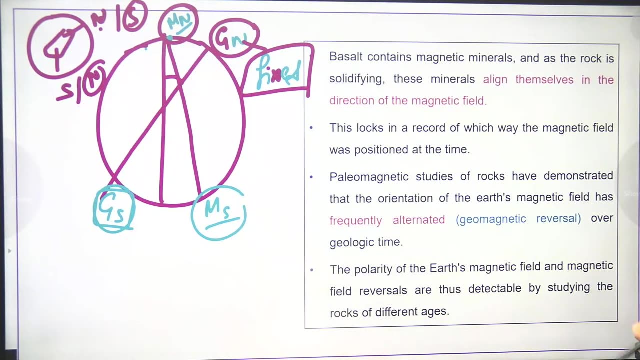 recorded in the rocks, the magnetic field of rocks. when we studied them we came to know from archaeological material the underwater volcanic activities. magma has come out from mid oceanic ridges. when we have seen things from there, we have seen that the magnetic property of rock, the magnetic property of rock. 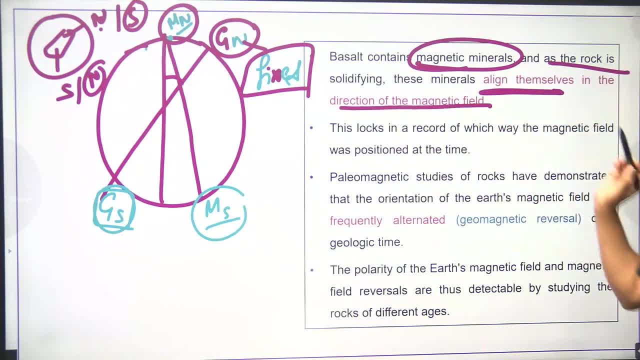 is aligned with the magnetic property of earth. ok, this rock, the record of which way the magnetic field was positioned at that time, due to which we have got a record that the rock of this age, its polarity at that time, what will be the polarity of earth at that time, at that position? 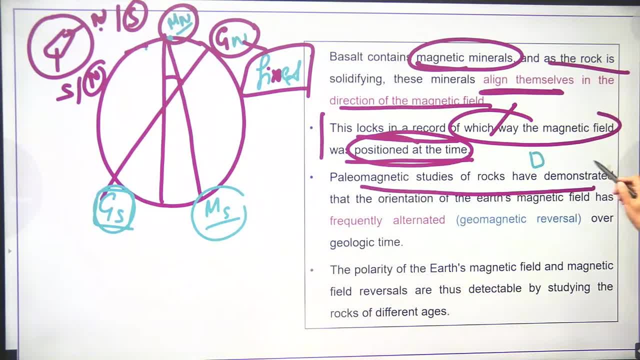 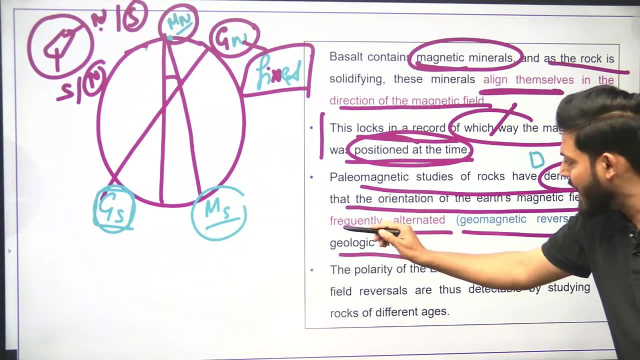 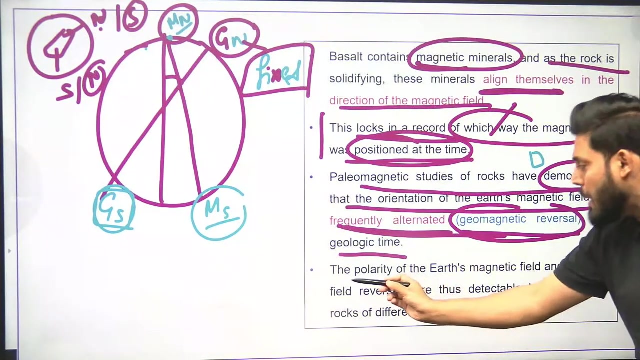 we have come to know from there, understood that the orientation of earth magnetic field frequently altered- geomagnetic reversal over geological time. we came to know that the magnetic field of earth is frequently changing. the geomagnetic field is reversing with time. due to this, the polarity of earth magnetic field 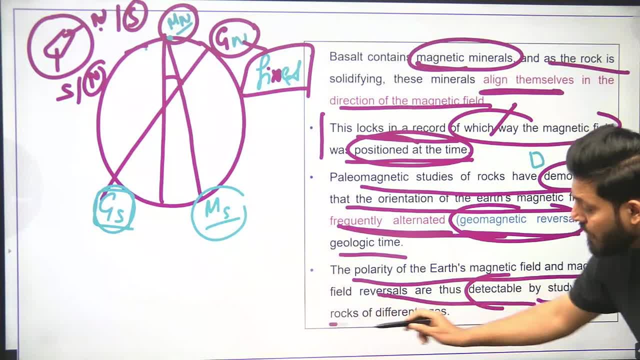 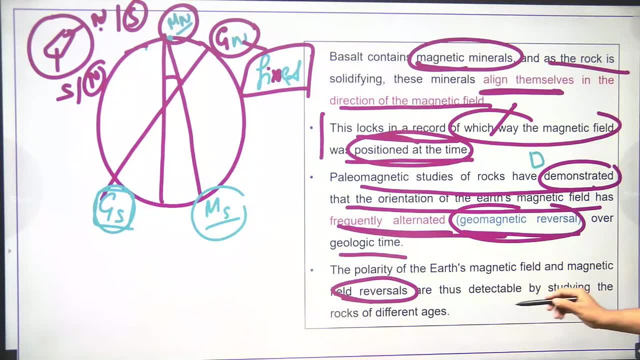 reverse are thus deductible. by studying the rocks of different age. how we came to know that our magnetic field is reversing? when we have deducted at different time of rock, when we have studied the rock at different age, we have seen that the magnetic property of rock is different. 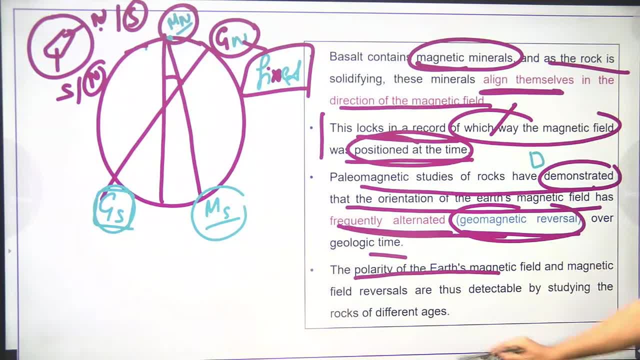 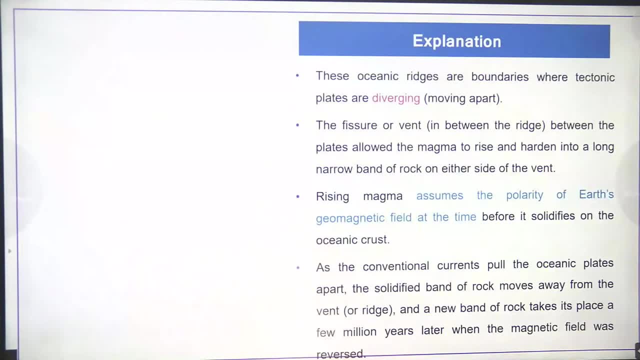 due to which we came to know that the polarity of earth is reversing. we came to know from the rock of earth. you must have understood these things. is it clear, if there is any problem? so this is the reason. the fissure and vent from where the magma is coming. 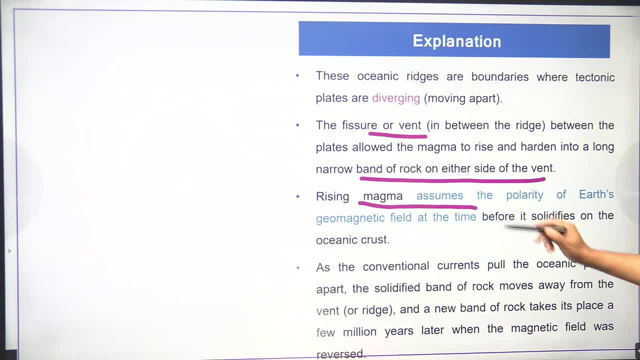 and after that it is solidified on both sides. so we have seen that the rising magma is aligning against the polarity, which is geomagnetic, of earth before it solidifies on the oceanic crust as the convection current pulls the oceanic. so after solidification, 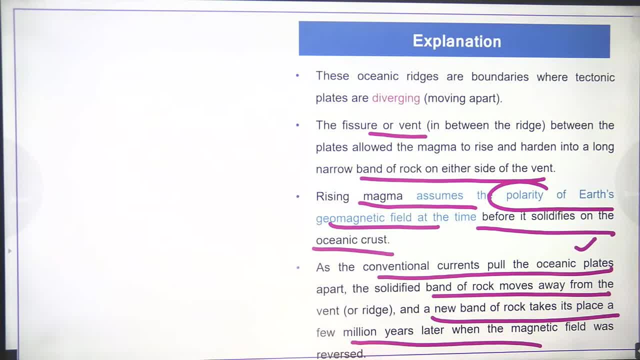 that new band of rock is formed and due to which our magnetic polarity has changed in few millions and thousands of years, due to which our magnetic property of rock has also changed. Carlsberg ridge, which we have studied- the name of that ridge is Carlsberg ridge- 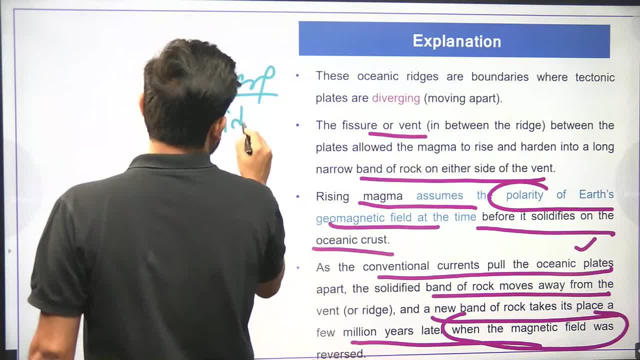 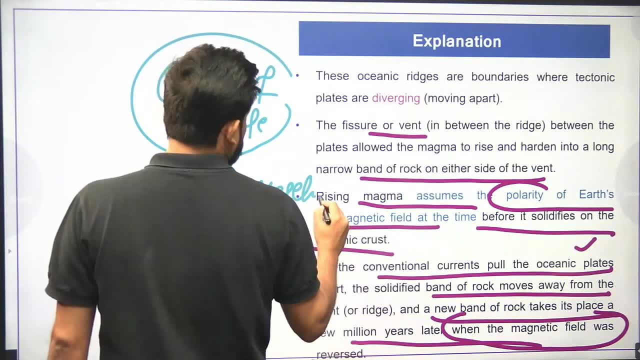 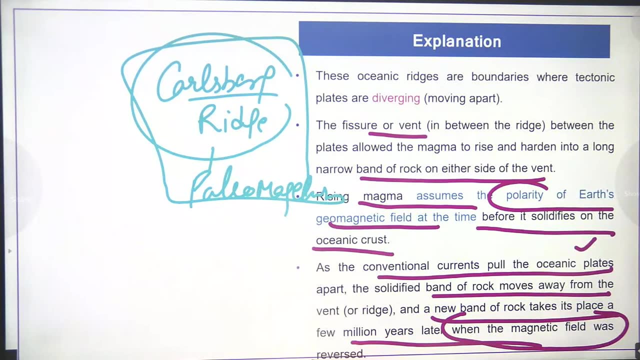 Carlsberg ridge. this ridge is in Indian ocean, where the study of paleomagnetism was done. remember of paleomagnetism. now tell me who all the students got to know about this theory, which I have studied till now. plate tectonic theory is more studied. 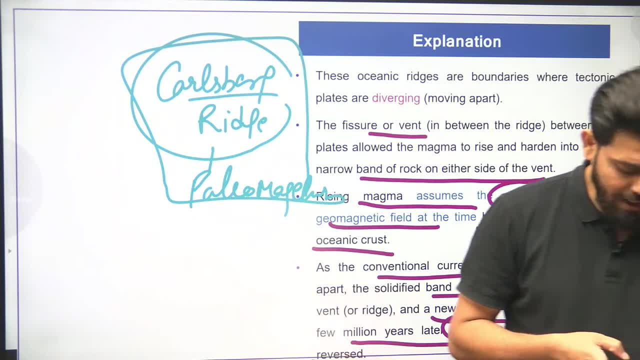 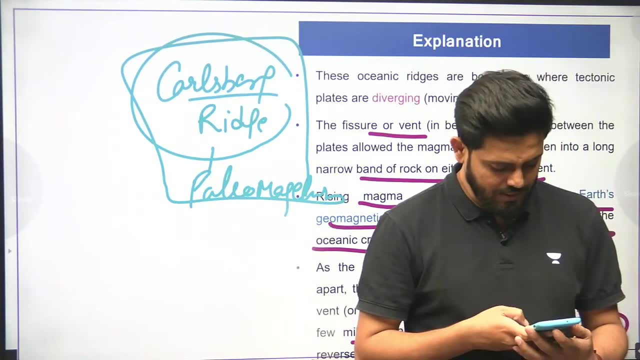 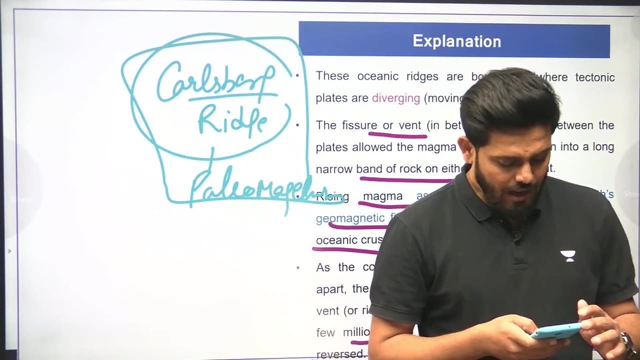 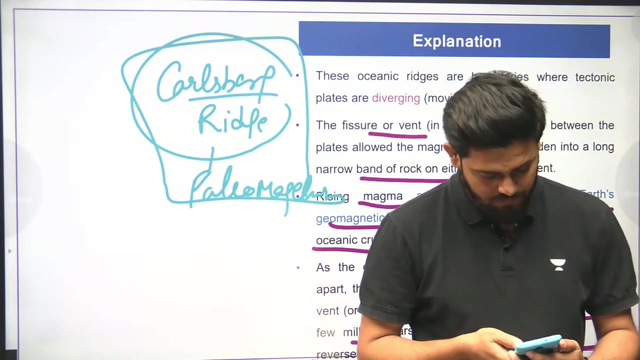 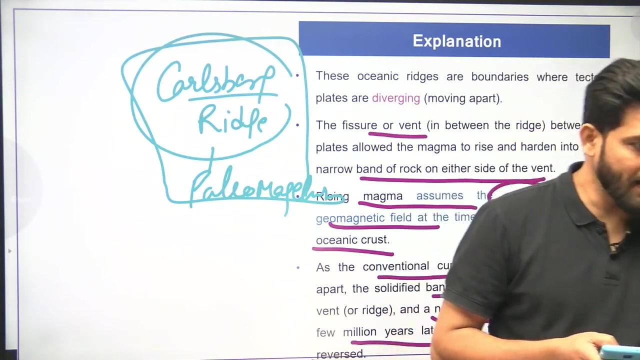 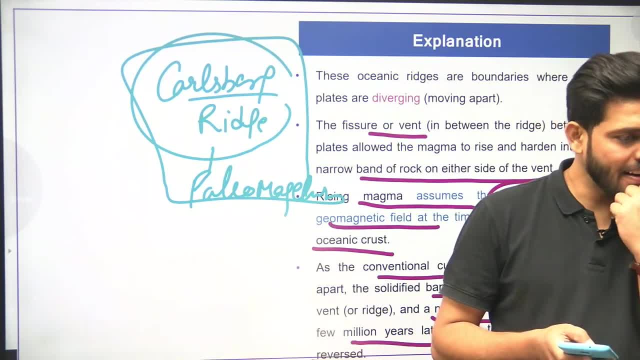 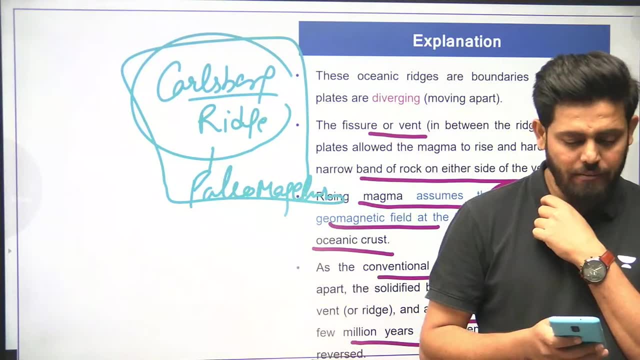 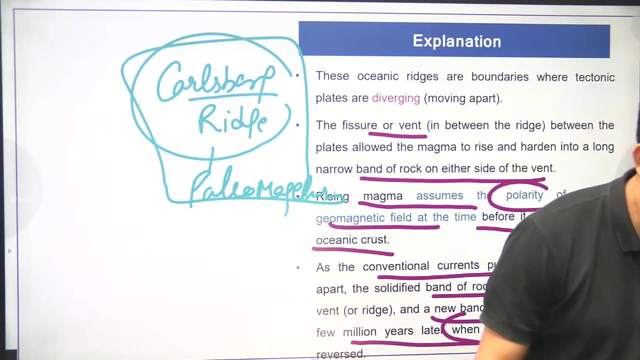 all advance from the beginning. tomorrow we will do plate tectonic theory. it will take half an hour or 45 minutes, or 45 minutes approx. now it depends on you how to do it. tomorrow we will teach plate tectonic theory. we will take a separate session of plate tectonic theory. 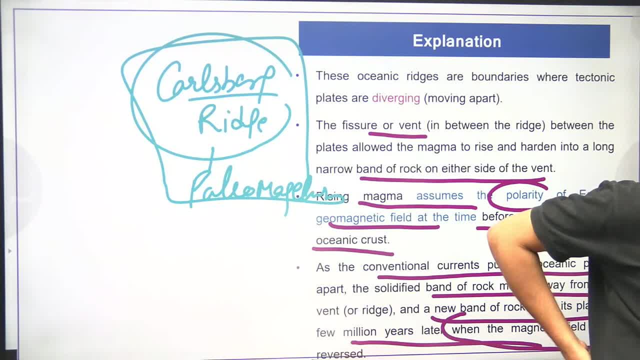 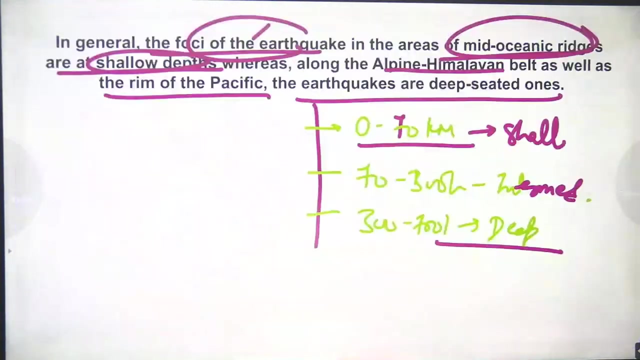 you tell me I am not trying to make the session long, then it will be too long. you know I will go in the flow. there are so many things in plate tectonic theory because I have told you I will explain and show you plate tectonic theory. 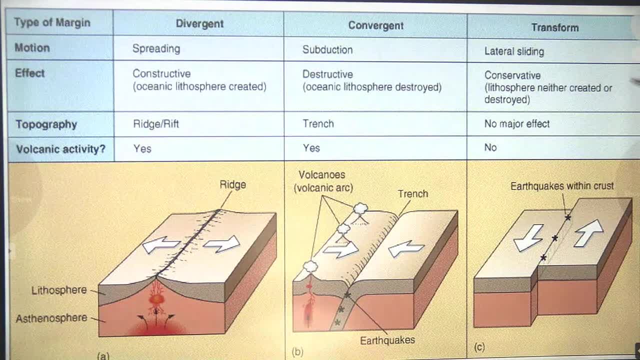 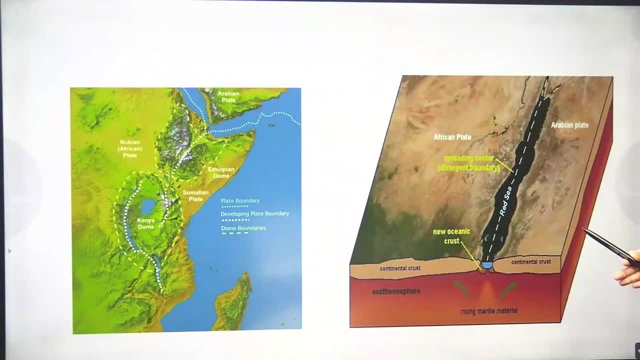 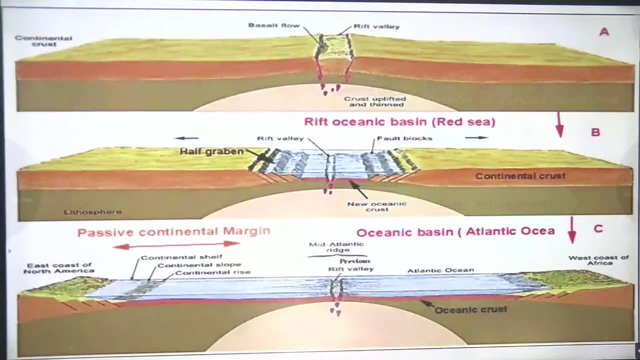 then I will tell you one thing: how different plates are then. who gave? what is convergent and divergent? where trenches will be made? what is san andreas fault? what is mid oceanic ridges? what are trenches? why earthquake came on antolian plate? what are the forces? 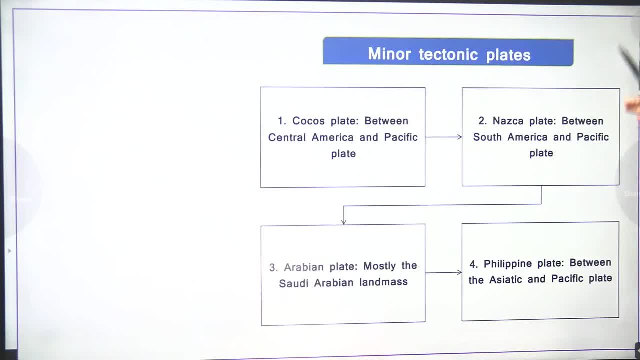 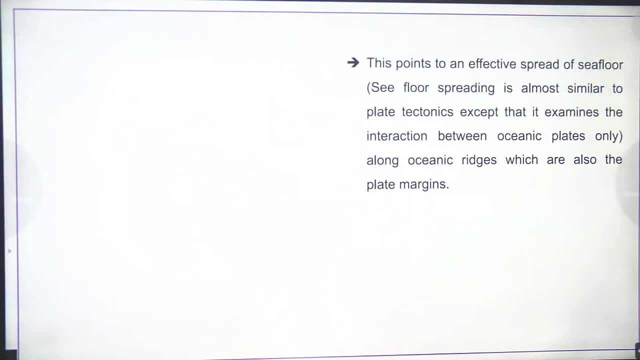 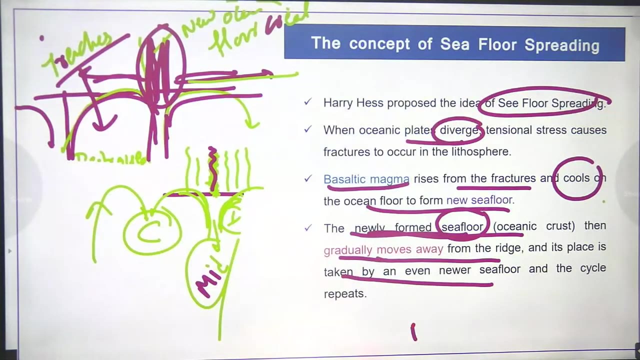 due to which? how red sea formation happened, at what rate plates are moving in specific ring of fire, why earthquakes come more. what is divergence? how indian plate moved, earthquake, volcano eruption. I will tell you about all these things, do you understand? then we will do it tomorrow. 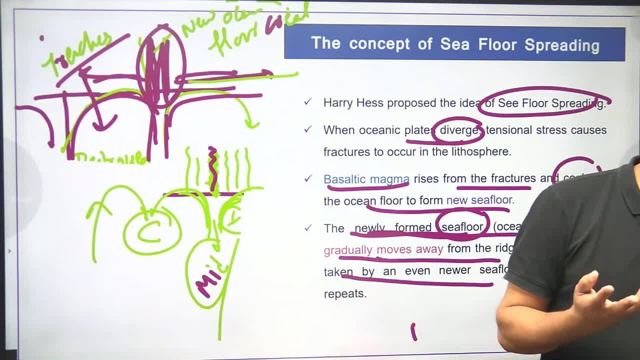 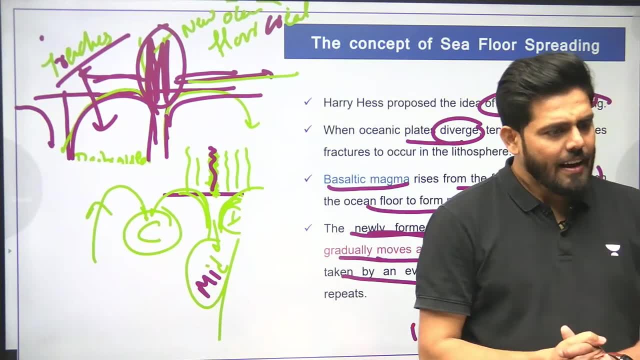 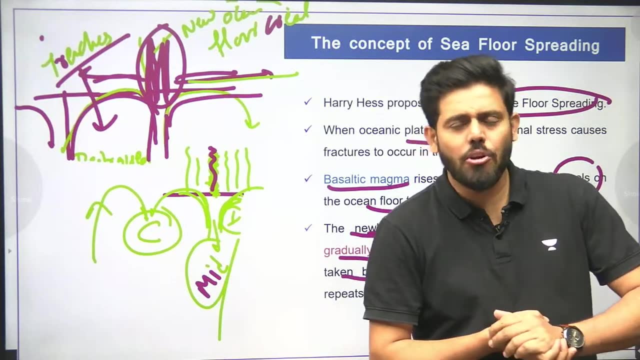 now you must have understood why tomorrow- because it is long, I know that I don't want to pass the time- we will do it tomorrow. tomorrow, we will do it. tomorrow. we will do one thing: plate tectonic theory, and with that we will do MCQ questions. 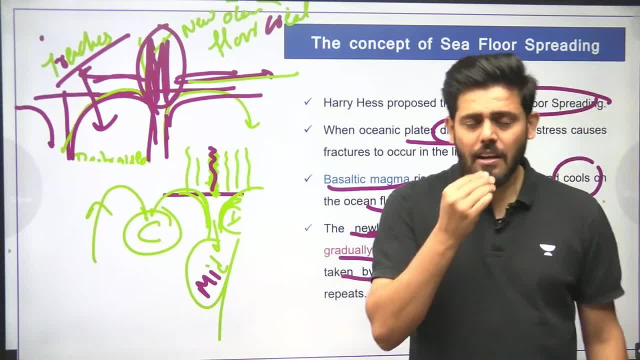 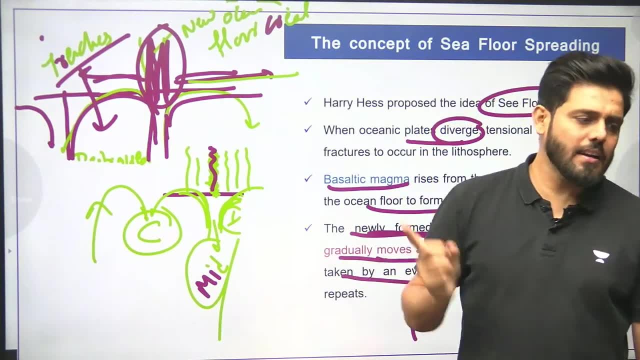 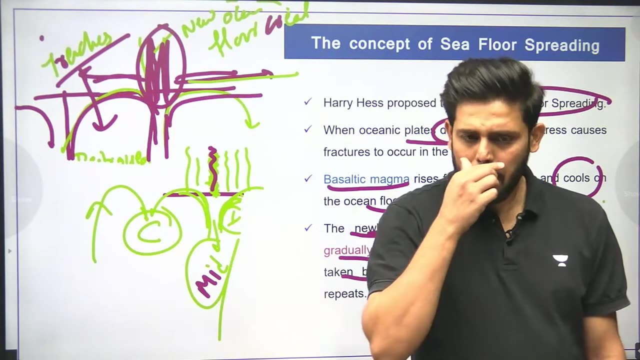 convection, current seafloor spreading, plate tectonic theory and continental drift theory. we will mix 5-7 questions and solve them. ok, things are understood: convection, continental drift theory and one more theory, plate tectonic. everything is understood. anyone has any doubt? 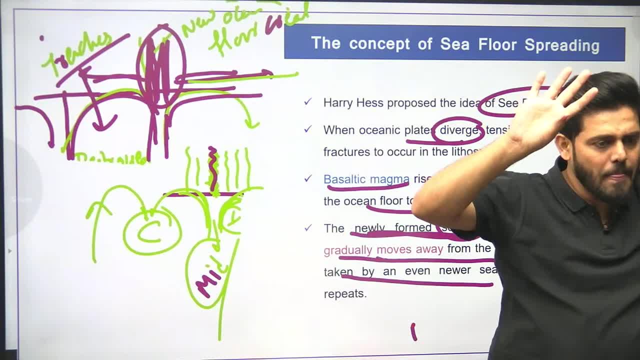 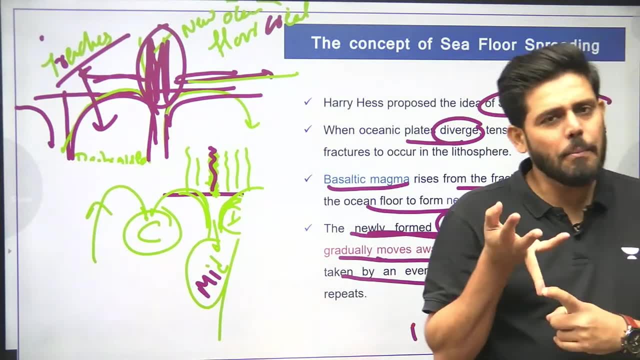 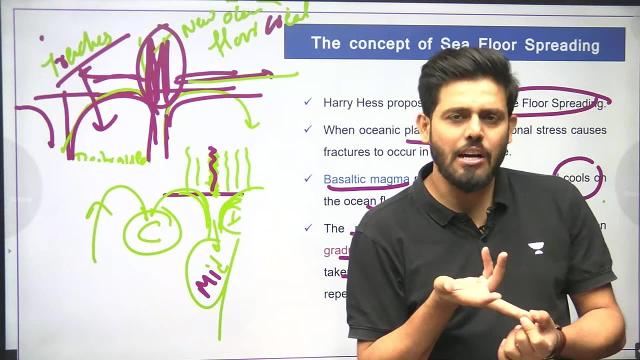 let's take 2-3 minutes. anyone has any doubt, any one of you, about anything about paleomagnetism that we know earth reverses its polarity. seafloor spreading theory: our seafloor spreads where there are mid oceanic ridges, where there is divergence. 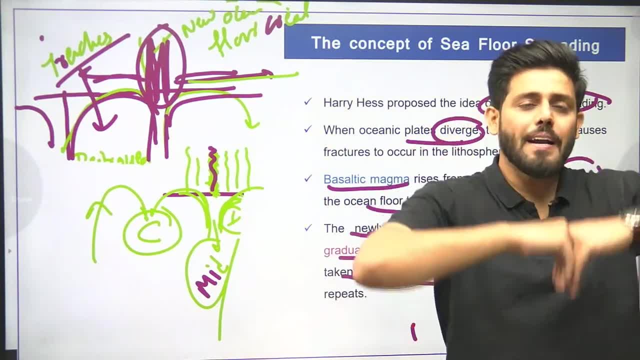 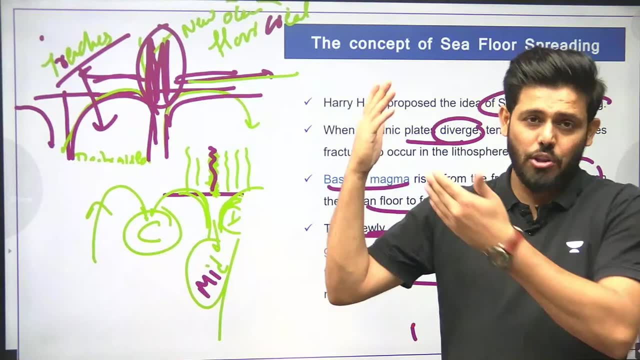 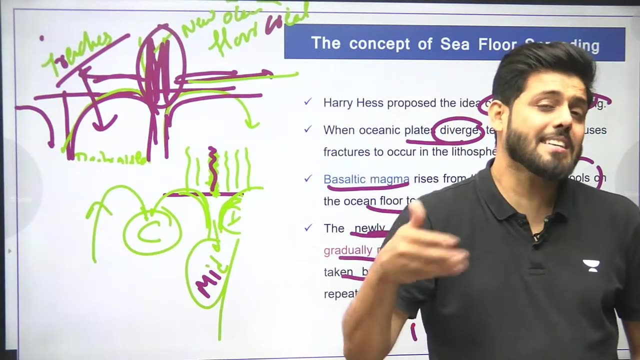 the floor will spread and where there is convergence, where two plates will collide. convection, current theory: our magma is rising, because of which our plate tectonic theory will tell us how our mountains were formed. plate tectonic theory will tell us how mountains and ridges were formed. 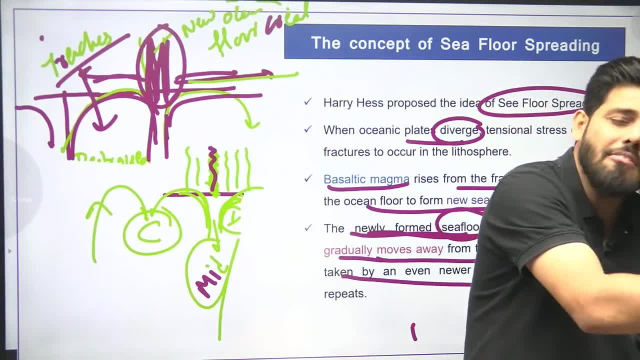 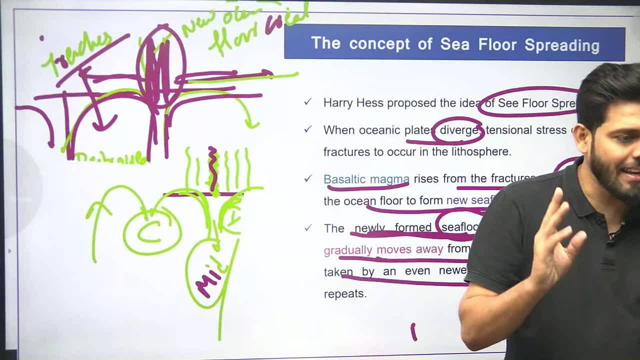 but whose help will it take? it will take help of seafloor spreading theory. it will take help of convection current theory. in 1967, mckenzie parker, wj morgan will talk about them. ok, keep doing things well, just keep this belief. 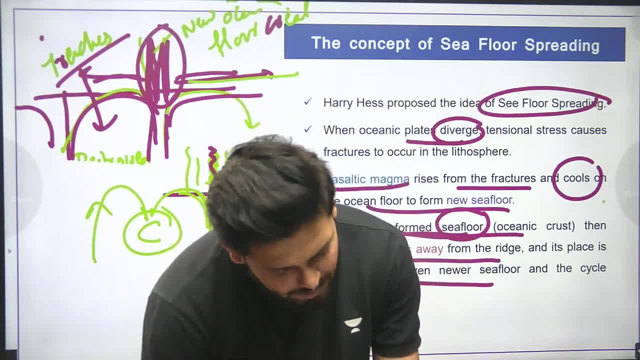 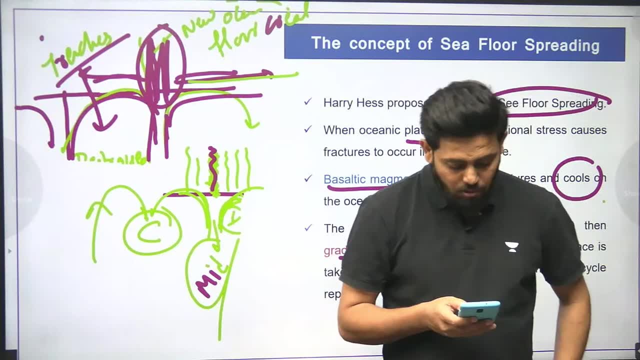 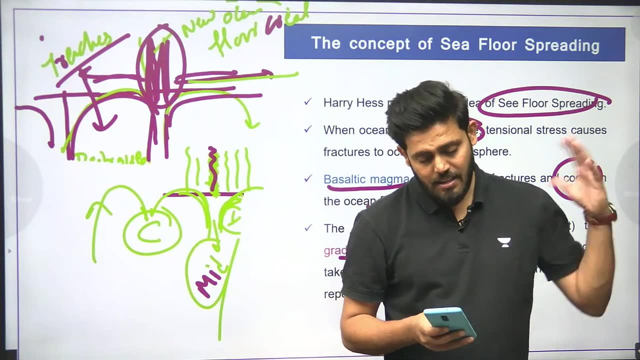 if i have promised that i will complete, please like and share. so i will complete this session, this topic and this course. remember, you will complete it for 2 months. i will cover you very well with points, what to do with each thing, how to do. they will cover it well. 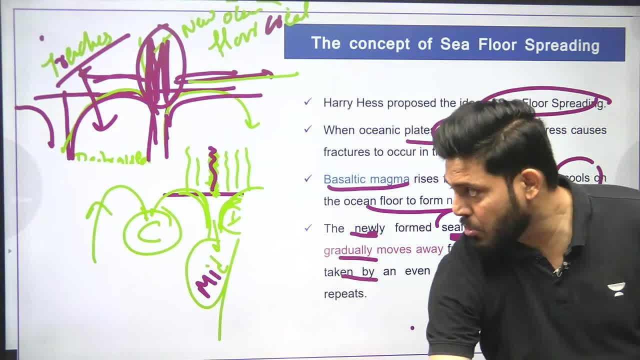 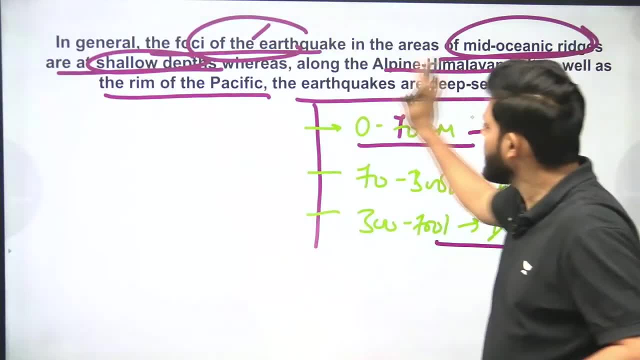 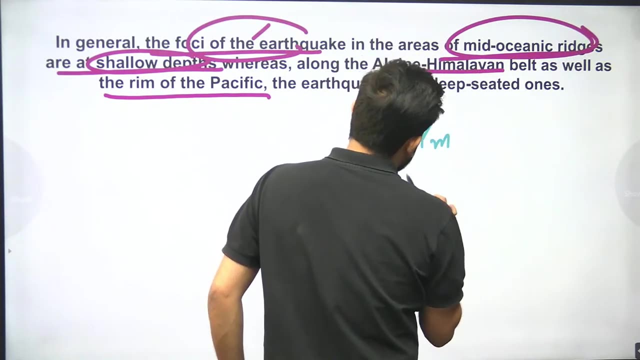 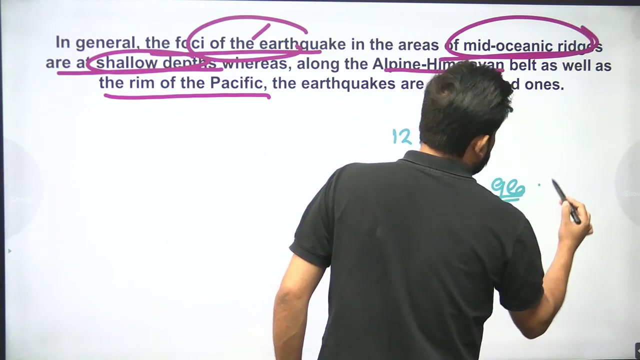 don't worry about that. we will read daily: what are the things? what are the things? come? let's understand. first of all, our daily 12 pm. our course is free course called sankalp mentorship program. sankalp mentorship through geography mc. through geography mc questions. 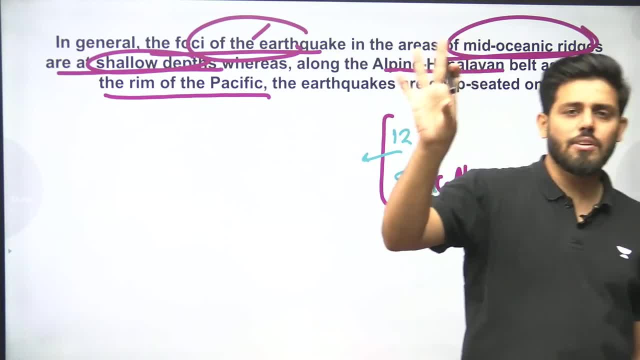 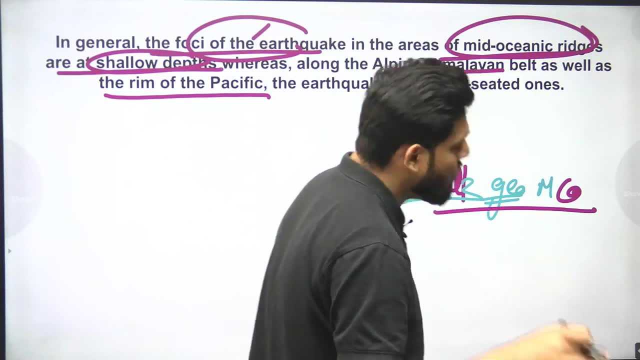 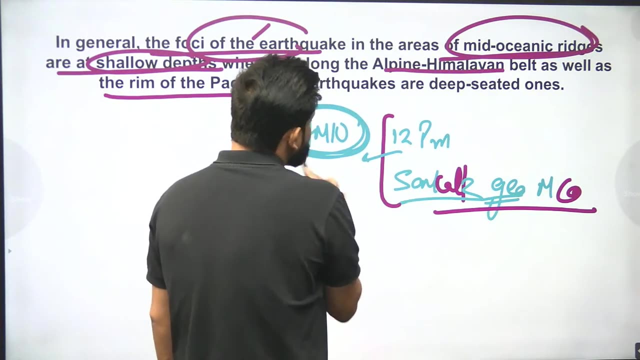 i am providing free mentorship and all the 5-6 students who have done top till now have been given mentorship. you can ask me. i think no one has missed. ok, so all the 12 pm students you can join using am10 code on the app. 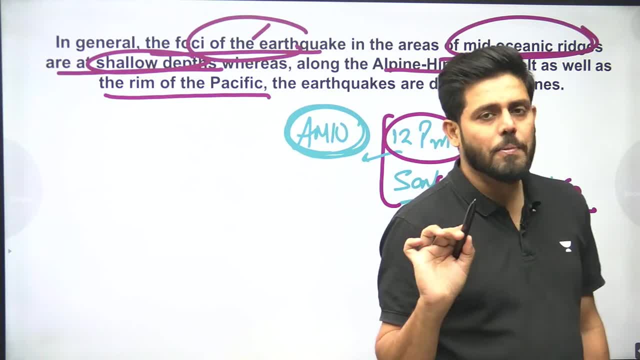 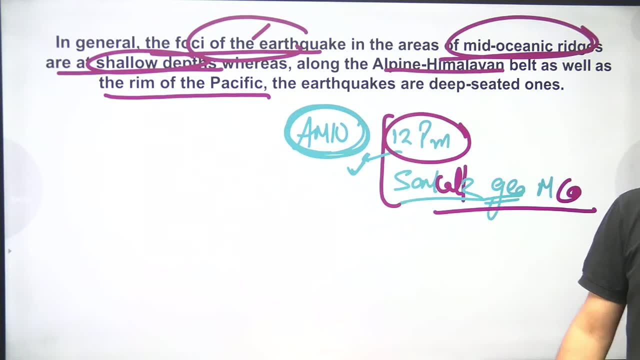 daily. my afternoon is at 12 pm. all the students who do top in this session in questions, i provide them free mentorship. those students who can't afford: that's why i have launched this course and very quality mc questions are covered here on afternoon, 12 pm.